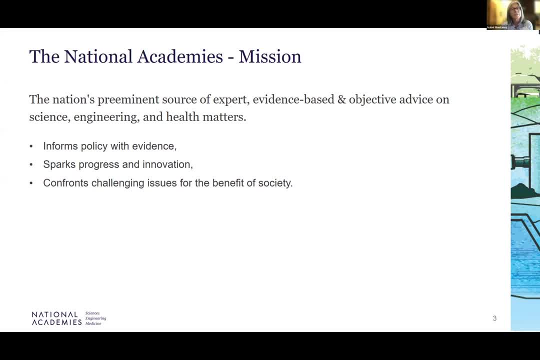 arm of the National Academy of Sciences aims to be the nation's preeminent source of expert, evidence-based and objective advice on science, engineering and health matters, And the NAS and its boards provide a neutral convening body that supports the use of scientific research for evidence-based policymaking and to 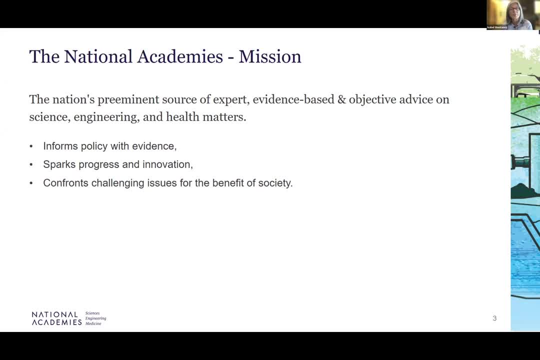 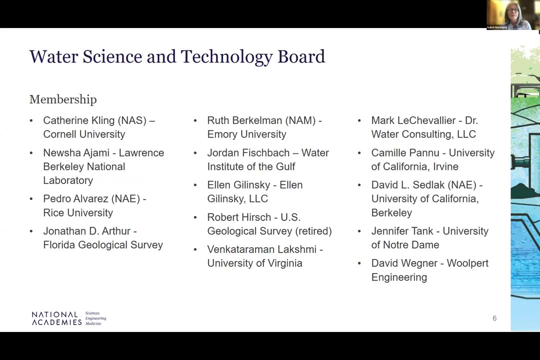 recruit scientific and technology specialists to participate in advisory work and confronting challenging issues for the benefit of society. Next slide: The Water and Science Technology Board is chaired by Kathy Kling, As I mentioned, of Cornell University, and consists of a board of volunteers that span a broad diversity. 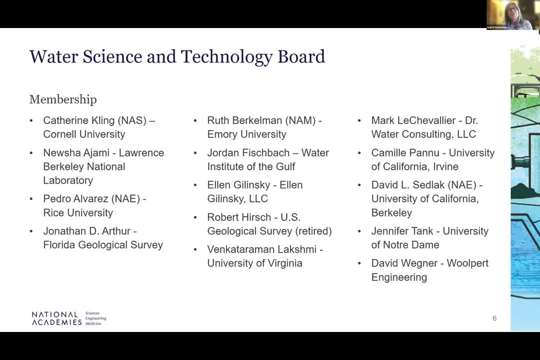 of expertise and backgrounds And I invite you to look through the agenda booklet for the members' bios. This board is the National Academy's focal point for activities and issues related to water science and resources, including surface and groundwater aquifers, and ecosystem restoration. 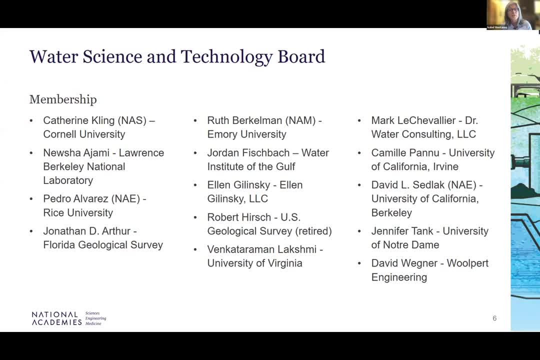 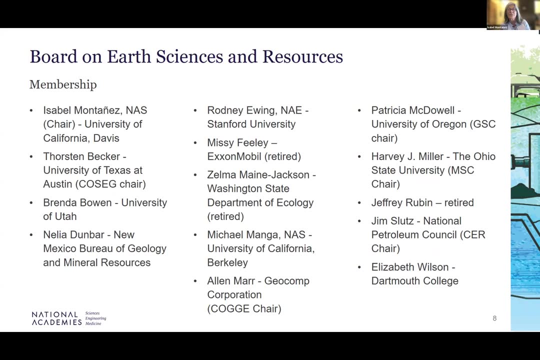 and management: water infrastructure systems, water reuse, wastewater and water resources. They are responsible for the correct diversifying and management of the geographic, geologic and geospatial mapping and modeling. geological and geotechnical engineering. carbon sequestration and the energy transition: strategic directions for earth science research. 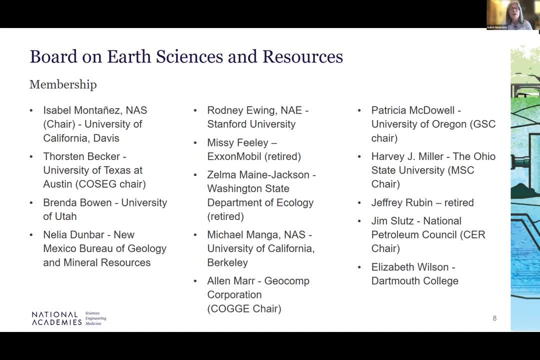 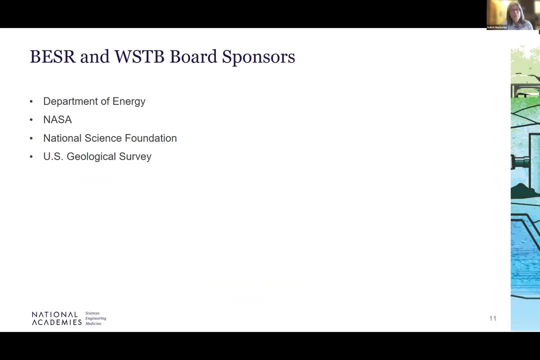 the intersection of geology and health, and environmental justice and equity in earth science, and education and workforce development. Dr Deborah Glickson oversees as director of both of these boards. Next slide, please. The funding sources for both boards are diverse and showcase. 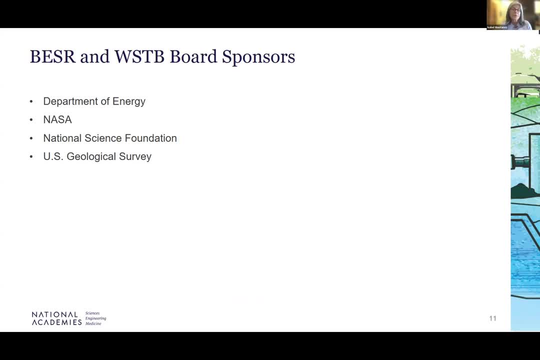 the breadth of earth sciences. Core funding is currently supported by the Department of Energy, Chemical Sciences, Geosciences and Biosciences Division and Basic Energy Sciences, NASA's Earth Surface and Interior Focus Area, NSF's Division of Earth Sciences in the Geosciences Directorate. 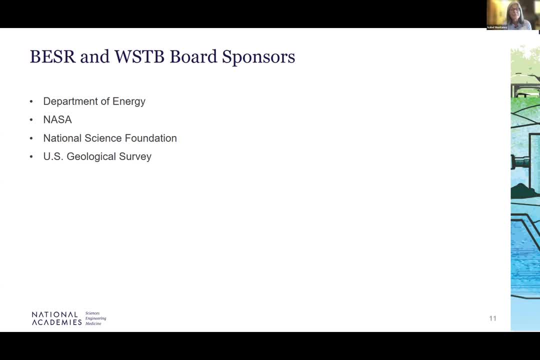 and the Chemical Bioengineering Division. The deal focuses on engineering environmental and transport systems in the Engineering Directorate. United States Geological Survey. Core Science Systems is one of our sponsors. energy and mineral resources and natural hazards- Next slide, please. So today we'll be discussing the current and emerging issues in managed aquifer. 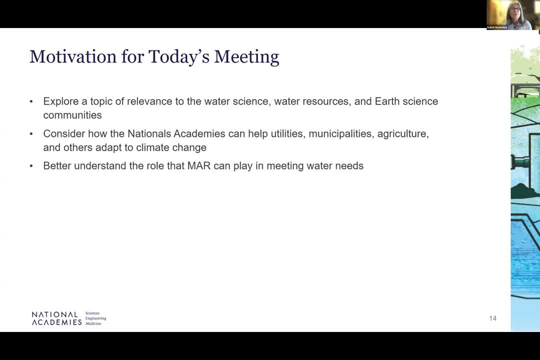 recharge in the US, a topic of great relevance to the water science resources and earth science communities. Assessing how the National Academies can help utilities, municipalities and agricultural sectors and others in the efforts to adapt to climate change and its impacts. 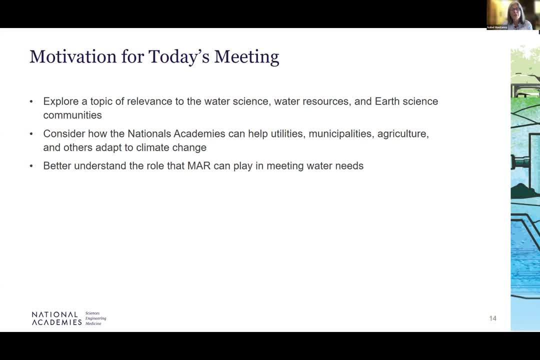 And we aim to better understand the role that managed and aquifer recharge can play in meeting water demands in the US over the next 30 to 50 years. Next slide, please. You'll find the agenda for the two-day meeting in the booklet. 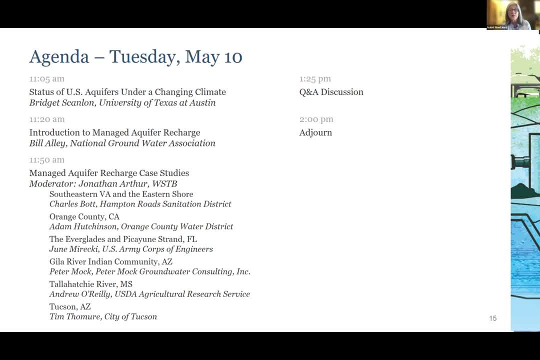 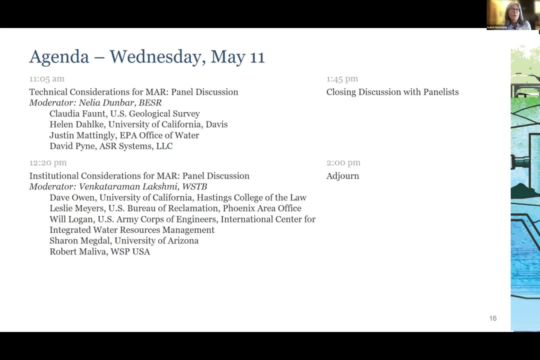 Today we'll start with two speakers who will address the status of US aquifers under climate change and an introduction to managed aquifer recharge, followed by a series of case study presentations, And the second part of the meeting- if I can go ahead and give me the next slide, please- will be held tomorrow. 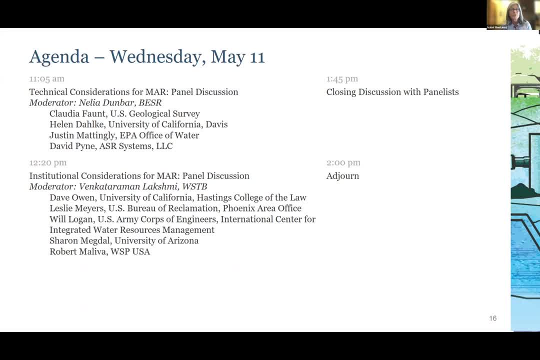 We'll include two panel discussions on the technical and institutional considerations for the managed aquifer recharge And, for today, we may have time for a question or two. following each of the first, We'll include two speakers who will address the status of US aquifers under climate change and an introduction to managed aquifer recharge. 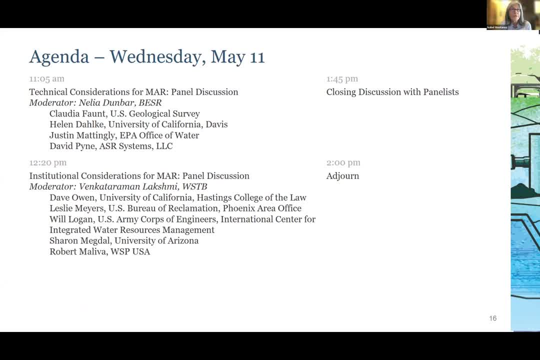 We'll include two speakers who will address the status of US aquifers under climate change and an introduction to managed aquifer recharge, But otherwise questions from the audience, the board and these responses will be addressed in the Q&A function following the case study presentations. 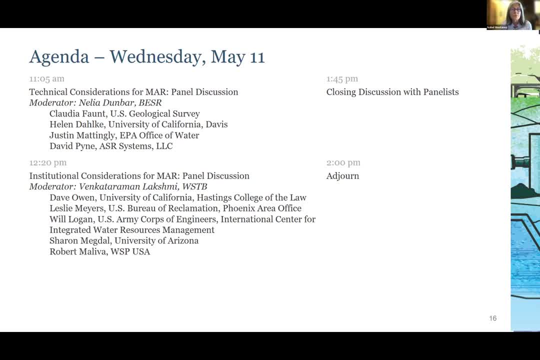 So please enter your questions into the Q&A function of the Zoom meeting. Note that the webinar is being recorded, so any questions you submit may be read aloud and will be included in our recording, And a link to the recording will be posted on our website. 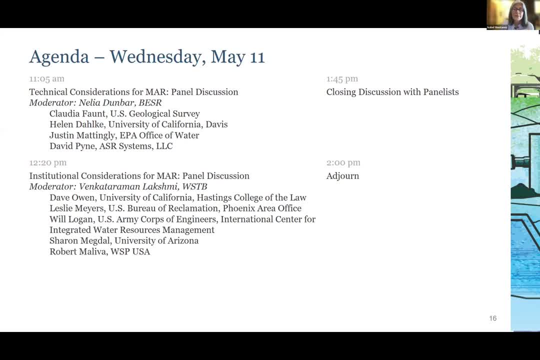 All right, So now I would like to. I would like to introduce our first speaker, Bridget Scanlon, who is a senior research scientist at the Bureau of Economic Geology in the Jackson School of Geosciences at the University of Texas at Austin. 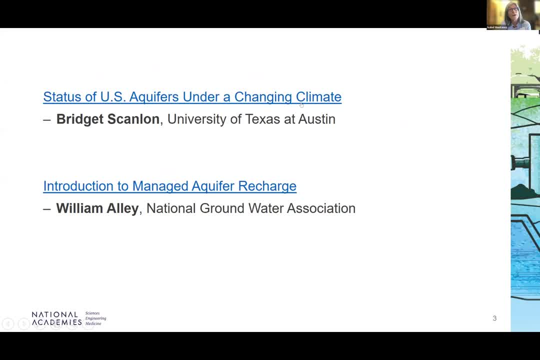 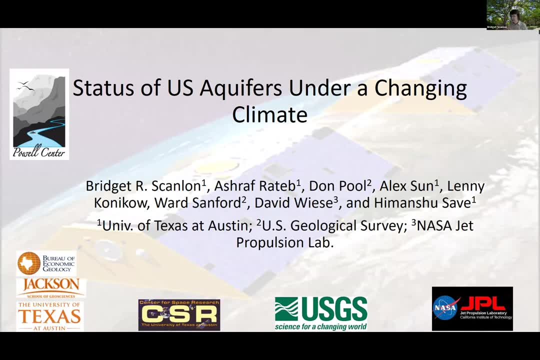 Bridget is a member of the NAE and has conducted research on groundwater recharge across regional to global scales. I'm going to turn the screen to you, Bridget. Thank you. Okay, Thank you so much, Isabel. I really appreciate the opportunity to talk a little bit about recharge at the beginning of this session. 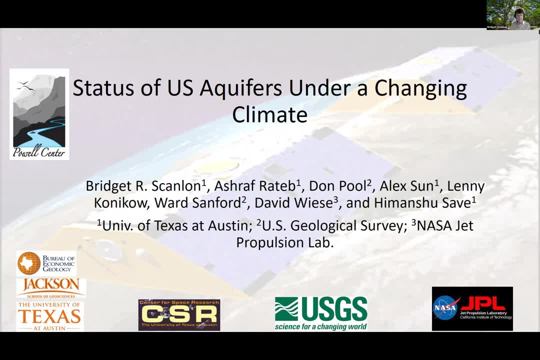 And I was asked to discuss the status of US aquifers under a changing climate. So I'm going to talk about what we did under the Powell Research Group with the USGS. that involved NASA and USGS and academic researchers, and some of them listed here. 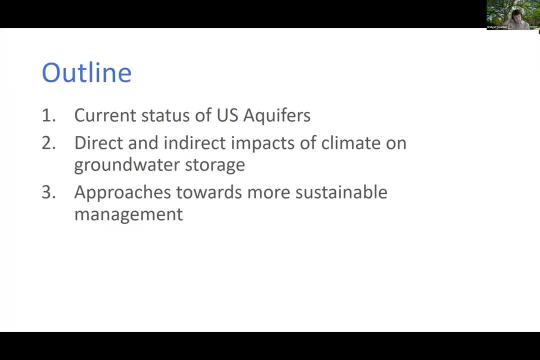 Next, Next slide. So I'll talk a little bit about the current status and provide some background on the US aquifers and depletion that has occurred to date, And then consider both the direct impacts of climate change and indirect impacts through changes in groundwater pumpage and other processes. 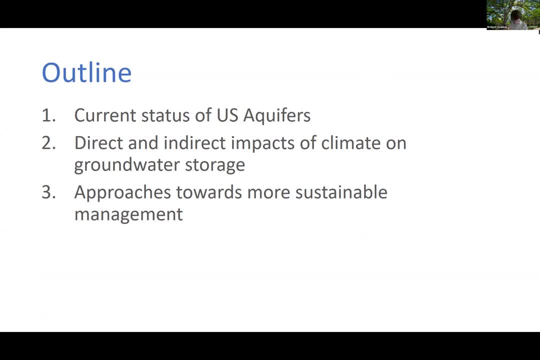 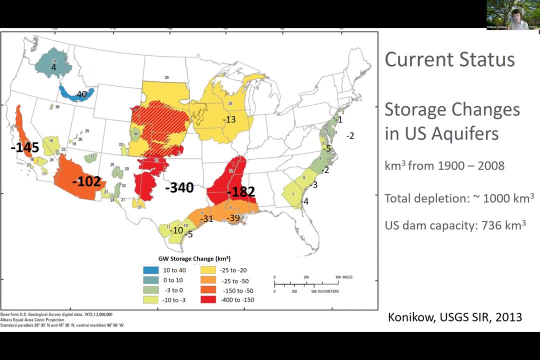 And then how we might be able to move towards more sustainable management. Next, So Lenny Conoco did a fantastic job, Thank you. So Lenny Conoco did a fantastic work on compiling data from regional models and monitoring data of the aquifers throughout the US. 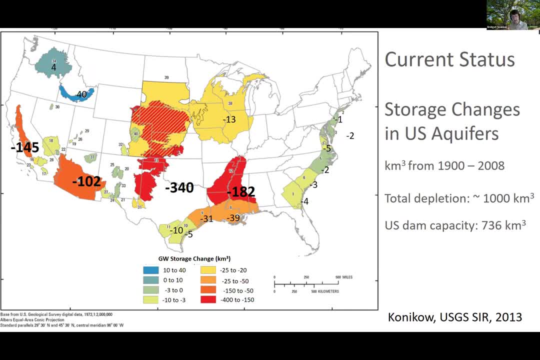 And this represents the results of his analysis based on data from modeling from 1900 to 2008.. And he estimated a total depletion of about 1,000 cubic kilometers And this represents a large subsurface reservoir that we could use. And this represents a large subsurface reservoir that we could use for storage for managed aquifer recharge. 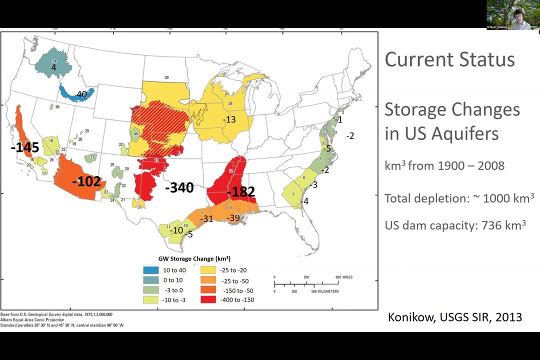 And that compares to current US dam capacity of about 736 cubic kilometers. So here you can see that Dr Conoco identified large depletion in the Central Valley in California: 145 cubic kilometers. Arizona alluvial basin is 102.. 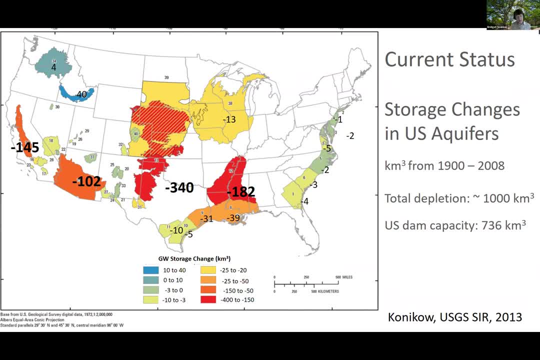 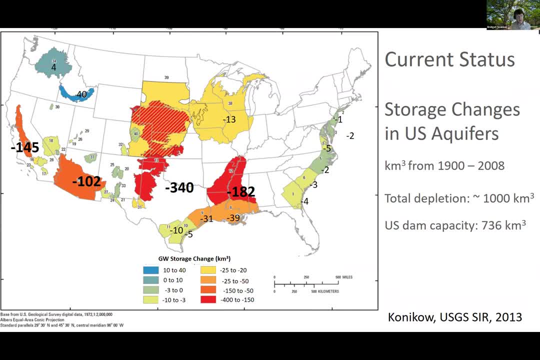 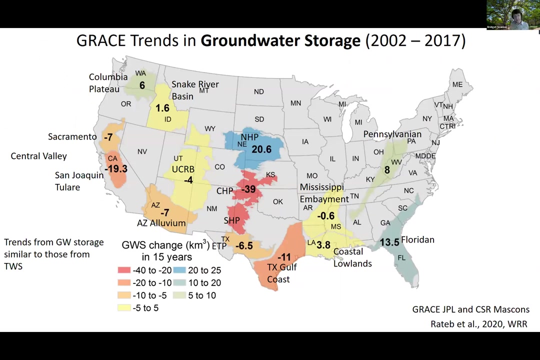 And the Mississippi alluvial basin 145.. And the Mississippi alluvial basin 145.. data for the first mission based on 15 years of data, 2002 through 2017, and Ashraf Rata published this work in Water Resources Research. 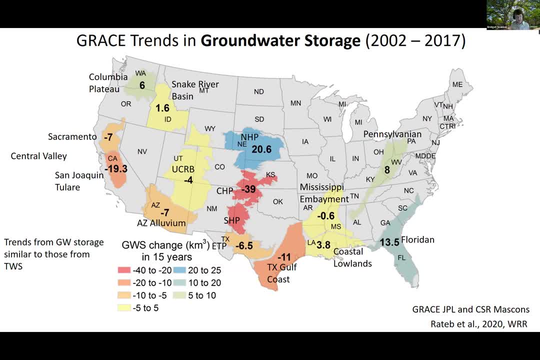 So over this much shorter timeframe. then you can see depletion in the reds and yellows in the Southwest and South Central US: about almost 30 cubic kilometers in the Central Valley, slight depletion in Arizona and for almost 40 cubic kilometers in the Central. 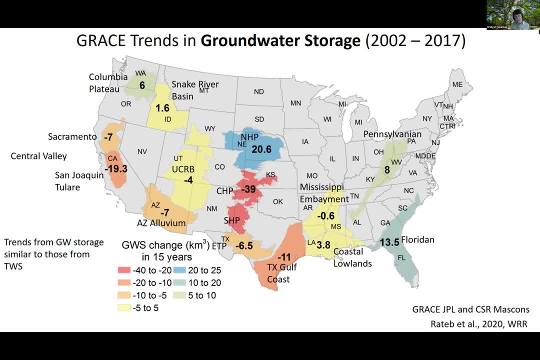 and Southern High Plains. The yellow areas show very little change in storage within the uncertainty envelope for the GRACE data in these basins of upper Colorado and the Mississippi and then slight rise in storage in the Columbia and slight rises in storage in the humid Eastern US Pennsylvania. 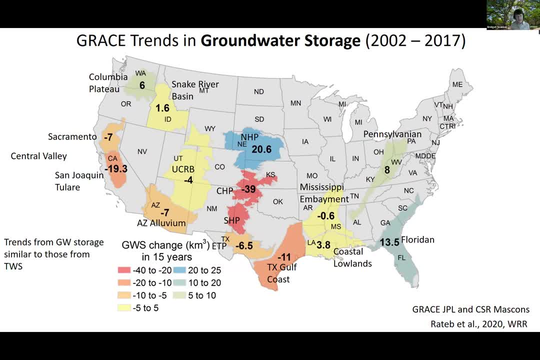 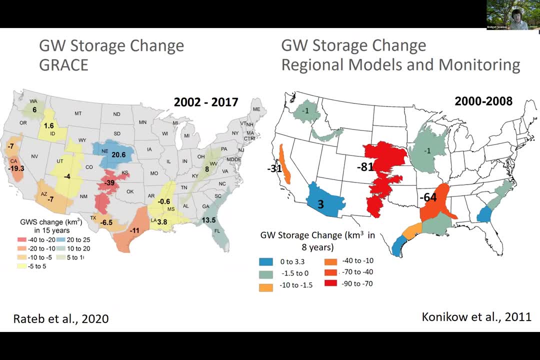 and Florida aquifer systems- Next slide. So if you look at the data, you can see that the data is very similar to the data in the Mississippi. If we try to compare, we don't have data for the same time periods. The GRACE data are shown on the left and Kanako's results for a much shorter time period. 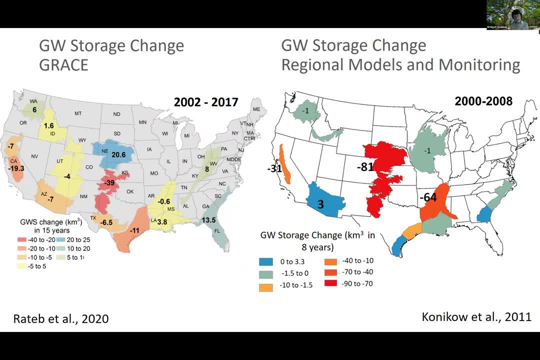 2000 through 2008,. are shown on the right And most basins there. they generally correspond, but the biggest discrepancy is in the Mississippi Alluvial Basin, where the GRACE data suggests very little change in storage, and the regional 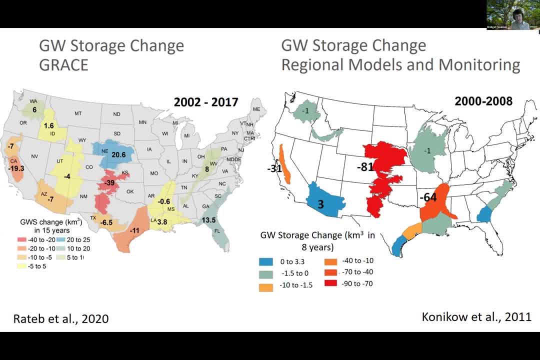 model suggests minus 60 cubic kilometer decline over this time period, And so we were working with the USGS on this study, and so they think that their regional model may not be accurate enough and may not allow capture of surface water storage, And so they're revising that model now. 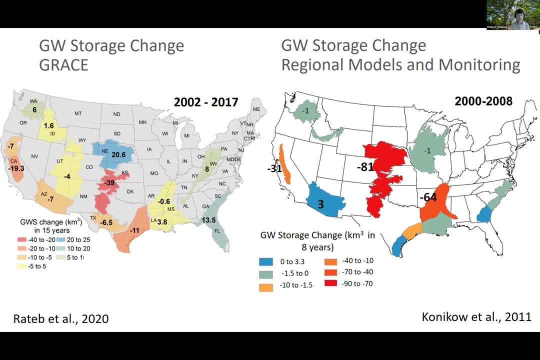 And so, even though a lot of hydrologists are allergic to GRACE data because they think it's too coarse resolution, I think it's just another data source that we need to look at when we're evaluating these systems. We can't ignore it. 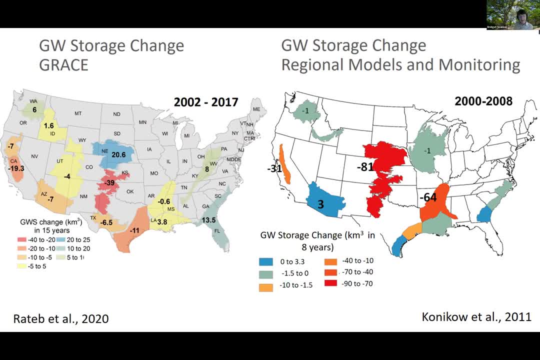 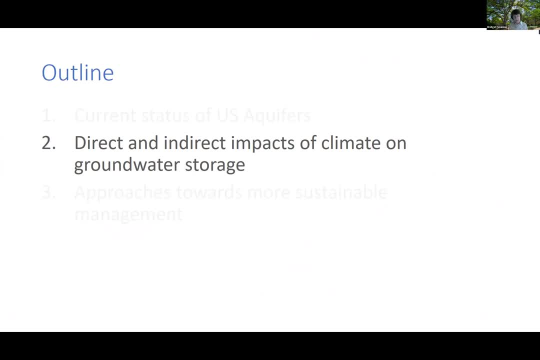 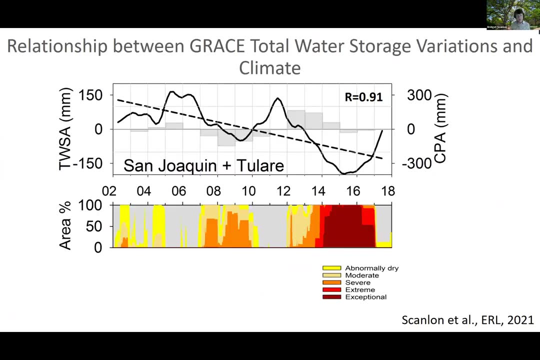 Next slide. So now looking at the direct and indirect impacts of climate and groundwater storage using the GRACE data next. So we looked at total water storage from GRACE and this example shows the southern Central Valley, San Joaquin, Tulare. 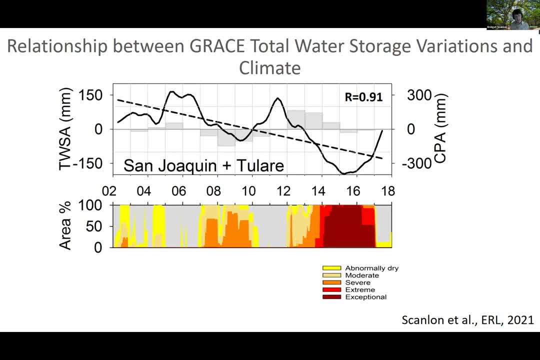 And you can see on the lower bottom part of the graph, we showed the US Drought Monitor data. So a drought from 2007 to 2008.. And then from 2007 to 2009,, and then 2012 through 2017, or 2017.. 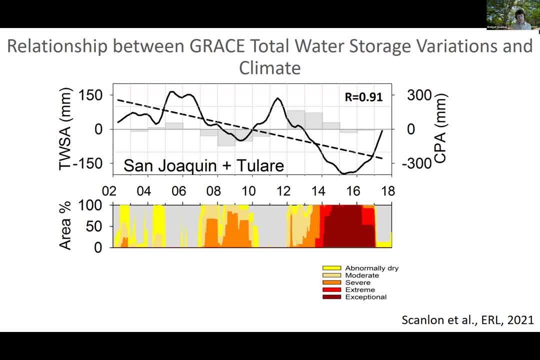 And the GRACE data corresponds to this. so we see declines in storage during the drought and large decline during the recent drought, with a correlation coefficient between the total water storage and the Drought Monitor data 0.91.. So this may reflect direct and indirect impacts of climate extremes on water storage. 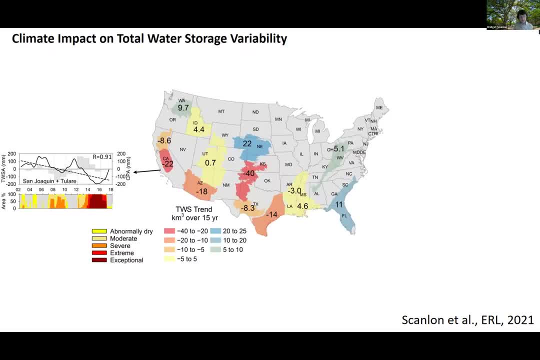 Next slide, So next slide. So I just talked about the Central Valley and the relationship with the US Drought Monitor. in the Northern High Plains We also see a strong relationship between total water storage and drought, with increasing storage during the non-drought periods and declines during the flash drought in 2011-2012.. 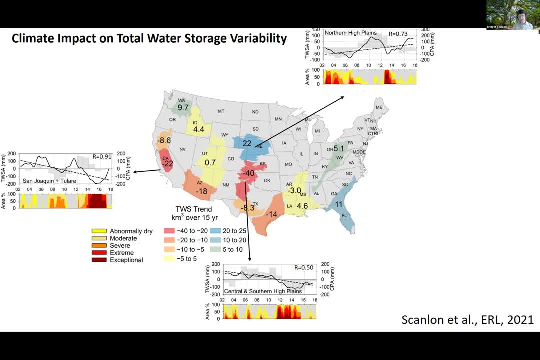 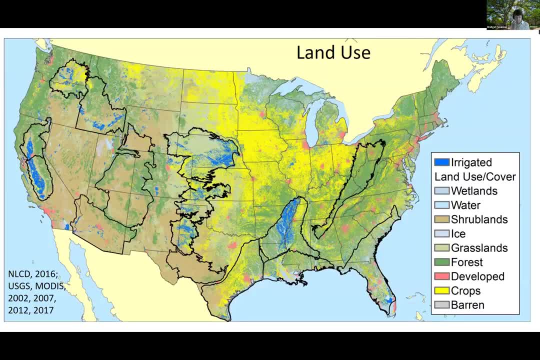 seen Next slide. So, in addition to the relationships between climate directly and water storage, we also need to consider the impacts of irrigation on the water storage, And so here you can see the major irrigated areas: the Central Valley and the High Plains, and the 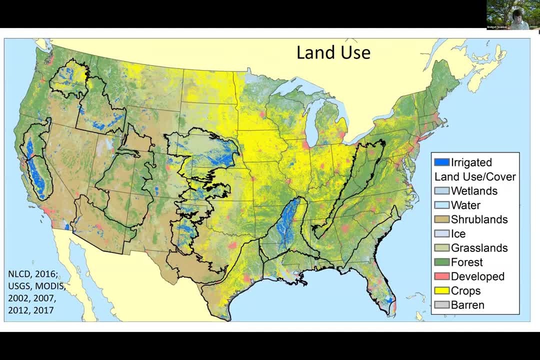 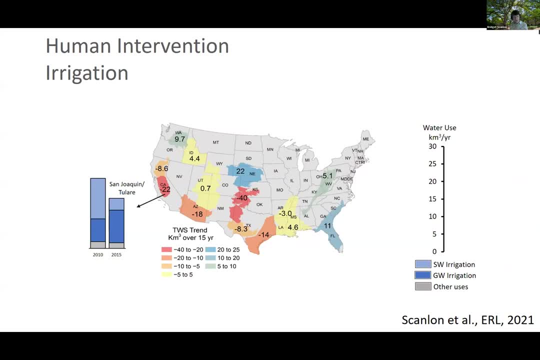 Mississippi embankment and the Northwest Next slide. So in the Central Valley we saw a strong correlation between total water storage, change and drought. but this partially reflects the fact that during 2010,, which was a wet year, most of the irrigation was from surface water, About 70. 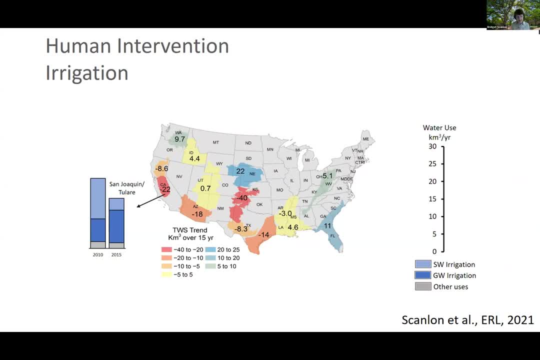 was from from surface water and about 30% from groundwater, And in the middle of the drought in 2015,, they switched from predominantly surface water to mostly 70% groundwater. So this change in human water use, then for irrigation, amplified the impacts of drought in the Central Valley. 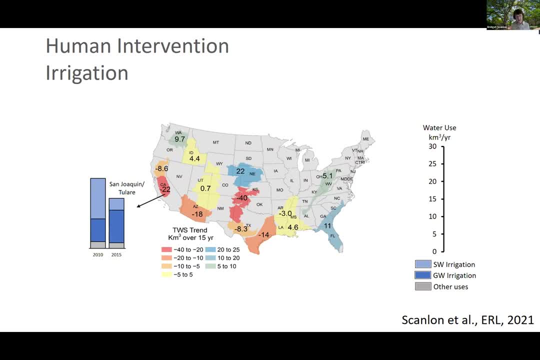 And Claudia Font has been reporting this for many years based on her regional modeling analysis. Next slide: So many people. there's a lot of emphasis in the Central Valley and all the groundwater pumpage that occurs there, particularly during drought, But it was interesting to me to see. 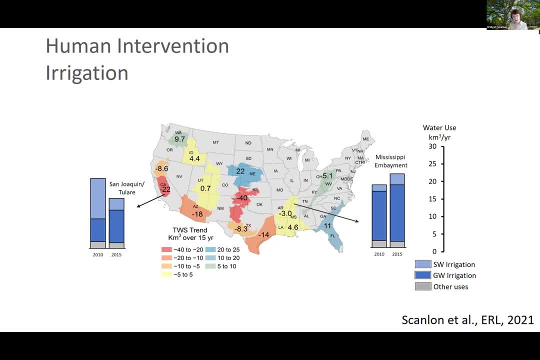 that groundwater pumpage in the Mississippi region aqua system actually exceeded that in the Central Valley And there wasn't really any intense droughts during this time period. But in this humid region then that groundwater pumpage is essentially capturing water from either surface. 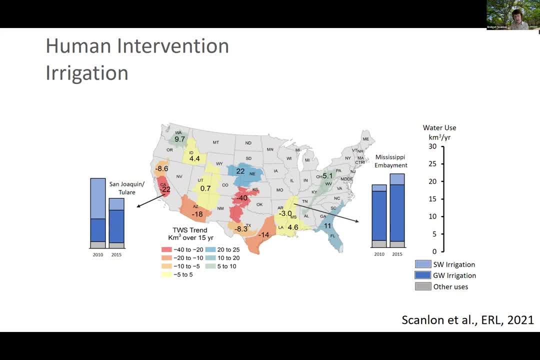 water or evapotranspiration, And so we're not seeing a large decline in storage, And hopefully the new regional model will be able to confirm this. So it's a combination, then, of climate impacts and human water use Next slide. So just one example, then, and I'm sure in the case studies, 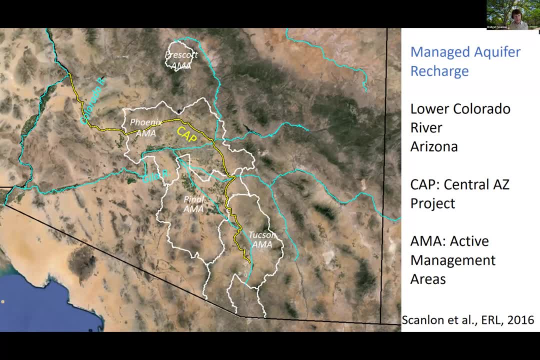 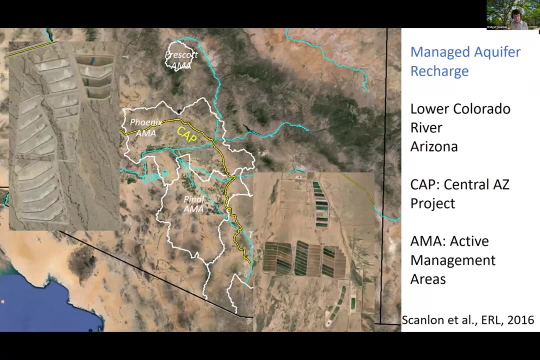 they'll be talking much more detail about this. This is Arizona and the Central Arizona project shown in yellow, bringing water from the Colorado River to these active management areas in Phoenix, Pinal and Tucson. And next slide, And these show the spreading basins. 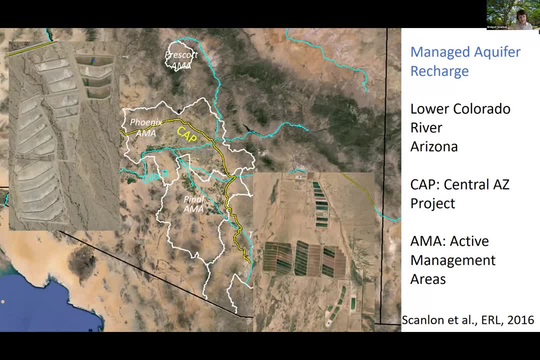 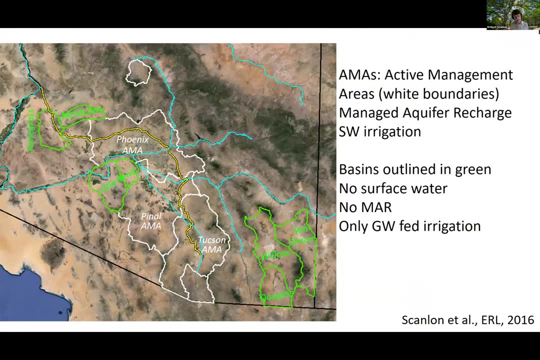 used for managed aqua recharge in these areas, in these active management areas. Next slide: And these green basins don't have access to surface water. And next I'll show the groundwater level hydrographs in these different basins. So next slide. 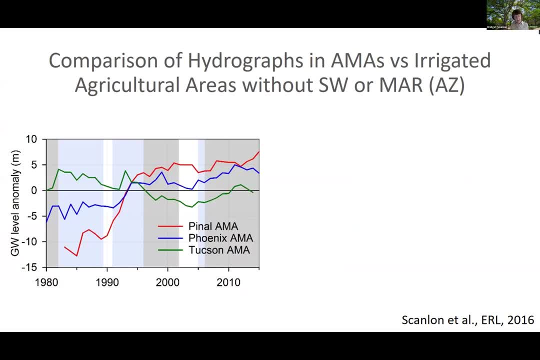 So in the areas where we have the active management areas, we see increases in groundwater levels over time, or stable or rising- slightly rising water levels over time. that can be attributed to surface water irrigation, which accounts for about half of it, and then 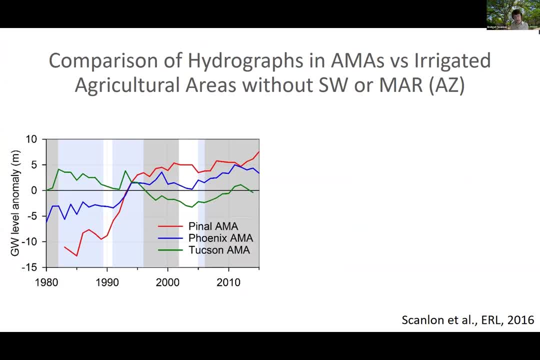 those managed aqua recharge basins, which accounts for the other half Next slide, And in the basins they don't have any access to surface water or the Central Arizona Project water. We see continual declines in water storage in these basins. 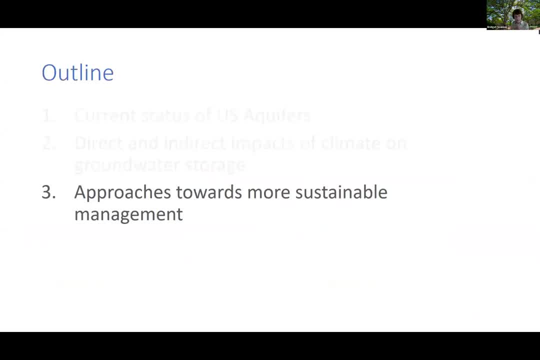 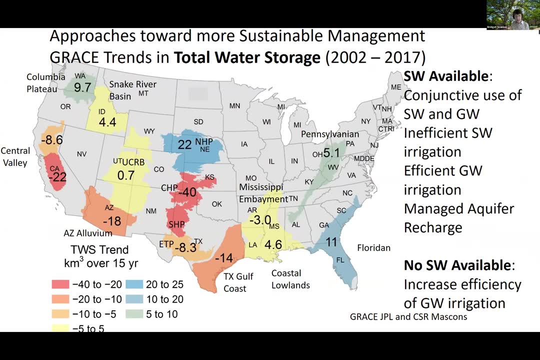 Next slide. So how can we move towards more sustainable water management? Next slide. So I think some of the analysis that we have been looking at show the importance of conjunctive use of surface water and groundwater, And I recall Claudia Fond mentioning many years ago. 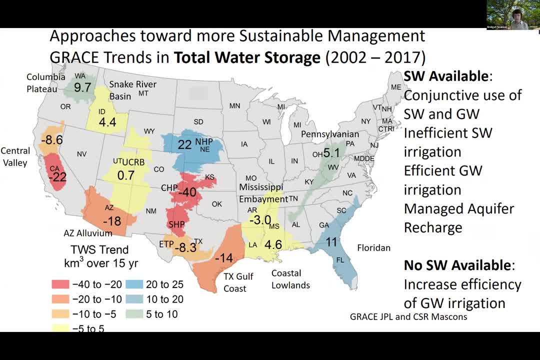 that when we are irrigating with surface water, maybe we could do it inefficiently as long as it doesn't impact the surface water resources. So we take into account the aqua recharge that's occurring as a result of that, whether it's managed. 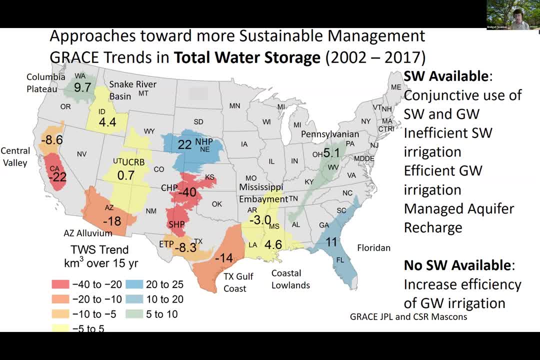 aqua recharge and flood managed aqua recharge, like Helen Duffy I'm sure would be talking about, or it just happens and it's unintentional. A recent study in Northwest India shows a net increase in water storage from canal irrigation in the last century of about 350 cubic kilometers, even though 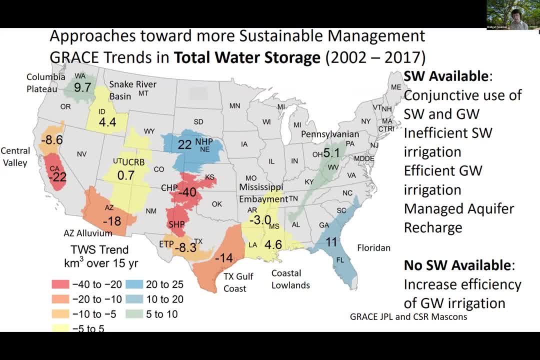 most of the studies recently have been talked about the depletion during the grace record And then when we're irrigating with groundwater because we're putting water directly in storage. it's important that that is efficient in drip irrigation and those sorts of systems, And to manage aqua recharge is a very important tool. 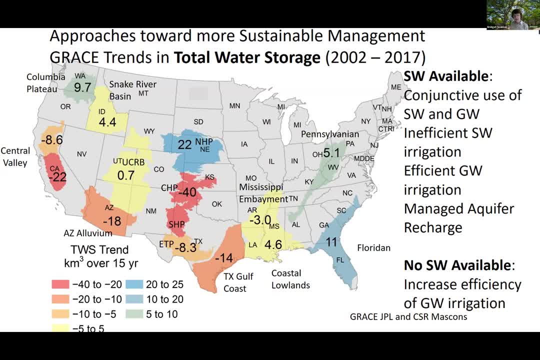 to increase resilience at the local scale. And in cases like the high plains, where we don't have any surface water, we just need very efficient groundwater and acknowledge that we are mining the groundwater. So next slide. So this work, a lot of this work. 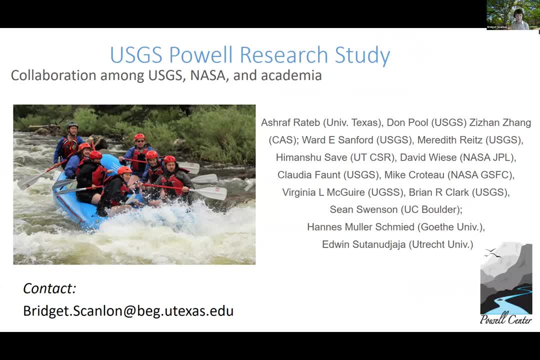 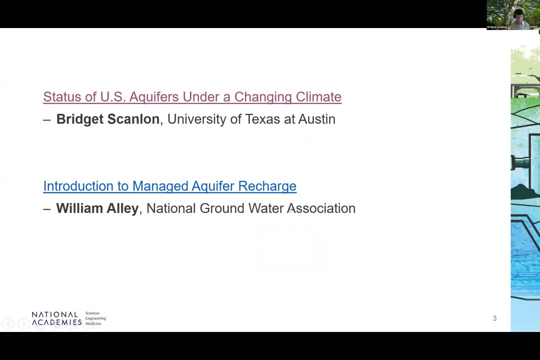 was during a power research group meetings that we had meetings every summer and really appreciate all of the inputs from the various contributors to that work. Thank you very much. Thank you very much for a very engaging talk. I think we have a couple of minutes for questions. 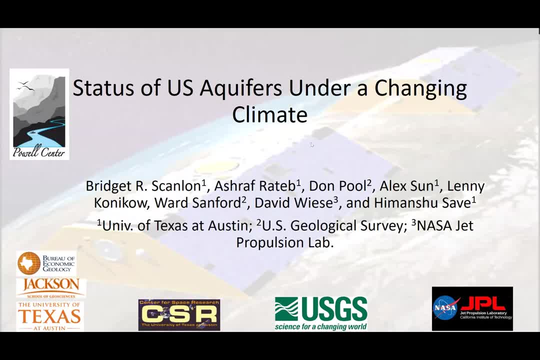 Please, please. Yes, Thank you for your talk, Bridget. I have a quick question: What's the relationship between soil structure and some of these dynamics? you see Because, for example, I wonder, in Mississippi they're using a lot of groundwater. 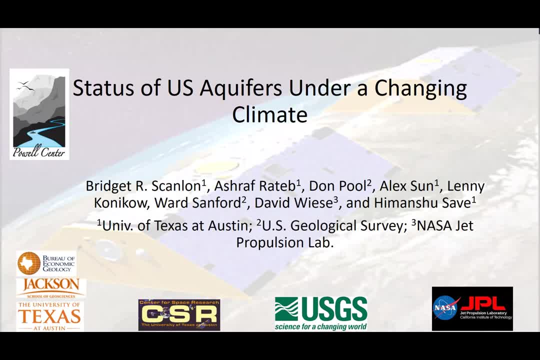 I'm wondering if it's like less evaporation, more recharge due to the soil structure, versus some of the other areas that are depending on groundwater Absolutely. And I also wonder: in Arizona, when you looked at groundwater level changes did you? you mentioned there might be because of irrigated agriculture. 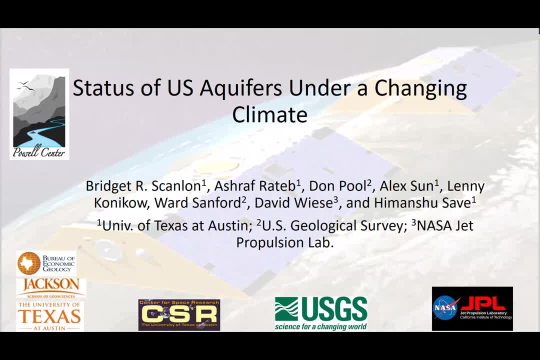 I'm wondering if you have tested that hypothesis, or is it more? I wonder what percentage of that is mostly because of managed aquifer recharge instead of irrigated agriculture. So the first question about soil structure. I think that's very important for recharge. 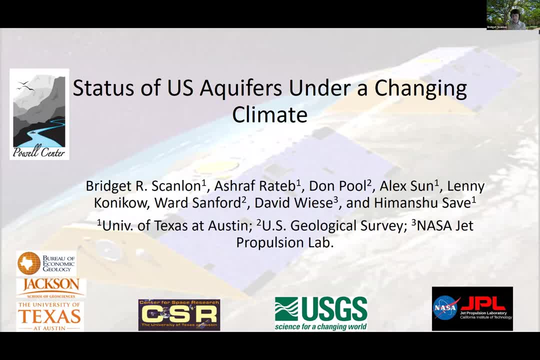 And I think we see this in the high plains, I mean the northern high plains in Nebraska- you've got the sand hills and you have very high recharge, natural recharge, And then you also have some surface water irrigation from the plat. 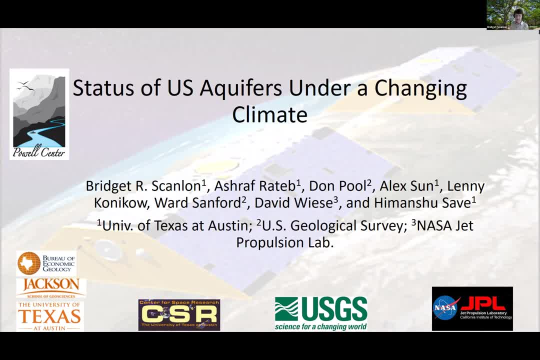 In the central and southern high plains, I mean in parts of Texas, it's like cement And but you do have some plier recharge. So soil structure is very important And I think the USGS in their new regional model of Mississippi. 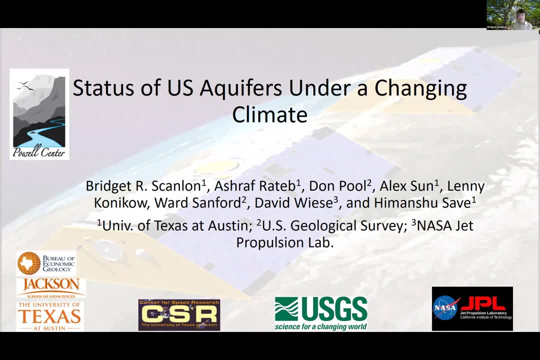 they're going to be. they have been doing geophysics to see the linkage between the rivers and the subsurface and the aquifers, the shallow aquifers, and trying to determine the linkages there and how they may be inducing recharge from different areas. 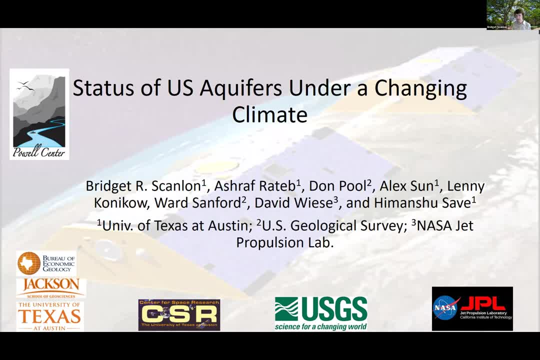 And then your second question on Arizona. Don Poole was involved in that. I think it was a study. we were looking at Arizona and they have regional models of the groundwater system and they were able to see, I think, from the surface water recharge and also from the water counting. 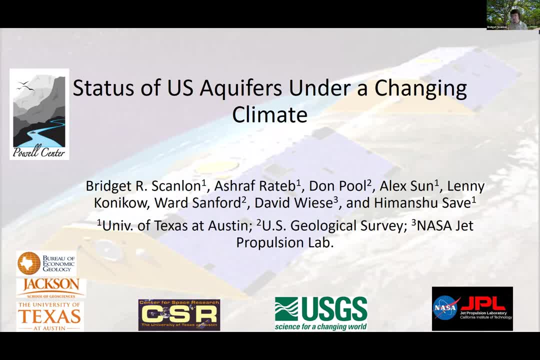 that the central Arizona project. much of that water was also used for flood irrigation And you know part of it was used in the recharge basins. So the flood irrigation from surface water contributed quite a bit to the water supply. Thank you, 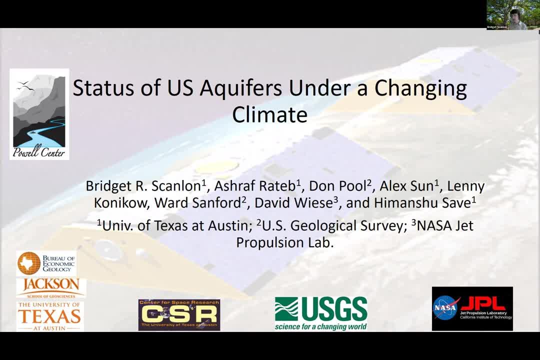 The increased groundwater levels and we saw it in the models and the data, And Don Poole had ground-based gravity data to show that also And the Maher Basin. we were able to look at those impacts locally. So I hope that answered your questions. 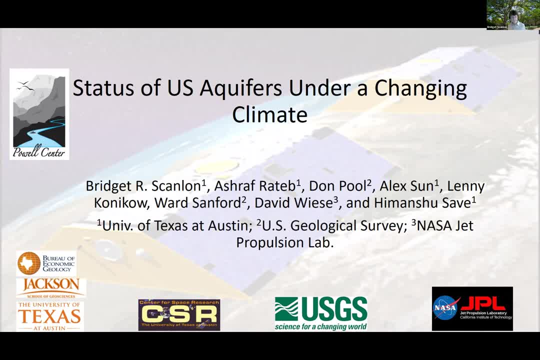 Thank you, Thank you. Thank you, Bridget. We are going to need to move on to the next speaker, but we there will be time to answer questions for Bridget in the Q&A discussion towards the end of this open session. 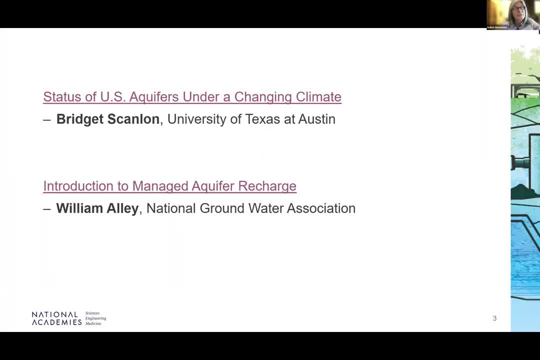 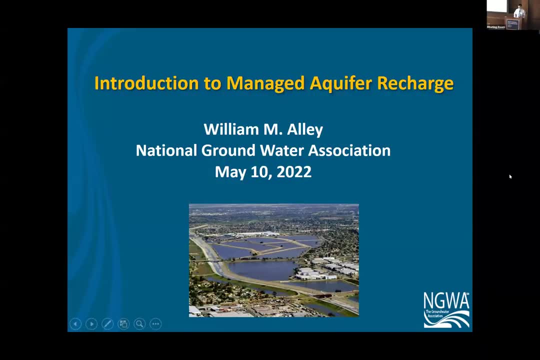 So I'd like to introduce Bill Alley, who is the Science and Technology Director at the National Groundwater Association and was previously the Chief of the Office of Groundwater at the US Geological Survey. He's published widely, including several general interest environmental science books. 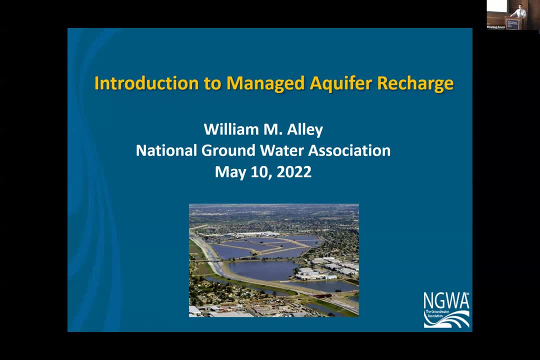 Bill. Okay, Thank you. My pleasure to be here And I guess my job is to give you an introduction to Managed Aquifer Recharge. Here's an. this particular picture is of the Montebello Four Bay Area above LA. These spreading: 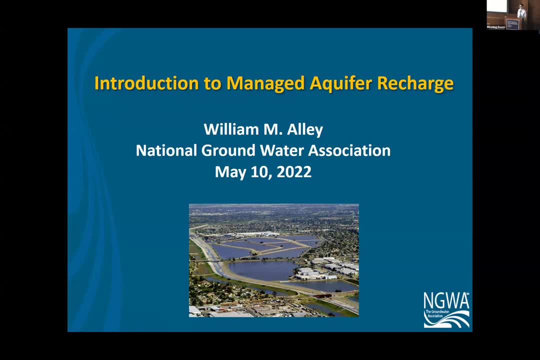 basins shown here off. that's LA's idea of a river there, that concrete channel, The spreading basin, has been operating since the 1930s where they were recharging stormwater. In the 1950s they started recharging, adding also imported water from the Colorado River. 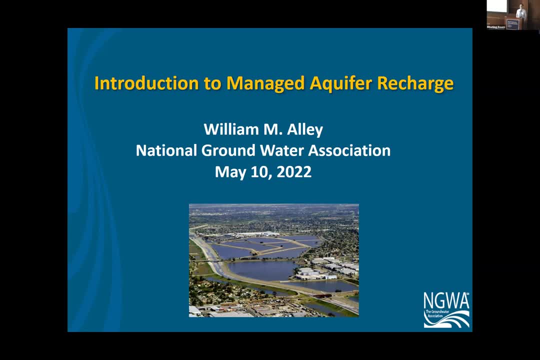 And 60 years ago they started using recycled wastewater recharging that, So it's that's the oldest potable reuse project in the United States In 2019, they actually took themselves off imported water from from anywhere in California. 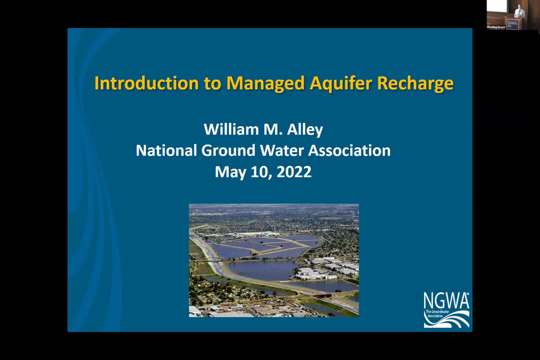 They've had a program they called WIN, which is Water Independence Now, and they've managed to to take themselves off imported water, which is very important for this particular year. if they can, they can continue and the Los Angeles plans to basically recycle all. 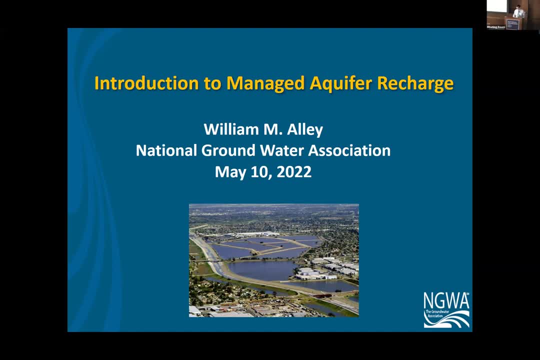 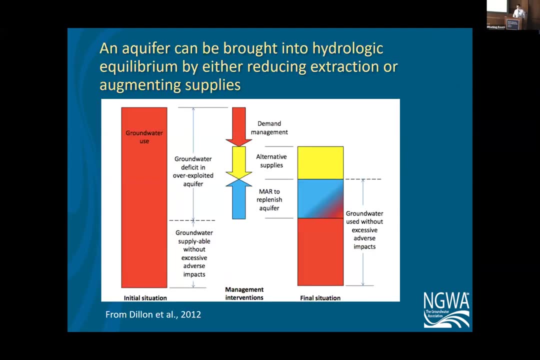 of its wastewater at some point in the future. Thank you, Thank you, Thank you. Okay, let's see if I can advance this. So there's a couple ways to hopefully that'll disappear on the screen there. There's a couple ways that you can deal with groundwater overdrafts. 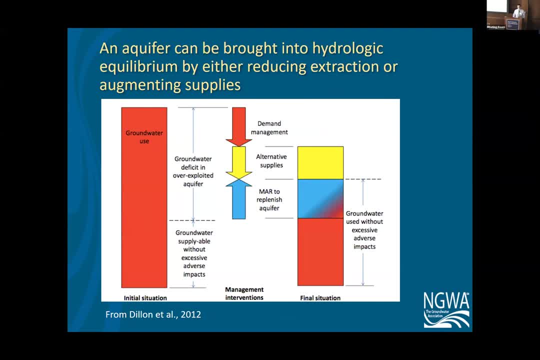 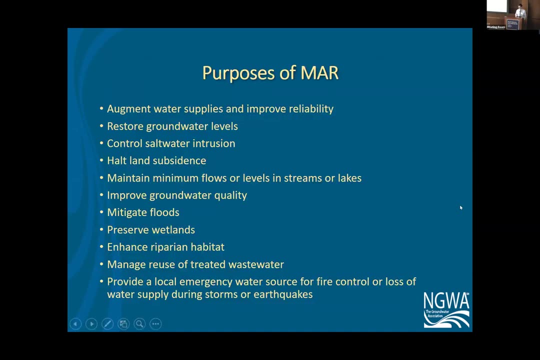 One is to replenish the aquifer, which is the MAR idea, but there are also demand management and alternative supplies, So it's really working together with those three basic ways of trying to control the amount of water in an aquifer. Okay, so I think there's a delay here. 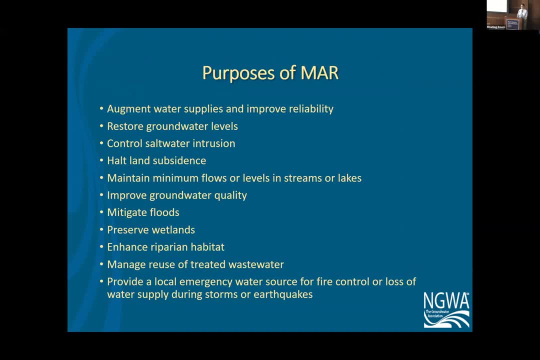 So there's a purposes. So we tend to think of storage as a purpose of of bandaged aquifer recharge, but actually they're also used for environmental benefit, for holding land subsidence, for preserving wetlands and managing the reuse of treated wastewater. 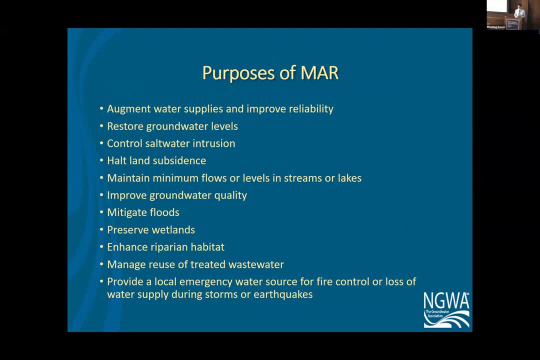 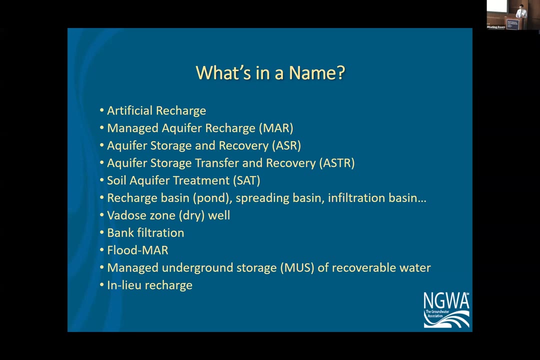 as well as providing, possibly, a local emergency water source for fire control or loss of water supply during storms. So there are a lot of different purposes of bandaged aquifer recharge. Now there's a very okay lots of names out there. 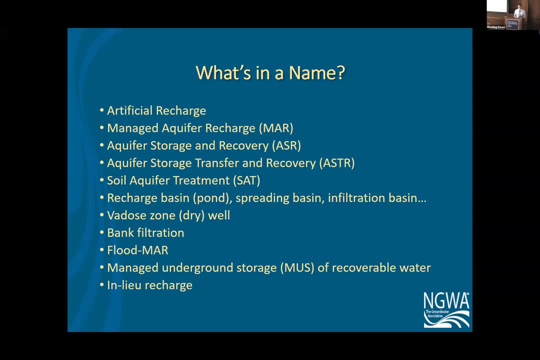 So originally it was referred to as artificial recharge and that term carries on today. Most people involved in bandaged aquifer recharge prefer not to use that term. They want to emphasize the management, because the idea is the purposeful recharge of water. 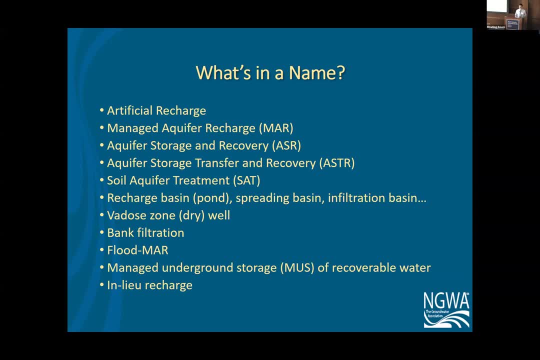 either for water- or for water- Okay, Okay, Okay Later withdrawal- or for environmental benefit. But there are a lot of other terms. Another one you hear a lot is aquifer storage and recovery, which I'll get into in a moment. 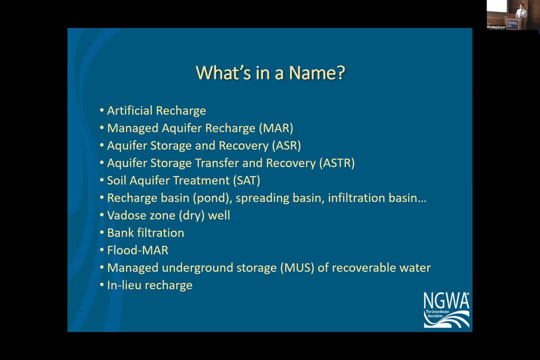 And that actually is a specific type of of bandaged aquifer recharge, but it's often used as a synonym for for bandaged aquifer recharge. And then I'll skip down to the bottom, to next to last there: Managed underground storage of recoverable water. that was a term invented by the National Academy. 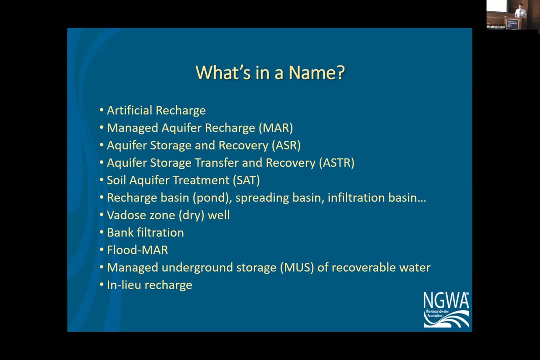 of Sciences in their last report, but it just tends not to be. And one can also think of in lieu recharge as related to our managed aquifer recharge, in the sense that you are not withdraw using surface water supplies during and letting your aquifers recharge during during wet periods. 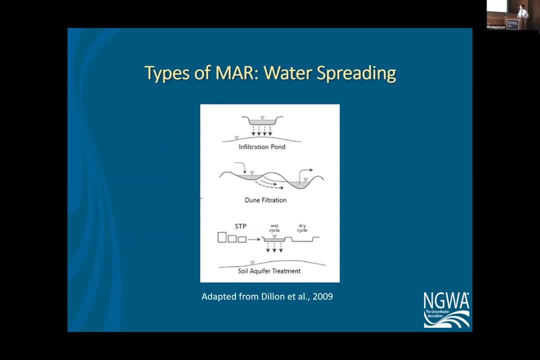 So let's look at some different types. Mar So there's water spreading. the top one, an infiltration pond or spreading basin, is, for example. I just showed you example on the introductory slide. but there are other types. in the Netherlands They do dune filtration. 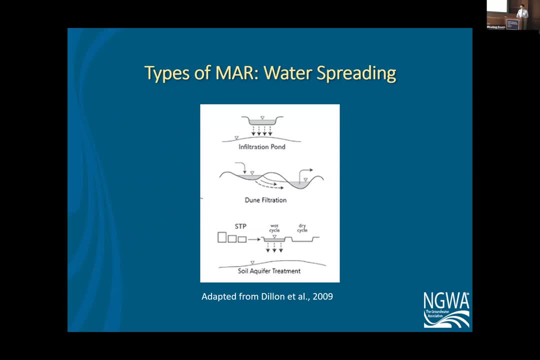 They do dune filtration. They do dune filtration. One that's received a lot of interest, is for a long time is is taking wastewater and using essentially spreading basins to to mostly purify the water from pathogens and to deal with nutrients. 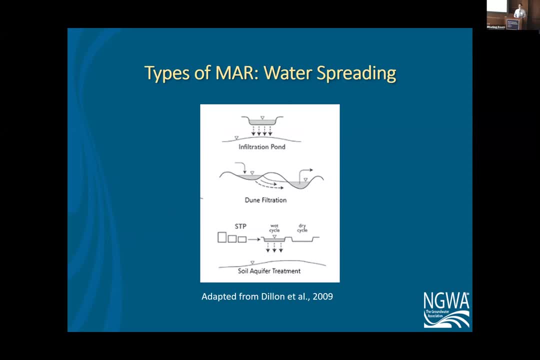 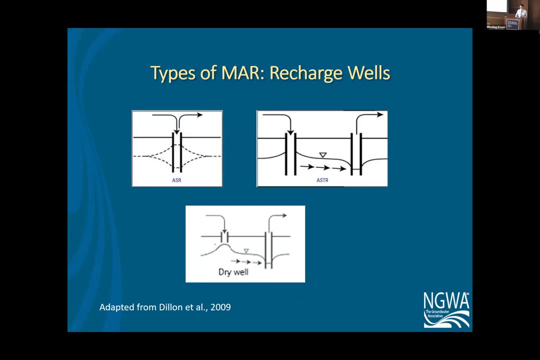 That's the main purpose there. It's been studied probably all over Herman Bauer back in the 1960s in in Arizona. So there are also recharge wells. Aquifer storage and recovery is actually where you use the same well or wells for recharge. 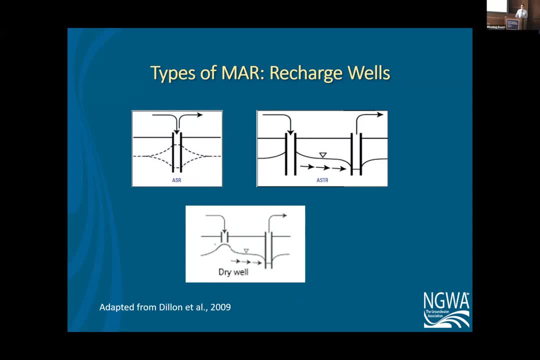 and recovery, And it's a little different, because you can actually use brackish aquifers that way and build up a freshwater bubble if you will, And so it's a very it should be used as a specific term So to distinguish that sometimes in texts you'll see the term aquifer storage transfer. 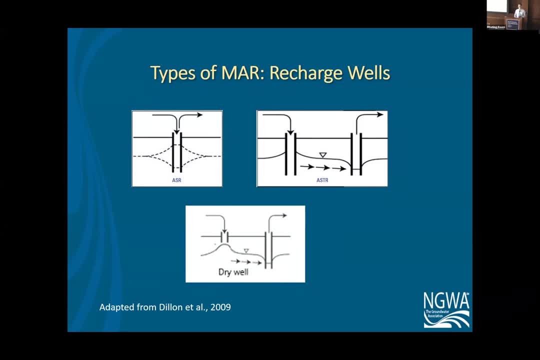 and recovery, which is helpful to show the distinction. but there's not a recharge project in the United States where somebody is recharging wells and they would say I'm doing aquifer storage, transfer and recovery. they would tell you they're doing well, injection or what's. 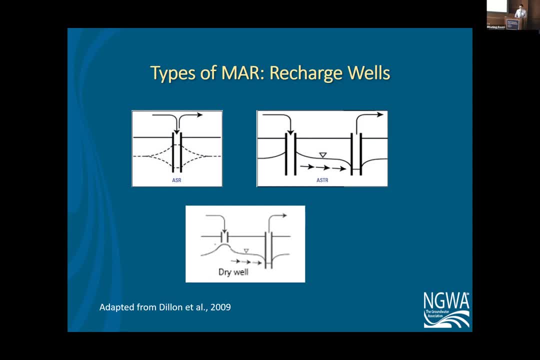 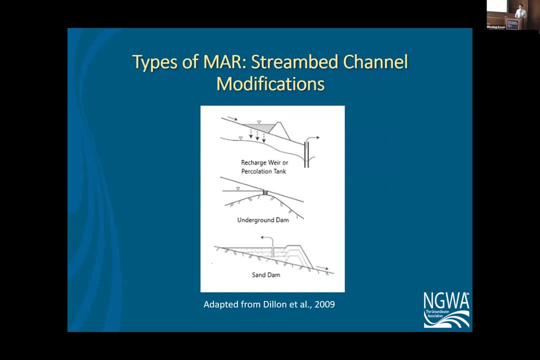 going on or what have you. So it's kind of not used much. And there's also dry wells, and I'll actually get to an example of that later. And then finally there's stream bed channel modifications. These are typically done on ephemeral streams, either, where you build a dam and capture water. 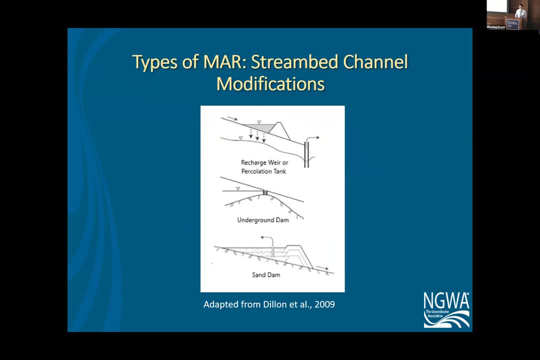 behind it for the express purpose of recharging the aquifer and using it down down gradient. Or if you have a low distance to an impermeable, relatively impermeable unit, you might build a dam, underground dam, The pond water, or you might actually build up gradually a series of dams and make your 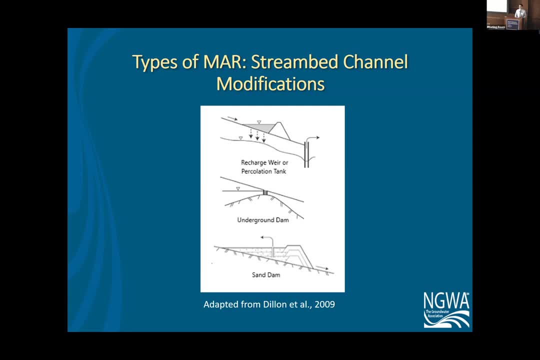 own aquifer, if you will, because these are used a lot in, for example, a place like India, And in fact, India recharges more water than anywhere else in the world. United States is second, but India is far out in number one. slot on that. 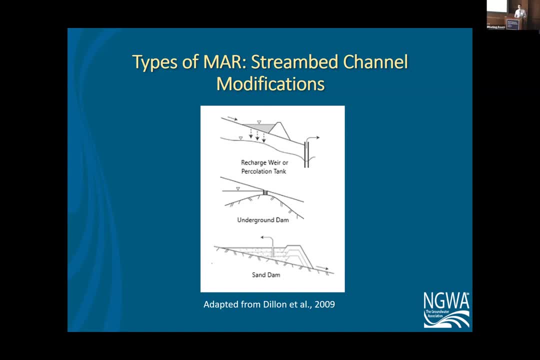 They also use more groundwater than anybody else. And another in terms of future use. approximately 1% of the groundwater withdrawals that are used today are recharged through managed aquifer recharge means, So there's a lot of potential out there. Oh, finally, there's also bank filtration. 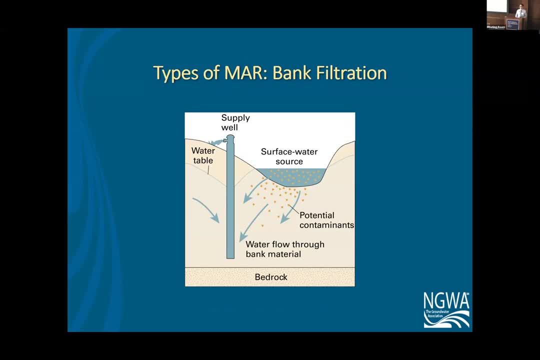 This is often used as a pre-treatment technique, particularly in places like Berlin and Hungary, but also in the US, And I'll get to an example of that, where you're using, essentially put, a well, maybe a couple of hundred yards from a stream, and you're pulling the water from the stream and 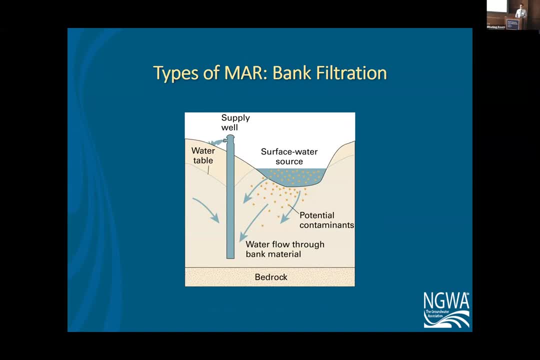 it's naturally cleansing itself And it's shown to be pretty effective in certain types of water And it's shown to be pretty effective in certain types of water And it's shown to be pretty effective in certain types of chemicals and not so effective. 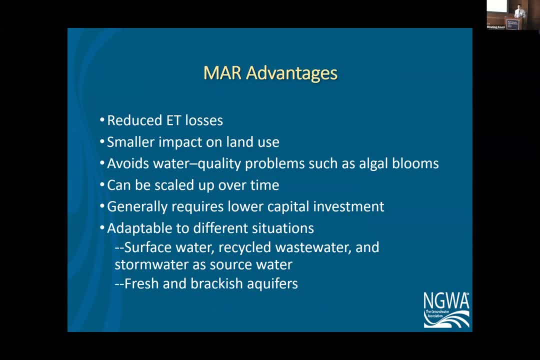 in others. So what are the advantages? Well, one is what most people think of immediately as a reduced evapotranspiration losses, but there's also a smaller impact on land use and also avoids water quality problems such as algal blooms. 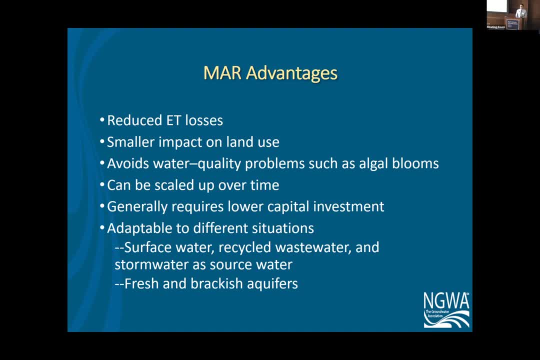 A very important part of it is it can be scaled up over time, and actually there's reasons for scaling them up over time, which I'll get to later. generally requires lower capital investment And it's adaptable to different situations, as I've already discussed. 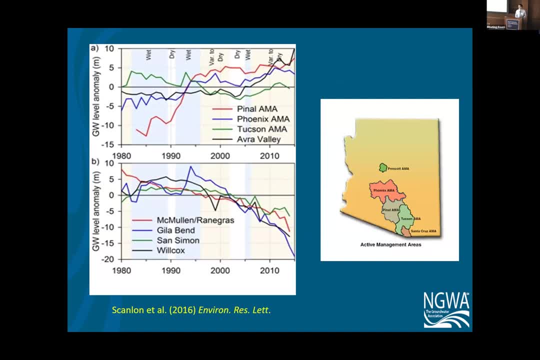 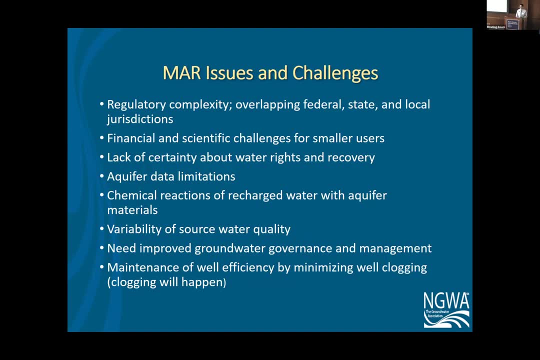 So Bridget included this. I included this in case Bridget didn't show this figure, so I'm going to go ahead and skip it. Okay, so what are some of the issues and challenges? One is regulatory complexity. Injection wells are regulated by the Underground Injection Control part of the Safe Drinking. 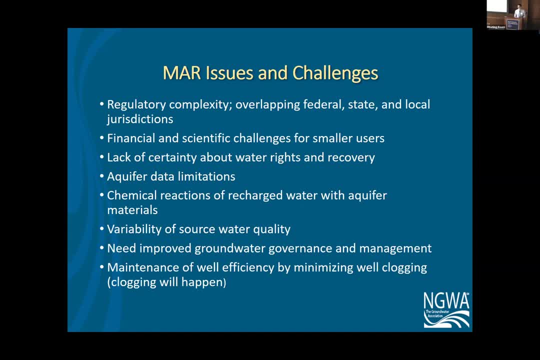 Water Act amendments- And there are. There are state and local jurisdictions that deal with things like water rights and so forth, So it can be a difficult thing to get one of these projects going. For smaller users there are financial and scientific challenges. 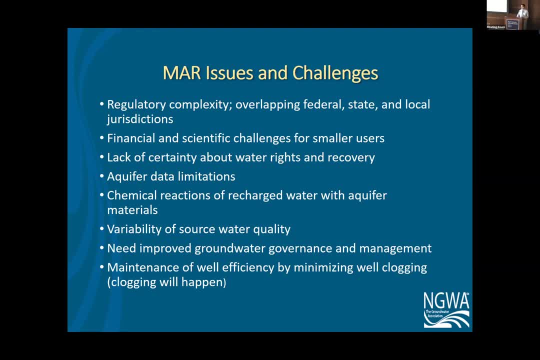 The lack of certainty about water rights and recovery- and I know you'll hear more about that tomorrow- is a challenge. Data limitations, Chemical reactions of recharged water would act for materials, Think arsenic. but there are other issues: Variability of source water quality. 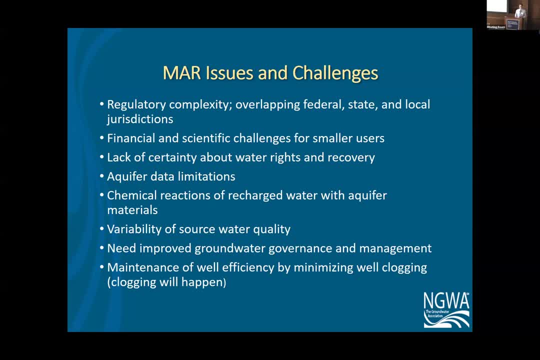 If you're using something like stormwater, Water has a highly variable water quality characteristics to it, as can surface water, And you need to improve groundwater governance and management really. And then, basically, you have to deal with well clogging, so almost insured. 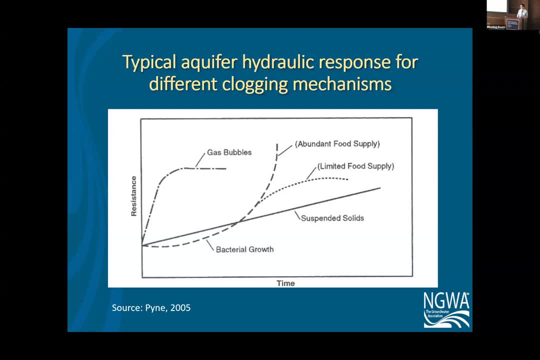 And well. clogging can occur in different timescales and different ways. This just shows the number of those, whether they're gas bubbles or abundant. or you may have bacterial growth that may depend on, essentially, the food supply for the bacteria, or you just 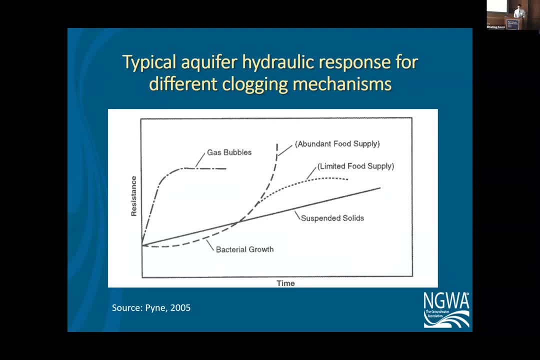 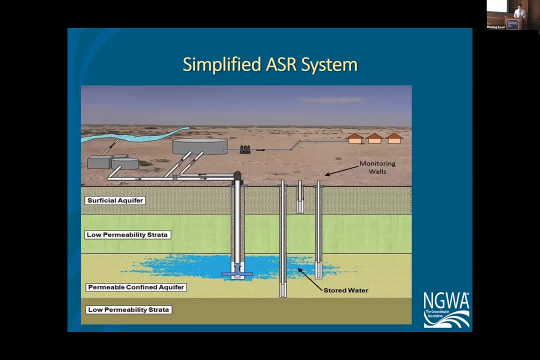 may have a gradually increasing suspended sediment clogging your well. So that's a challenge. So those all have to be dealt with in either well injection or in spreading basins. So let's take a simplified aqua storage recovery system here: Same well pumping and withdrawing, or recharging and withdrawing some monitoring wells around. 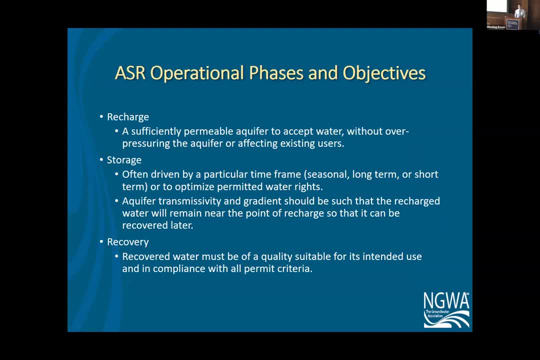 it And you have to think in terms of various operational phases. So with recharge you need a sufficiently permeable aquifer that you have without overpressuring it. For storage, That depends on the timeframe, So these may be seasonal, long term or short term. 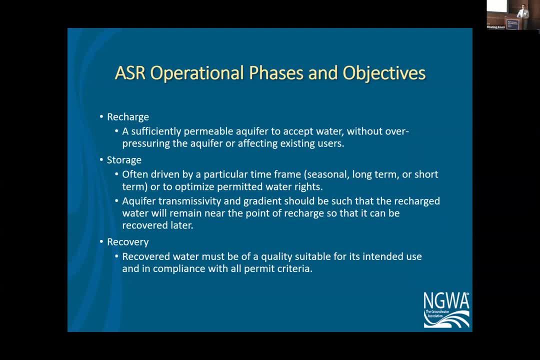 And so- or maybe to optimize permitted water rights and surface water rights, So the aqua transmissivity and gradient should be such that the recharge water is going to remain close enough to the point of recharge that you can recover it. So that's an issue with longer term issues. 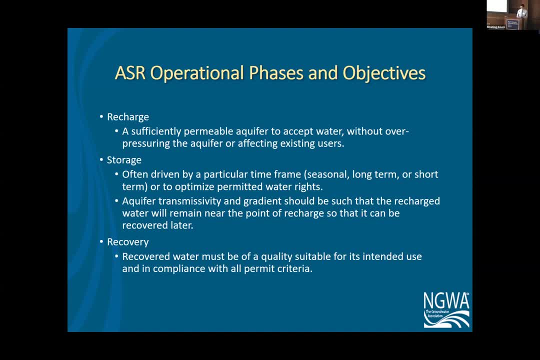 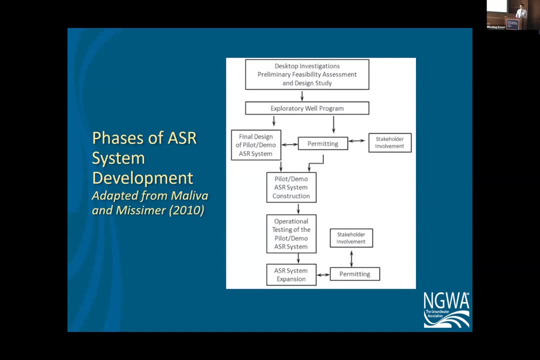 And then recovery. water quality becomes a big issue on on the water quality side of things, And typically these projects, as I mentioned, are staged. You start with a sort of a design. you might have a pilot and a demo project, particularly. 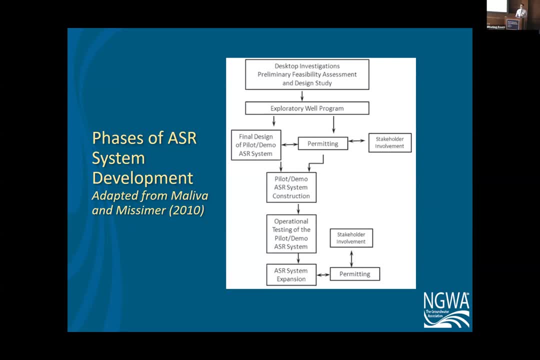 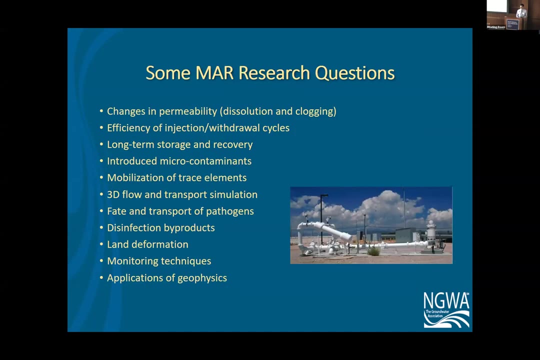 with what recharge? well, you've got permitting and stakeholder involvement that may come into play here, And so it's a gradual process and oftentimes so there have been projects where where they've decided to just go full steam ahead right from the beginning and they've had problems. 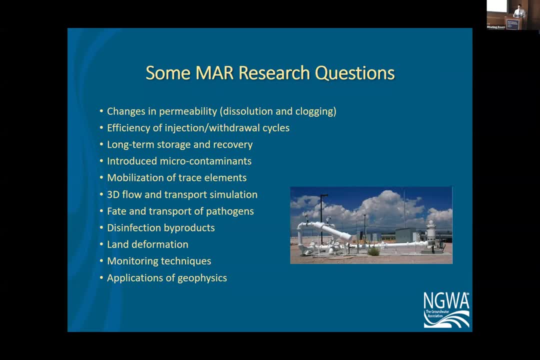 So what are some research questions? I list a number of them there. I'll point out the introduced micro contaminants. So PFAS is a big deal these days, But there are others- are still the issues of pathogens, disinfection byproducts either forming or being injected into wells. what's going to happen to them? monitoring techniques. 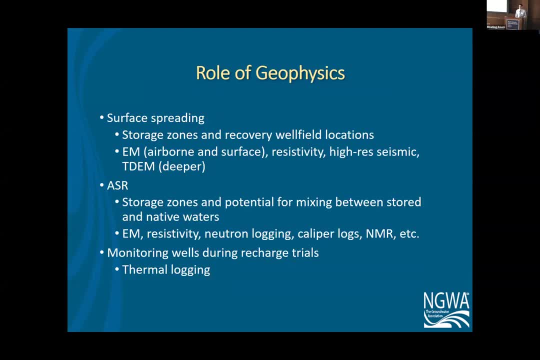 applications of geophysics And just to show you an example there, they can be applied to surface spreading for identifying storage zones and recovery wellfield locations, And I know that you probably all Heard about airborne electromagnetics at one time or another. you will probably by tomorrow. 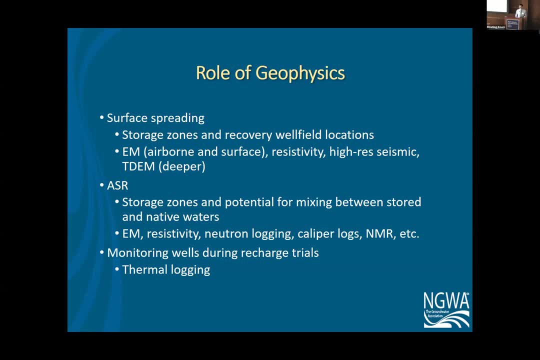 which is very, which is being done in a big scale in California With aquifer storage and recovery. you can do it, for you need storage zones and potential for mixing. Again, there's a whole range of geophysical techniques And finally you can do thermal logging it to monitor wells during recharge trials. 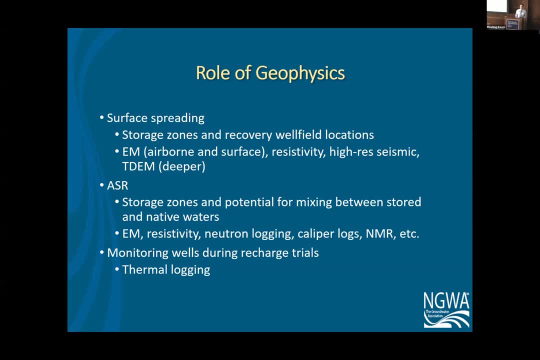 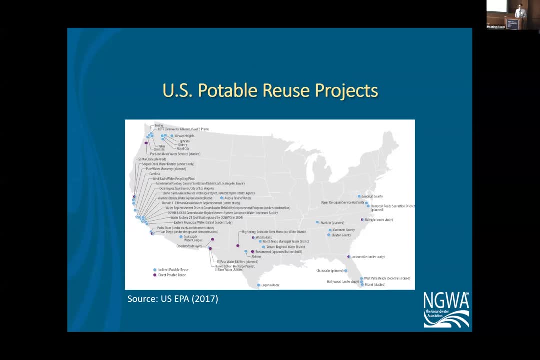 So there's a lot about, there's a lot of tools that are out there that could be applied to manage that for recharge Very in various ways. Okay, So I'm going to end with focus on potable reuse projects And I'm going to. I can't stop myself from passing around a book that my wife and I just 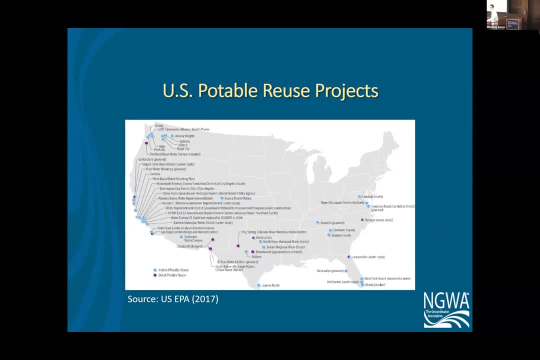 published a month ago, but it's totally on this topic. It's a fascinating topic. This is an EPA map. It's actually a little out of date- 2017, but all those blue dots are Indirect potable reuse. 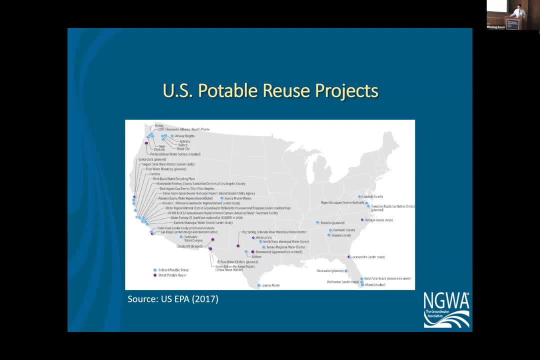 They're not all groundwater. Some of them are surface water, such as Gwinnett County and the Occoquan, not far from here, but you can see there's a lot of them and there's a lot California and along the coast, for good reason. 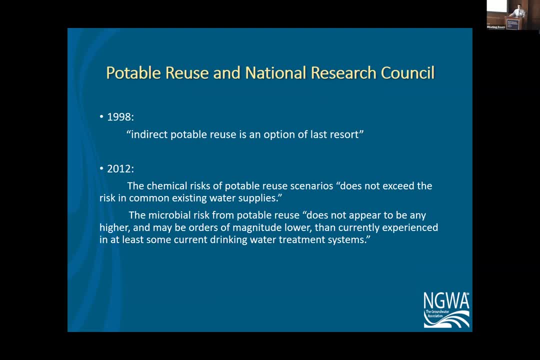 So with national research councils actually looked into potable reuse back in actually a previous report, but in 1998, there's a book about this stick. It has a 12 page or so executive summary. Embedded in that summary somewhere are the words indirect potable reuse is an option. 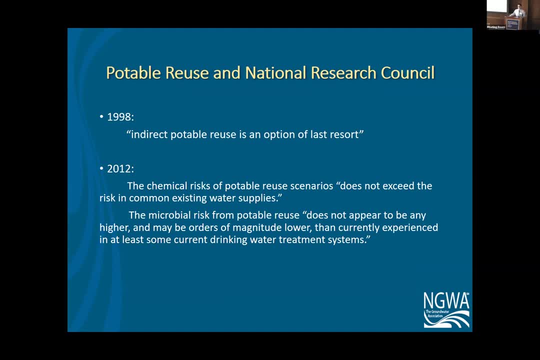 of last resort. It shows up one other place in the report. There's nothing else in that report that ever really mattered, So that became a real red flag for a lot of people, unfortunately, and it was still a developing technology really at the point, and they made it then in the report, which 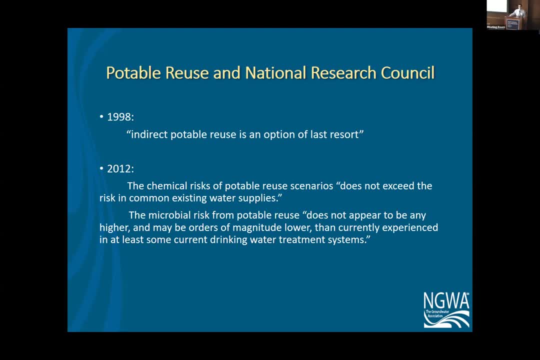 is a fine report, made that point in 2012,. it was looked at again by another Academy group. This time They compared the chemical and biological risks of potable reuse with what's in a de facto water reuse, if you will- normal situation, and they basically concluded that the chemical 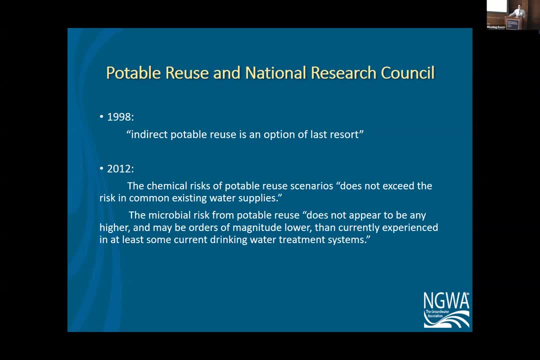 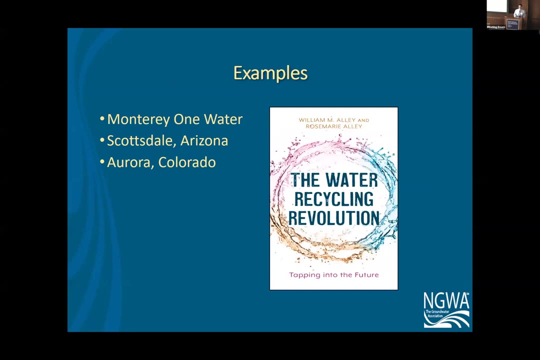 risks are about the same, maybe, and the microbial maybe even better. it might be even better to do the potable reuse. So it's come a long ways in a couple decades. So here's the book I'm passing around. I'm going to give you three examples from it. 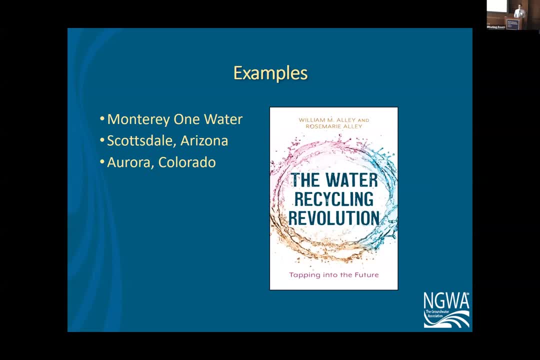 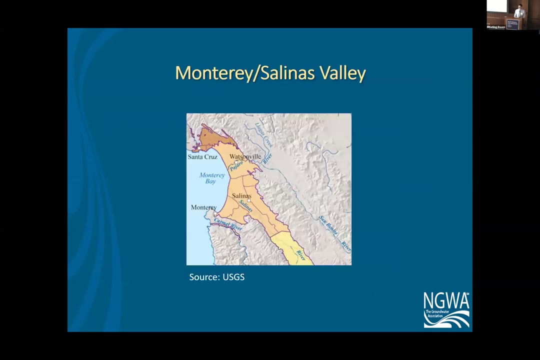 One is Monterey, one water which is a classic case of the application of the one water idea. Scottsdale, Arizona is, I'll mention that, mainly from a dry well and Aurora, Colorado, has an interior, very interesting study. so if this is the modern, but you see Monterey there. 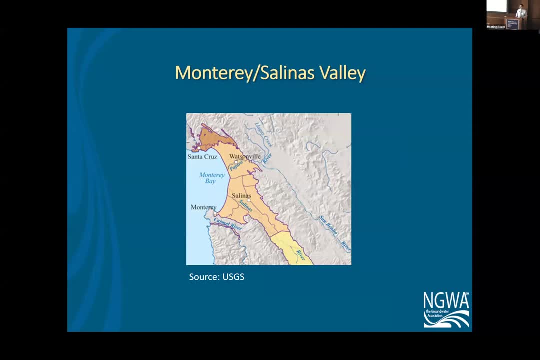 the Monterey Peninsula, and the orange area shown is the salinas Valley, otherwise known as a salad capital the world. uh, it also has had seawater intrusion. uh, from pumping for that. uh, all the leafy stuff. uh, back in the 1970s, uh, it had. it's this: uh. they undertook an 11-year study of application of. 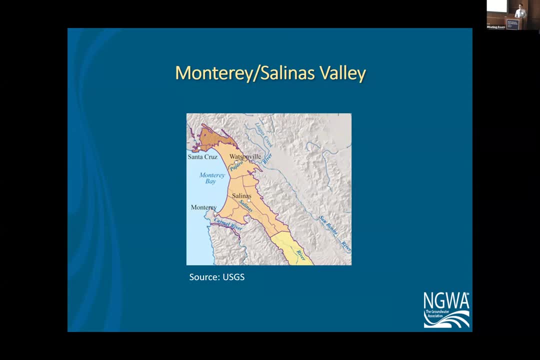 tertiary treated wastewater to food crops eaten raw. it was a classic study and eventually, in 1998, they started irrigating. they built a regional wastewater treatment plant and started irrigating 12 000 acres with tertiary treated water, and so that was a setting for another problem: that 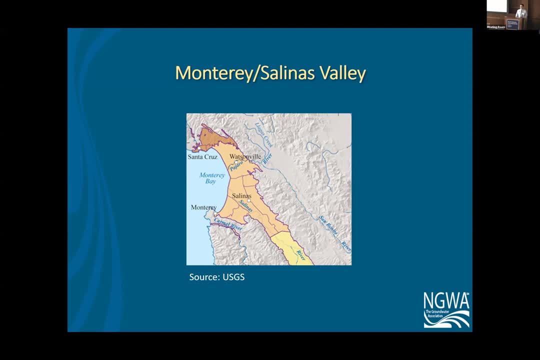 existed in monterey, which is the people and businesses. there's not enough water. they're drawing water from the carmel river, which you'll see south of the of there, and from a seaside groundwater basin, a relatively small groundwater basin, and they've been told for years. 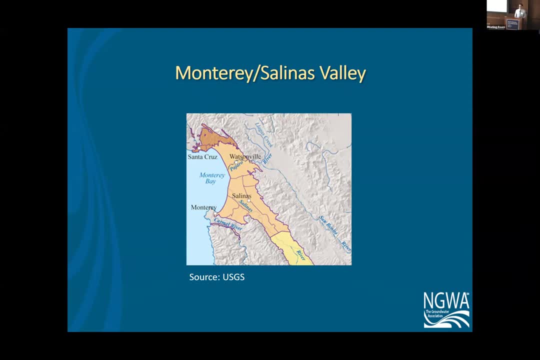 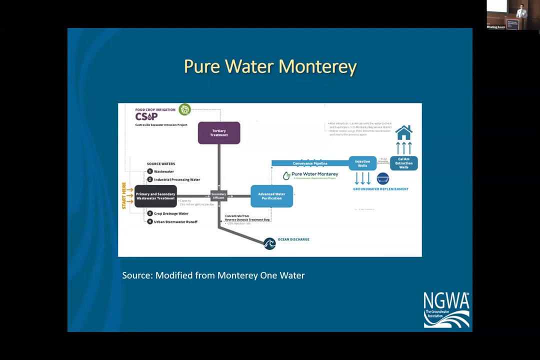 to cease and desist on the carmel river, at least reduce their flows, because of the damage to environmental, uh, environmental issues, salmon, etc. um, and so they started: monterey, one water, or pure water. monterey, uh, just came online maybe a couple years ago. this is a diagram of it, so they 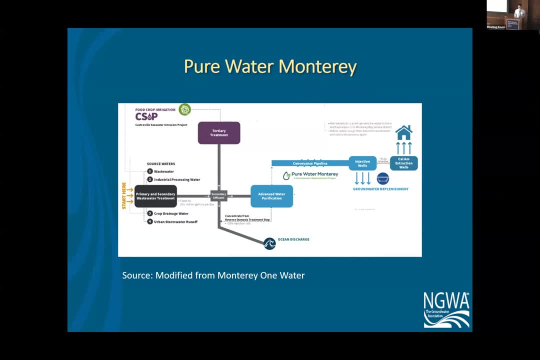 have four sources of water: wastewater, industrial processing water from washing that leafy vegetables, crop drainage water and urban stormwater runoff and they're able to essentially either direct that to tertiary treatment for application at the top there to their seawater project- uh with the 12 to 12 000 acres, or they can put it through the advanced water. 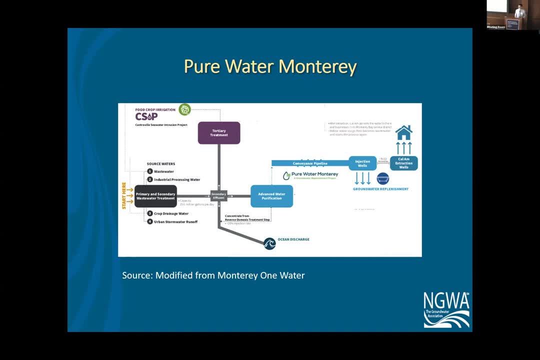 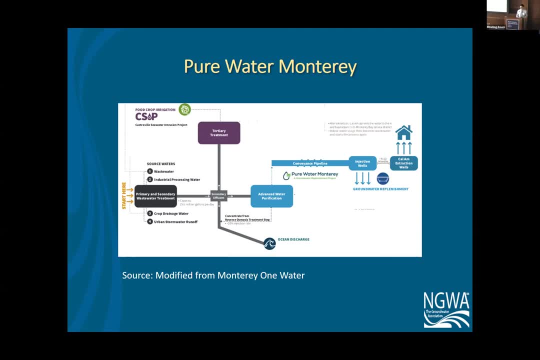 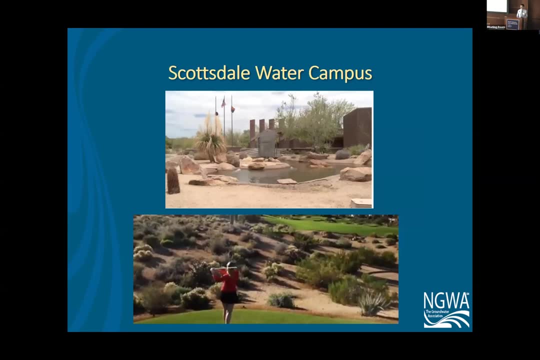 case of the application of one of one water: scottsdale water campus. uh, interestingly enough, uh is actually a collaboration between 23 golf courses and the city of scottsdale. uh, and they use dry wells, uh, because they're about 500 feet to water, so they use advanced treated wastewater for. 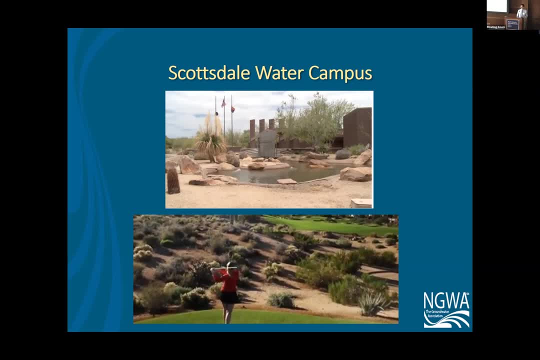 uh recharging those dry wells and they then use the water during the wet season. they can put it injected underground through those dry wells and during when the irrigators need it, they can uh send the water up for irrigating uh eating crops, and and the golf courses pay part of. 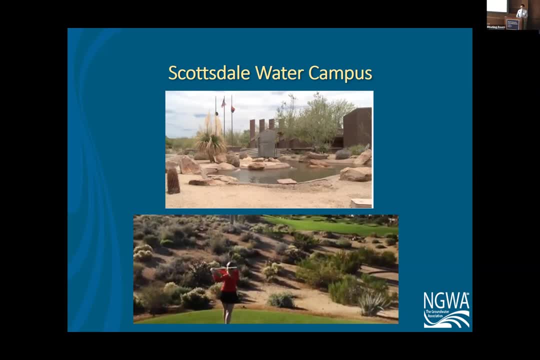 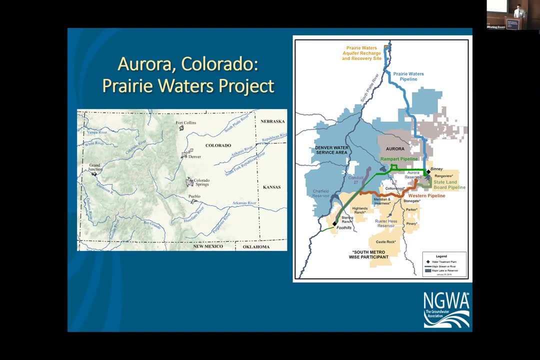 the cost of this whole operation. so and it's worked very well, uh, over time. finally, uh, aurora, colorado is a very interesting case of most of the south platte rivers downstream from denver and certain times of the year has actually treated wastewater from the wastewater treatment plant and they pick. 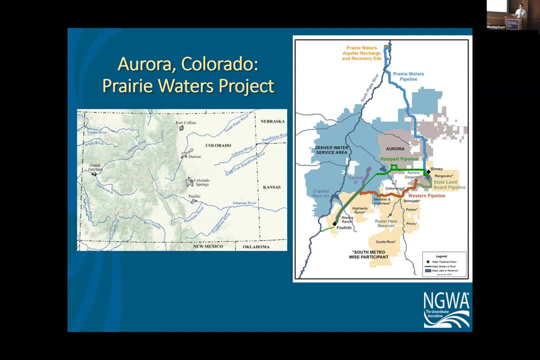 it up further downstream, use the bank filtration process that i that i mentioned, pump at 26 and a couple other things, and pump it back to back to aurora uh, where they treat it with advanced techniques and then provide it uh for drinking water uh, and they've been doing that since uh, the 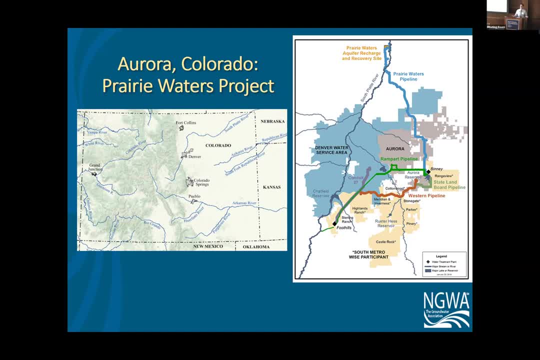 beginning of about 2010, i think, and interestingly enough, there's a whole nother story where they're actually sharing this capability and their capacity with with the uh south metro areas, which are all dependent, mostly dependent on the denver basin aquifer. so it's been a very successful 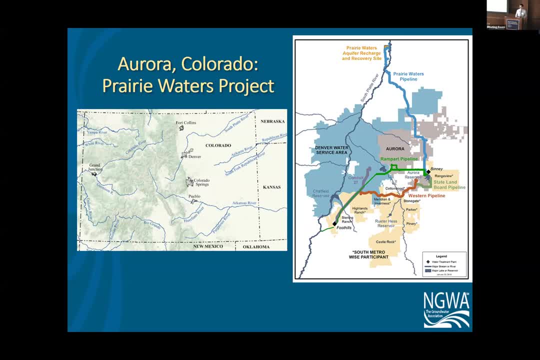 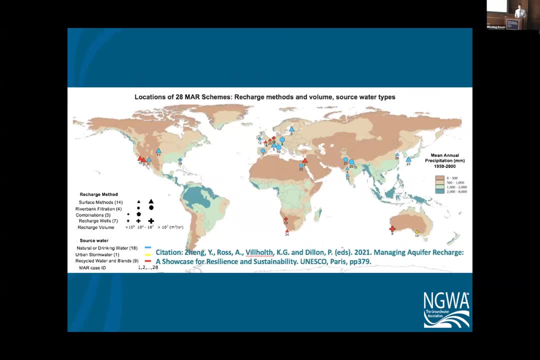 uh, very successful uh project. it doesn't get as much press as some of the other managed aquifer recharge projects do. finally, a couple things about uh. i've mentioned the us, but there's a lot of managed aquifer recharge. This is a recent report that was just by UNESCO. 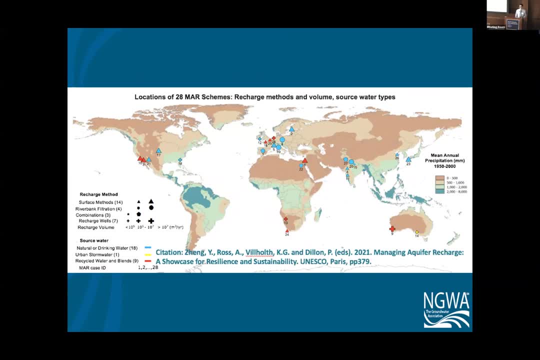 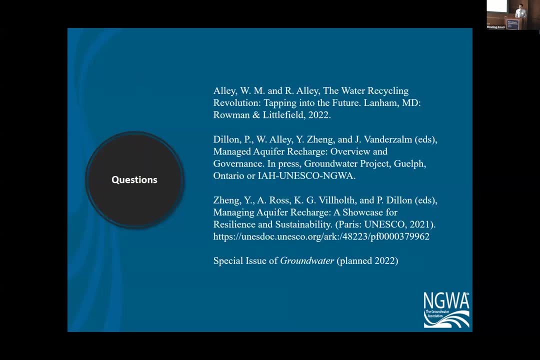 looking at 28 managed aquifer recharge schemes around the world, including some in the United States. Very interesting report. And then finally, I'll end there with just a few references. I mentioned the first and the third on the list there. There's also under the John Cherry's Groundwater Project. 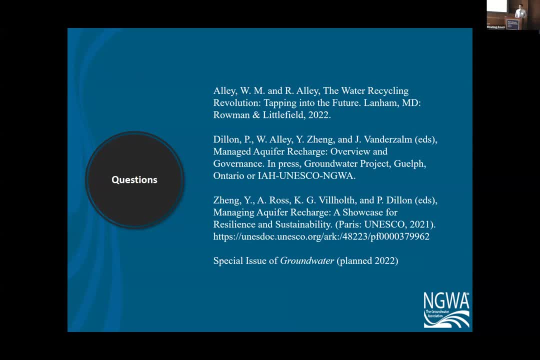 an introduction intended as an introduction in aquifer recharge has become much more and much more very heavy on the governance, management and governance side. Probably will be coming out soon this year as a joint publication of IAH, UNESCO and the National Groundwater Association. 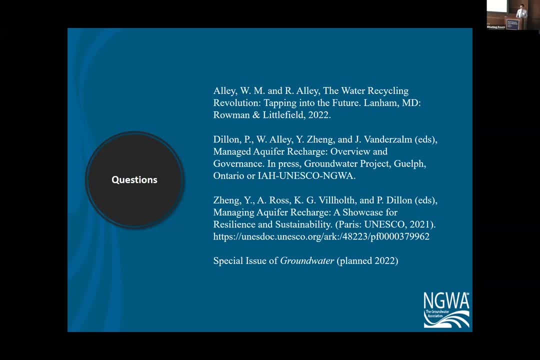 And finally, we at NGWA are planning a special issue of groundwater. We're almost there. It's like herding cats. I think we've almost got all the authors and that's planned for 2022.. Thank you very much, Bill. 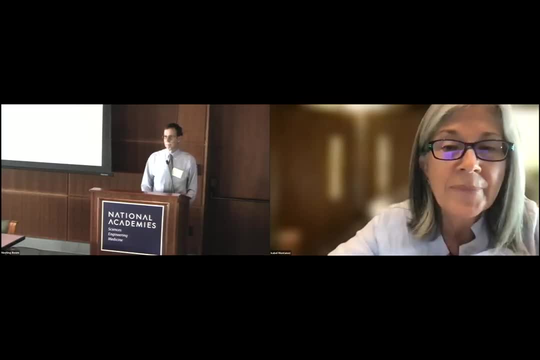 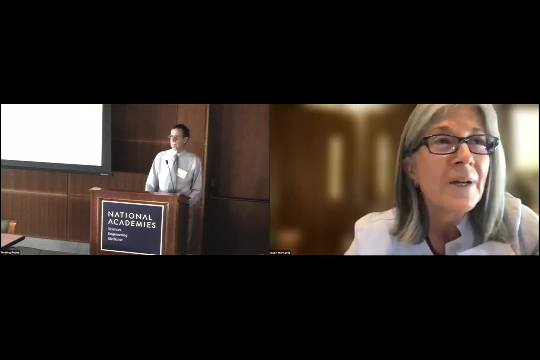 That was a really wonderful introduction to the topic. today We have plenty of time for questions, And so those in the room, raise your hand on Zoom, and then we'll have questions in questions and answer Bob or Robert. Yes, thanks, Bill, for the presentation. 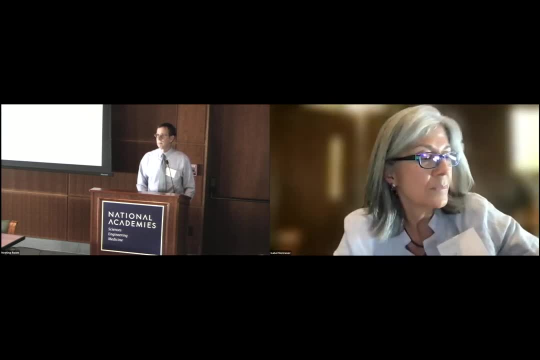 You made a particular note of the comment. the line in the 1998 Academy we study indirect potable reuse is an option of last resort. If somebody said Bill, would you rewrite that? What would you say? I would say that indirect potable reuse. 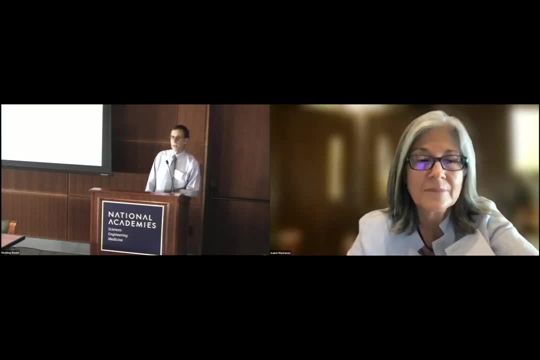 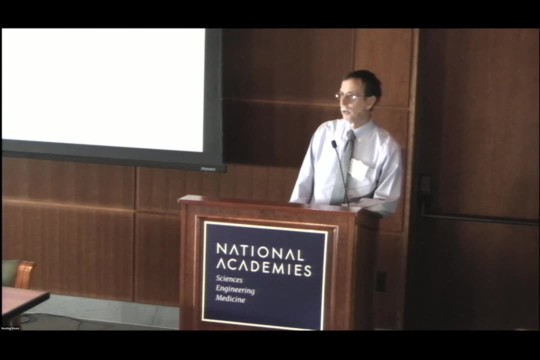 first of all, let's separate the two. if I'm correct, is a fairly advanced technology and it's used in many places. There are many cautions. you don't just jump into it. You need to make sure you've got like the sewer shed idea. 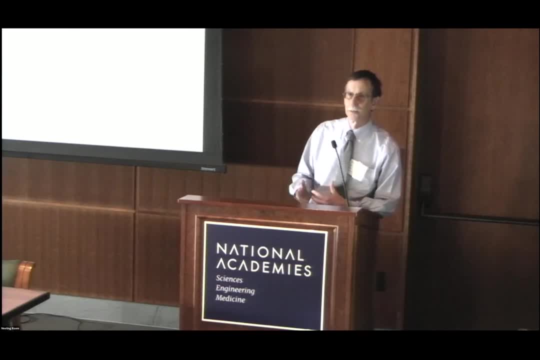 where you try to control the chemicals that people are injecting into the sewer system in the first place. There's operator training, So it's not something that it's easy to jump into, but it's something that people should be planning for in a measured way, I'd say in a small way. 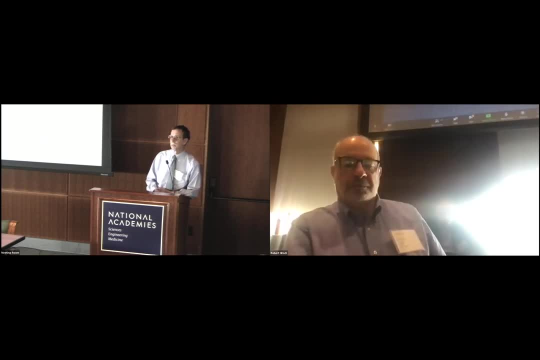 That's what I would say to them. Direct potable reuse is becoming very popular, which is where you don't have the intervening aquifer or the surface water reservoir. Scottsdale, Arizona, is the third place city in the United States that's received essentially. 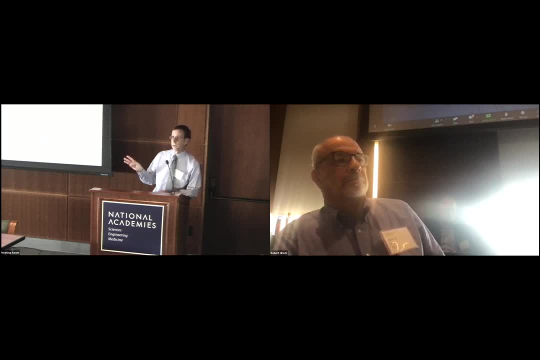 to go ahead for doing direct potable reuse, but they don't plan to do it because they like the aquifers for storing the water for when they need it. So that's one of the downsides of direct potable reuse. There's only one city in the United States. Big Spring, Texas. that does that now, but there's a lot of interest. There's been a lot of pilot studies around the country on that And what we found was that the people, the people who wanted a direct potable reuse- to do, direct potable reuse was. 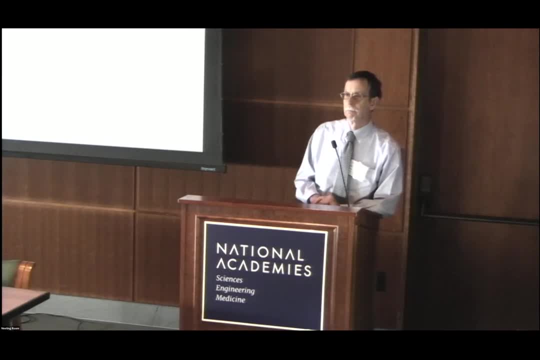 one of these folks and it was all the same. So they were trying to do it with water And I think they're gonna do it with a lot of water, And what they did with that water was they checked the water and they were like: 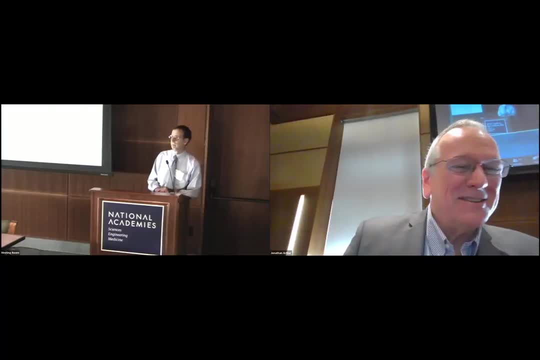 it's going to be under six months of pruning, So there's probably not enough water to actually get it to a certain level. So we spent a lot of time on the fact that they didn't have to do that. So the point is they need to have a lot of water. 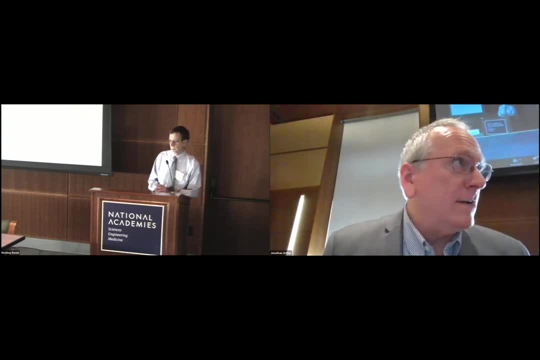 at the time to cover up that water in terms of governance and internationally, uh, can you identify anything without, um, you know, unless you just need to remain quiet until it's published? but are there any aspects of governance that uh, and here in you know? domestically, we, there are some things we could learn from that. 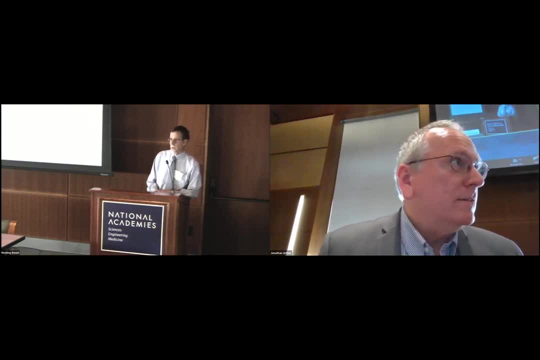 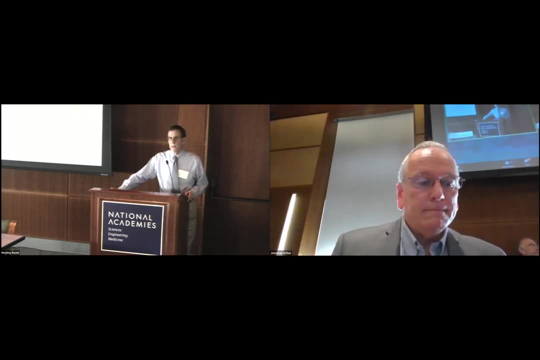 other countries are doing that we just haven't brushed against yet. yeah, so a couple interesting things. first of all, the unesco document that was published. they actually did, um an interesting thing: they came up with indicators of sustainability, uh, for the projects and they evaluated with them. they actually based it on an epa, uh reporter methodology for for that. so, um, 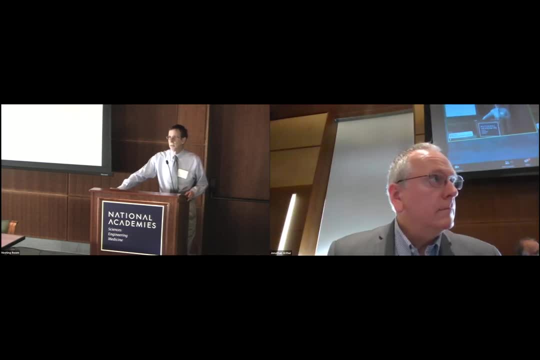 that's one i think thing people need to think about the long term. uh, there um the other part, uh, in the document that i mentioned, the iah, unesco, ngwa, um, there's, there is a lot that's been done by australia, also in governance, peter dylan in particular, but others um, and there they kind of divide up they. 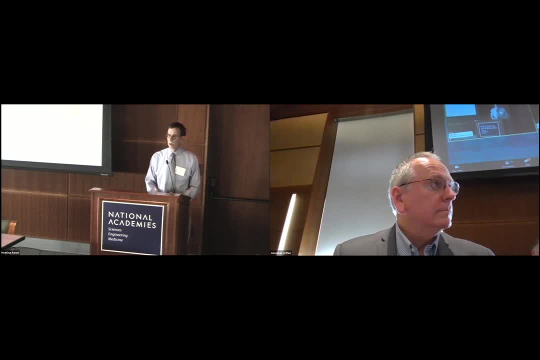 they kind of look at it, um, depending on where you are development-wise in terms of how you proceed forward with uh trying to to, uh to, to manage the manage the situation. but there there are it's very case dependent, of course, um, but there are a lot of issues to think about in terms of, you know, 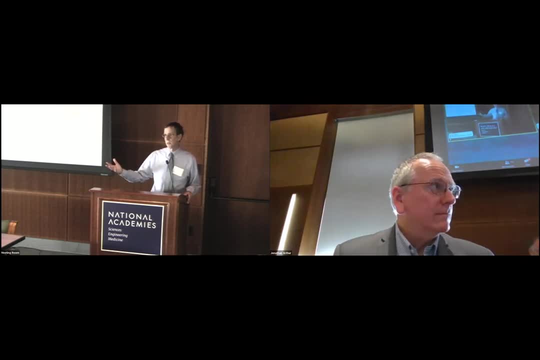 if you uh recharge an aquifer that's been dry for a while and all of a sudden you have springs just showing up, um, in somebody's backyard that bought a house that was dry. so so you have to think a lot about what's going to happen to that, to that water, and what it's, how it might change. 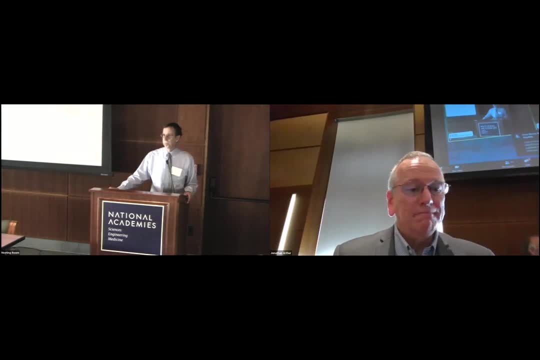 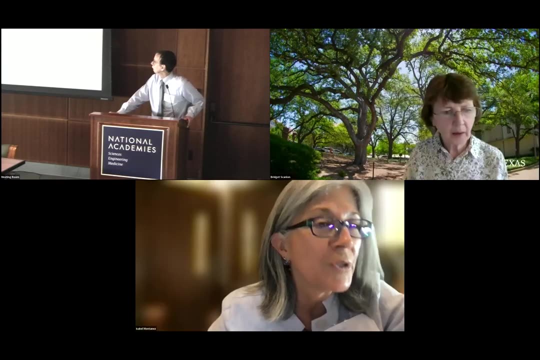 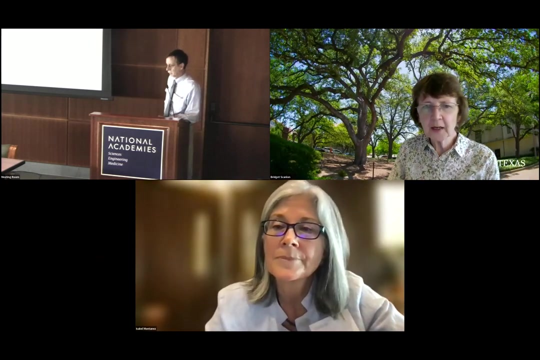 the environment along the way. thank you, uh, bridget, i know you have a question and then there's actually one that i'm going to follow up for you. so, bridget, um thanks, um fantastic presentation bill. um one question in the aurora case, you said the water. 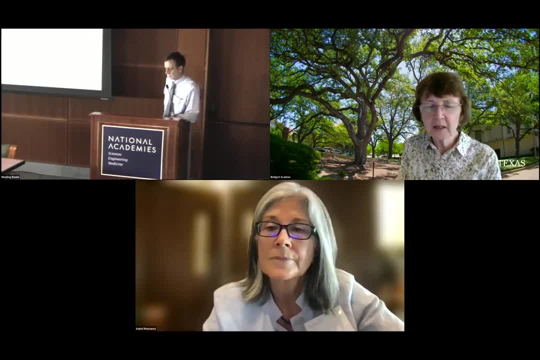 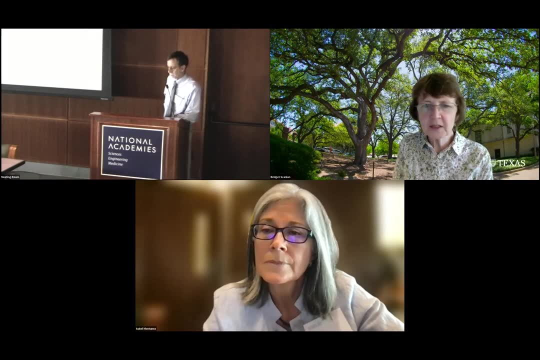 table is about 500 feet deep. how deep are the dry wells and is that the recharge actually reaching the opera? i know claudia font in california sometimes questions the spreading basins and if they're actually recharging the upward that's being pumped um. you know when the 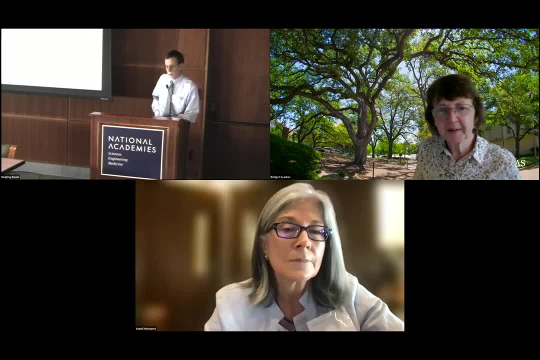 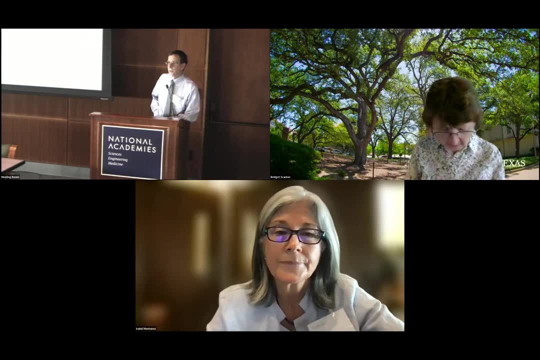 wells that are pumping are much deeper, so just maybe. so that was scottsdale, arizona, actually, and so there's about 500 feet of water. the dry wells are about 180 feet, uh down, so you've got, you know, another 300 feet um it. what's interesting, their water levels have gone up, um, and actually 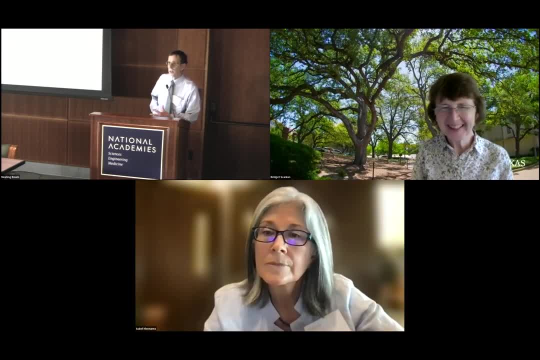 as you may know- i know you know, bridget, but others here may know the um, arizona has set a safe yield, what they define as safe yield, where, in other words, you don't pump any more than you recharge, and scottsdale was the first city in arizona to actually achieve that goal, which is, which is a 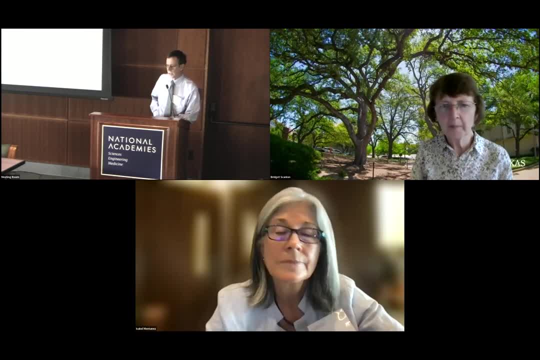 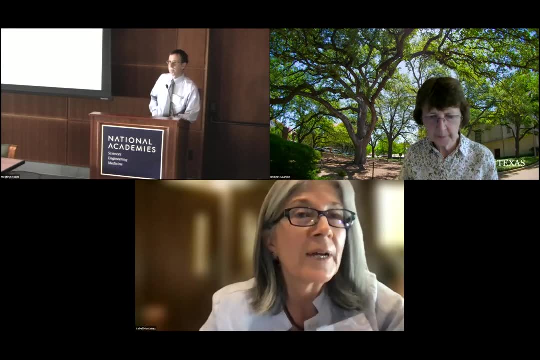 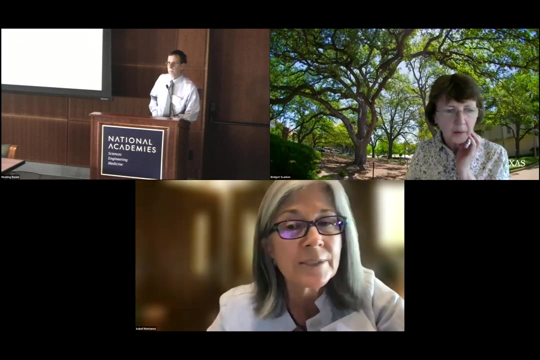 goal set for 2025, but they, they said it some years ago, so i'm i'm guessing it's fairly effective. um, bridget, thanks, okay, and before i go to your question, bridget, um, i did want to comment that sharon meghdal uh said that she'll be providing a link to the unesco book that was just referred. 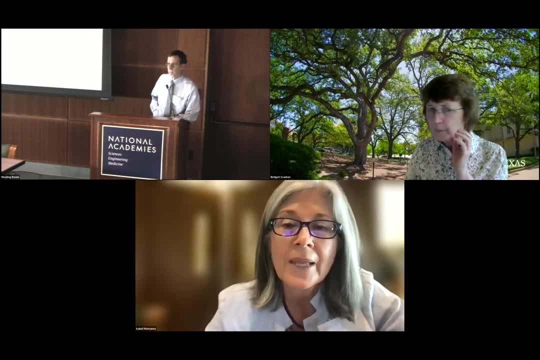 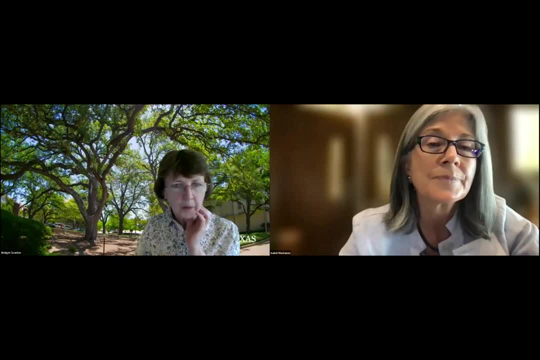 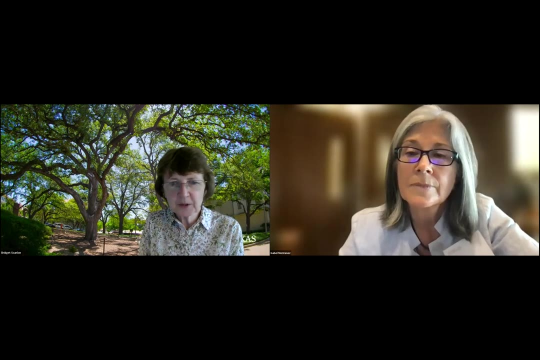 to in her presentation tomorrow. uh, so, bridget, um, do you have a story about the us gs basin characterization model for california available for other states? well, usgs originally had the rasa program and bill could probably speak to this more directly, but now they have regional models in many areas and they continually update them. so 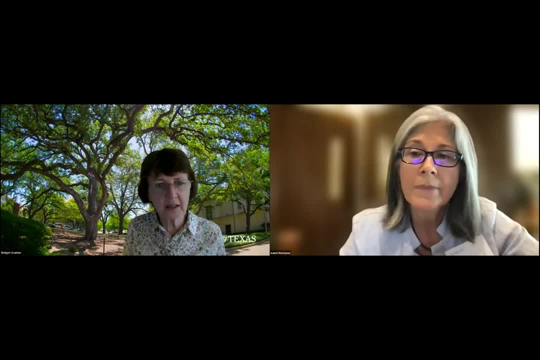 yes, there are models in many regions that texas has the uh, its own modeling program, the groundwater availability modeling, and they have models for most of the aquavers in that area and there are also models in many areas that um. so you know, there are models in many regions. texas has the uh. 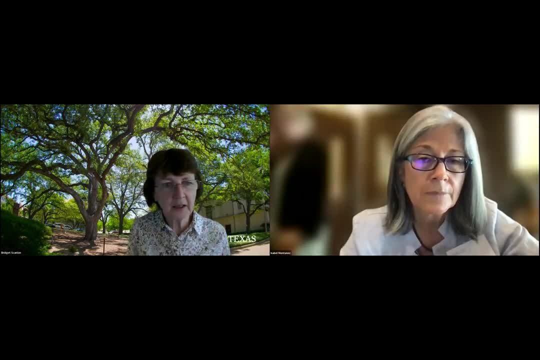 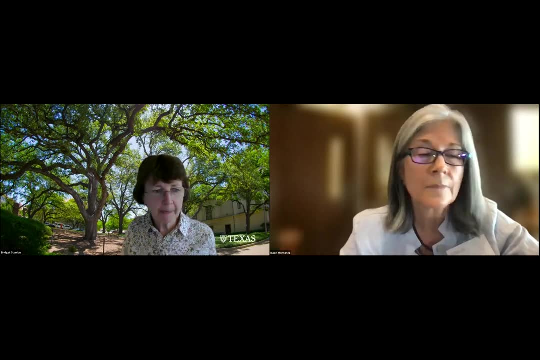 its own modeling program, the groundwater availability modeling, and they have models from most of the aquas in Texas, including the Oglalaal or High Plains aquifer. So, Bill, do you want to add to that? The only thing I'd add is: you'd be amazed. 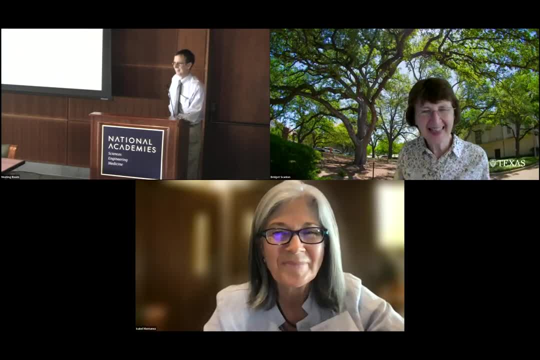 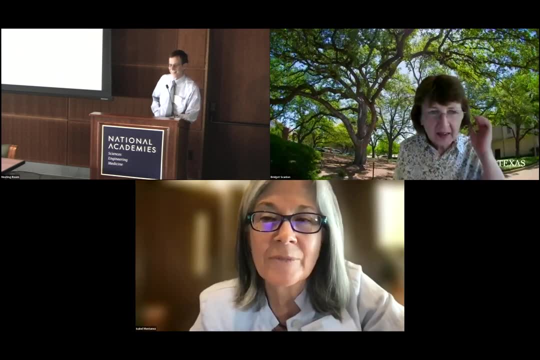 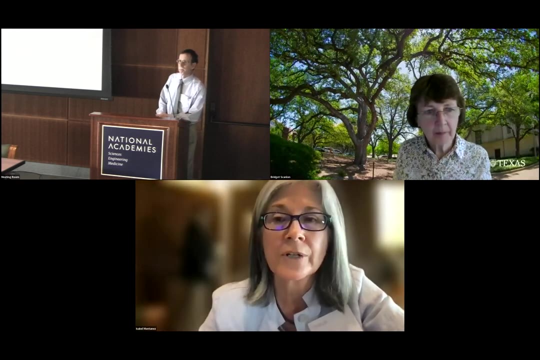 how many groundwater models there are out there. They don't always agree with one another, Thank you. So I have a question that I think from the audience, that I think both of you could probably address: What are the spatial time and spatial scale and temporal lead times at which recharge technologies? 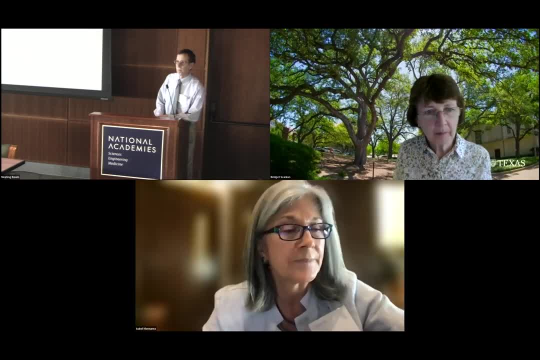 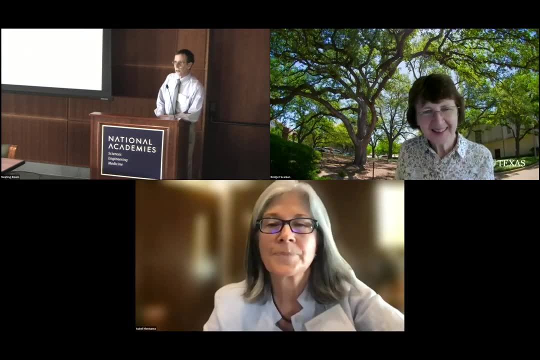 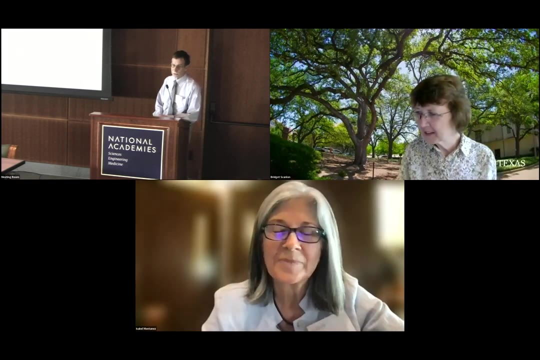 are considered successful water management operations. So either of you want to take that, I'll start. Actually, the person you want to talk to is Sharon McDowell tomorrow. since you have her on the line there, She can help you a lot also. 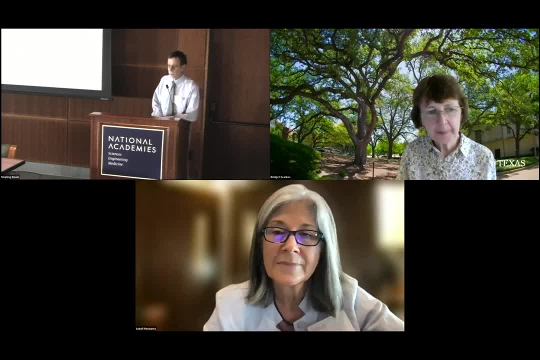 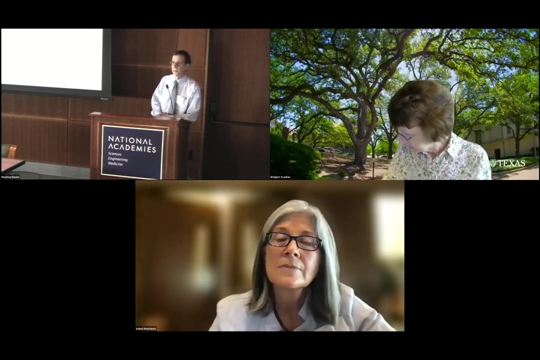 with your governance questions. for sure, Some of it depends on the timescale of the use. So in Florida you may be injecting water underground for use The next season, And so your timescale is that particular season If you're in Charleston, South Carolina. 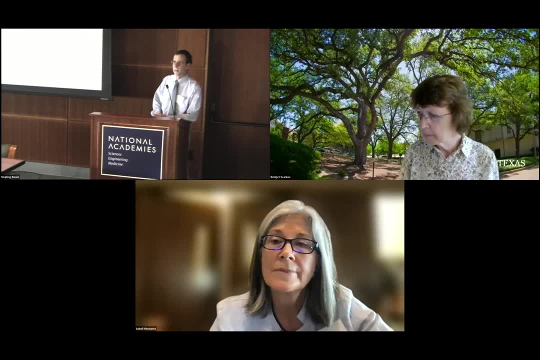 you may actually be putting it underground because you've had an earthquake and floods there and you want to have an emergency source of water, So it's going to be there for a very long time. The Arizona situation is interesting because they have been, as shown by Bridget's work. 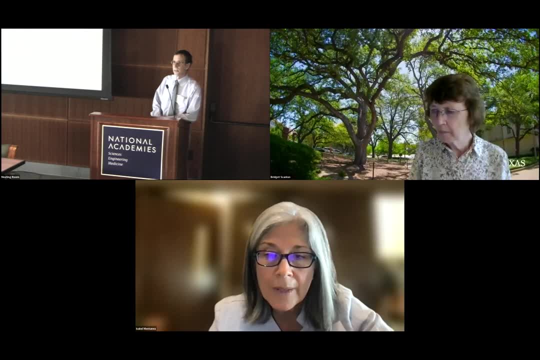 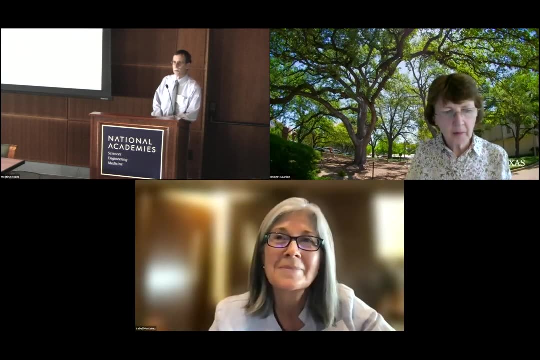 they've been recharging a lot of water And now, as you well know, it looks like they're going to need it. But the question is: where is that water now, And how do you extract it? Maybe just add a little bit. I mean Arvin Edison, one of the basins that has been doing it since the 1960s. they tried to store enough water for the multi-year droughts that they have, So they're putting it in continually when it's a wet period. 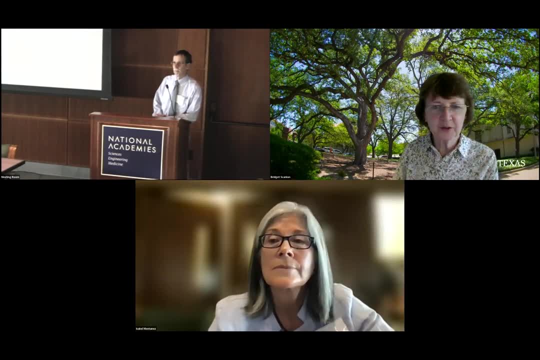 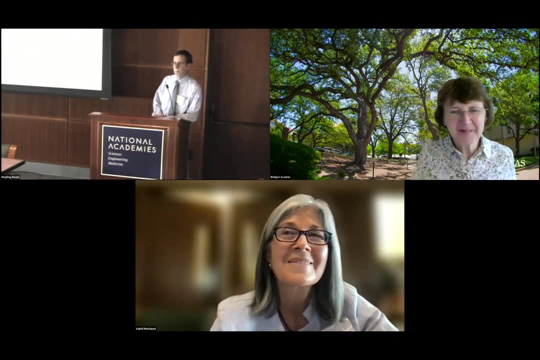 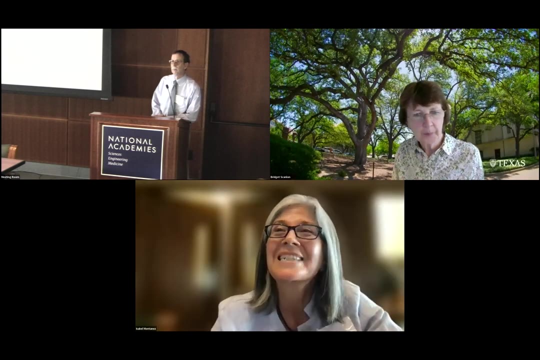 and then all of the wells are pumping during the drought, 24, seven, 365, until they can't, I guess, Neil, I think you had a question. Sorry, I'm having a hard time using the mic and looking at the speaker both at the same time. 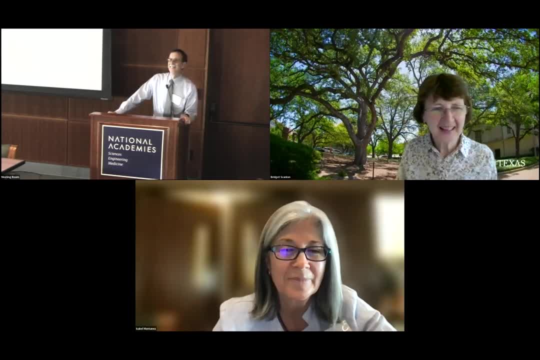 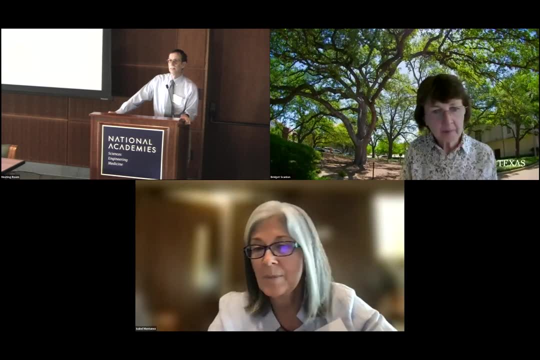 But I can hear you. So I think in the Southwestern US, one of the implications of climate change over the next 50 years is that we will expect more extreme precipitation events, And I think in say, for example, in New Mexico, 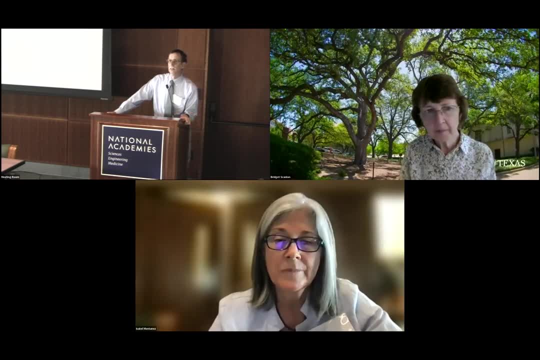 we know roughly what part of the state is likely to get more extreme precipitation, but we don't know exactly, obviously, where that's gonna happen. Do you have any comments about how methods for capturing water associated with extreme precipitation events in an ASR context? 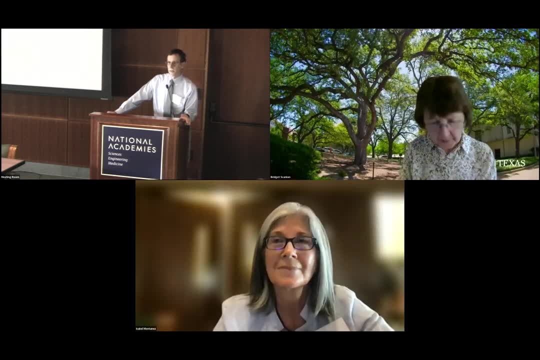 So I know tomorrow you have Helen Dolke on the schedule And I'm sure she's gonna talk about a very large effort in California- I don't wanna say California called flood Mar. that's trying to and actually learning how to operate reservoirs better, to make take maximum advantage of them for recharging the water while you have it. 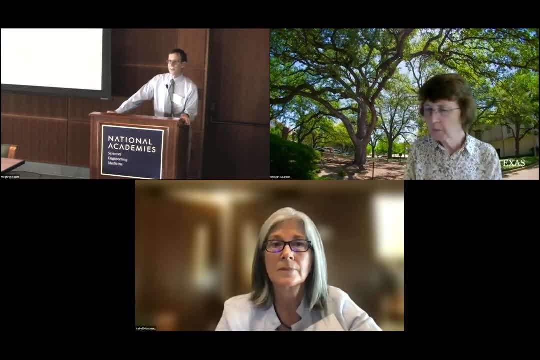 You know, in New Mexico, you know you've got major water issues, especially down in El Paso, and El Paso, by the way, is the first city in the United States to have actually used wells for injection of potable reuse, back in 1985, and they have continued. 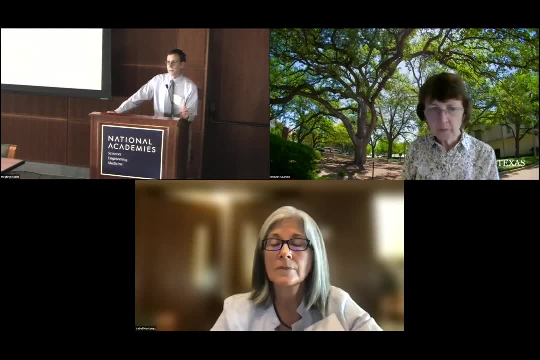 they're continuing to expand their program there. one city that's actually going to be the largest city in the US that has a sizable direct potable reuse program, probably within the next 10 years. So so it's, it's a big deal. 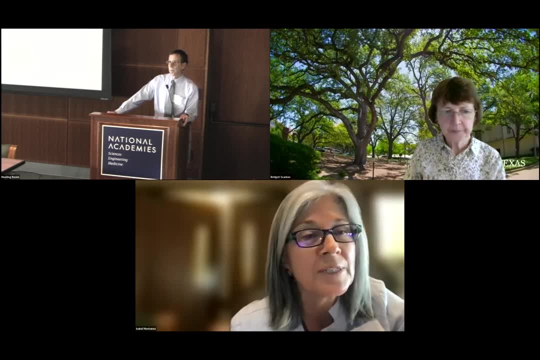 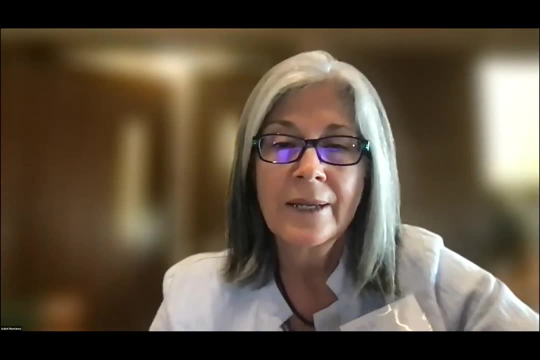 Okay, thank you, We are right on time. there are some additional questions and I'm going to encourage people to bring those up in the q amp a discussion in a little while. So thank you to both of our speakers, And now I'm going to. 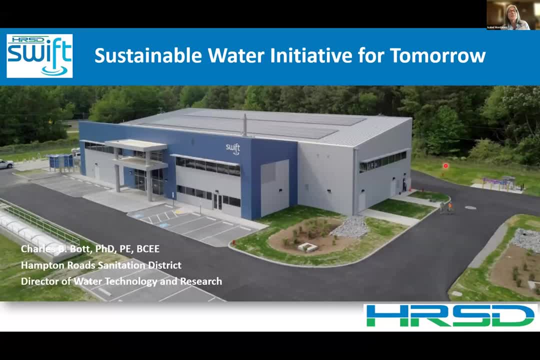 You're going to hear from A series of case studies, presentation presentations moderated by john Arthur, the ex director for the American Geosciences and executive director for the American Geosciences Institute- you didn't know that- And the previous punchy, already previous state geologist, Florida and director of the Florida Geological Survey, and he is a member of the water science and technology board. 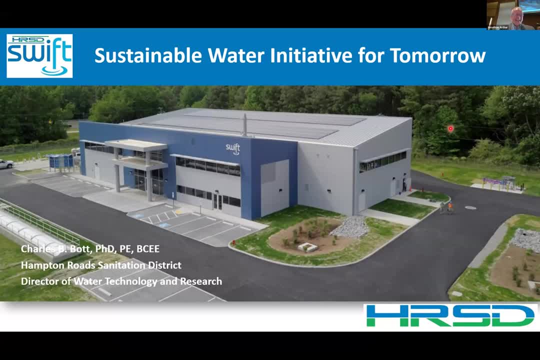 John, Thank you, And thanks for reinstating me so quickly. So in this next session, managed act for recharge case studies. There are abundant applications, as we just heard for Mr, and today we're going to hear from six geoscientists and engineers with experience in these various systems from across the country, through their unique lens. 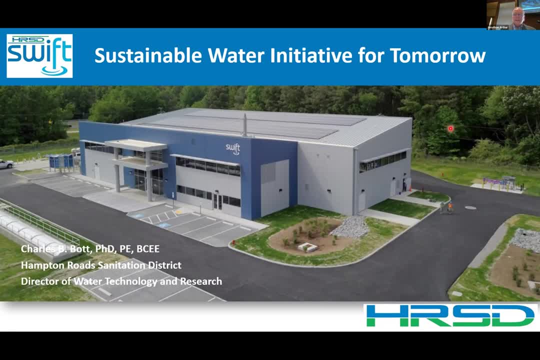 we will hear case studies, successes, caveats, lessons learned, and not only in relation to systems design but also operation management, as well as scientific and engineering considerations that are shaped by local hydrogeology and regulatory requirements. And with that we'll start with our first of our 15 minute presentations with Dr. 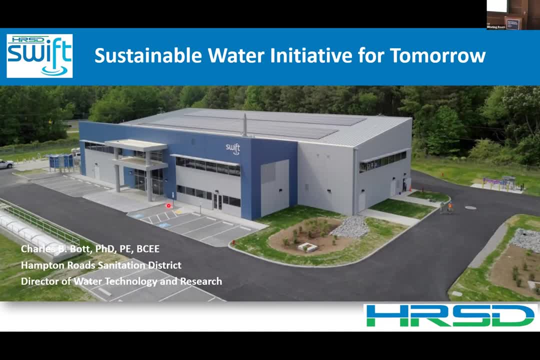 Charles but who is the director of water technology and research at Hampton Road Sanitation District. He manages technology innovation and research and development at the district, 16 wastewater treatment, 17 wastewater treatment plants, And he is also adjunct professor at the Department of Departments of Civil Engineering and Environmental Engineering at Virginia Tech and Old Dominion University. 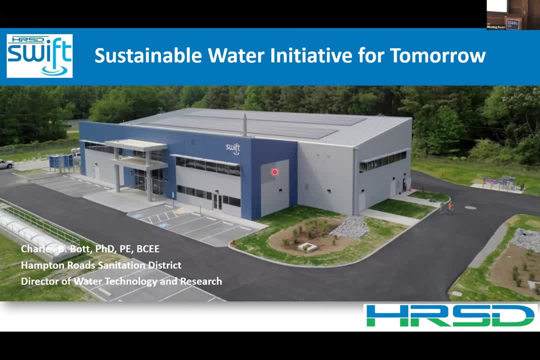 So, Charles, please tell us about Virginia and the Eastern Shore. Okay, thank you. Can you hear me? okay? Yes, good, Well, I think that the slate of speakers for these case studies is an alphabetical order. I I feel a little nervous about speaking ahead of Orange County Water District and the groundwater replenishment system, which is, of course, very well known. 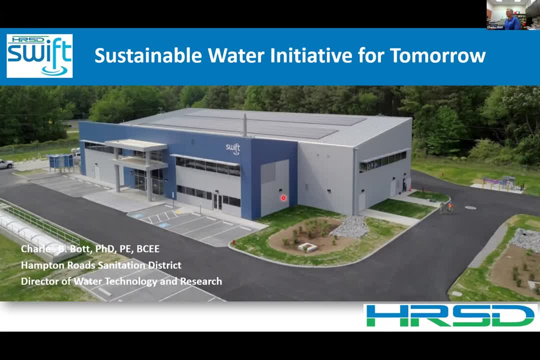 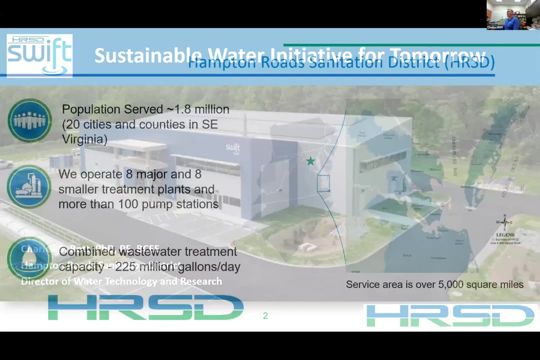 And and many, many years, light years ahead of what we're doing at HRSD. So, anyway, this is our swift research center, a demonstration facility for indirect potable reuse and managed aquifer recharge, and I'm going to tell you a little more about our study here. 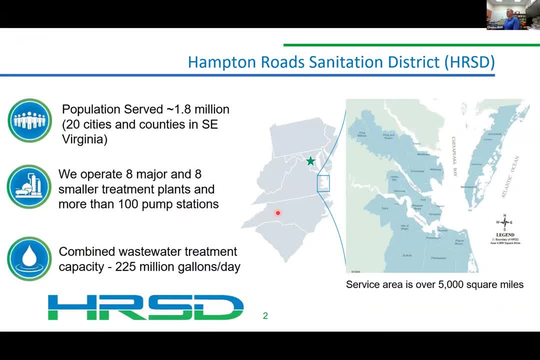 Our work here. This has been going on now for about five years. we're into the swift program. but but first a bit about HRSD. we serve about 1.8 million people in southeast Virginia and operate about eight medium to large plants and eight or so smaller plants with a combined 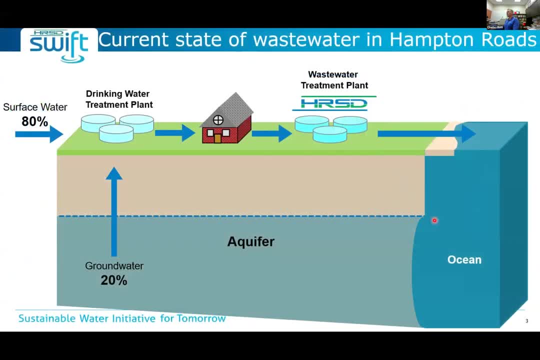 capacity of 225 MDD. The status of water in Hampton Roads is, that is, that approximately 20% is supplied by groundwater. about 80% of the population is supplied by surface water. As we move west in our service area There's much more reliance on groundwater than surface water and more reliance on surface water at in the east. 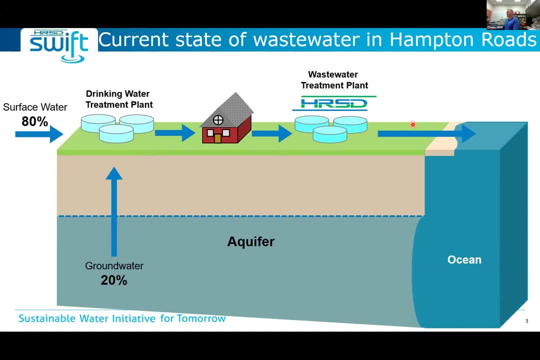 We treat wastewater to now really high standards because we discharged mostly into the Chesapeake Bay watershed. so we've been upgrading treatment plants over the last 20 years for much more substantial nitrogen and phosphorus removal. so as we contemplated our future, One of the considerations was we treat 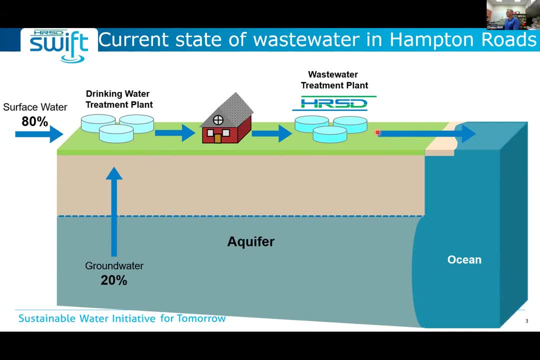 To really high standards and we effectively take this resource and we discharged into saltwater and sort of throw that resource away and it was bothering us and five or six years ago we really started to think about this and over the course of a few years of study, 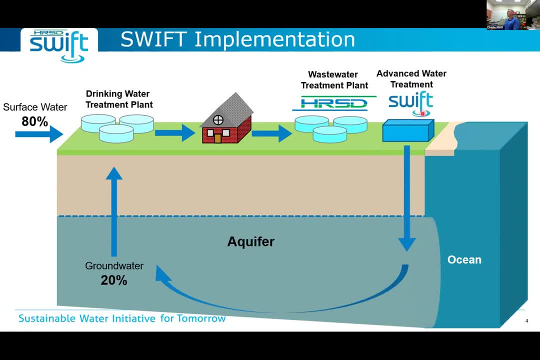 and and and piloting and careful work, we developed the swift program, which involves adding advanced treatment and managed aquifer recharge, and there are a number of benefits for that. first of all, the Hampton Roads area is second only to New Orleans in terms of water. 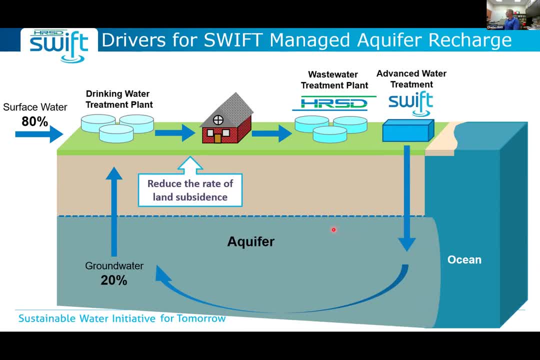 In terms of population and infrastructure at risk of sea level rise, and about half of our observed sea level rise is due to land subsidence. so perhaps managed aquifer recharge has the opportunity to to reduce the rate of land subsidence. Perhaps provides us some regulatory stability by taking our water quality sort of to an endpoint in terms of drinking water quality. 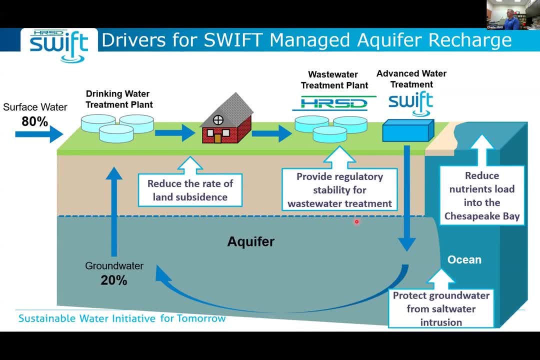 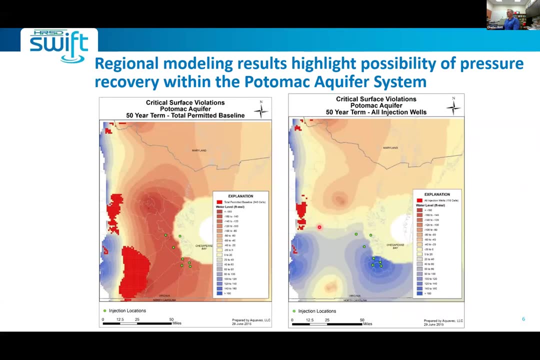 It further reduces our nutrient loads into the Chesapeake Bay. It protects the area of the Potomac aquifer from groundwater saltwater intrusion and provides a sustainable supply of groundwater. so the Potomac aquifer is under pressure of extraction and has been for many years. 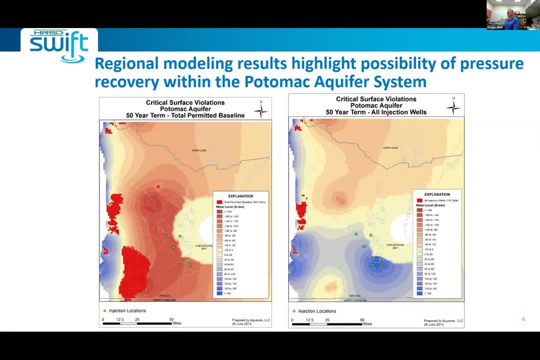 On the left shows Critical surface violations of the Potomac aquifer for over 50 years simulation. The green dots are our treatment plants and this shows a look after 50 years of recharge at. these plants have substantial Rebound and pressure. 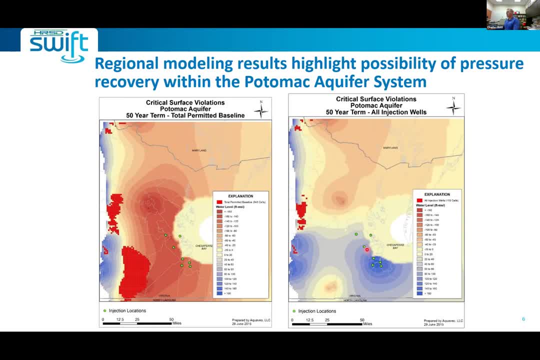 So in this case I'll just make clear that the travel times in the aquifer are thought to be quite long from these treatment plants. you know, more than 100 years for a mile of transport through the aquifer. so swift is really about repressurizing the aquifer and and ensuring 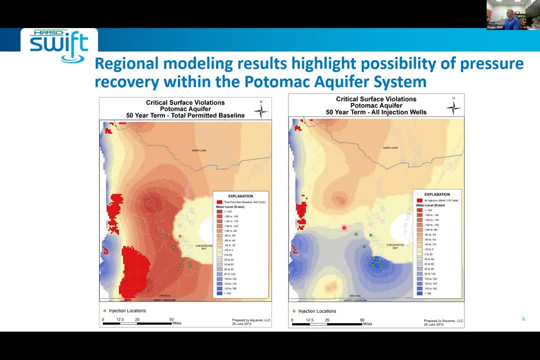 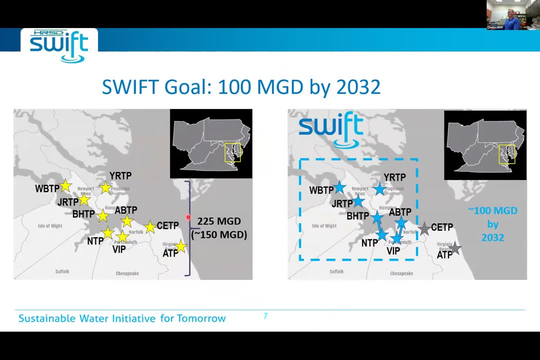 that the that that the pressures in the aquifer remain sustainable, along with the other drivers I just talked about. So the swift, So the swift goal for, first of all, the on the left is our larger treatment plants treating about 150 million gallons per day. The swift goal is 100 million gallons per day by 2032.. Several large capital projects I'll talk about at the end of the presentation. This star Chesapeake Elizabeth treatment plant has already been shut down, shifting flow to Atlantic treatment plant. the Atlantic treatment plant is our one ocean discharge plant. it's too far east in the Potomac aquifer to really be able to. 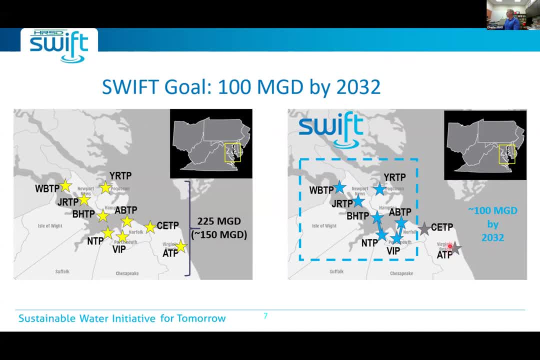 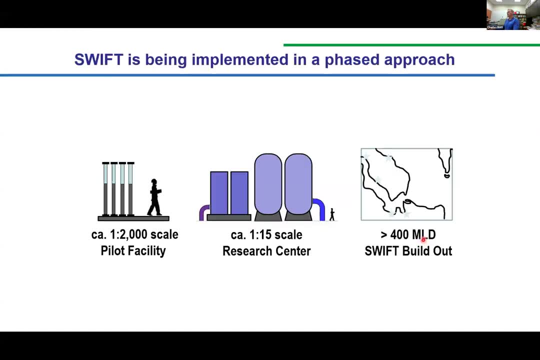 really be useful and it will never be a swift plant by our current planning, in fact, also not a nutrient removal plant, which is a big, which is a big leap in order to get to Swift for our facilities. So we started, as I mentioned, about five years ago, with some pilot testing. we've scaled up now to our demonstration facility, our research center, and we're now starting the build out. 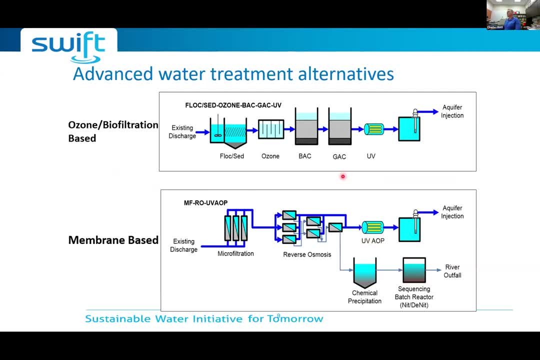 When we started this week, we took some time to consider the advanced treatment approaches And broadly- And I think probably there will be more discussion on this there- to general approaches and the way I like to describe it as the top approach is basically a tricked out drinking water plant that might be treating water from a relatively contaminated surface water. 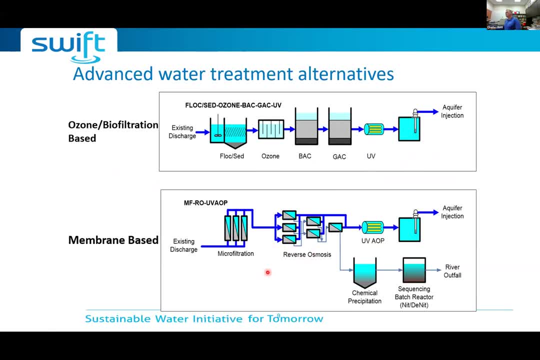 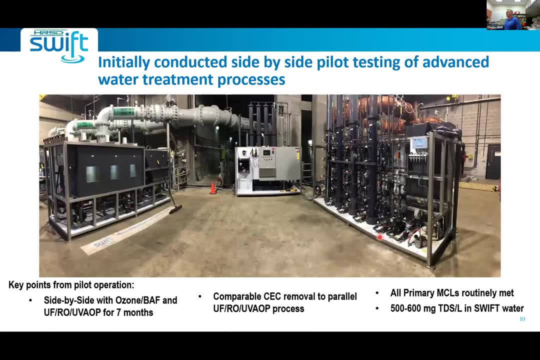 supply And the bottom approaches, what has been typically used in California, involving ultra filtration, reverse osmosis and UV advanced oxidation. So we set out about some pilot testing to determine which of these approaches made sense for us And we worked with- And we worked for quite a while and summarizing a lot of work in one slide- to convince ourselves that ozone by filtration GAC was equally protective in terms of emerging contaminants and pathogens and we could routinely and easily meet primary maximum contaminant levels. 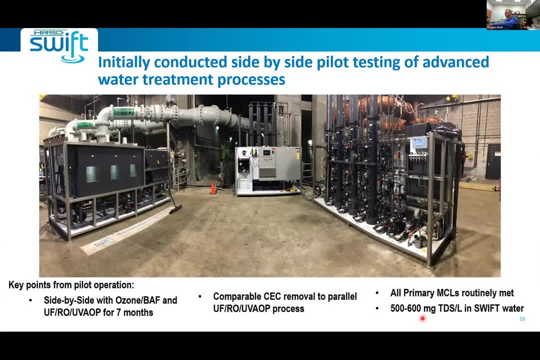 But, of course, there's no TDS removal. It turns out that the status of atomic aquifer in the region where we're injecting is already quite salty and so, to be sustainable in terms of In terms of injection and being compatible with the geochemistry of the aquifer, we really need this TDS for sustainable recharge into the aquifer. 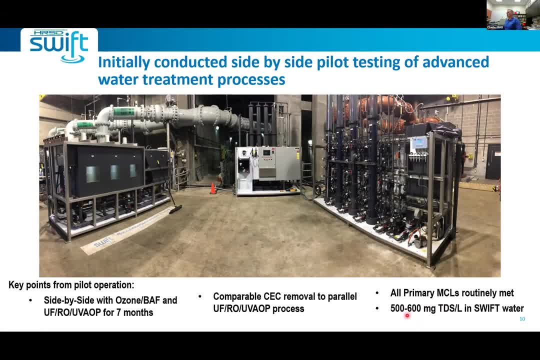 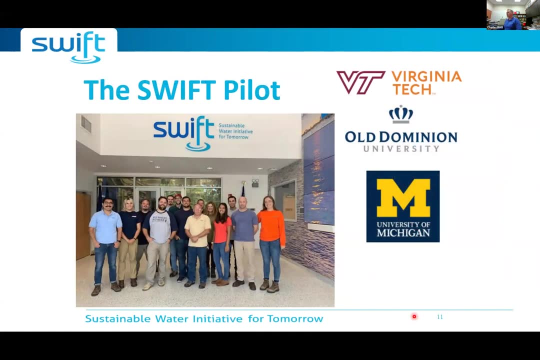 Recharging water, that is, you know, in the 50 to 100 milligram per liter TDS range, is just not sustainable in this aquifer, at this, at this, at these locations, And that pilot work was done by a combination of HSD staff and and quite a few universities. 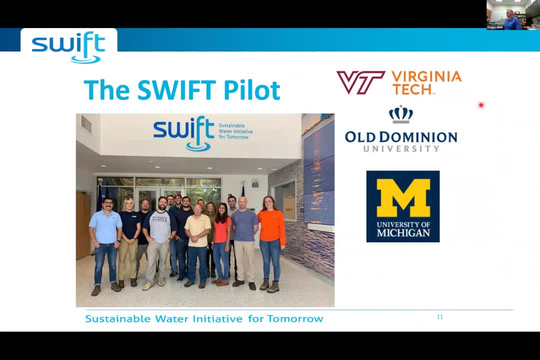 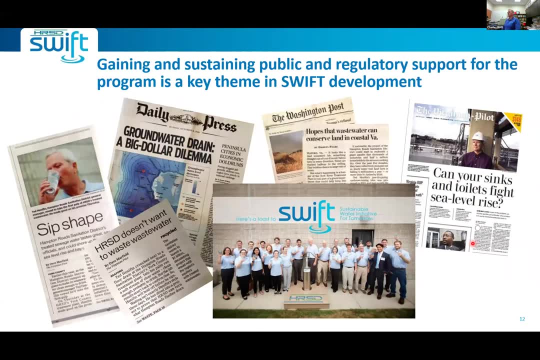 I'm not naming all of them, But the major work by Virginia Tech, ODU and University of Michigan. The other thing that's going on in parallel- and I'm not going to spend much time talking about today- is is gaining really public and regulatory support in the region for SWIFT and within the state and and EPA in Virginia. 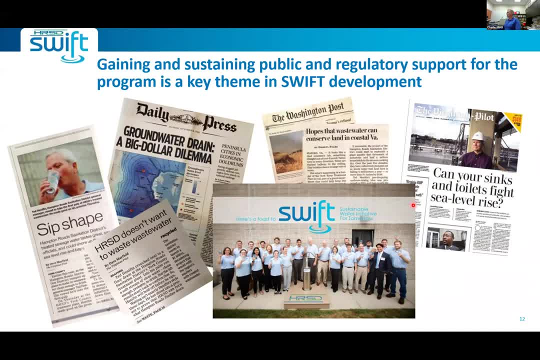 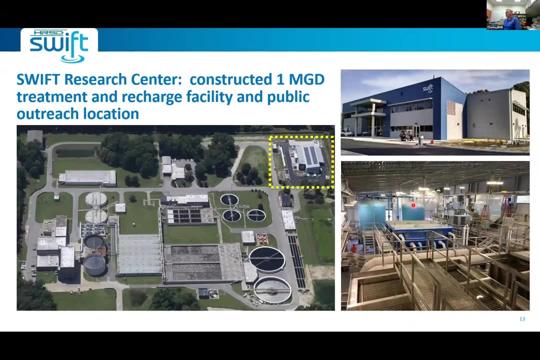 Virginia did not take delegated authority of underground injection control, So our permitting authority is really EPA region three Through the underground injection control program. Three years ago we started up our SWIFT demonstration facility that we call our SWIFT Research Center. This is a 1MGD advanced treatment facility. 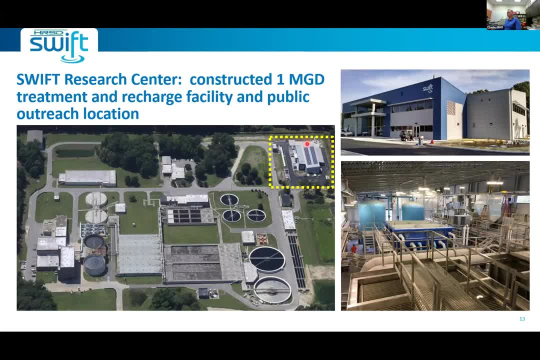 We also have recharge wells and monitoring wells, which I'll talk about, But it's also a public outreach location and public education facility. Even at the 1MGD scale, we're capable of making changes and modifying them In order to test new approaches. 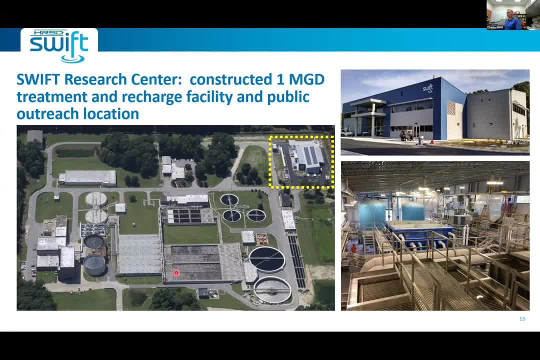 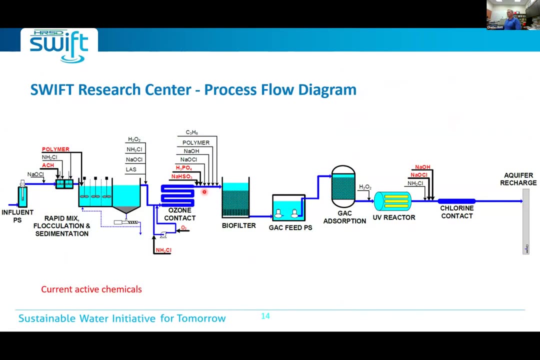 And we located this at a wastewater plant. that's already a quite sophisticated wastewater plant, consistent with the best nutrient removal plants in the Chesapeake Bay watershed. So a five stage Barton Folk plant already doing really good nitrogen and phosphorus removal. The SWIFT Research Center process flow diagram is that ozone bifiltration approach. 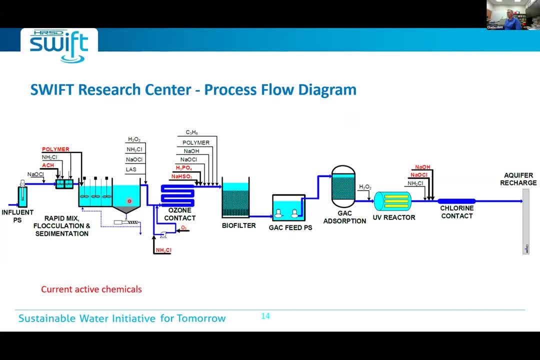 So coagulation with aluminum chlorohydrate polymer addition, flocculation, sedimentation, Ozonation and then biofiltration. And the purpose of ozonation here is both emerging contaminants oxidation, pathogen disinfection, as well as oxidation of bulk organic carbon to make that organic carbon more biodegradable in the biofilter. 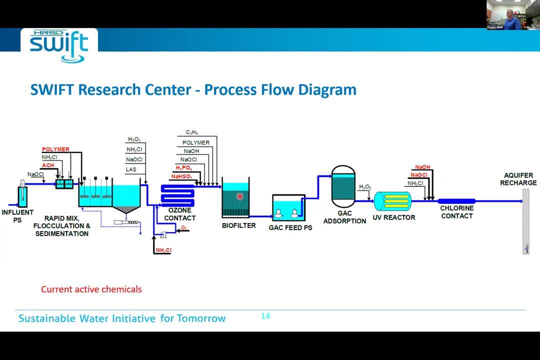 The biofilter is operated like a drinking water filter with very stringent turbidity requirements. And then GAC, granular activated carbon absorption, for polishing of emerging contaminants, Like PFAS, for example, That aren't well removed. upstream UV disinfection. 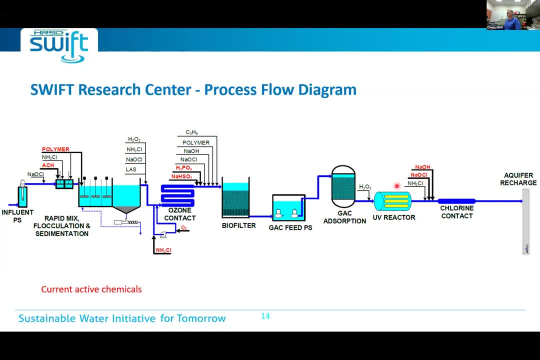 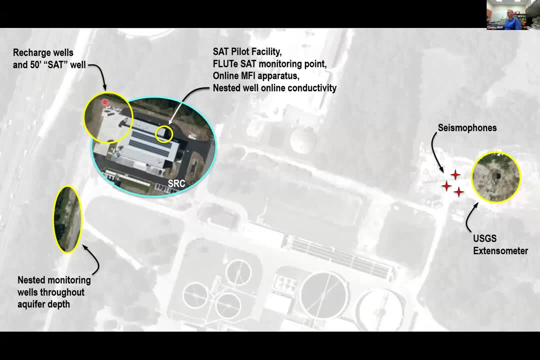 Chlorine addition and pH adjustment prior to recharge. So at the SWIFT Research Center we have a couple of interesting features. One is a recharge well and a very closely located well to look at soil aquifer treatment Monitoring wells, which I'll talk about in a second. 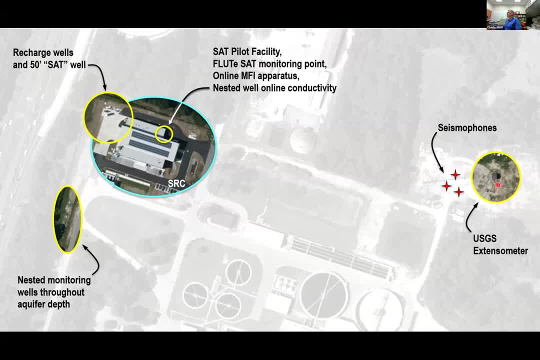 We partnered with USGS to install an extensometer to really measure land subsidence and contraction- I'm sorry- Land subsidence, Distance and rebound as a result of just this one million gallon per day. well, We partnered with Virginia Tech to put in a network of seismophones to look at seismic activity as a result of recharge over the future years. 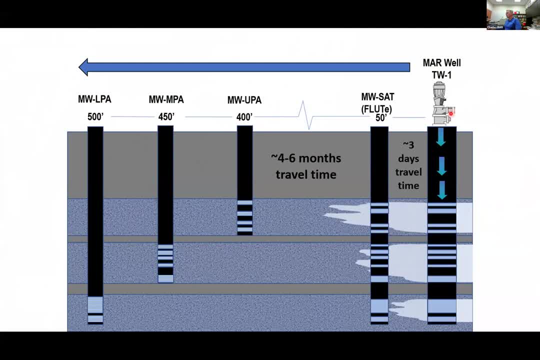 And so in cross section, this demonstration facility includes a recharge well located 50 feet away and three days travel time, and screened in exactly the same locations. There's a monitoring well with a flute sampling system That allows us to take discrete samples from the system. 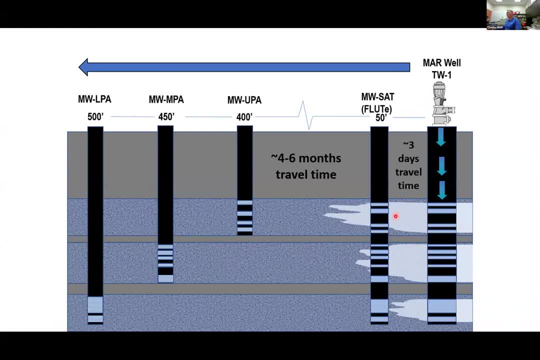 We see already a lot of soil aquifer treatment, with three days of travel time, and some interesting trends as a result of both organic and inorganic contaminant transformation and removal through the aquifer. And then, some months away, is wells, a nest of wells, located in the upper, middle and lower Potomac. 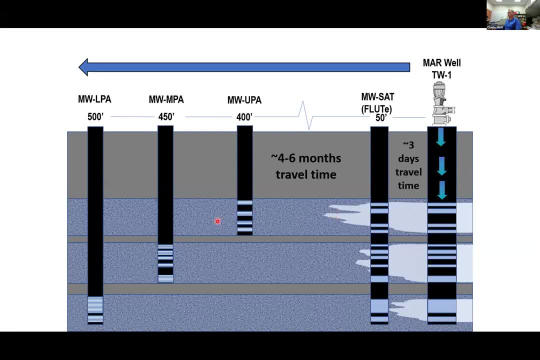 The upper Potomac. the SWIFT water has reached the upper Potomac aquifer. It has also reached the middle Potomac, but not hasn't, seemingly, passed by completely. but it has not reached the lower Potomac. 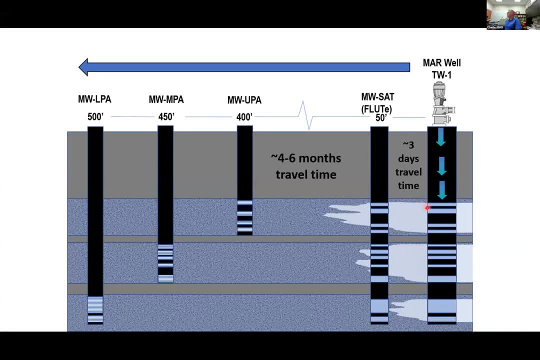 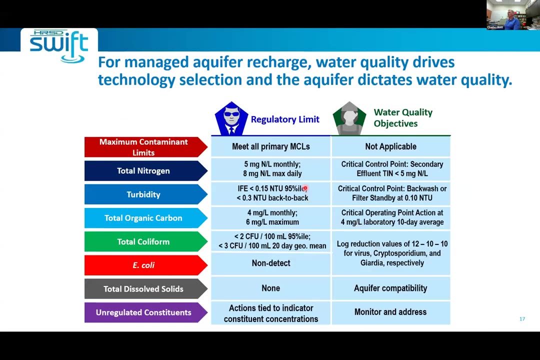 So there is some very significant differences in preferential flow through the aquifer, with the more transmissible zones sort of transporting more water. From a regulatory standpoint, this is what the SWIFT Research Center is requiring And also our first full-scale facility meeting all primary MCLs. it turns out that's pretty easy. 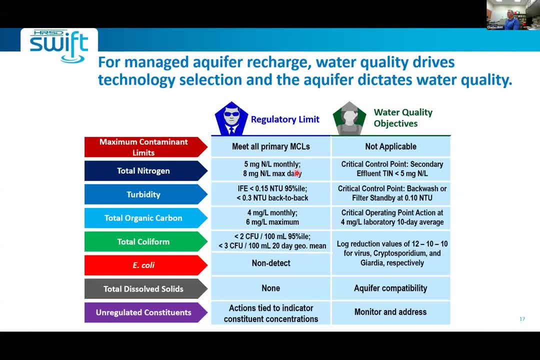 We do that at the secondary effluent of the wastewater plant. Total nitrogen: five monthly eight max day, not challenging for our wastewater plants But a critical control point. effluent: TIN. secondary effluent: TIN: less than five based on ammonia and NOx. measurements that are online. 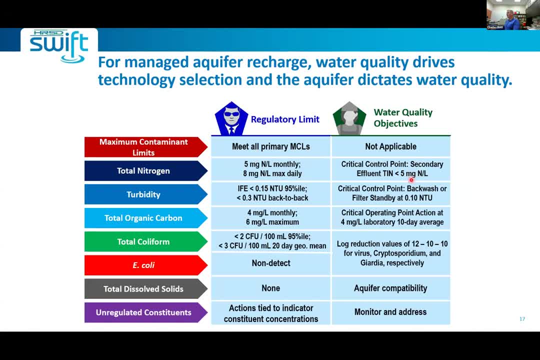 So online measurement of TIN? That's really challenging because it's spectacular. A 15-minute level of performance. Turbidity requirements consistent with drinking water TOC of four maximum month six maximum any sample Total coliform and E coli requirements consistent with the groundwater standards in Virginia. 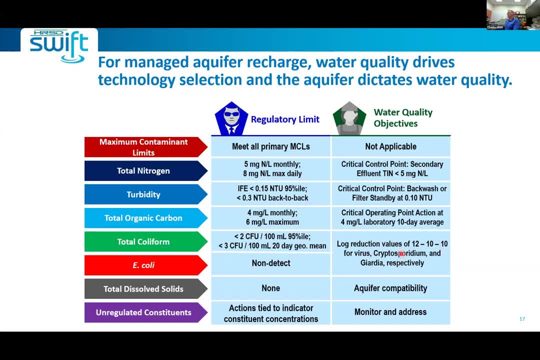 But treatment goals of 12,, 10, 10 consistent with the California requirements. No requirement for TDS, so that we remain compatible with the aquifer. And unregulated constituents are being handled very similar to other potable reuse applications, with two lists. 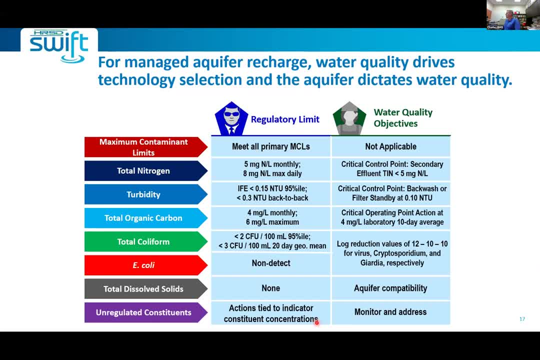 One short list of contaminants that tell us something about the performance of the advanced treatment facilities, advanced treatment processes, And another list that are the compounds of concern and potable reuse Things that we know are concerning in these types of treatment systems, like PFAS and 1,4-dioxane and NDMA and so on. 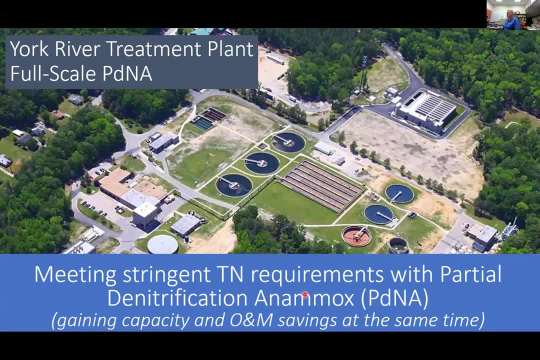 So I mentioned the nitrogen removal required. This is something that at HRSD, we're quite proud of And, you know, maybe in the end is more substantial and meaningful than SWIFT. We are really excited that we've been able to deploy mainstream animox through the partial denitrification pathway. 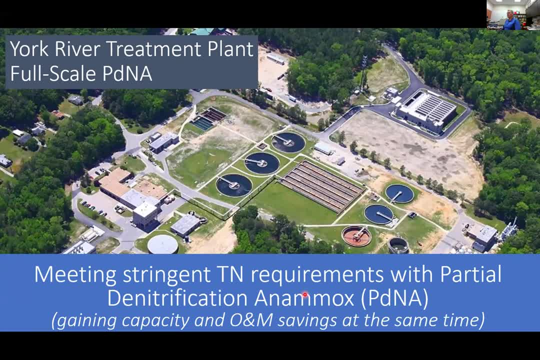 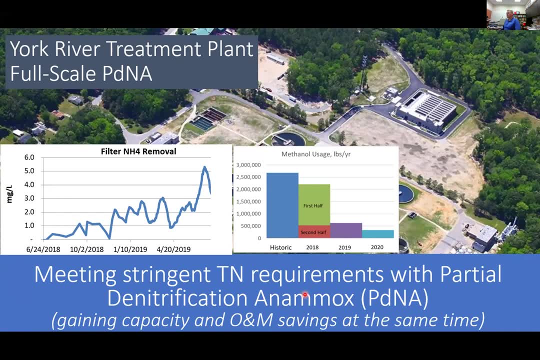 We're doing this at our York River treatment plant. We're in construction right now at our James River treatment plant And the benefits are just tremendous In terms of making nitrogen removal stable and reliable And doing it in smaller and smaller and more intensified wastewater treatment plants. 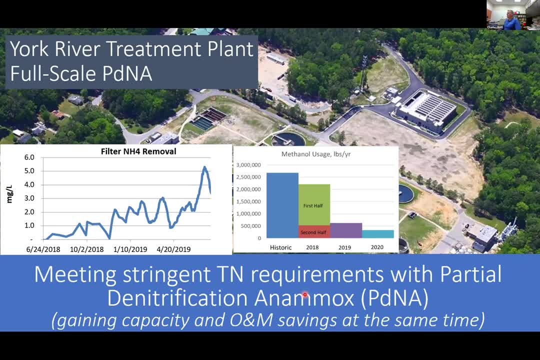 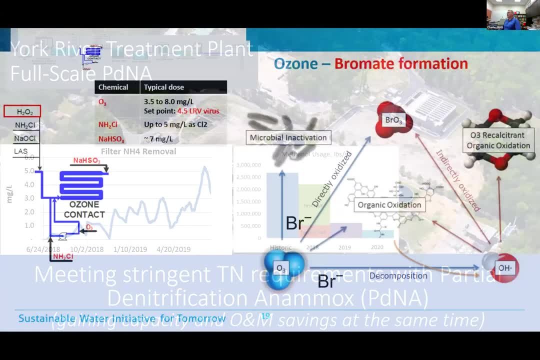 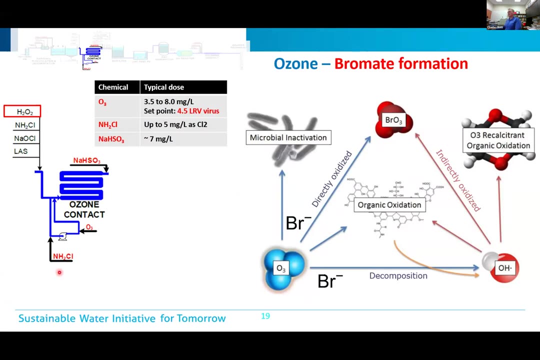 And this is really a requirement if we don't pursue reverse osmosis-based potable reuse. So a little bit about some advanced treatment topics that we've been working on. So our current ozonation process uses preformed monochloramine to control bromate. 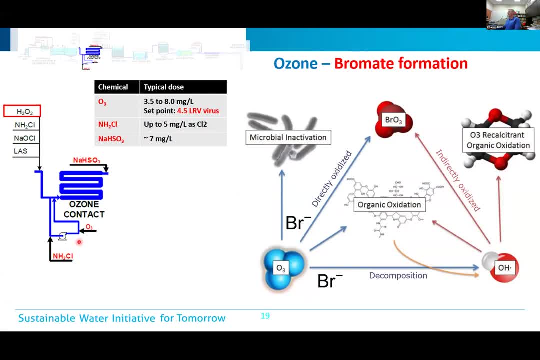 To control bromate formation and high bromide secondary effluent, And that works quite well. We rely on ozone, as I mentioned, for both disinfection and oxidation, And ozone in wastewater really acts like an advanced oxidant because it very quickly decomposes to hydroxyl radical. 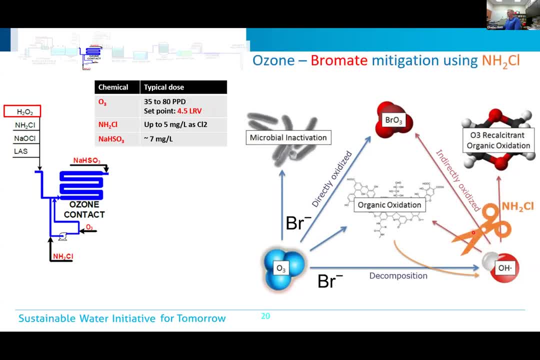 The way preformed chloramine works is by partly shielding. It works in several ways, But one of the mechanisms is by partly shielding and serving as a sink for hydroxyl radicals, While preformed chloramine does a nice job of minimizing bromate formation. 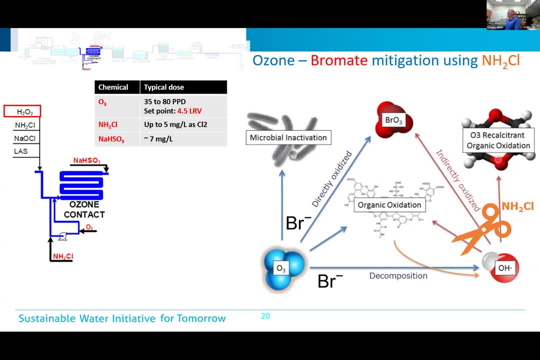 It also hurts us to some degree from the standpoint of oxidizing emerging contaminants. Hey Charles, we've got about a minute, Okay. Another possibility is hydrogen peroxide. Hydrogen peroxide enhances the removal of emerging contaminants, But it hurts us because we don't get CT credit for disinfection. 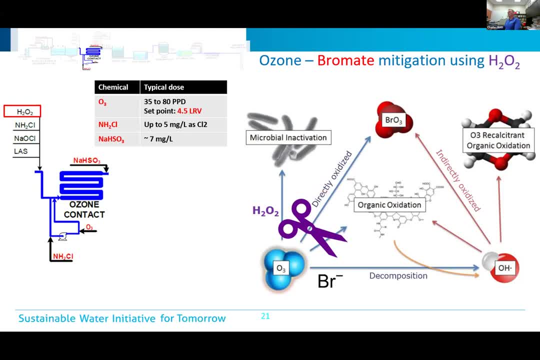 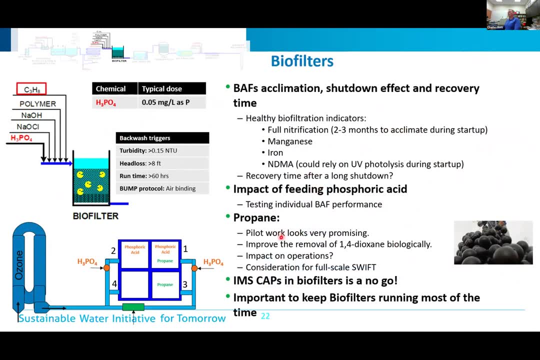 While we know we actually do get disinfection With peroxide. I'll just say quickly that from a biofiltration standpoint, we've learned a lot. We're doing some work on adding propane to the biofilters to enhance 1,4-dioxane removal. 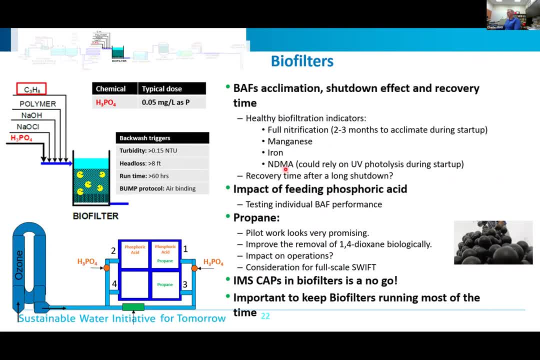 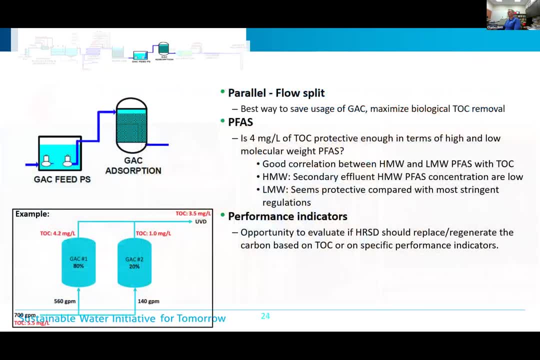 We've learned a lot about how these biofilters remove effectively NDMA, fully nitrify a little bit of ammonia. This is a picture of those modifications to the full-scale filters From a GAC standpoint. one of the questions that we get all the time is PFAS. 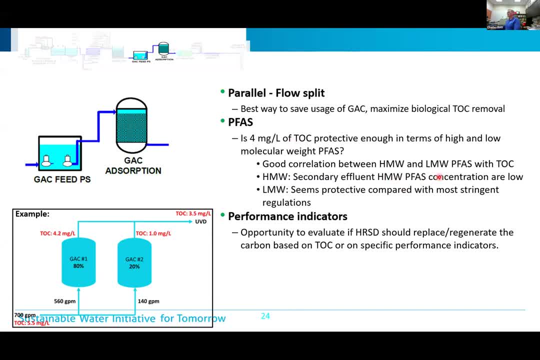 And we've done a lot of work to look at that. We look at both high molecular weight and low molecular weight PFAS, Getting ourselves really comfortable that 4 mg per liter TOC is really protective of low molecular weight PFAS compared with the most stringent regulations from around the world. 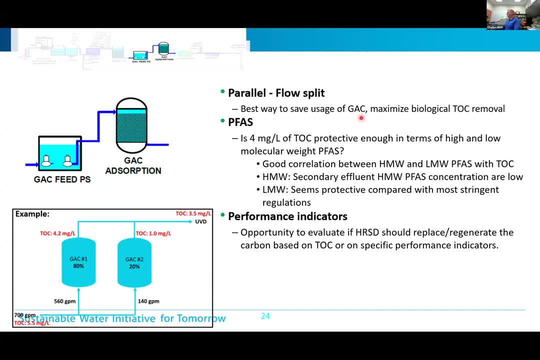 And, of course, we'd like to minimize GAC utilization. GAC is a big cost for the SWIFT program And really maximizing biological removal of TOC in the GAC contactors is a real benefit, particularly in the summertime. So the build-out looks like this: 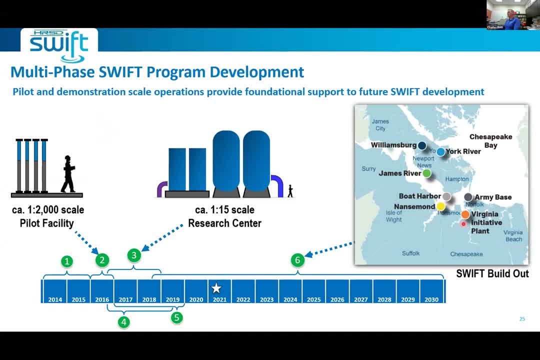 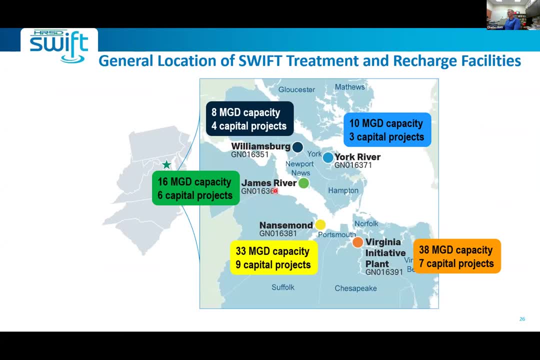 So the SWIFT facilities are shown here. The James River plant is our first full-scale SWIFT facility. It will be. We're in design for this facility. right now We're at the 60% design for this facility. This is a project that's between $400 and $500 million capital project. 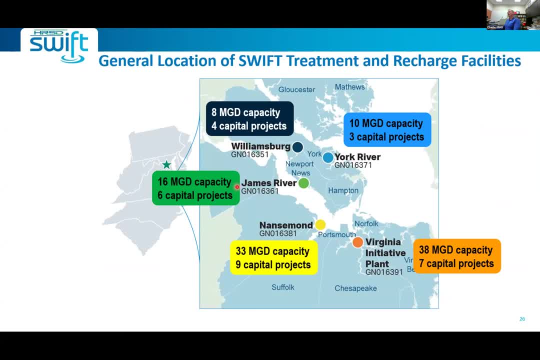 So a huge project for us And the James River project is proceeding ahead with the EPA Region III And we're looking forward to it- The EPA Region III- hopefully very soon, hopefully within the next week or two, issuing our full-scale UIC permit for public review. the draft permit for public review. 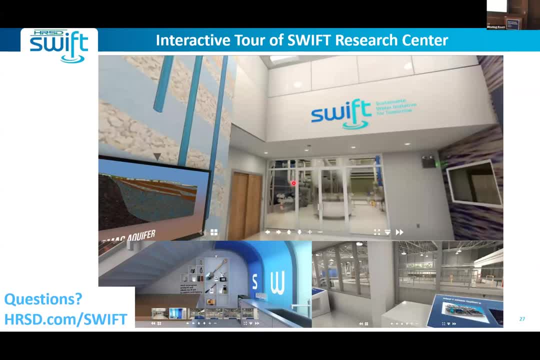 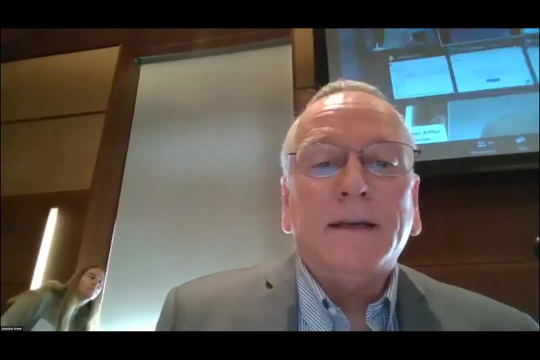 And that's it, Thank you. Thank you, Charles, for an excellent talk, And it sounds like you've got a lot of balls to juggle there. Thank you, And we'll move on to our next speaker, Adam Hutchinson, And so we'll flip over to the West Coast. 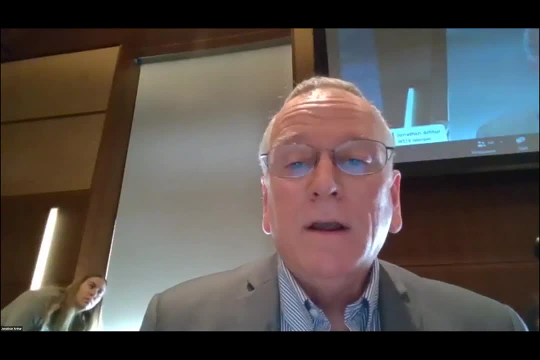 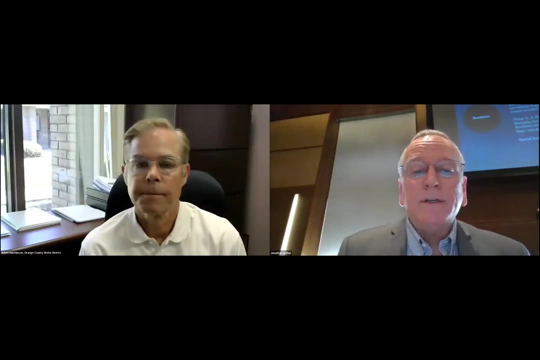 Adam Hutchinson is the Recharge Planning Manager for the Orange County Water District in Southern California. He's responsible for testing and evaluating new methods to increase the capacity of existing recharge system and planning for future expansion of that recharge system and assisting recharge operations and developing optimization strategies. 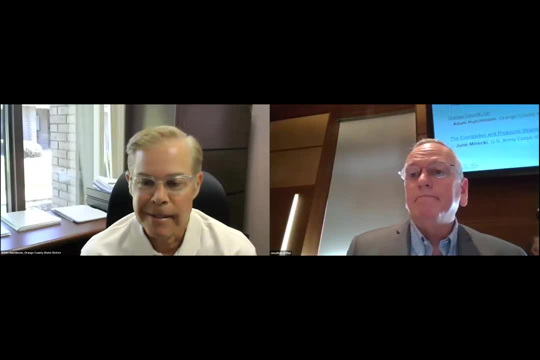 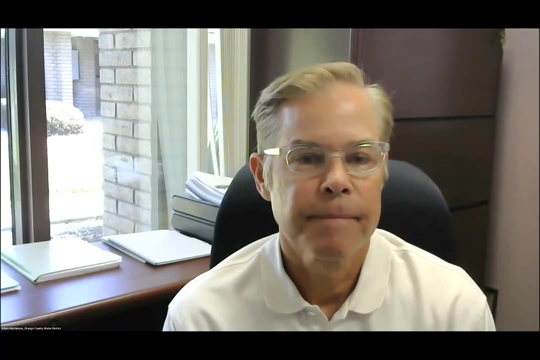 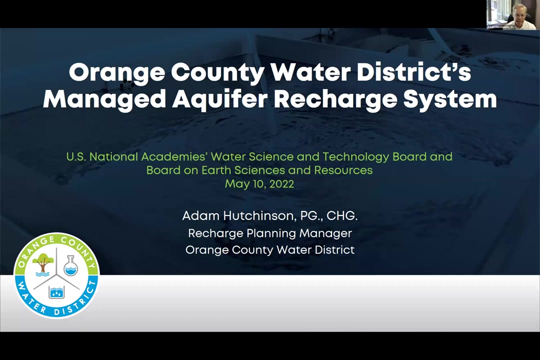 Adam, Hello everybody, Great to be with you. Can we go ahead and put the mic on? Can we go ahead and put the slide presentation up? So we're going to talk about Orange County Water District and our managed aquifer recharge system and what we can learn from that next. 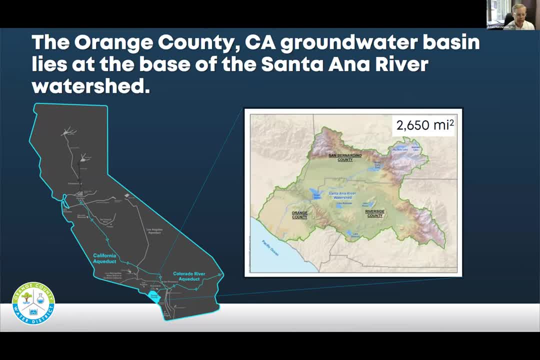 So, just to get everybody oriented in terms of where we are, We are in Southern California, Orange County, Florida, but Orange County, California. We are in the Santa Ana River watershed, which covers over 2,500 square miles. Fortunately, we're at the bottom of the watershed, which has some good characteristics in terms of stormwater capture and receiving water from the Santa Ana River. 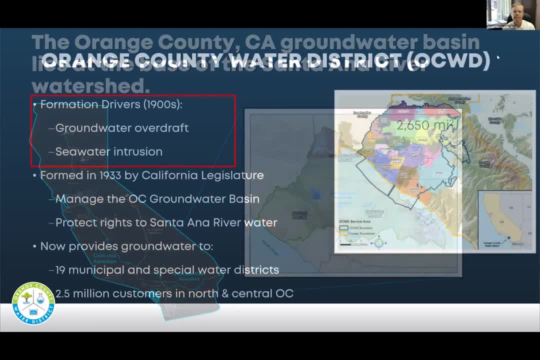 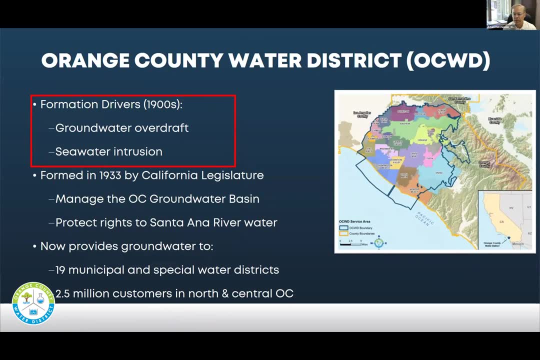 Next, Next slide. So why was Orange County Water District formed? Well, back in the early 1900s There was an explosion of agriculture in the area, hence the name Orange County. A lot of orange growing and other crops being grown. 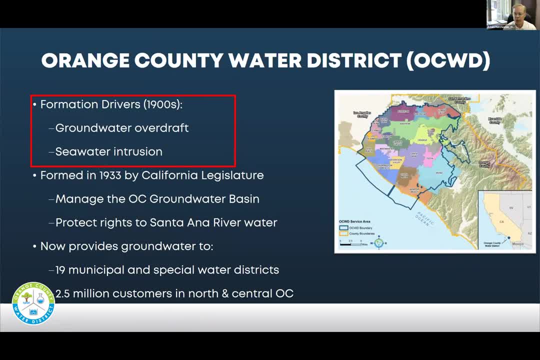 And as a result- not surprisingly- we had a lot of groundwater overdraft, We had seawater intrusion. So the locals in Orange County at the time went to the state and said we need to create an agency to manage the groundwater supply as well as protect the rights to the Santa Ana River which were being diverted upstream of Orange County. 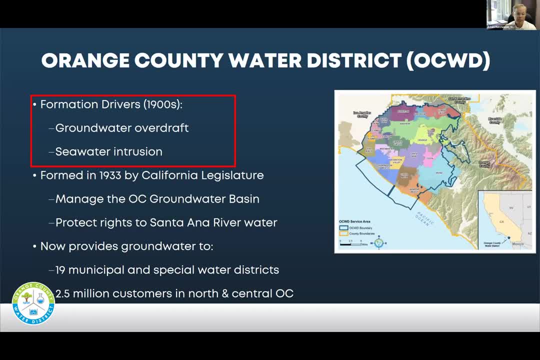 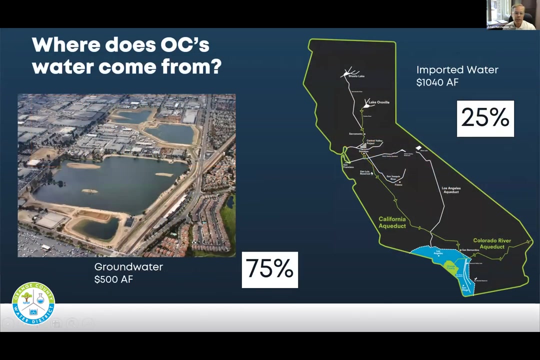 So the Orange County Water District now provides water to 19 different cities and special water districts And there's 2 and a half million people that rely on the groundwater supply in North and Central Orange County. Next slide, please. So in Orange County, where do we get our water? 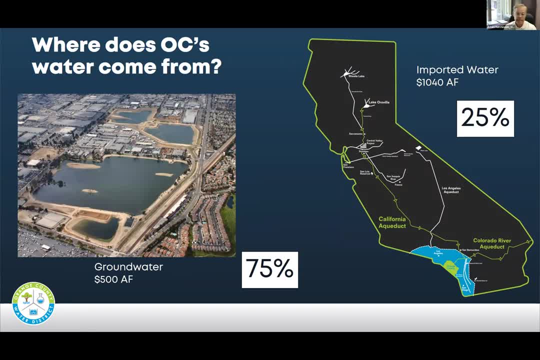 So 75% of the water supplies Of those 19 different agencies is met with groundwater And the cost of groundwater is $500 an acre foot And we charge that fee for every acre foot of water pumped out of the basin. And the alternative, the supplemental source of water, is imported water. 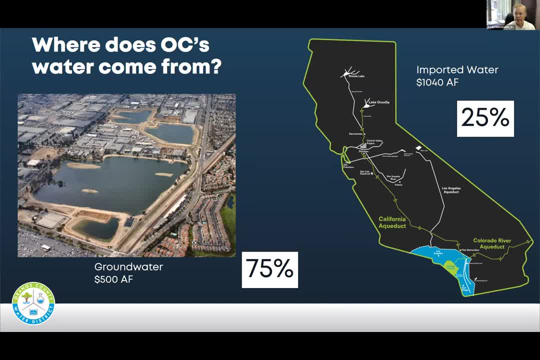 And the cost of that water is more than double. So we're $1,000 an acre foot And that water comes from the Metropolitan Water District of Southern California, which gets imported water from Northern California And the Colorado River. So we have a strong financial incentive to obviously maximize the amount of groundwater available. 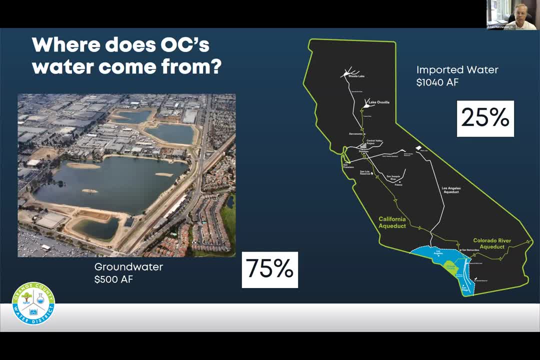 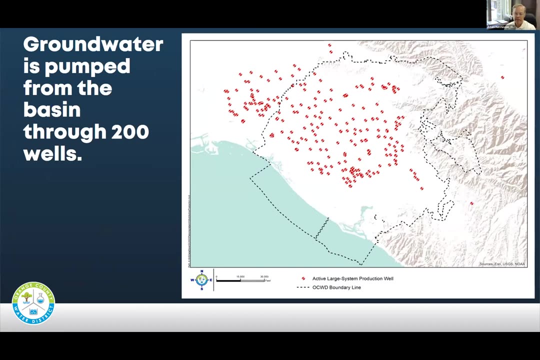 It not only benefits the region, but it benefits our producers directly from an economic standpoint. So next slide. So we have 200 wells that pump water out of the basin, And all these wells have been metered since the 1950s. 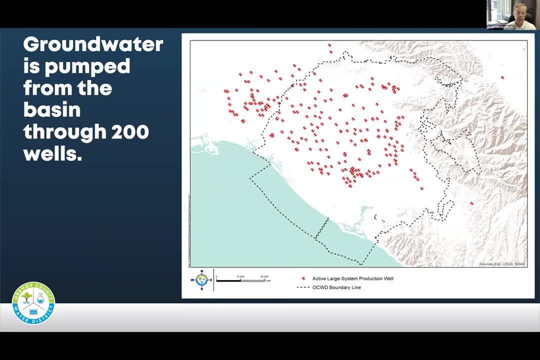 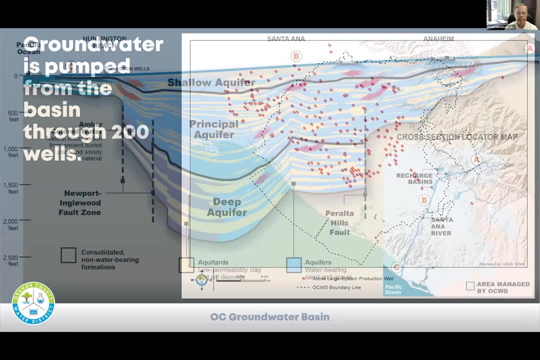 So we have a very good handle on our groundwater budget- what's being pumped, what's being recharged, And so that's a very important element in terms of allowing us to manage the basin properly. Next slide: So this is the cross-section of the groundwater basin. 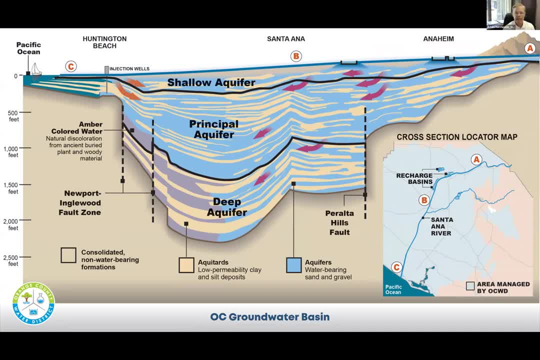 It's a typical alluvial system sedimentary basin of three different aquifer systems, like a layer case. It's a shallow, principal and deep aquifer. The aquifers merge as you go inland toward the canyon area And that's where our surface water recharge facilities are located, where the water can easily percolate down into these three different aquifers. 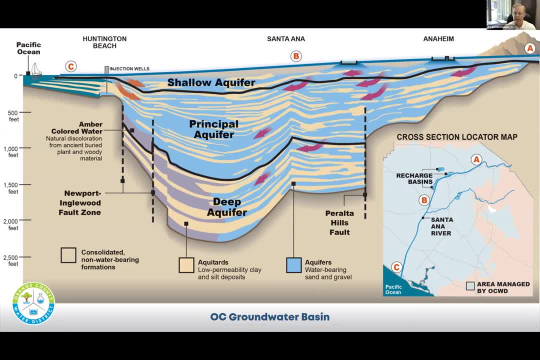 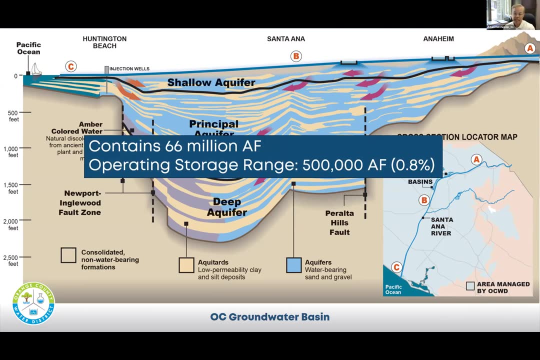 If you try and do surface recharge as you move to the southwest, it won't work because of the subdividing layers, or clay layers, that start to create these three aquifer systems. Next slide: See it dropping. So the basin itself contains a massive amount of water: 66 million acre feet of water. 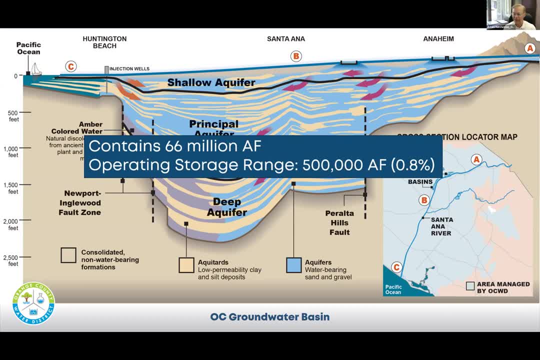 But obviously you can't withdraw all that water without causing a lot of problems. So our operating storage range that we actually try and keep the basin within is only 500,000 acre feet, which is still a substantial amount of water, But it only represents, you know, less than 1% of the total storage in the basin. 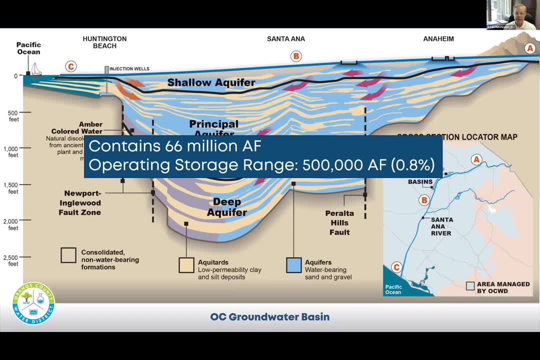 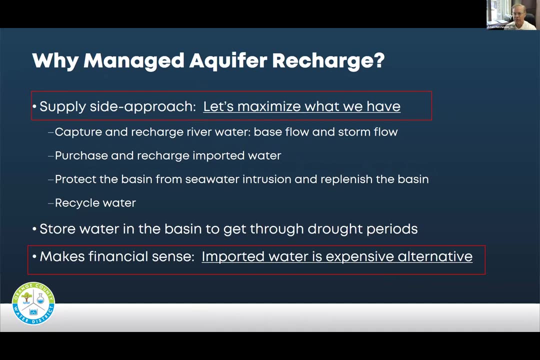 And so that's the operating range. We stay within it And it works really well for us. So next slide, please. So why do we do managed aquifer recharge? Well, going back to the 1930s, when we were formed, the district really had a supply-side approach. 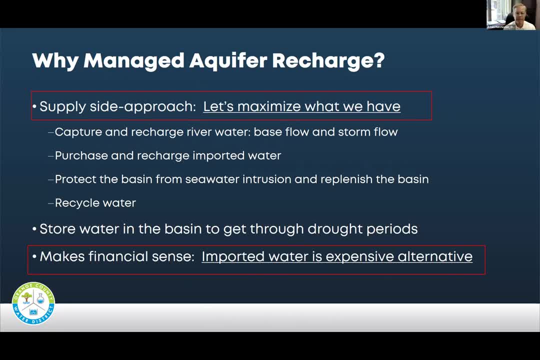 Really, let's see what we can do to maximize what we have available to us. So in the early stages it was really about the capsules We had to recharge our river water- the base flow as well as storm flow- that were coming down to us. 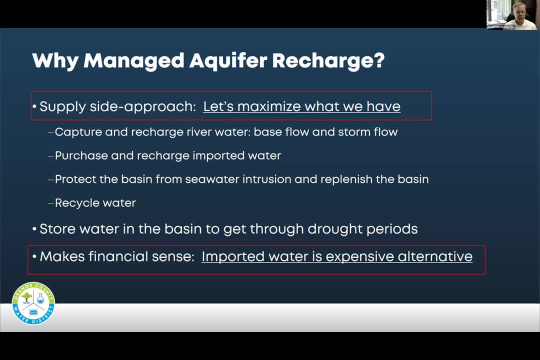 And then later, as the imported water became available, we started recharging imported water and buying it. And then in the 70s, with seawater intrusion, we built the barrier to protect the basin from seawater intrusion and replenish the basin as well. 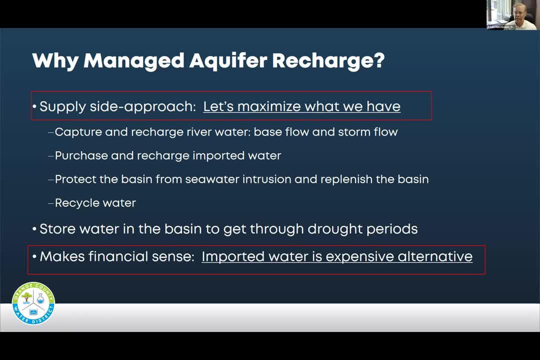 And then more recently recycling water, has been a really key element of our water supply chain. Yet the reason to do managed aquifer recharge is to store water in the basin, to get through drought periods and take that water during the wet periods and bank it and get prepared for droughts. 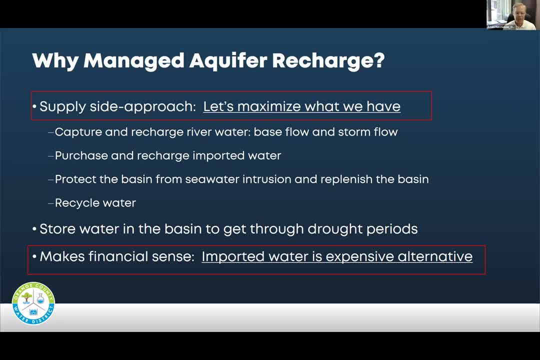 And that's currently what we're in. right now We're in a dry period, And so basin storage is going to go down. But that's what that storage is for And, as I said earlier, it makes financial sense. Imported water is a very expensive alternative. 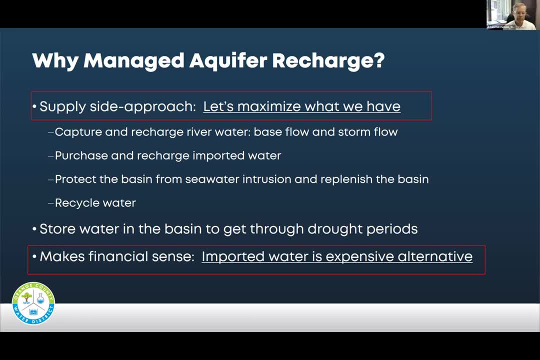 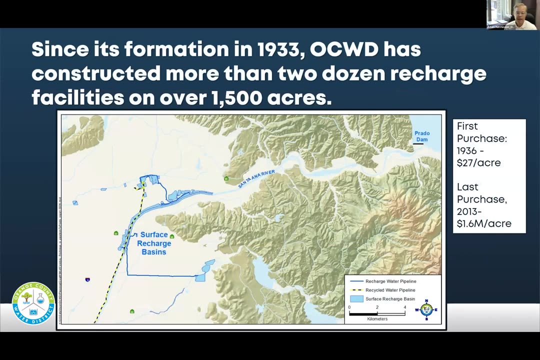 So we have a very strong economic signal to our water supply chain And that's why we're trying to maximize our recharge program as much as possible- Next slide. So, as I mentioned, since we've been formed, we've been developing our managed aquifer recharge program. 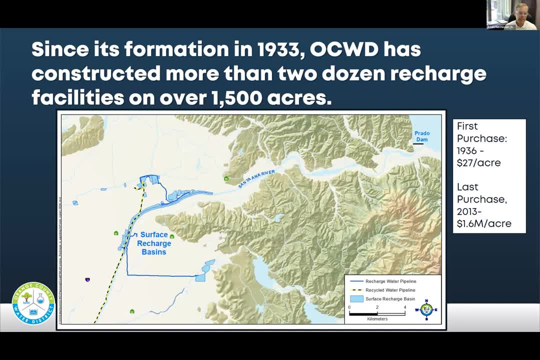 This map here shows the surface water basins that we have. We have 1500 acres of land purchased, starting in 1936 all the way to the present, Our little factoid. on the right, there is our first purchase of land. Our first purchase of land in 1936 was $27 an acre. 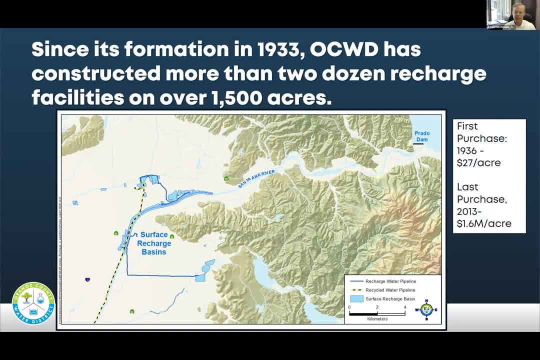 Our last purchase in 2013 was $1.6 million an acre, So tremendous increase in land values in the area. If we were to try and build this system today, we could not afford to do it, So unfortunately, we started a long time ago and really lucky to have all that property under our belt. 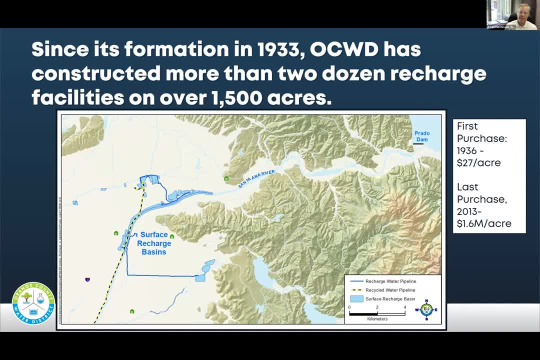 One thing I want to highlight to you in this map is if you look on the upper right you see Prado Dam. That is the Army Corps of Engineers facility built in 1941. And we actually have a program with them to temporarily store stormwater behind that dam and let that stormwater out slowly, so we can recapture that water and not leave it to the ocean. 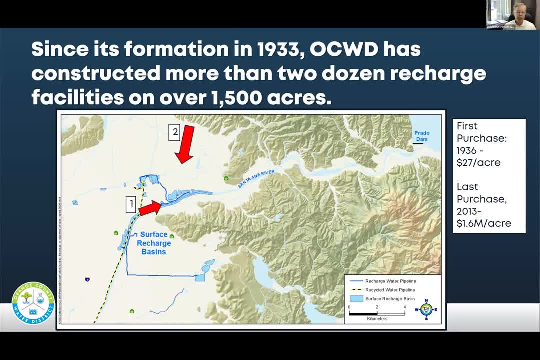 So next slide. So what I'm going to show you here are a couple of a picture and a figure. So number one, you see that, the arrow, That's going to be a photograph looking to the northeast At the Santa Ana River from the aerial view. 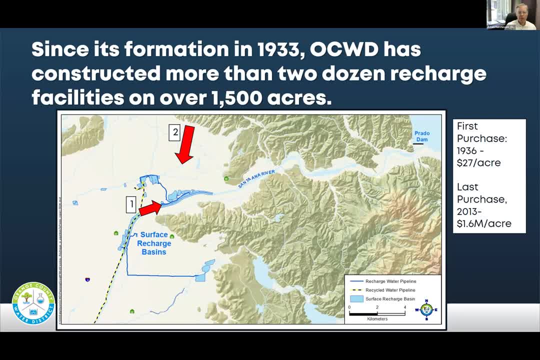 And then number 2 is the figure I'm going to show you: the annual new chart done in 2021.. Schematically, a 3 dimensional cartoon showing the amount of water that all these different facilities you see on the map were able to recharge in one calendar year. 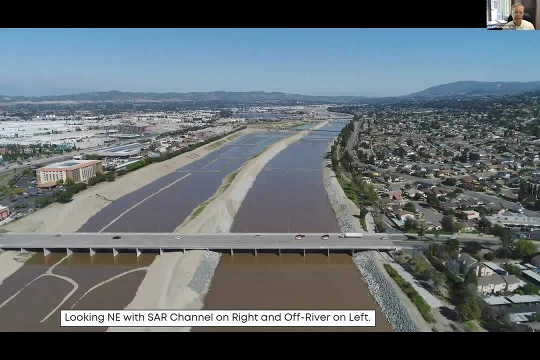 Next slide. So here is a area photograph of the Santa Ana River Channel on the right. On the left is called the offer of the system. So you're looking to the north, towards the canyon, towards Prado Dam. So this is a very urbanized area and the river is really one of our best recharge facilities because it is very long and wide and it doesn't clog like the recharge basins do. 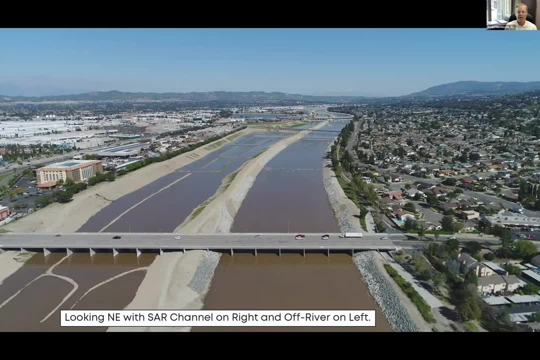 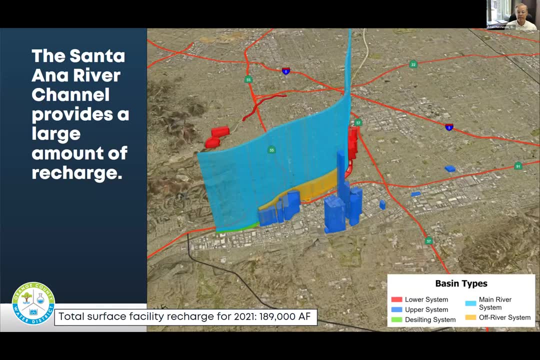 So it's really the backbone of our recharge system. Next slide here I'll show you the actual recharge That was conducted in 2,021.. So you can see the river showed up with a long skinny line there, But it did the most recharge of any facility in that particular year. 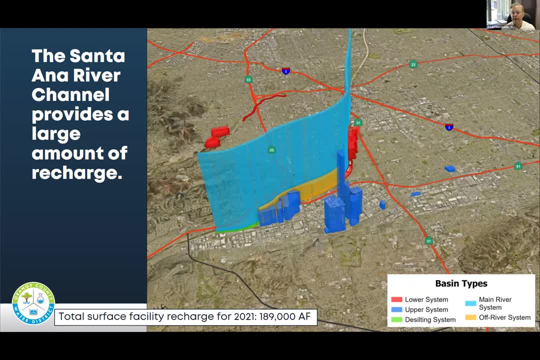 And then the recharge basin show up at the different columns popping up there And in the foreground the tallest one you see popping up there is our La Palma recharge basin, which only recharges recycled water. So it's a relatively small footprint, but the water is so clean and so pure that our recharge rates are far and exceed any other facility we have in our system. 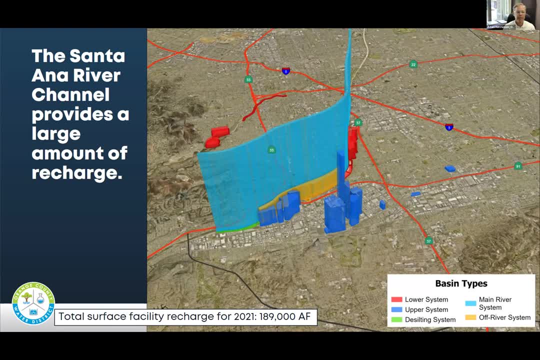 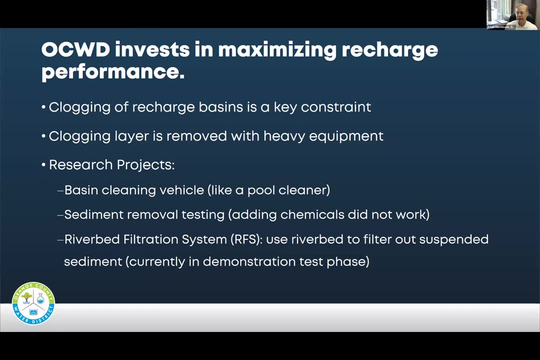 So we're really glad to have that source of water for us. So next slide. So we do a lot of research and development to maximize the amount of recharge we can get. Clogging of our recharge basin is a key constraint. That's true of any management facility. 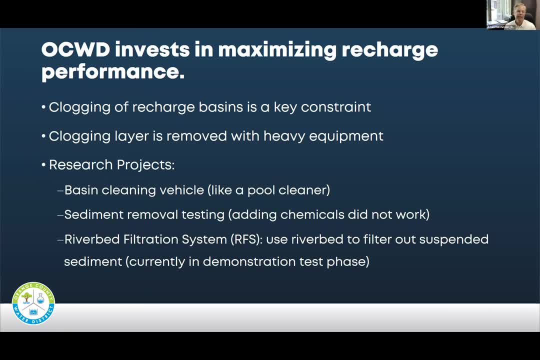 That's true of any management resource system. They're all clogged. It's just a matter of how quickly. For our recharge basin the clogging layer has removed the heavy equipment. The technology there hasn't changed too much, But we are doing research to try and optimize that process. 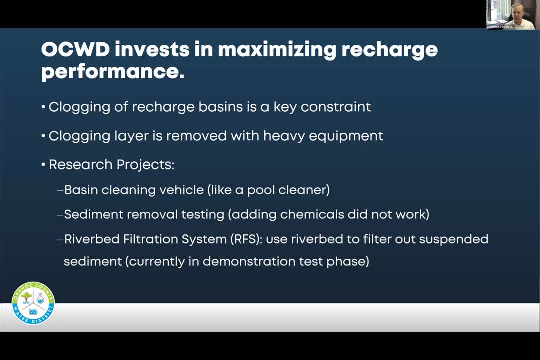 We did a lot of research in what we call basin cleaning vehicles. It's almost like a glorified pool cleaner that would go on the bottom of the basin and sweep up that clogging layer, which is just a really fine silty clay-type sediment. 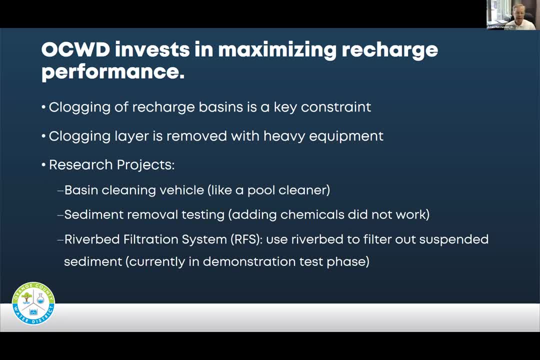 It's a really fine silty clay-type sediment. It builds up in the bottom. That process did work. However, the ability to do it on a scale that makes economic sense for us did not work. We did a massive sediment removal testing project. 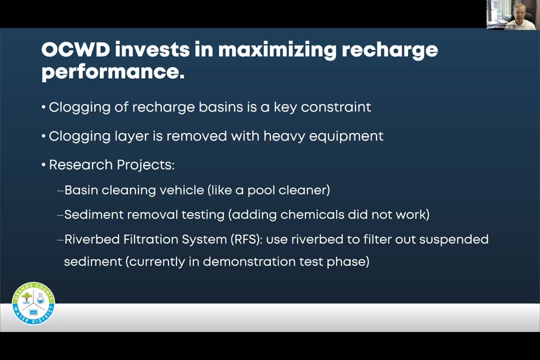 We would look at all the different treatment technologies to remove suspended sediment from the river water. We found that adding any chemicals did not work. That would actually cause clogging on the back end, even if the turbidity levels were low. One of the systems that came out of this testing process was what we call riverbed filtration, where we used the riverbed to filter out the suspended sediment. 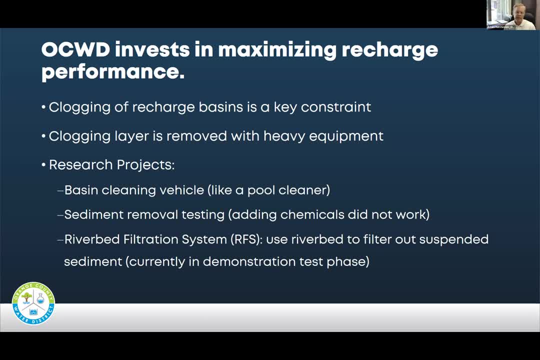 Like what Bill talked about earlier with riverbank filtration. this is riverbed filtration, where we're actually building a collection gallery of pipes about three feet under the riverbed, collecting that filtered water and conveying it to a recharge basin and let the sediment remain in the river where it gets washed downstream. 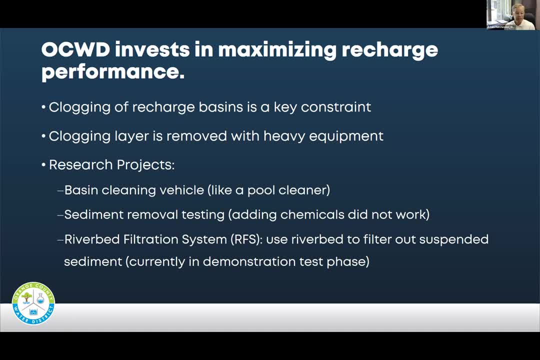 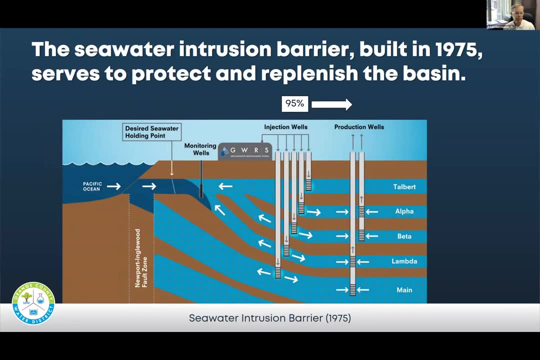 That's something we're doing, So that's something we're seeing very good success with, and we may expand that to a full scale here in the future. Next slide, please. So, as I mentioned, we built a seawater intrusion barrier in the 1970s to protect the basin from seawater. 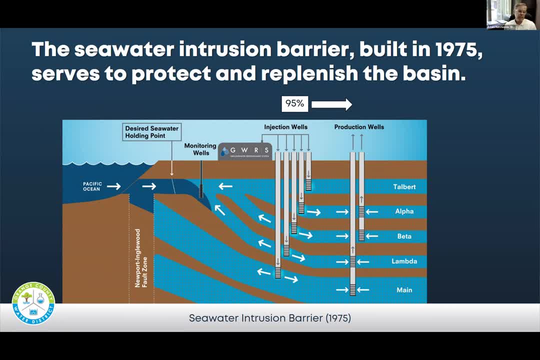 We built over 30 injection wells, And what's really good about this is that not only protects the basin from seawater intrusion, but 95% of that water flows through the seawater. So that's something we're seeing very good success with, and we may expand that to a full scale here in the future. Next slide, please. So, as I mentioned, we built a seawater intrusion barrier in the 1970s to protect the basin from seawater intrusion, And what's really good about this is that not only protects the basin from seawater intrusion, but 95% of that water flows into the basin itself and becomes part of the water supply. 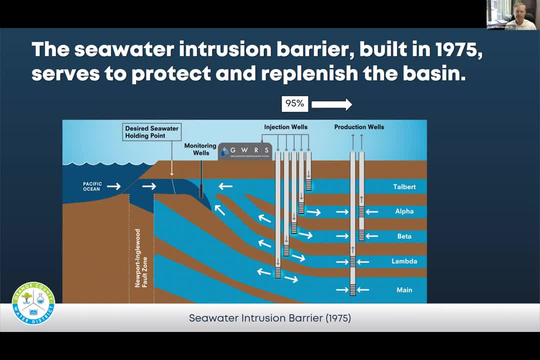 So it's a really multi-benefit type of project. Next slide, please. So over the years we've developed a really diverse water portfolio. These are different sources of water that we recharge into the basin, and the percentage is on average. 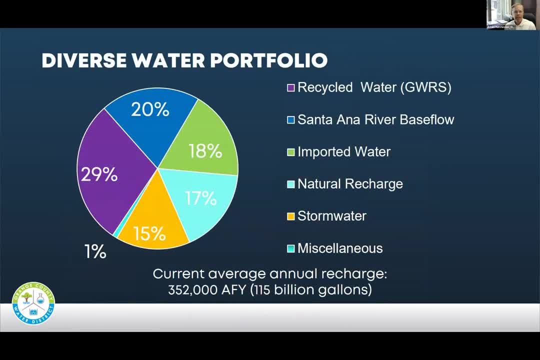 And some of these are more affected by weather such as stormwater, for example. That's going to be highly variable depending on local weather conditions, And we also have a lot of water storage in the basin, So we've got a lot of water storage in the basin. 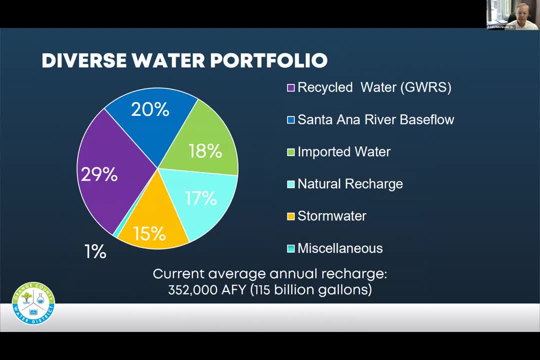 And we've got a lot of water storage in the basin. Imported water is less affected by local weather but can be affected by regional weather conditions such as we have today. So extreme drought condition, the mortgage water supply- they're much lower. 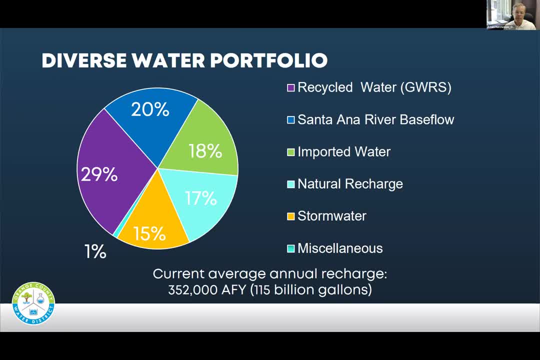 The Ch Disney River base flow and recycled water are very reliable sources of water. They're very resilient. They're not as affected by climate change and other impacts, So we're really fortunate to have a diverse portfolio that can get us through drought periods. 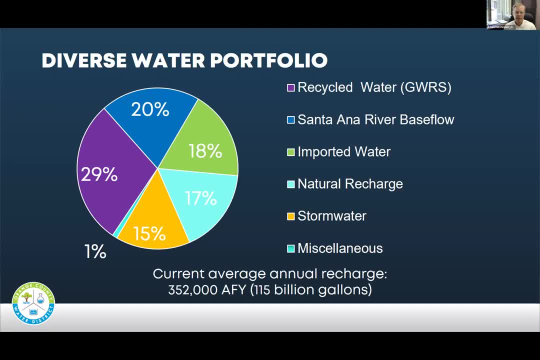 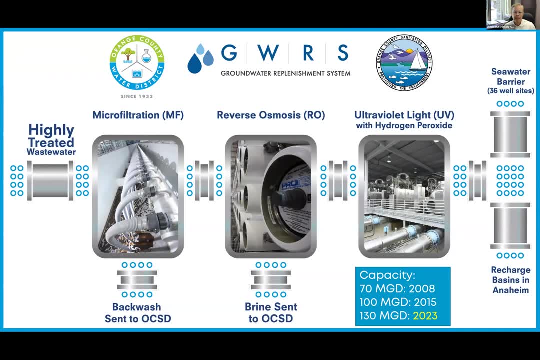 and sustain our groundwater patients. So the next slide, please. So I'm sure many of you have heard about our groundwater replenishing system project that went online in 2008.. This is a typical California approach for microcultivation: reverse osmosis. 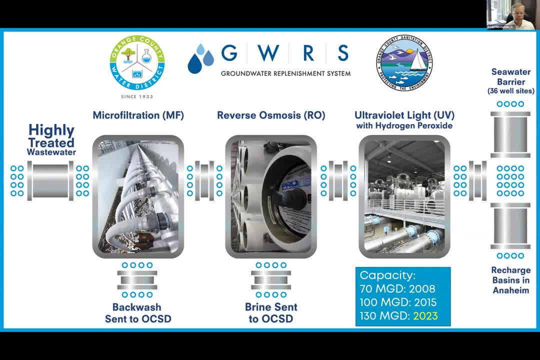 advanced oxidation process, 70 MGD plant was put online in 2008.. We are currently underway in building the final expansion, where we'll go up to 130 MGD next year. That will basically be the final, because there's no more recyclable water. 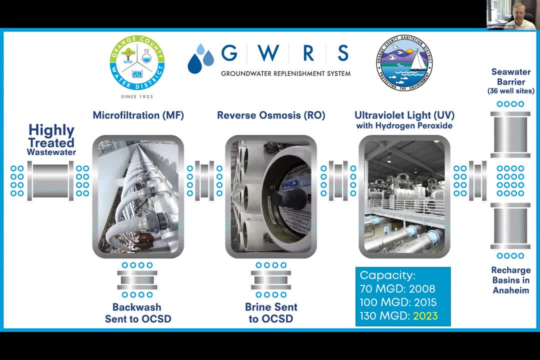 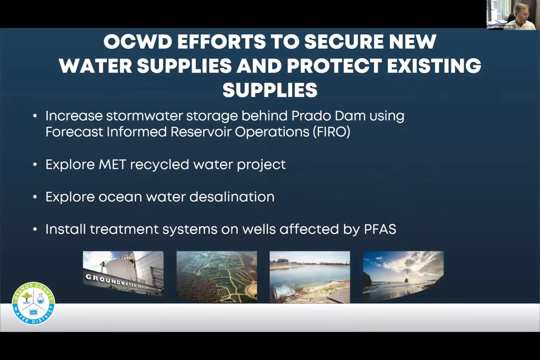 to be had in our area. So we'll basically be recycling everything possible, and all that water will either go into the barrier or up to our Anaheim spreading ground. Next slide, Adam, you have about a minute. Thank you, Yeah, I'm almost done. 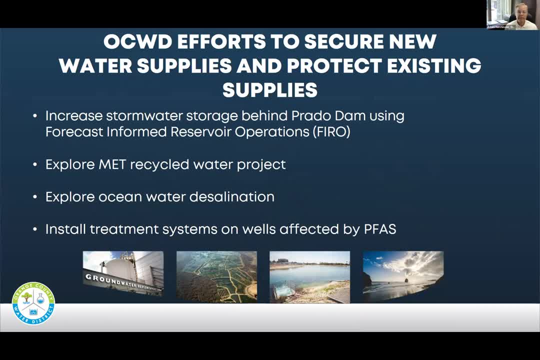 So effort to create new supplies, we're looking at increasing the amount of stormwater we're gonna capture behind Prado Dam using forecast-informed reservoir operation, Reoperating the dam using forecast information rather than the old approach of water on the ground. 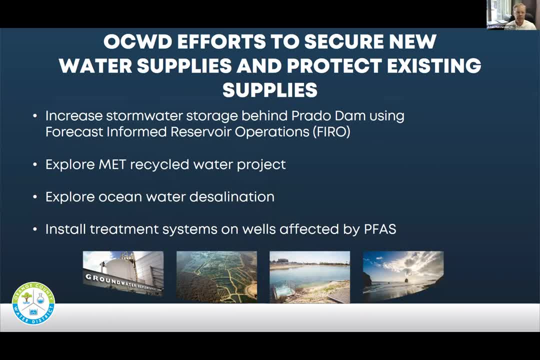 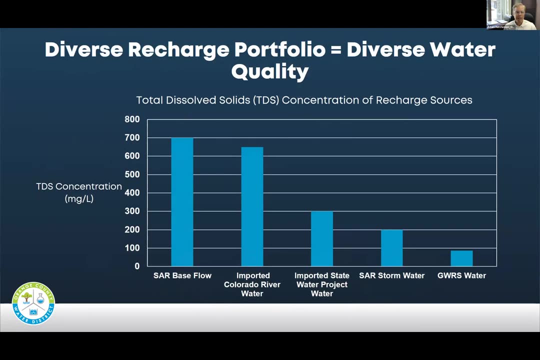 Metropolitan looking at their own recycled water projects and you might participate in that. And then finally PFAS treatment at the final bullet point. So that's the final bullet there. I wanted to quickly cover that Next slide, Just a little out of order here. 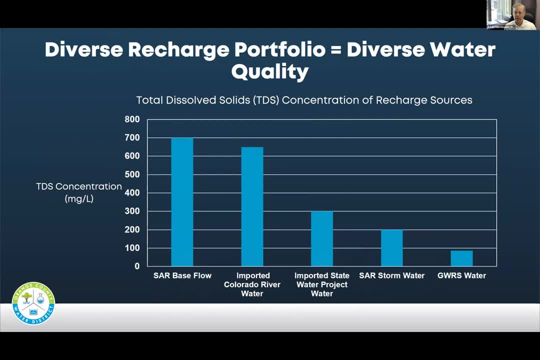 So we talked about the diverse portfolio, also diverse water quality sources. So base flow of the river 700 TBS all the way down to GWS water which is under 100 milligram per liter TBS. But what's really interesting about our groundwater basin? 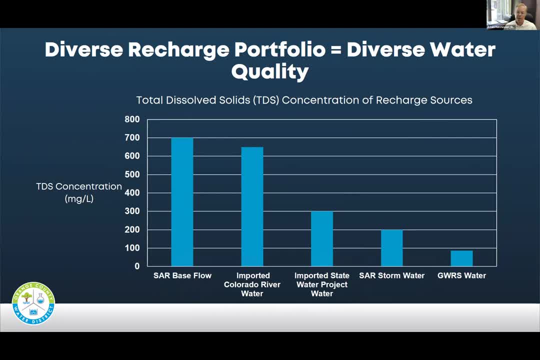 is because we have so much recycled water that's of pure quality. we are actually we're. you know, we have a lot of water that's not recycled. We have a lot of water that's not recycled. We have a lot of water that's not recycled. 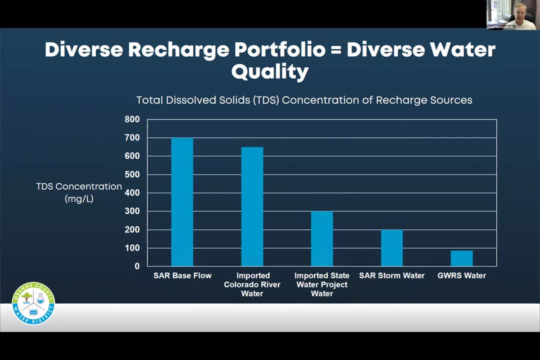 So we're not reversing the salinity balance in our basin. We're going to actually be freshening the basin over time rather than more salinity level going up. So we'll be putting a paper together and publishing that result in probably a year or so. 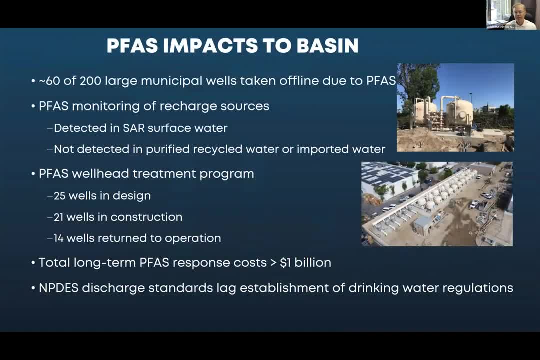 Next slide. So I'm going to wrap up with the PFAS. We've had a lot of PFAS impact to our basin. 60 of our 200 wells were taken offline. This is in the treated wastewater that we're receiving from upstream. 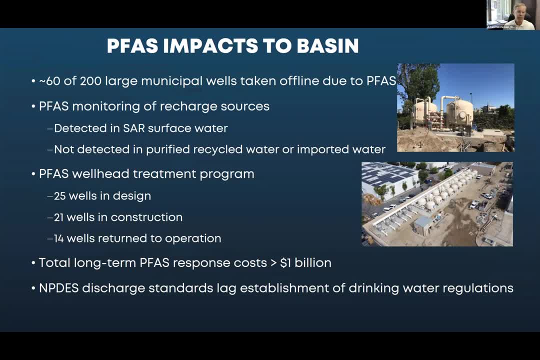 PFAS levels are in that water, And so it's caused us to have to do a massive wellhead treatment program. It's been cost over a billion dollars long-term, And so we are paying for this. We're going to go in and pay for these treatment systems. 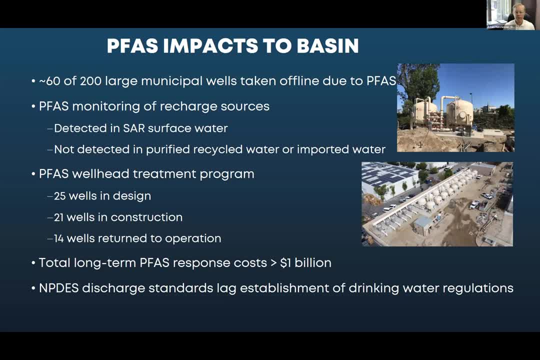 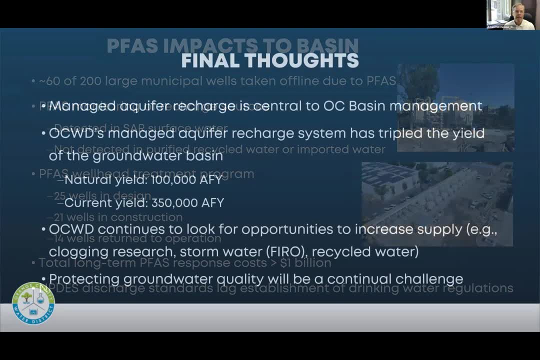 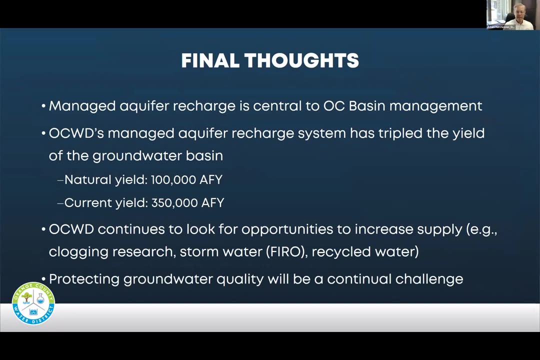 and then the utility to be on the hook for some of the O&M long-term. So final slide. next I want to wrap up with. you know, Man of Doctor, Recharge is central to our ability to manage our groundwater basin. This program has more than doubled or tripled the yield. 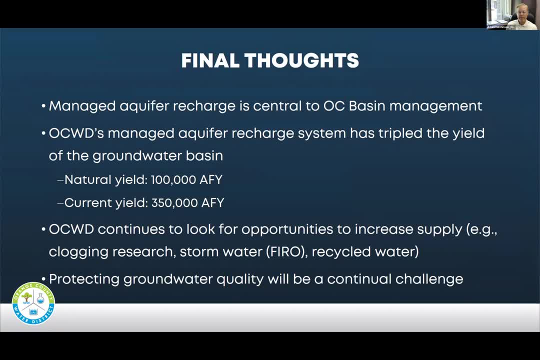 of the groundwater basin. The natural yield is 100,000 feet per year. OCWD weren't doing anything, but the current yield is over 350,000 feet per year. We'll continue to look for opportunities to increase supply with zero recycled water. 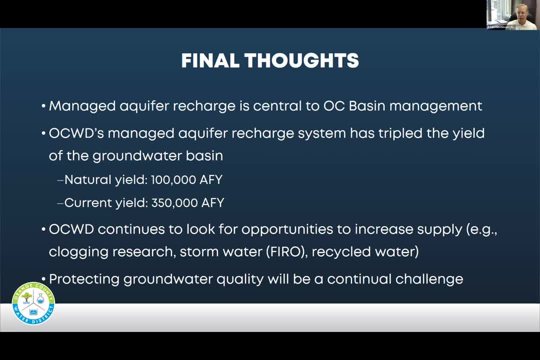 and just protecting groundwater quality is going to be a continual challenge from our project, because PFAS wasn't on our radar. It was on our radar several years ago and now it's a huge issue that we're having to address, And so as our technology detection approaches get better, 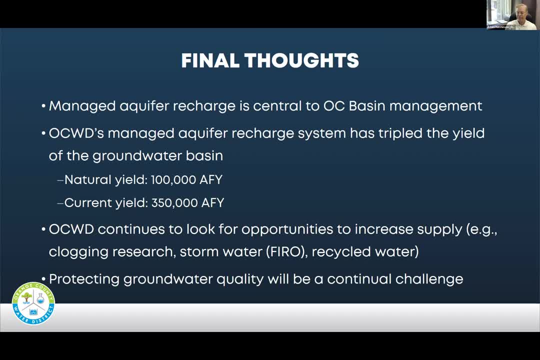 we're going to continue to find more challenges in the future, So that's what keeps us busy. That concludes my presentation. I look forward to questions later on, Thank you. Thank you, Adam, very much, And we'll move on to Dr June Murray. 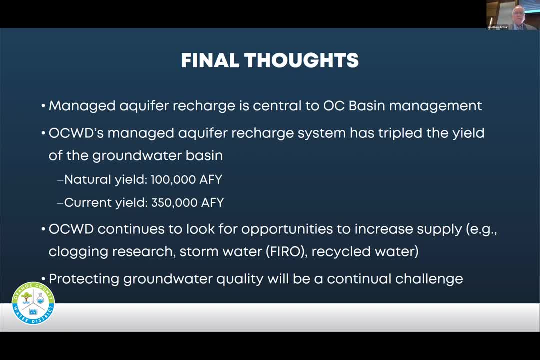 Dr June Murray of the VAAS Astrology Center on the National Geological Survey. And June comes to us with a story from Florida. She's senior hydrogeologist with the US Army Corps of Engineers and a licensed professional geologist in Florida. 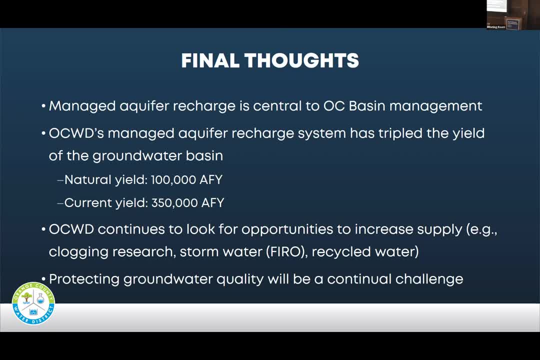 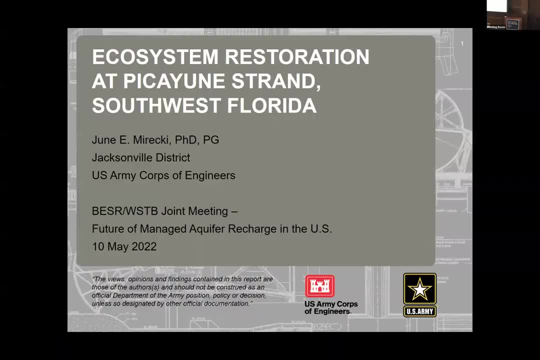 She's an hydrogeochemist and then some, and serves as technical lead for the ASR projects, or has served as technical lead for you can correct me: June, the ASR pilot projects, Glades, Restoration Projects to Increase Water Storage in Southern Florida, and June, all yours. 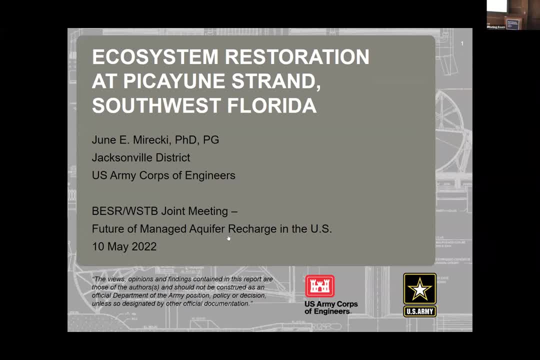 Thank you very much, John. I apologize. I cannot get the camera to work on my federal laptop, so the wheel just keeps going round and round, So unfortunately you can't see me Today. I'd like to present a decided or a comparatively low-tech approach to 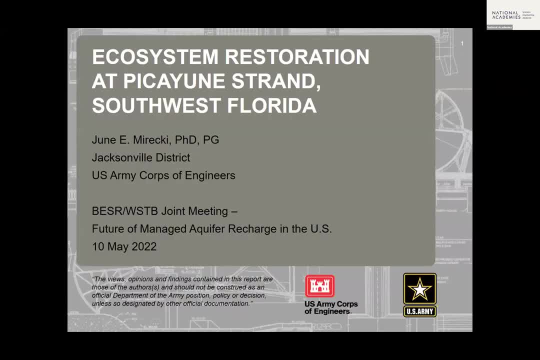 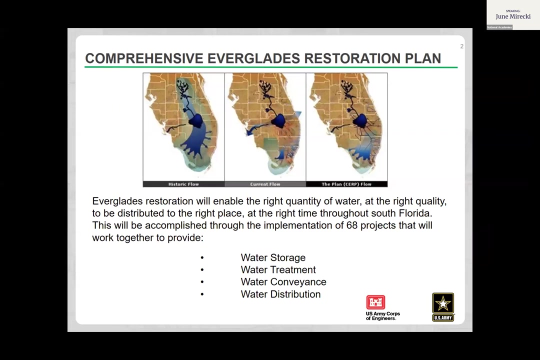 managed aquifer recharge specifically for ecosystem restoration, And this project at the Picayune Strand Ecological Restoration Project is part of the comprehensive Everglades Restoration Plan. Next slide, please Just one slide, about the Comprehensive Everglades Restoration Plan, or SERP. 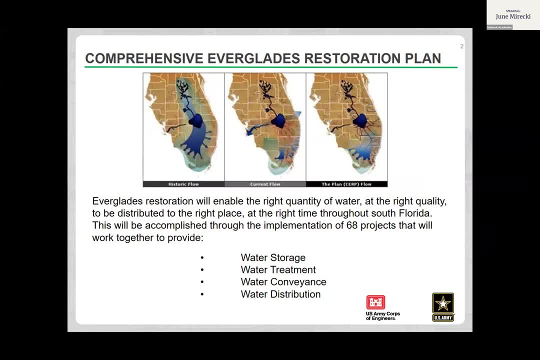 This suite of projects, 68 projects in total, is designed or was compiled and integrated to replumb Southern Florida, both from a surface water sheet flow and surface water-groundwater interaction standpoint. The entire attempt to re-plumb Southern Florida is to allow a more natural, but controlled- for flood control purposes- movement and conveyance. 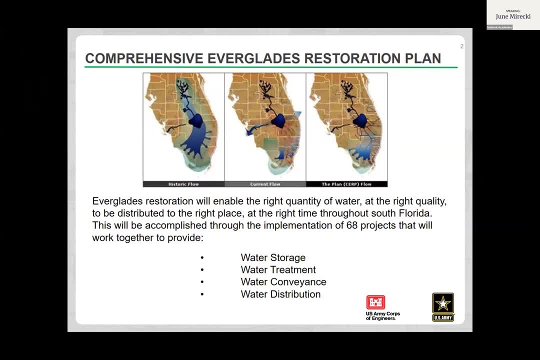 of surface and groundwater from the headwaters of the Kissimmee River Basin up north near Orlando, southward through the Kissimmee River Basin and Lake Okeechobee and then into the areas south of Lake Okeechobee. 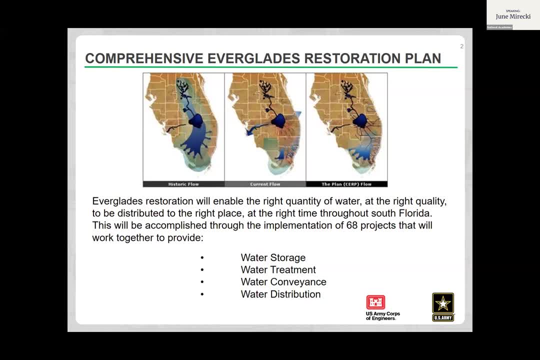 including the Everglades National Park. The SERP is the acronym, and it is a compilation of 68 projects, of which the project I will discuss today is one of the first to come online. When all of these projects are implemented, it will improve the volumes of water in storage. 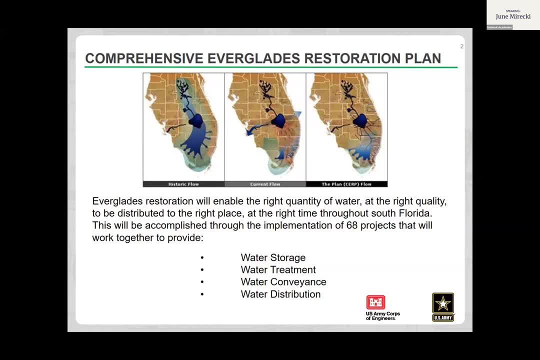 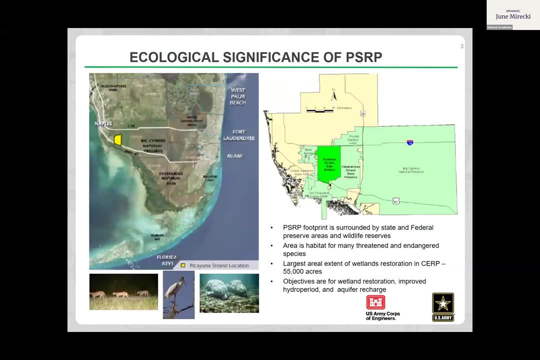 Some of the projects will provide nutrient reduction by water treatment. It will provide a more natural rate of water conveyance from north to south and will enable and continue water supply for ecosystem restoration purposes. Next slide, please Now. the Picayune Strand Restoration Project was one of the first ecosystem restoration projects. 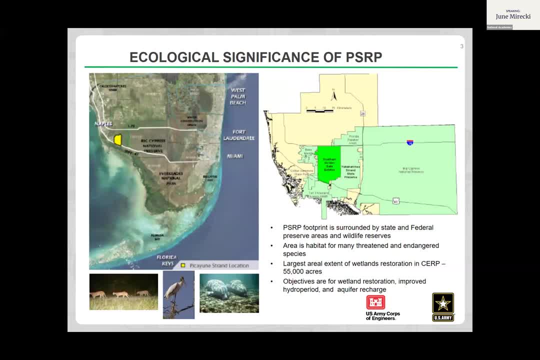 to come online in SERP in the mid-2000s. The importance of the Picayune Strand Restoration Project. it's located in western Collier County and toward the city of Naples. It is a keystone to ecosystem restoration in this area. 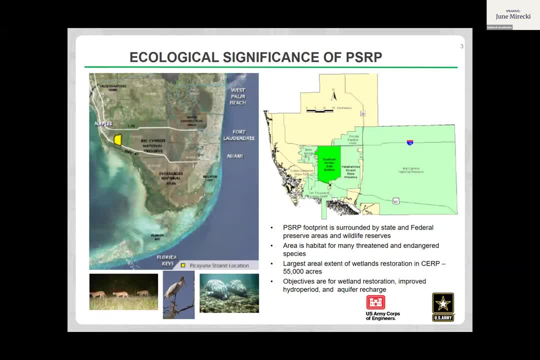 As we'll see in a moment, it was proposed suburban development. The figure on the upper right shows that dark green world green areas, the northern golden glades states. But notice that that proposed suburban development is surrounded by natural wilderness areas: state preserves, national preserves, National Wildlife Refuges. 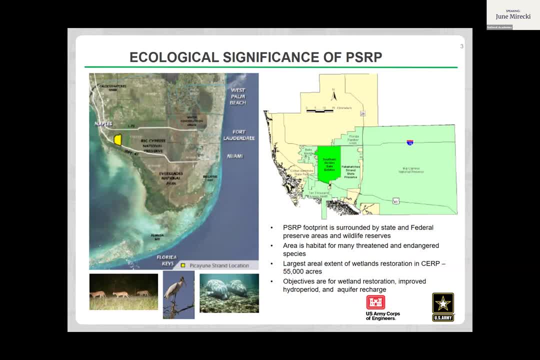 Them. this footprint is actually a keystone to ecosystem restoration for this entire area. In addition, it's the location of of the big important endangered species in South Florida, and that includes the Florida panther, the endangered wood storks, and there's even a feature for manatee restoration. 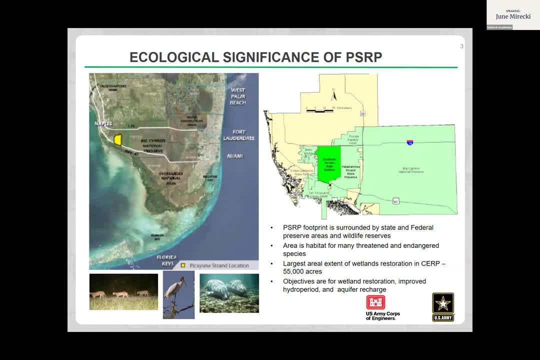 or a manatee restoration also in this area. The other important feature about the picayune strain restoration project is that it is the largest wetlands restoration project in all of SERP. It's 55,000 acres of rehabilitated wetlands. The objectives for this project. 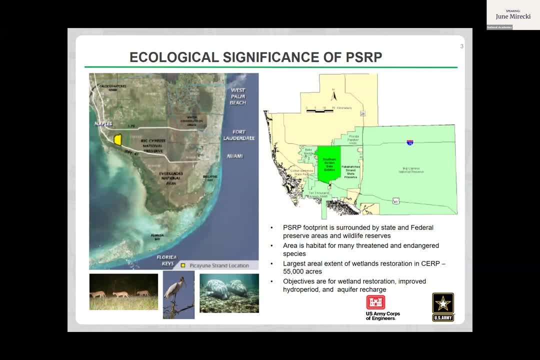 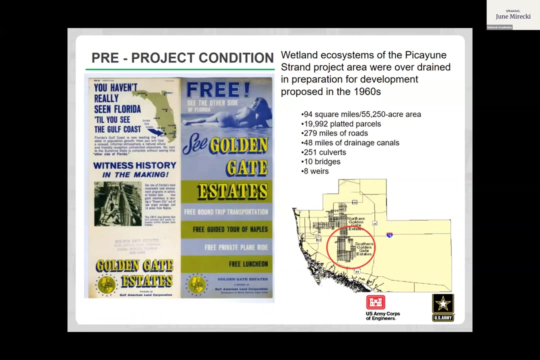 include, of course, wetland restoration and habitat improvement, improved hydro period of these wetlands to more mimic the natural wet dry season cycles. and, finally, what we're all interested in is aquifer recharge. Next slide, please. Now the pre-project condition of the Southern Golden Gate Estates. 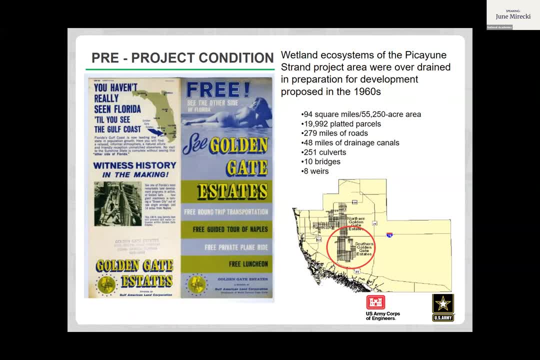 This was a proposed suburban development and one of the largest at the time suburban developments of all of the United States, and the developers proudly declared that this would be the giant machinery is creating a dream city of new out of virgin territory, and they were quite proud of that. Well, the proposed development was again. 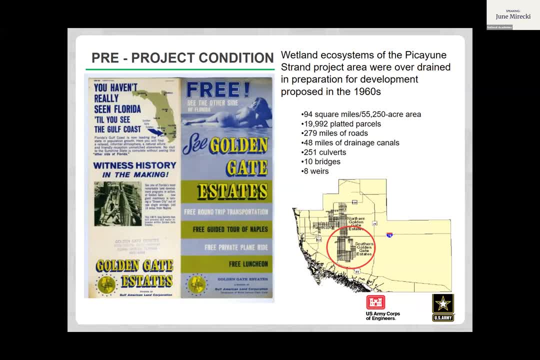 the 55,000-acre area, almost 20,000 plotted parcels, roadways, drainage canals, culverts and bridges, and weirs for water flow conventions, low conveyance, and what this resulted in was over draining of this sensitive wetland area. 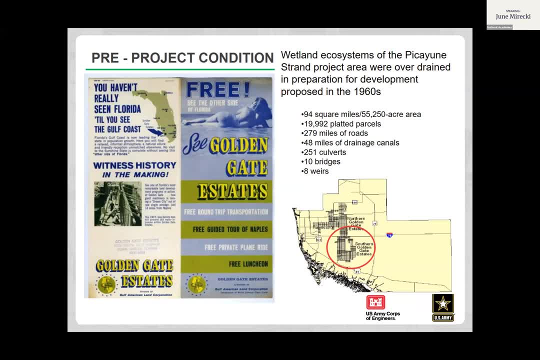 and it's probably the basis of that, that, that statement: if you want to buy some, uh, i have some swampland in florida to sell you. because one of the failures of this developed, proposed development was the fact that, during wet season flows, all of this area was under feet of water and the 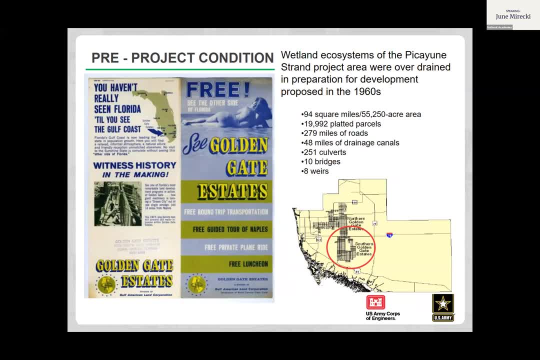 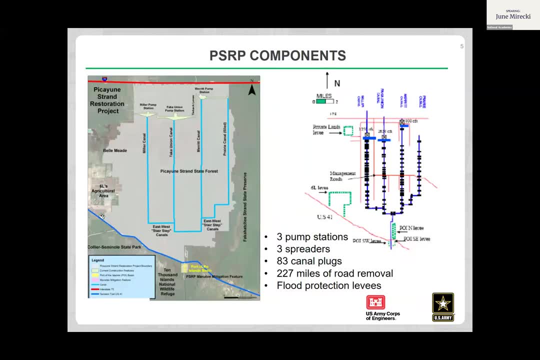 development was just, even with all the drainage activities, they could not develop it further. next slide, please. okay, so how, what? how will we restore this area, prevent the over drainage of the wetlands, uh, promote wetland restoration and managed aquifer recharge the components of the picayune? 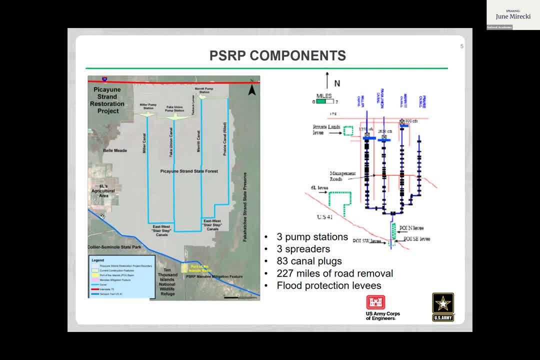 strand restoration project in, and again, these are low tech compared to the talks that you've just seen. uh include the construction of three varying size pump stations, and you can see those along the top: the merit pump station, the faka union pump station and the miller pump station. now, these are not just pump stations to 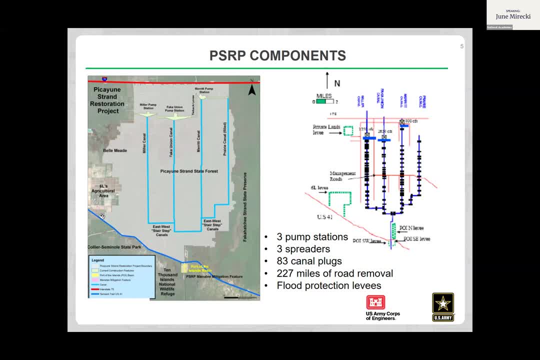 convey water down canals. they are positioned near the existing canals, but these pump stations will are positioned near the existing canals, but these pump stations will be are positioned near the existing canals, but these pump stations will be also where the water is from: from the chamber. 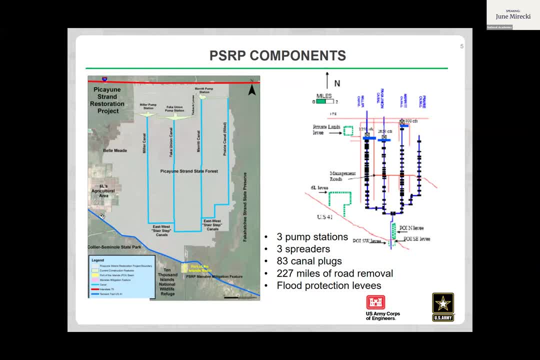 and then there are solar panels are positioned on the canals, or canal plug systems. The project also includes 227 miles of road removal and also some flood protection levees. These are actually small berms around private lands and agricultural lands to the south. There's also a manatee mitigation feature that allows controlled water levels, so that 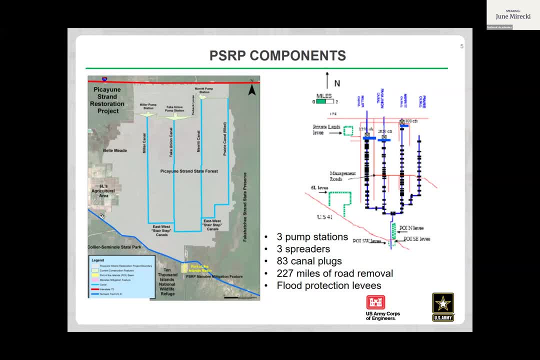 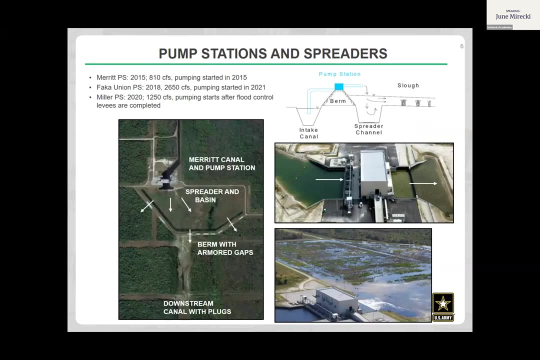 manatees can access the area and the canals in the very southern part of the project area. So we have all these. The important thing here is the integration of pump stations, spreaders and canal plugs. Next slide, please, And here we can see how these features work in conjunction. 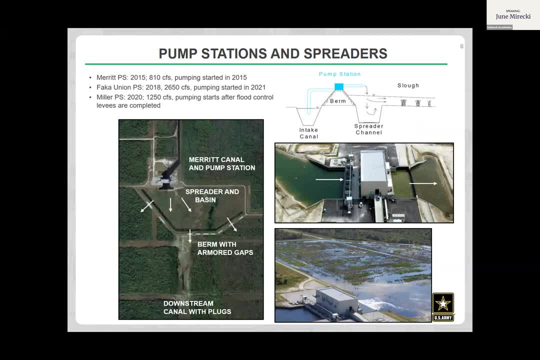 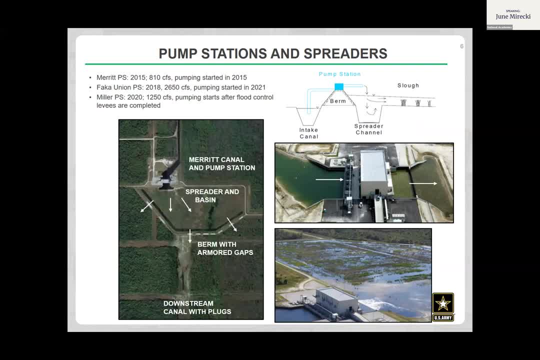 online in 2015 and started pump conveying water in earnest in 2016.. If we look at that figure on the left side you can see from north to south. you can see the existing Merritt canal and on the southern lower part of that photograph- the Google Earth photograph- you can see where the canal plugs. 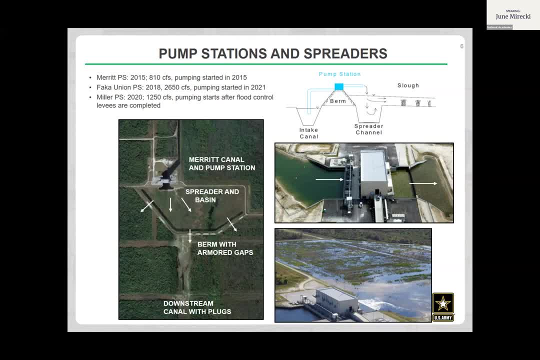 are starting to infill. The pump station is situated within a berm, at the dogleg of that Merritt canal, So water is brought into the pump station through the dogleg canal and the flow is controlled by conveying that pump station down gradient through a stilling well, over a spreading canal, a spreader feature, and then 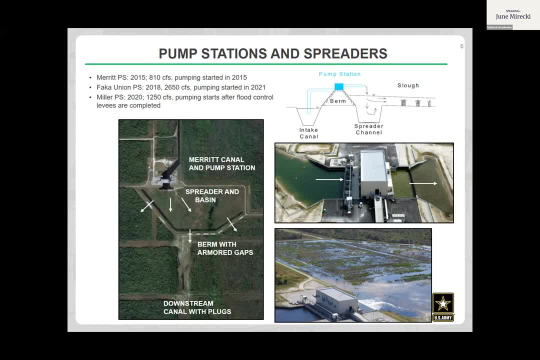 into a recharge basin. So if we go kind of counterclockwise, in these three photographs we have all of the features are shown here: the canal and pump station for intake and the spreader basin for discharge. That spreader basin has a levee around it to contain the basin. 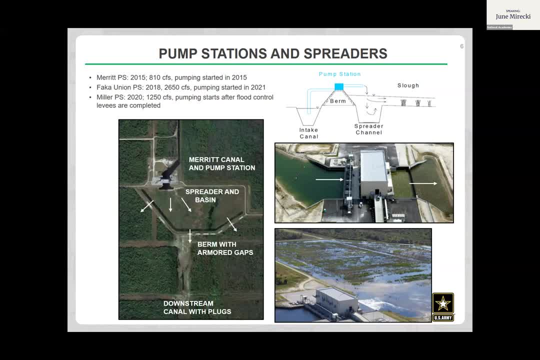 but also armored gaps that allow overflow once the tailwater pool depth is reached. So the second upper right photo shows the directions of water flow conveyance and that bottom photo shows what the recharge basin looks like as it operates About a minute Already. Oh, I'm sorry. Okay, next slide. 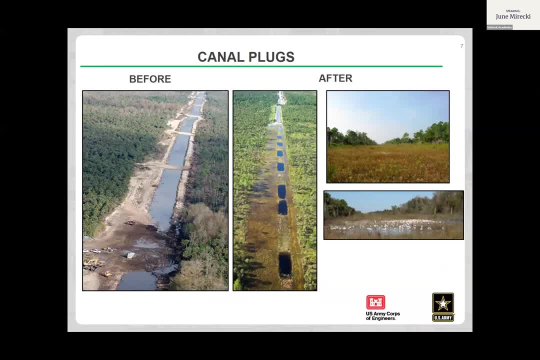 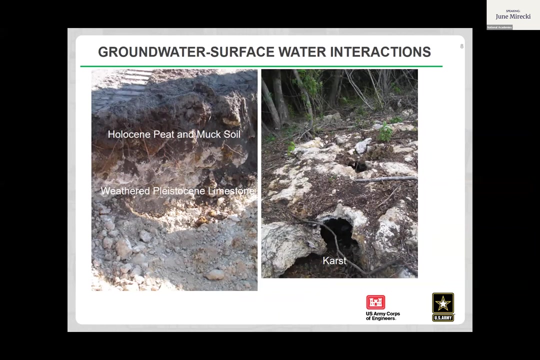 Please, Here are the canal plugs Before and after. we show the canal plugs in construction, then in restoration to the left- or to the right, I'm sorry- And also the wading bird populations that develop. Next slide, please. Now just for groundwater surface water interactions to discuss. 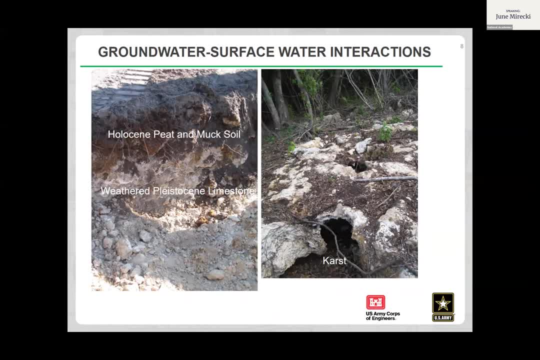 our. Okay, This is the. As the water gets into the Upper Aquifer, we have a Holocene peat underlain by fractured limestone, and underneath that is marine sands and silt, ultimately underlain by karst of the Tamiami. 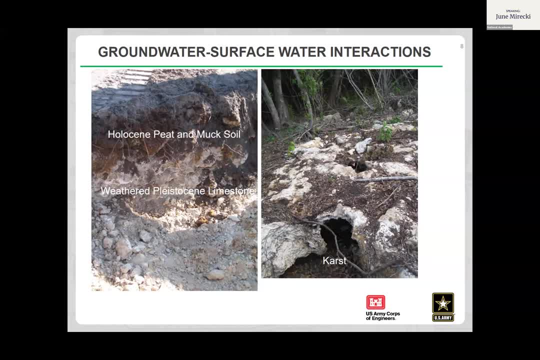 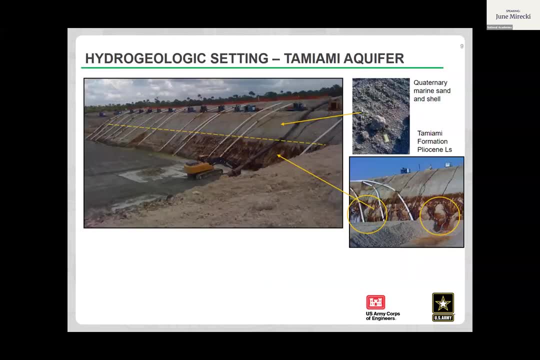 Formation. Next slide, please. Okay, This is the excavation of, not the Marriott Pump Station but the larger Fakir Union pump station in the Upper Aquifer, and this is a separate excavation of the larger Fakir Union pump station but the larger Fakir Union pump station. and this is a separate excavation of not the Marriott Pump Station but the larger Fakir Union. 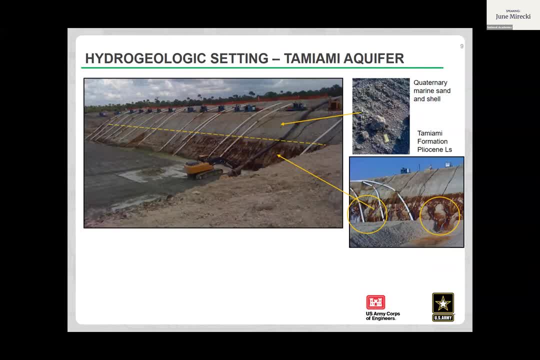 Union Pump Station Foundation and we can see the hydrogeologic setting consists of undifferentiated quaternary marine sands and shells overlaid by a tamiami formation which here is rusty colored, and it's because we're dewatering the pump station foundation and surface water. 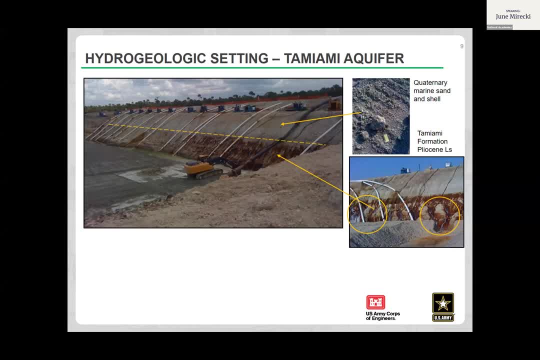 with a lot of iron is coming through. What's important here is that you can see just rivulets coming out of that foundation and which causes issues with dewatering, but it also indicates the transmissivity of this particular aquifer in this area. 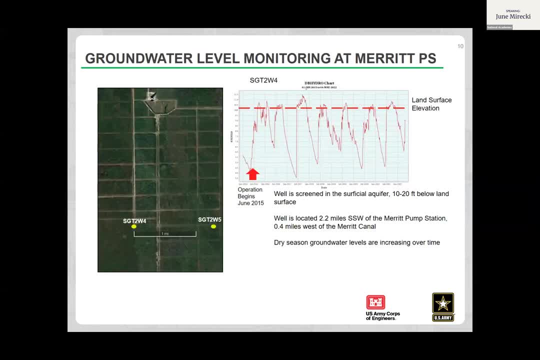 Next slide, please. Now. restoration success takes a while to develop and basically we don't have a water budget with a water budget, But we do have a water budget for recharging versus evapotranspiration in this rainfall driven system. There are two monitoring wells down gradient from the Merritt Pump Station. 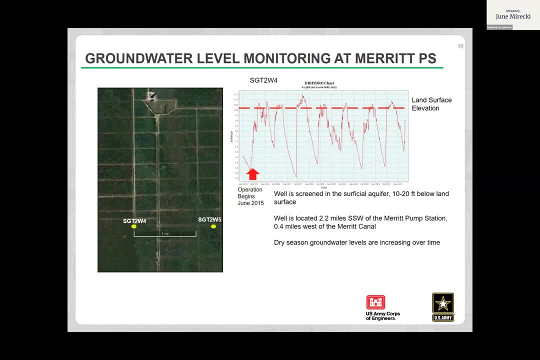 The hydrograph on the left or on the right from one of the closest monitoring wells shows a typical wet season dry season sawtooth curve And one of the indications that we are getting recharge is that the dry season potentiometric surface of the tamiami formation. 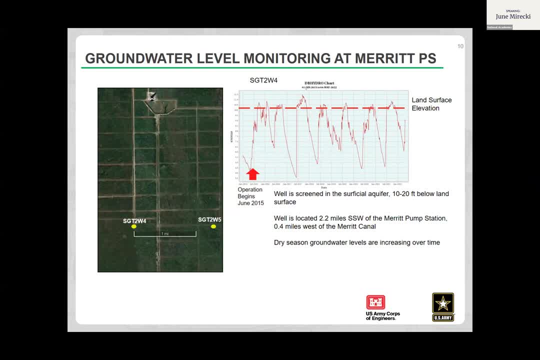 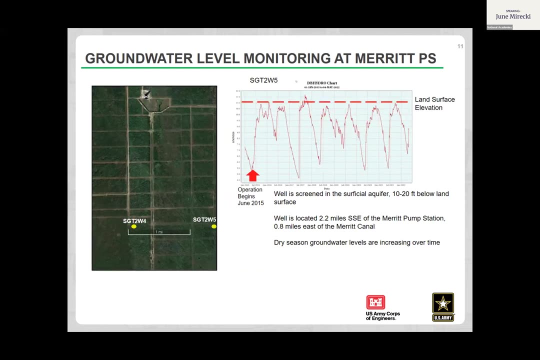 Is increasing over time. you see, those low values are show a higher and higher elevation. So it's a qualitative evaluation, but it seems like we are starting to recharge the aquifer. Next slide, please. And this slide shows the same tendency. this is a little farther away from the pump station. 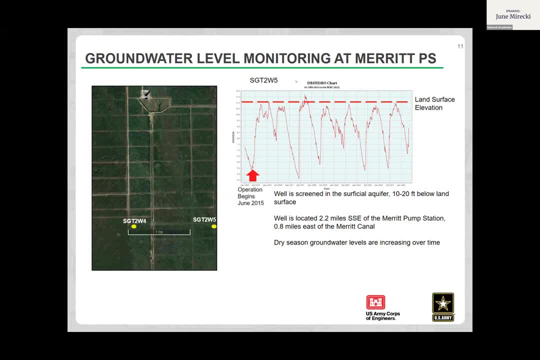 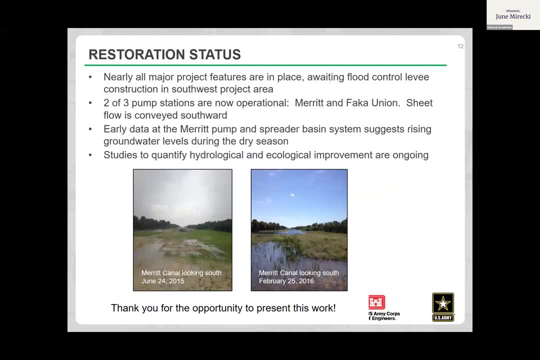 We see increased dry level or dry season water levels over time. Okay, Final slide, The restoration status. nearly all of these features are in place. We just have to finish construction of the flood control levees around the agricultural and private lands on the western side of the Picayune Strand. 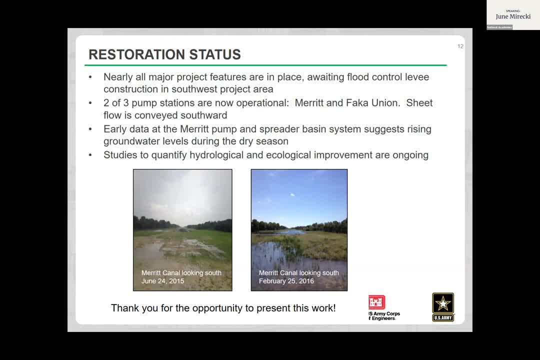 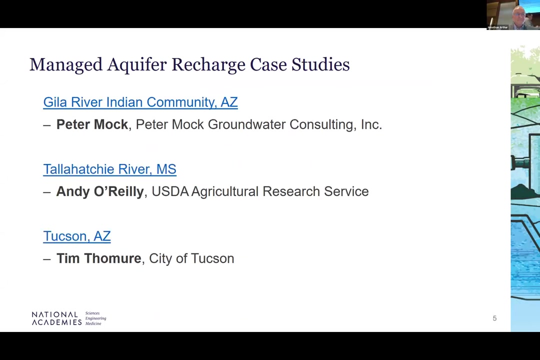 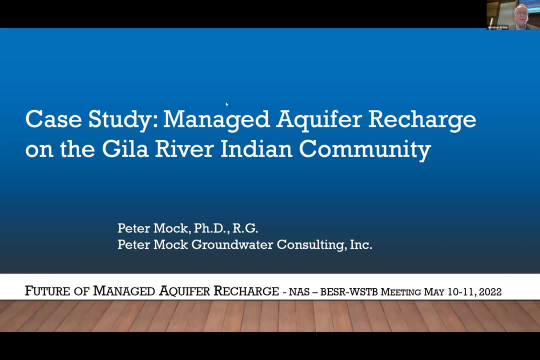 Two of three pump stations are now operational. early data from the Merritt Pump Station spreader system. An example of those is the map of the flood control levee. Here is the map of the flood control levee. The map shows the ground water levels are increasing during the dry season and the studies to evaluate 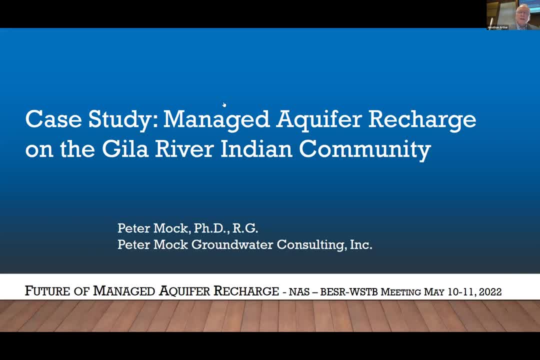 restoration success are in progress, And that's my final slide showing before and after. Thank you. Thank you so much, June Peter Mott, Groundwater Consulting Inc. and a registered geologist who conducts studies in hydrology, geology and environmental science. He worked extensively on several remediation. 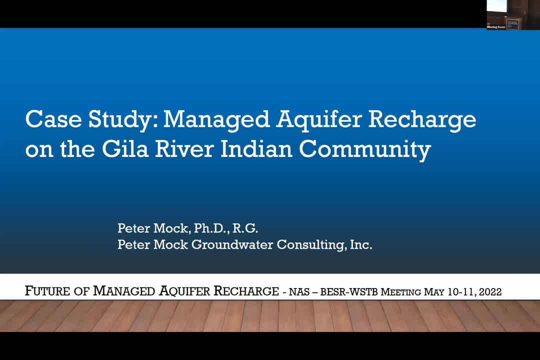 investigations related to Superfund sites across the West, and I'll turn it over to you, Peter. Good morning, Can everyone hear me? Yes, Very good. Okay, So thank you for having me here to give you a presentation on the Gila River Indian. 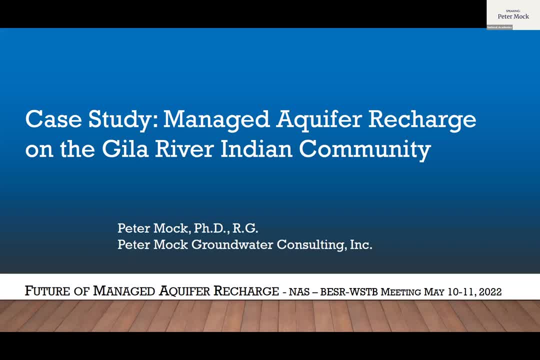 Community's Managed, Aquifer Rechart, I'd like to start by saying I'm not a community member, but I've been a consultant to the community for about 20 years. So if you could give me the next slide, The Gila River Indian Community is in the middle of Arizona. You saw some of those. 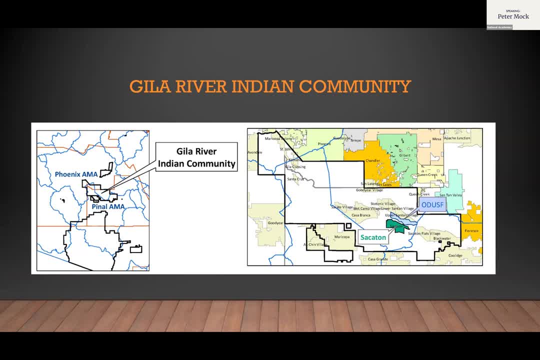 pictures before of the blue outlined active management areas in Arizona are how the Department of Water Resources and the state manages groundwater, at least in the more urbanized areas. So on the lower left you can see there's the Phoenix AMA and the Pinal AMA. 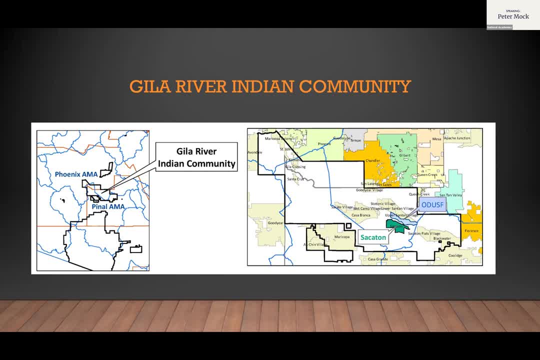 and the Gila River Indian Community sits right on their border, with quite a bit of a jagged line going through it, which makes it interesting in a regulatory process. On the right, we see briefly that the cities of the Phoenix metropolitan area, Phoenix, Chandler, Gilbert, Queen Creek, etc. 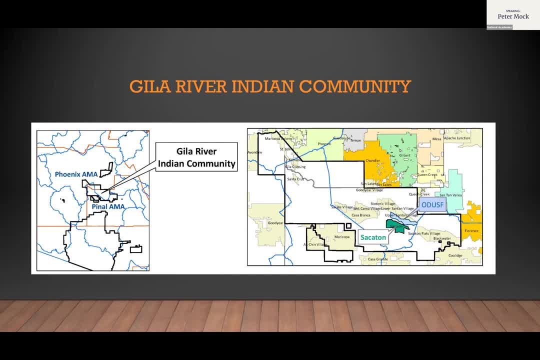 are right up against the Gila River Indian Community's boundaries on the north and then on the south of the growing community. So the Pinal AMA, Maricopa, Casa Grande Coolidge, But more importantly for now, I'd like to see the ODUSF, That's, the Old Bird BAM Underground Storage Facility, which is 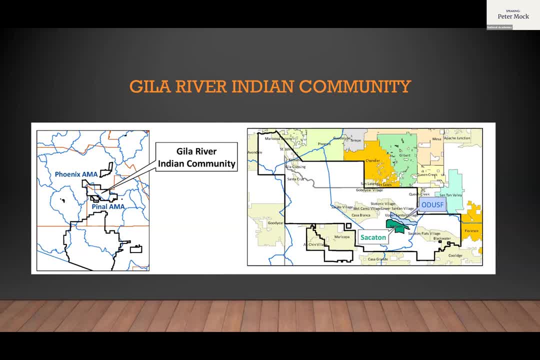 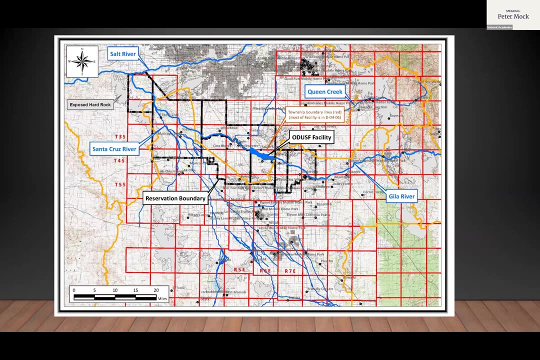 the largest and first of the community's MAR projects. It's in the middle of the community roughly, And the Sacaton is where the governance center is for the Gila River community And you can see it's right there in the middle, Next slide. So I'll give you a little bit bigger picture. 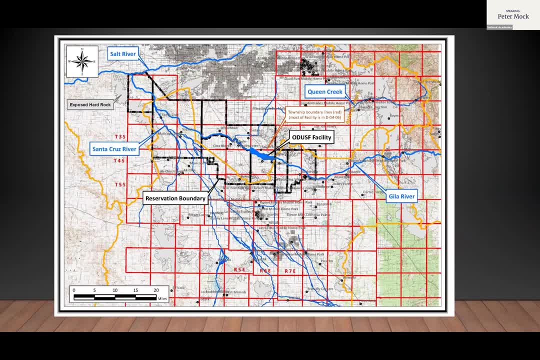 Here's the community. the black outline and the blue line going through the middle is the Gila River And of course the reservation was drawn to incorporate the people who lived along the Gila River here in central Arizona. Gila River starts in the mountains in New Mexico, high-altitude. 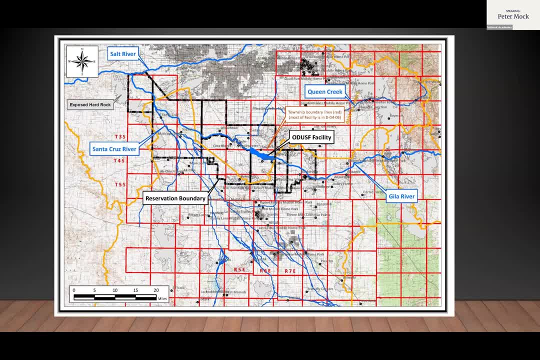 forests and then flows west through. here where you see it. It joins the Salt River near the top of the picture, and then the fragments of the Santa Cruz River as it goes across the flats to the south of the Gila River. And again I'm showing where the Old Bird BAM Underground Storage Facility is. Next slide: 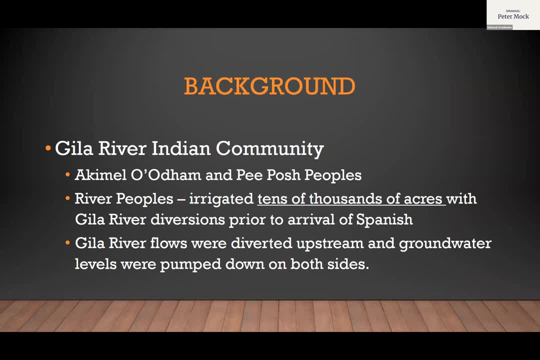 So I'll give you a little bit of background, and I'm not going to do justice to this at all. There's an entire book called Stealing the Gila by David DeYoung, who was going to speak to you but was unavailable. He is the director of the Pima Maricopa Irrigation Project. But briefly, the Gila. 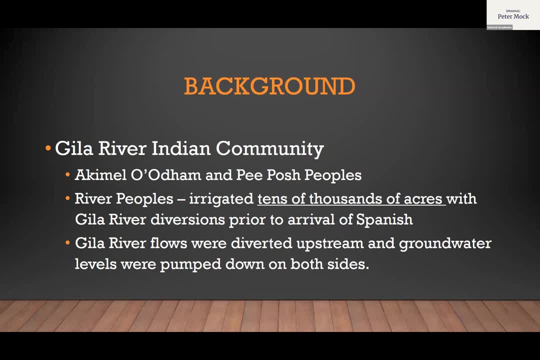 River community is a combination of the Acoma'o O'odham and the Peeposh peoples. Acoma'o O'odham are better known as Pima and the Peeposh Peoples are better known as the Peeposh Peoples, But these are river peoples and they irrigated tens of thousands of acres with Gila River. 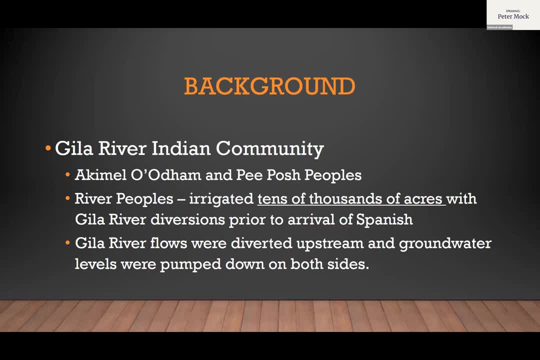 divergence prior to the arrival of the Spanish, So they've been here a very long time and they had a very thriving agricultural economy. Since that time, the Gila River flows were diverted upstream, They completely cut off and groundwater levels were pumped down on both sides of the 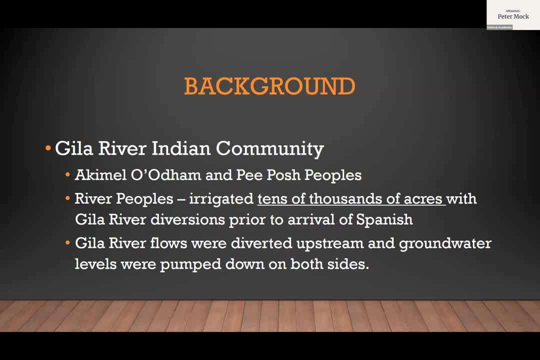 community. So, whereas the river was in tight connection with the groundwater system, before, the water can be seen at the surface And then about 4.4 billion engines are placed into those channels. The scratches that you can see here on the bare surface of the Gila River supplies: 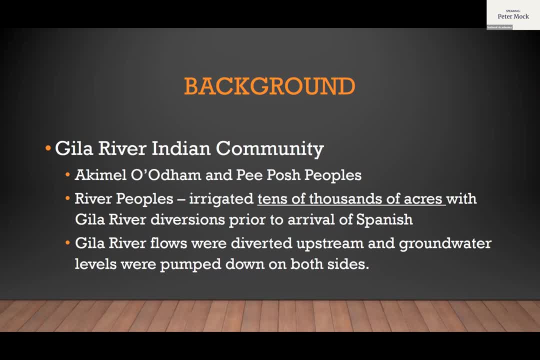 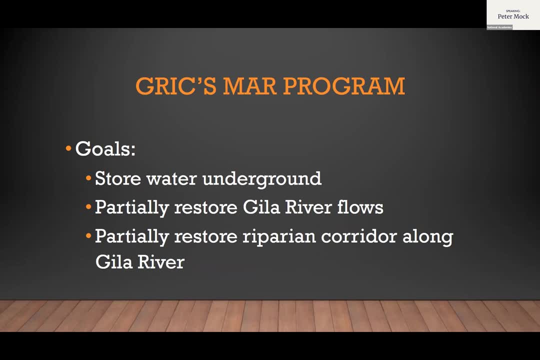 you can see 70 in the 50 years that those columns were here do exist. The 2005 plan for Gila River flows begun in 2019, and some in 2019.. So that comes mainly to provide infrastructure to our next generation of ships and crews. 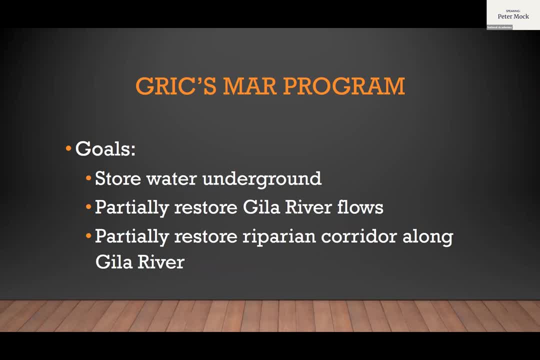 And then two handouts on the Gila River And these are Palaua, Healer River. this is so important to the river people but they understand they cannot completely restore the Healer River flows or completely restore their apparent corridor. They're just looking for some sections of it. 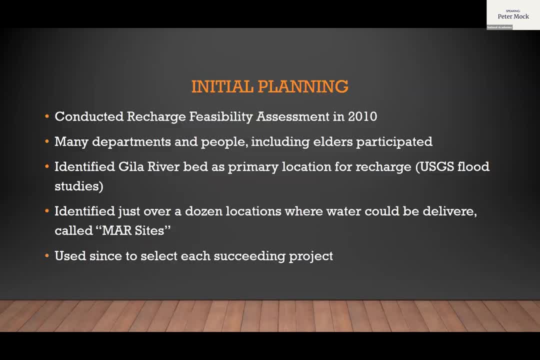 to help restore their culture. Next slide. So we conducted a recharge feasibility assessment in 2010.. When I was at CH Stonehill, I worked on the Tucson recharge feasibility assessment as a young hydrologist and I brought that same approach to this. 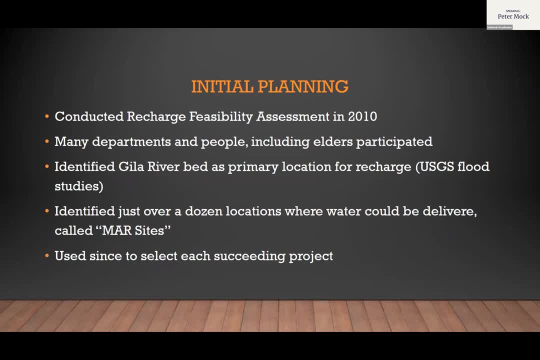 Many departments and people, including elders, participated in that process. We took our time and really listened to everyone and talked through all the options. We identified the Healer River bed as a primary location for recharge and I knew this was looking good because the US Geological Survey had looked at some floods. 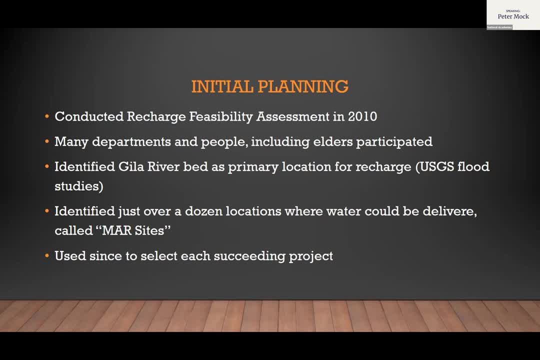 during five months of 1983 and 1984, when a hurricane stalled out over the watershed and 250,000 acre-feet recharged beneath the community during that time, And using that same process that the USGS did, I estimated though: 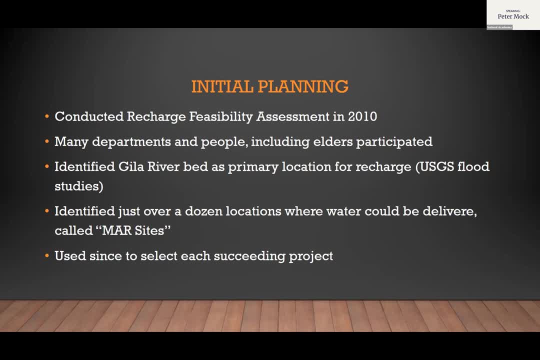 that over a million acre-feet went in in 1993 through 1998, along with 83 floods, That's up 1.5 million acre-feet infiltrated. naturally Again, we had some tremendous atmospheric rivers that came in in 1993.. 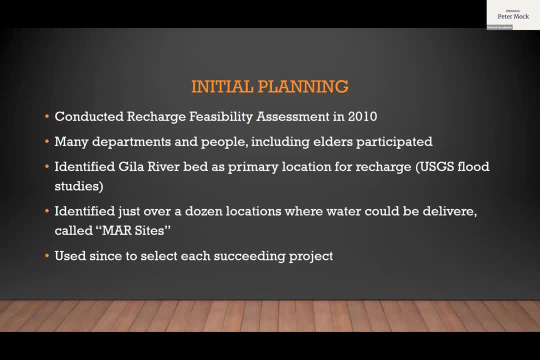 And so that was a great test. I couldn't ask for a bigger test for recharge facility. So I identified just over a dozen locations where water could be delivered to the Healer River channel bed. These are called MAR sites. We numbered them and we talk about them in that vein. 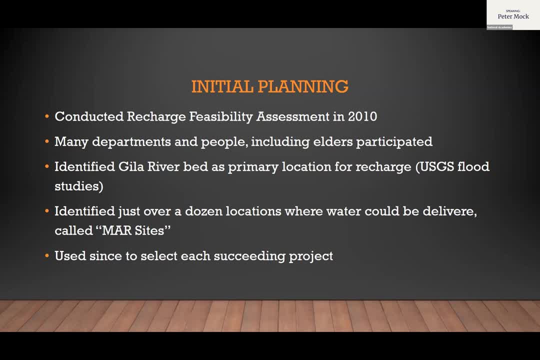 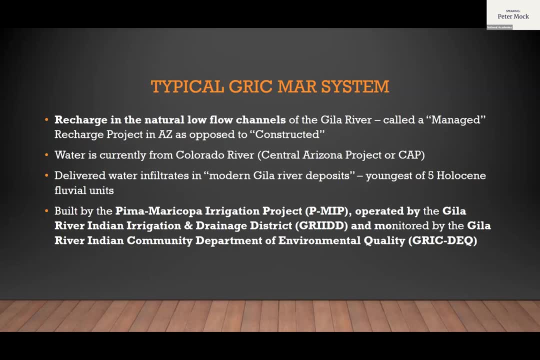 like MAR 1B or MAR 5.. And these MAR sites have been used and the recharge feasibility assessment's been used since to select each succeeding project. Next slide, please. So a typical GRIC MAR system is just to put the water. 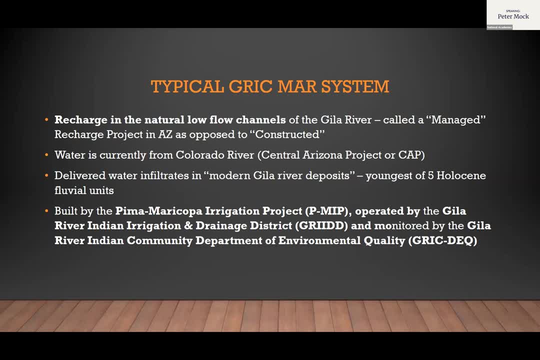 into the natural low-flow channels of the river Healer River, and these are called managed recharge projects in Arizona, as opposed to constructed. The community has an intergovernmental agreement by which this recharge is permitted, and so you know we're going to have to make sure that the recharge is permitted. 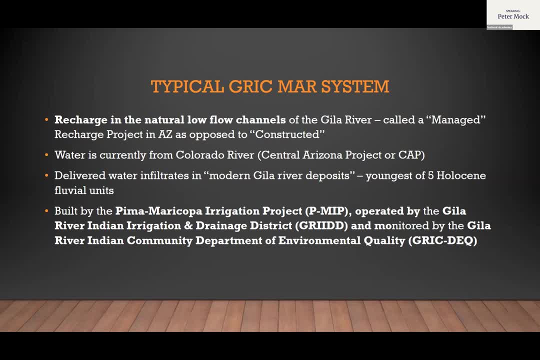 under the state of Arizona system and that system considers this managed recharge, where you don't do anything to the channel as opposed to putting in basins Water's, currently from the Colorado River. This is called Central Arizona Project for CAP Water. They showed you a picture of the CAP. 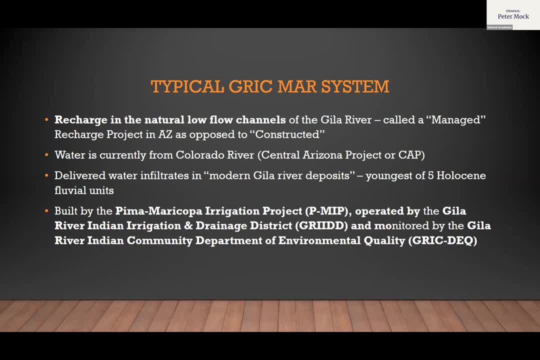 coming through Central Arizona previously. The delivered water infiltrates into the modern Healer River deposits, which are the youngest of five Holocene fluvial units. We have extensive surficial geologic mapping through the area and this one. these are 500 years or old, or less. 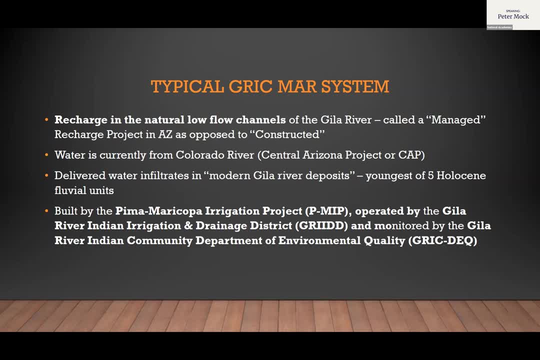 So this entire system is built by the Pima Maricopa Irrigation Project, It's operated by the Healer River Indian Irrigation and Drainage District and it's monitored by the Healer River Indian Community's Department of Environmental Quality. Next slide: 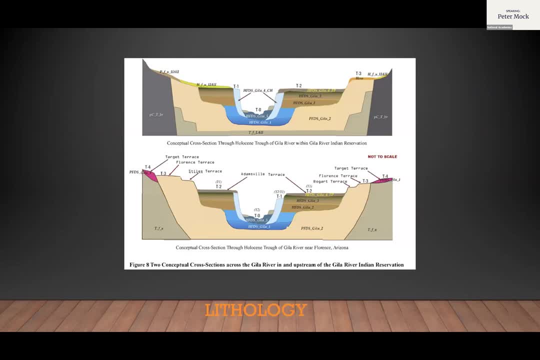 So just to give you a feel for the cross-section, these are vertically exaggerated, but the Healer River does its work by cutting and partially refilling, and where we are doing our recharge is where you see T0. there It's the youngest unit. 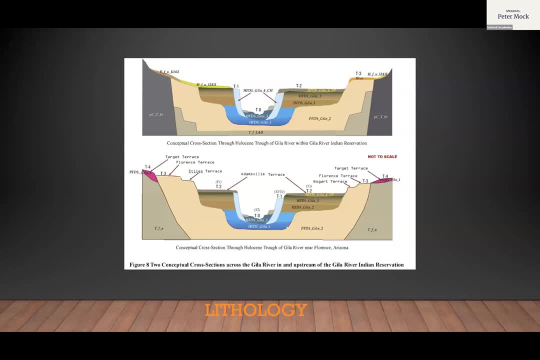 In the latest incision and refilling. and these are not big cliffs. These are only about that inner cut that, you see, is only about two or three feet, two, four feet high, But beneath it are the Pleistocene River sediments. 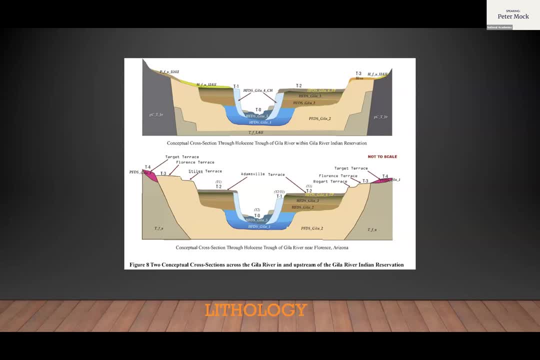 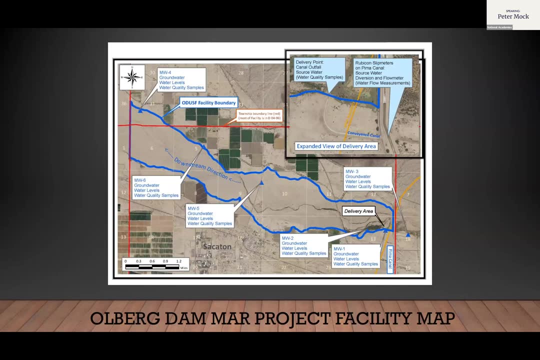 of the Healer River and beneath that is more typical sedimentary basin. Next slide, please. Here's the Oldberg Dam Underground Storage Facility. It's about six miles long and the river flows from the lower right to the upper left. 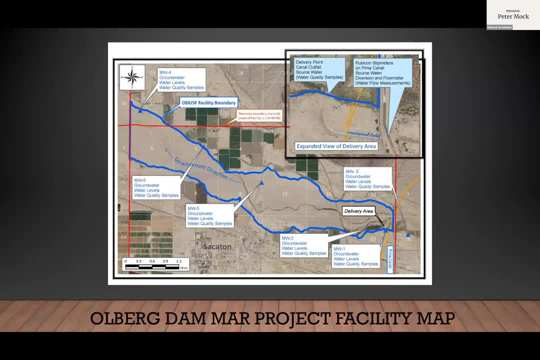 and the deliveries are to the point says delivery area. We have six monitoring wells to track water levels and to take water quality samples. There's a blow-up here in the top corner, expanded due to the delivery area where an agricultural canal is used to obtain the water. 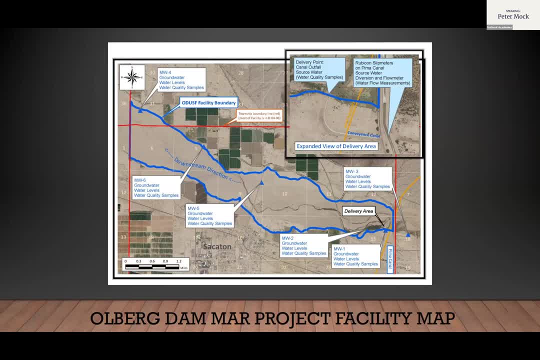 Two Rubicon slip meters are used. We'll talk about that in a little more detail- to a delivery point and you can see just really quickly under the word delivery area that multiple channels are receiving the water, Just the natural low-flow channels of the Healer River. 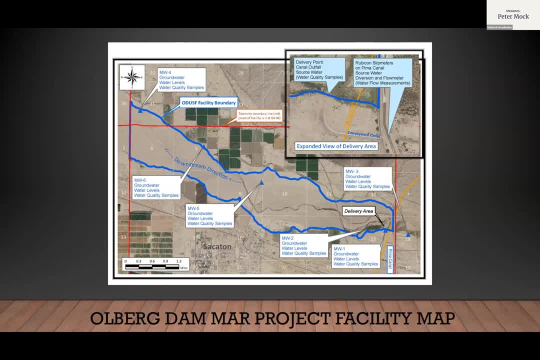 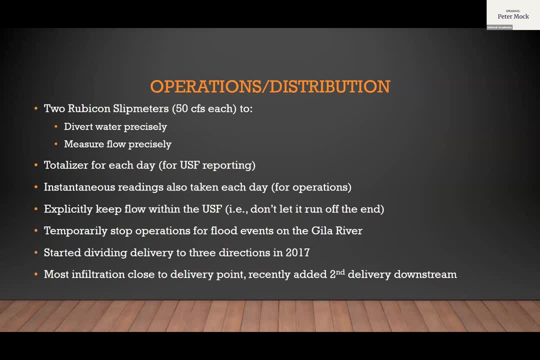 and then it extends for about three miles before sinking in all the way. Next slide, please. So two Rubicon slip meters, 50 CFS, are used to both divert and measure quite precisely. It's an impressive piece of machinery. We have totalizers for each day, for USF. 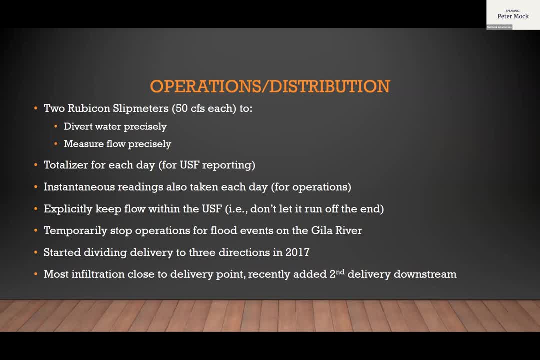 or Underground Storage Facility reporting under the permits, as well as instantaneous readings that the staff takes every day just so operations knows about what the flows are. They explicitly keep the flow within the USF. This is a permit condition. so we define arbitrarily define that lower boundary. 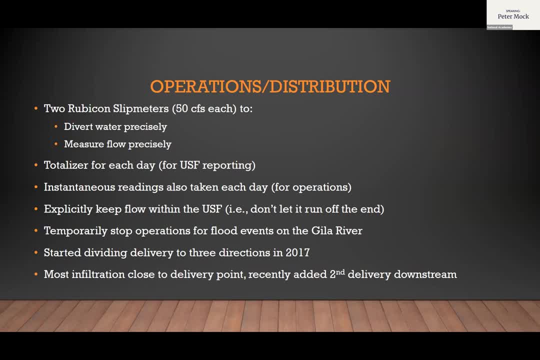 and just keep the flows all within them and we temporarily stop operations when there are flood events on the Healer River, which have occurred a few times. We haven't had any large ones since we started recharging and we started dividing the delivery to three directions. 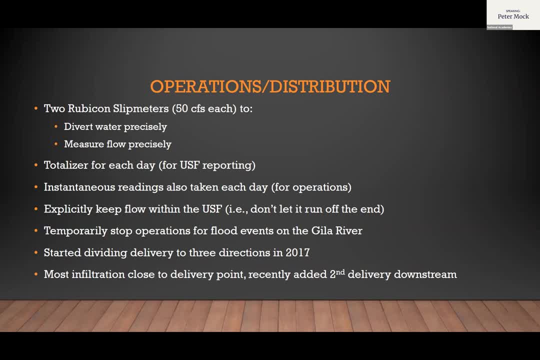 as you saw before back in 2017.. We found most infiltration happens close to the delivery point, as you'd expect with such a system that can infiltrate water so well, and so we've recently added a second delivery downstream underneath the permit, and that's been operating for much of 2021. 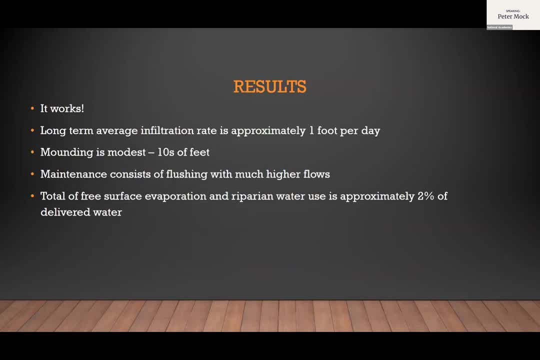 Next slide, please. So it works. Long-term average infiltration rate is approximately one foot per day. Mounding is modest. It's 10 to 20 feet or so. The pre-recharge depth of water was 90 to 100 feet. 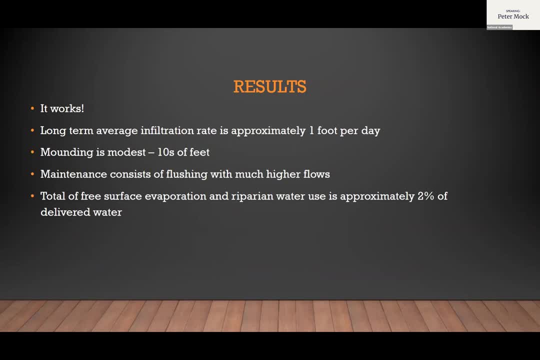 and in general in the area it's come up a few tens of feet. Maintenance consists of just flushing with much higher flows. so if they run at 20 to 30 CFS they'll blast it at 100 CFS for a day or two. 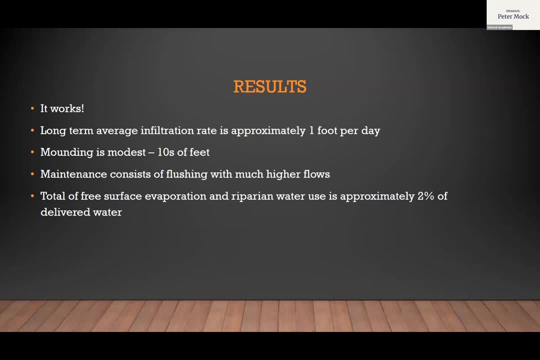 to scour the channels, naturally, And, what was interesting, although we're comparing notes with other operators of similar systems- found similar results. the total of the free surface water, surface evaporation and the riparian water use is approximately 2% of the delivered water long-term. 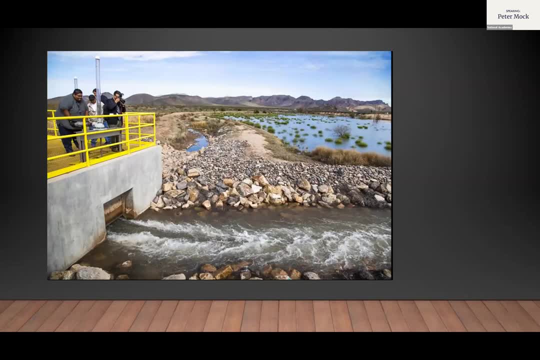 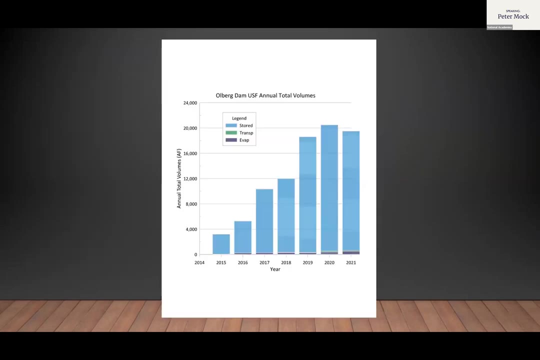 Next slide, please. So here's the outlet structure. There's some riprap there to control erosion And then you see an area where the low-flow channel causes a bit of extended pining and then off it goes. Next slide: Two-minute warning. You bet. Here's the total volumes that have been recharged from 2015 to recently and you see we've been running at about 20,000 acre-feet per year And you see the proportions of the water that's stored. 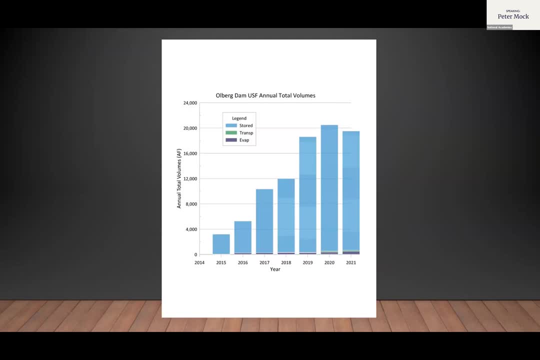 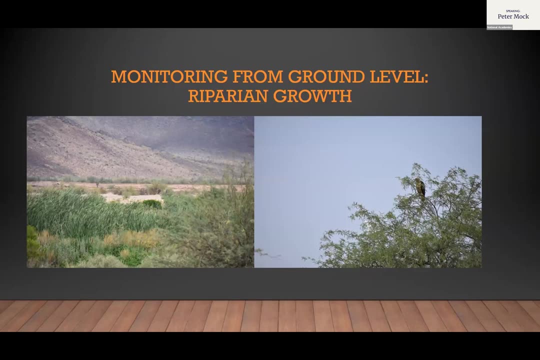 actually recharged versus transpiration evaporation- Next slide. So monitoring happens Both at the ground level for riparian growth. You can see the riparian growth that's now come in in certain areas And on the right is one of many raptors and wonderful brood. 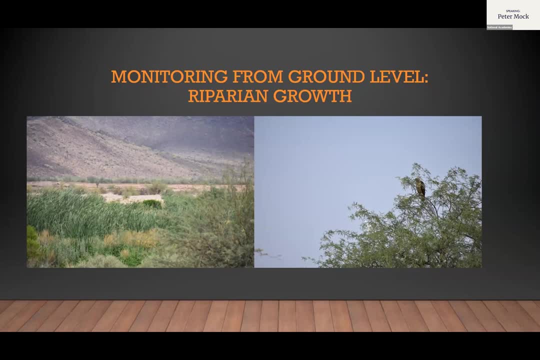 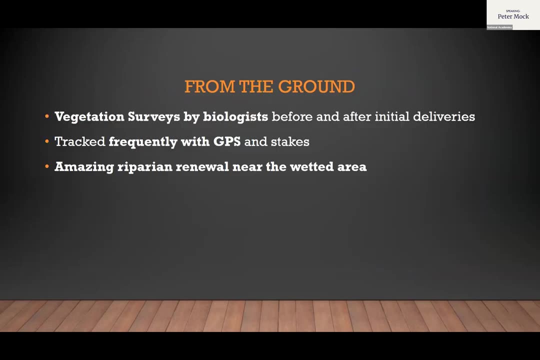 populations that have moved into the area. Next slide, Next slide, please, Thank you. We started with vegetation surveys by biologists before and after deliveries. We tracked it with GPS and stakes. It's just been amazing renewal. Next slide: Now we've gone to using drones. 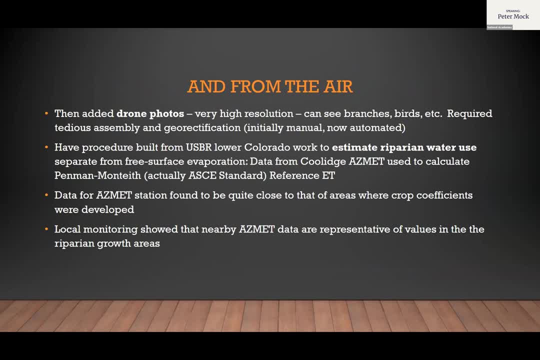 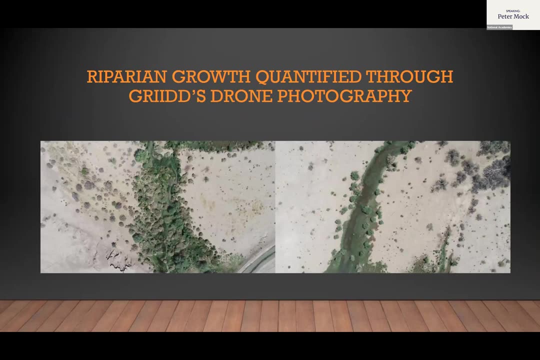 The drainage district. staff fly the drones and we have an on-bed procedure for using that And we estimate riparian use with a fairly sophisticated process. Next slide, And that's what the drone photos look like of the re-establishing riparian area. 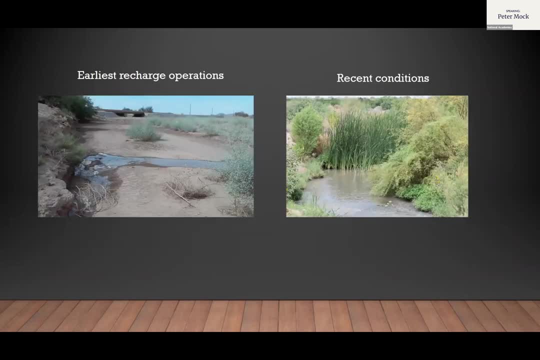 Next slide, please. On the left, you see what it looks like when the first dribbles of water came across, And now you see what it looks like in some of these needs near the wetted area. Next slide: A really big part of this that's different from what you may have. 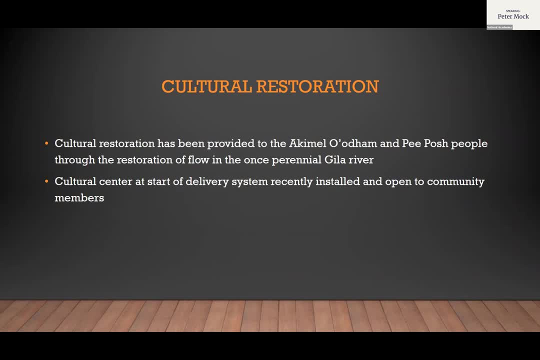 seen before, is that this really has helped cultural restoration for these peoples? I can't go into the details of what it means for them to have a re-established river and riparian, natural riparian growth And, by the way, the riparian growth was not. 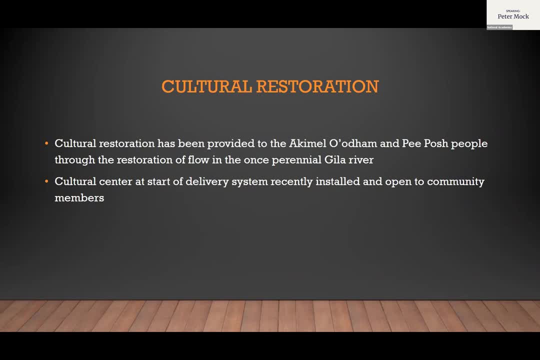 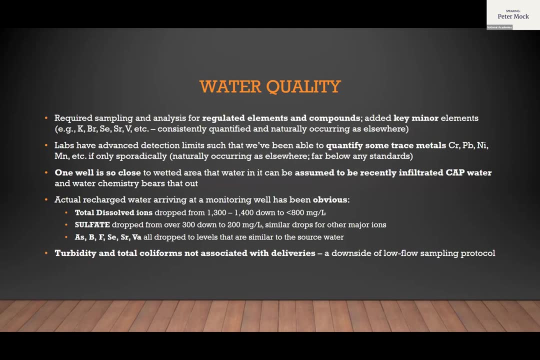 seen with all the dry channels When the water was added. that just sprung up. Next slide The water quality. just briefly, let's just skip down to the bottom. Here are the total dissolved ions dropped from the native water: about 1,300, 1,400, down to about 800 milligrams per liter. 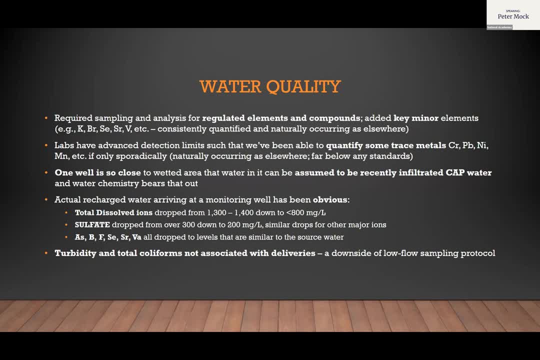 And sulfate drops from 300 to 200.. There are similar drops in the other major ions and some minor ions, But we have noticed that we had some problems with turbidity and total coliform. They really weren't serving as indicators of the arrival of pollutants. 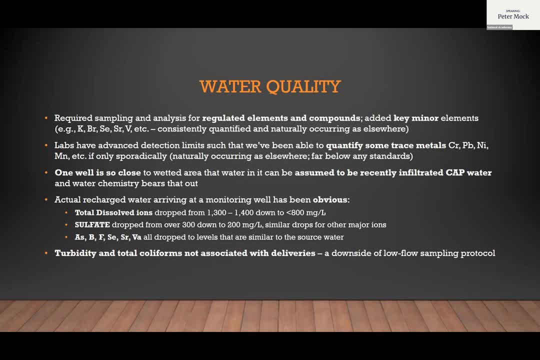 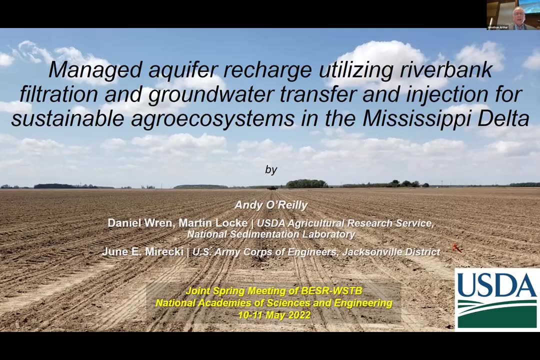 These are biofilms that build up in stagnant wells, And this is a downside of low flow sampling. Although it's an industry standard, it does cause some problems for the water. just sitting there. With that I'm done. Thank you, Peter. thank you. 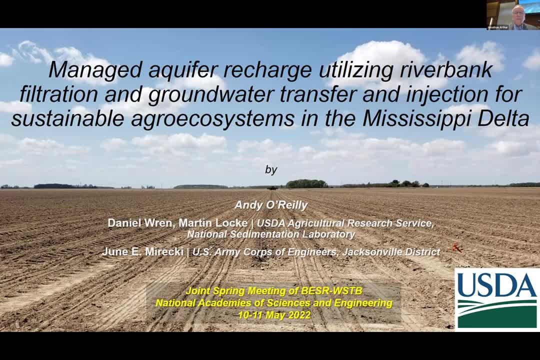 We'll move on to our next speaker, Andrew O'Reilly, with the USDA Agricultural Research Service, where he is a research hydrologist, And he also works at the National Sedimentation Laboratory in Oxford, Mississippi. Andrew Conductor Research on Groundwater Sustainability and Agroecosystems. 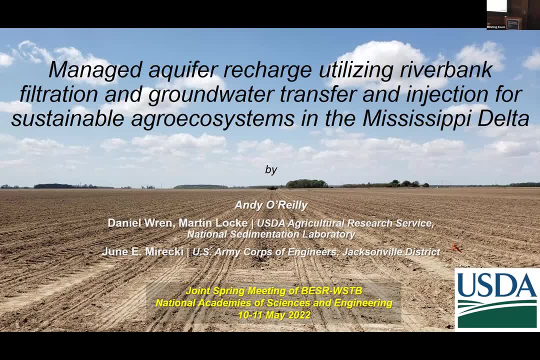 focusing on beta-osone and groundwater, hydrology, green infrastructure and much more, Andrew. All right, Thank you for that introduction, John. I appreciate the opportunity to speak with you all today And I want to talk to you about a pilot project. 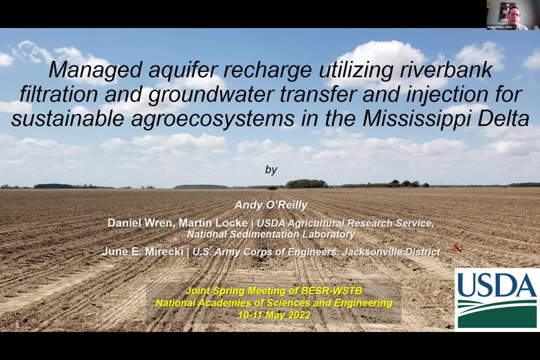 It involves utilizing riverbank filtration. combine that with the groundwater transfer and injection with the objective of obtaining a sustainable agroecosystem, And the project area is in the middle. We're in the middle of the city of Mississippi Delta. I'd like to recognize my collaborators: Daniel Wren. 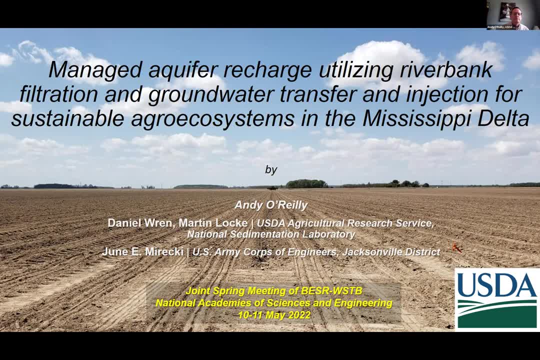 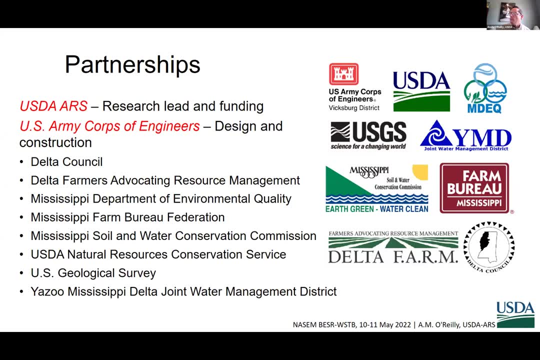 Martin Locke of USDA and June Berecky with the Corps of Engineers. Next slide. I'd also like to acknowledge a wide variety of partnerships. In particular, the USDA, ARS and the Army Corps of Engineers Vicksburg District have been working closely. 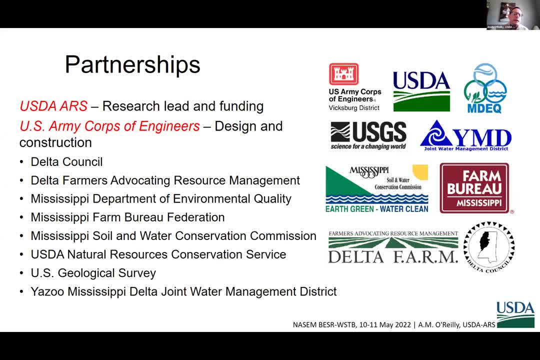 to design and implement these projects And I'd like to acknowledge the partners of the USDA, ARS and the Army Corps of Engineers Vicksburg District who have been working closely to design and integrate these projects. We also have worked closely with石wood andIRV to build and build. 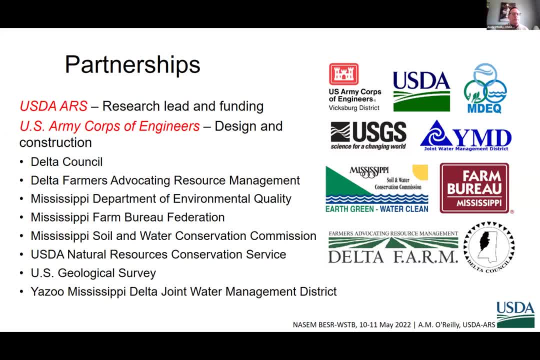 perform the research and operate and maintain the system, And without the two agencies working together, it wouldn't be happening. Also, there's wide variety of other stakeholders at the local, state and federal level that have been instrumental in getting the project going and keeping it going. 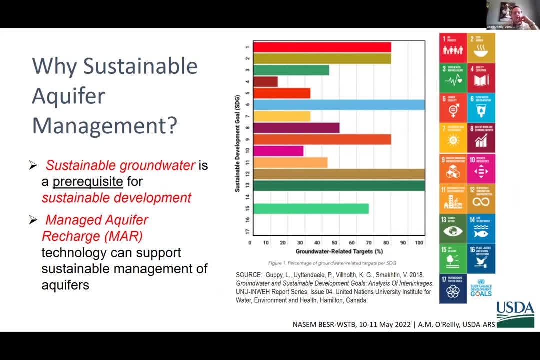 Next slide, please. Let's first start off with sort of the obvious question, And I think we all kind of know the answer here. But why? Why we want to be concerned about sustainably managing aquifer, and I kind of summarized it as sustainable groundwater, as a prerequisite for sustainable development, As you may know. 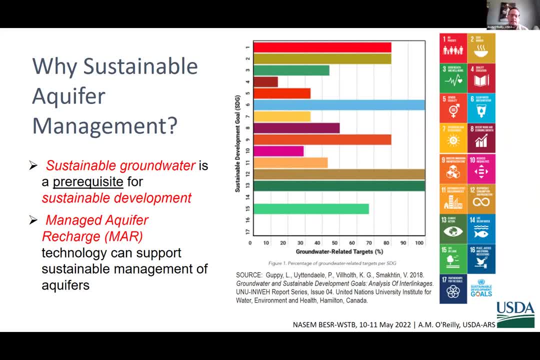 the United Nations developed 17 sustainable development goals and you see this little graphic here to the right that 14 of those 17 goals have a groundwater-related target. So in order to meet that goal, there's targets that have to be met that are related to groundwater. 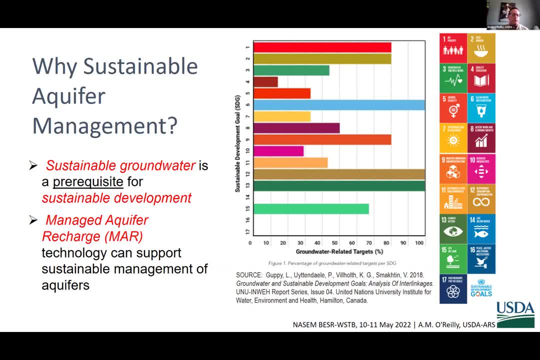 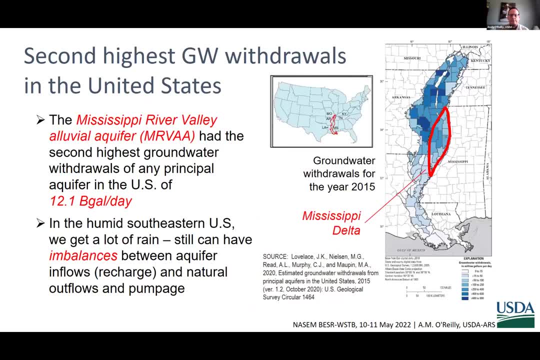 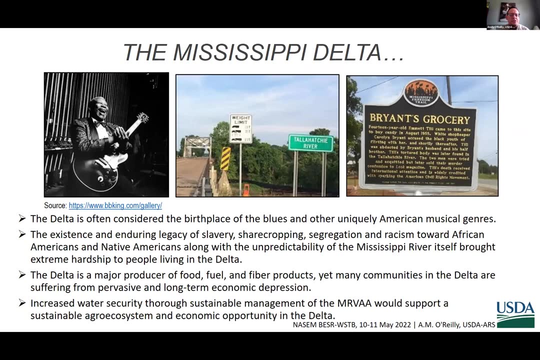 So groundwater can't be underestimated and, of course, managed aquifer recharge, which is one technology that can support this Next slide. please Taking one slight diversion to a little bit about history of the Mississippi Delta. If you've never been there, it's a very unique, very unique region. 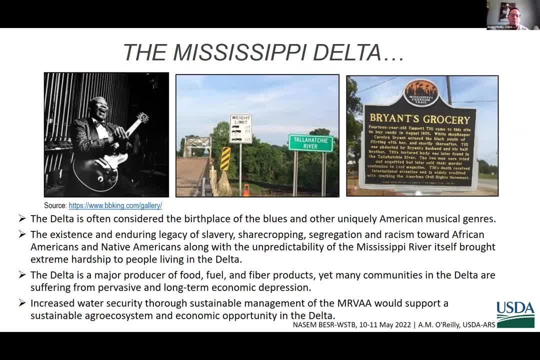 It's generally considered to be the birthplace of the blues and other American musical genres, But it also has a long history of racism, slavery toward African Americans and Native Americans. The murder of Emmett Till and his body was found in the Tallahatchie River. It was largely 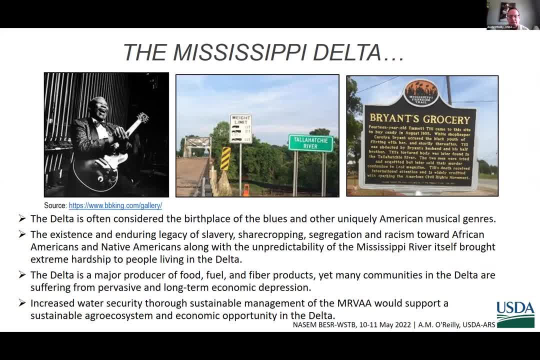 considered a seminal event in getting the civil rights movement rolling. So a lot of difficulties in the Delta. The Delta is a major agricultural region, but many communities of the Delta still suffer from pervasive, a long-term economic depression. So, ultimately, the objectives, the overarching objectives of this project, or a follow-up expansion the project would be the 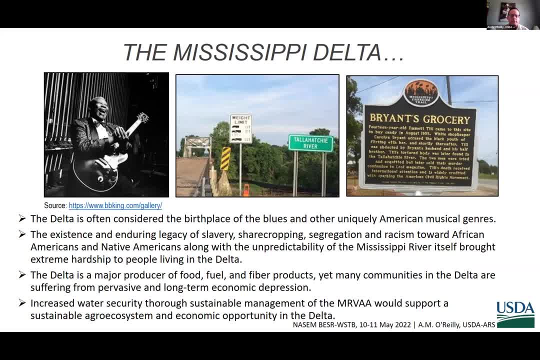 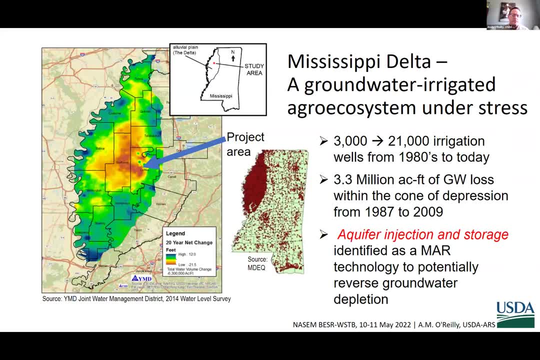 increased water security in order to provide a sustainable agro ecosystem and sustainable economy in the region. This is essentially a nutshell, the main scope of this project, But in the first instance, Michael B came up and outlined when it came to sustainable agronomic ecosystems. Here you can see the 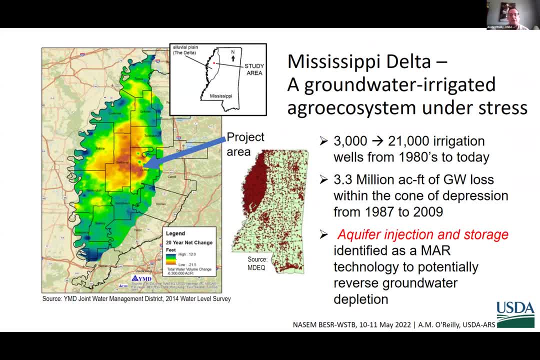 the Mississippi Delta is a groundwater irrigated ecosystem under stress. There's been a seven-fold increase in the number of irrigation wells in Mississippi from the 1980s to today. And the little diagram of the state of Mississippi you can see the vast majority of those are located. 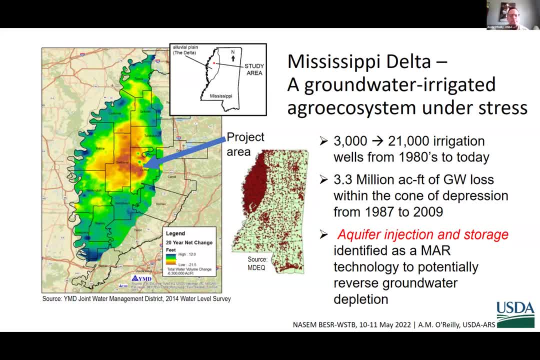 in the northwestern portion of the state, which is the Delta, And estimates of over 3 million feet of groundwater have been lost within the central part of the Delta within a COVID depression from the mid-80s to the late 2000s, And this has been a well-known problem. It's 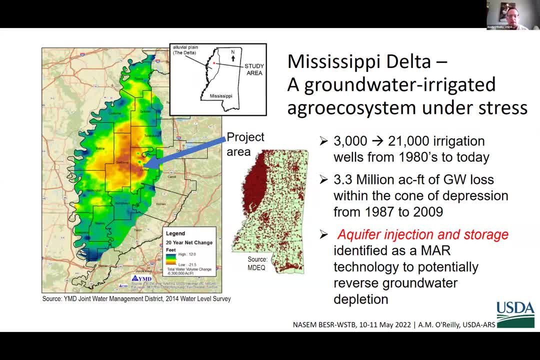 been going on for decades. A number of studies have been done and aquifer injection storage identifies one more technology that might potentially reverse this trend to groundwater pollution. Next slide, please. This slide pretty much subs up the entire project. It's a little bit more detailed, but it's a little bit more detailed, This slide pretty. 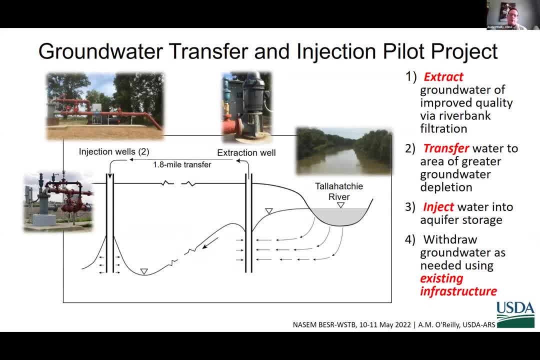 much subs up the entire project. It's a little bit more detailed. but it's a little bit more detailed. This slide pretty much subs up the entire project In a nutshell. we can look at it as four components. First, we extract groundwater from an extraction well that's adjacent to the 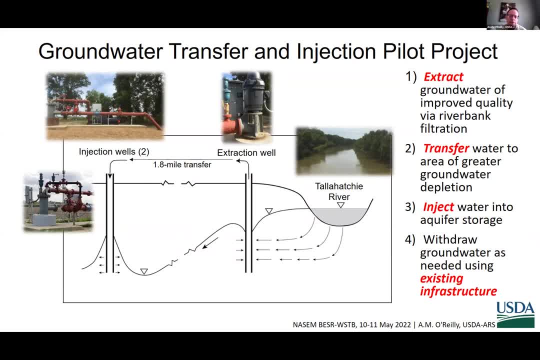 Tallahatchie River. So this is a riverbank filtration scheme. So by pumping that well we induce leakage of water from the river and improvement of the water quality In the process. we take that water, we pump it about two miles to the west and inject it into two injection wells. 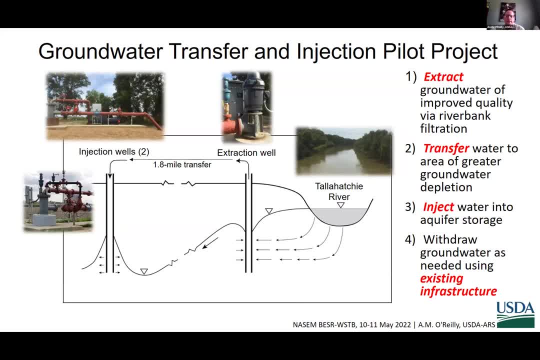 And fourth, one of the key attractions of this scheme is that, of course, the water is stored in the aquifer and then it can be withdrawn as needed using the existing irrigation infrastructure in the region, So the farmers don't need to develop. The vast majority of the farmland is irrigated with. 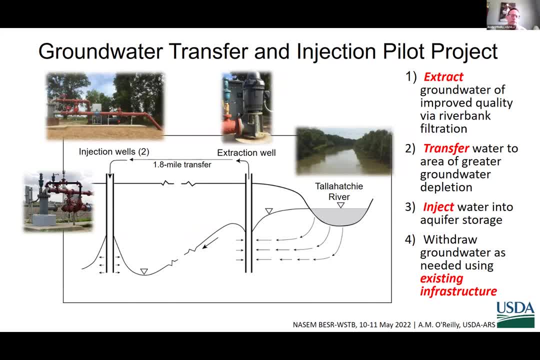 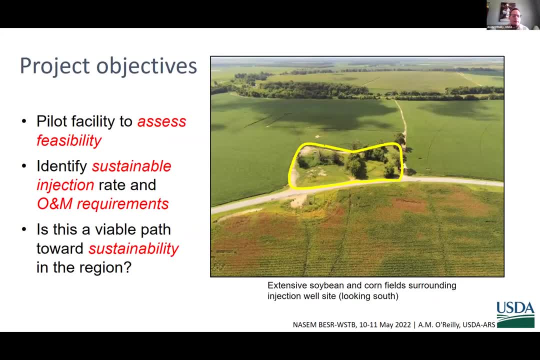 groundwater already, so they don't have to develop any new irrigation infrastructure with a scheme such as this. Next slide, please: The project objectives. it's a pilot project, So we're assessing feasibility. We want to identify sustainable injection rates and appropriate 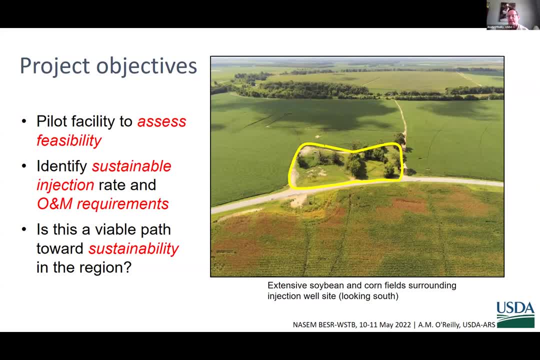 operation and maintenance requirements. The photograph here to the right is the aerial view of the injection well site, as soybeans and corn were planted at the time. This is typical view of the delta. You can see pretty much everywhere you see is cultivated And ultimately, 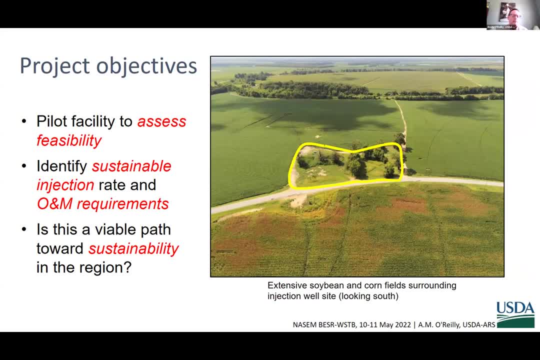 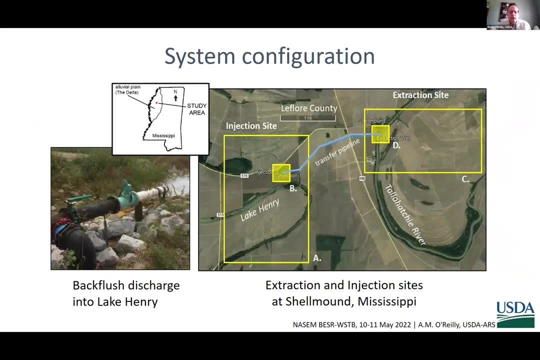 we want to determine: is this technology a viable path forward towards sustainability in the region? Next slide, please, A little overview of the layout of the system. On the right-hand image, the extraction site. as I mentioned earlier, there's one well adjacent to the Talianchi River. 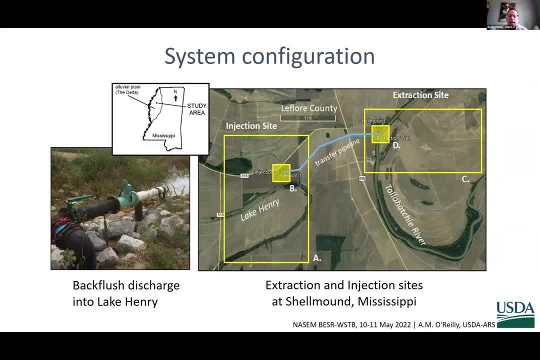 You can see there's a bend in the Talianchi River And the pipeline shown in blue, and then the two injection wells located at the injection site And the large yellow boxed regions are areas that have about six-to-eight monitor wells, monitoring impact for the system And look with 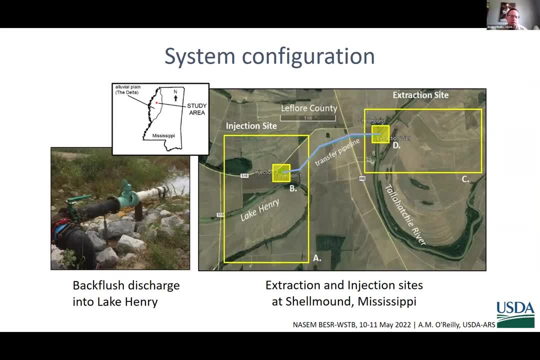 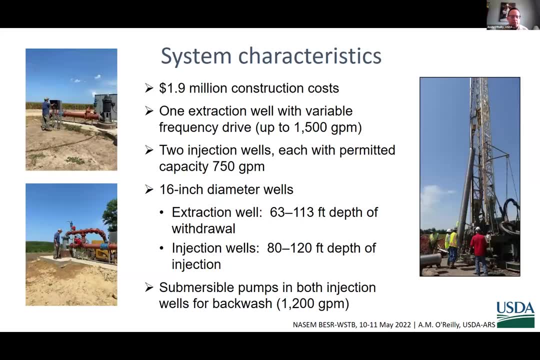 any injection well, back flush is part of the necessary operation maintenance practices. So we discharge your backwash water to Lake Henry, which is just south of the injection wells, And, yep, you can go to the next slide. A little bit more about. 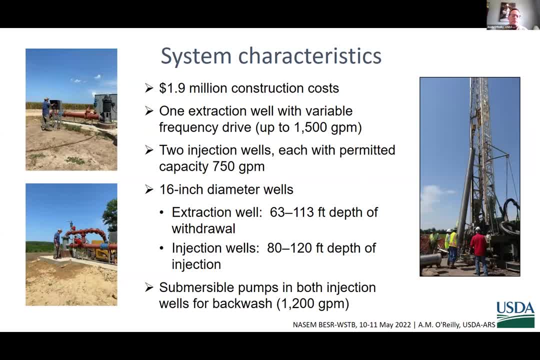 the system characteristics is about nearly the $2 million construction costs. We can adjust the flow rate on the extraction well as needed. Each injection well is permitted for a capacity of 750 gallon per minute. All the wells are 16-inch diameter. They're all essentially identical. 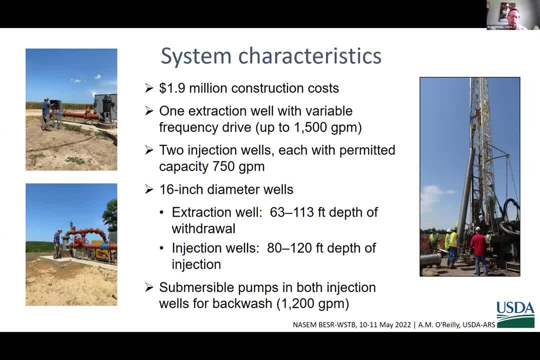 The extraction well is a bit shallower than the injection well, but it's still on the range around 220 feet deep And each of the two submersible- I'm sorry, each of the two injection wells have a submersible pump for back washing at about 1,200 gallons per minute. Next slide, please. 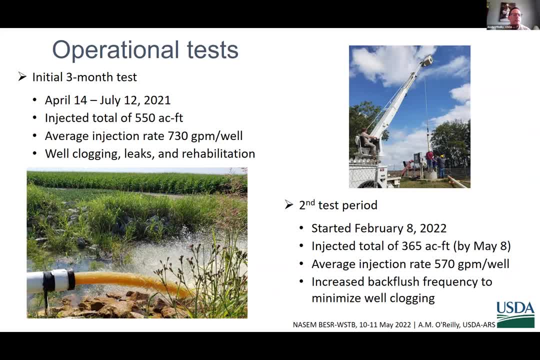 So we've conducted two operational tests so far. The first was an initial three-month test. from mid-April to mid-July of last year. We injected a total of about 550 acre feet of water. The average injection rate was about 730 gallons per minute per well, And it ended with the unhappy 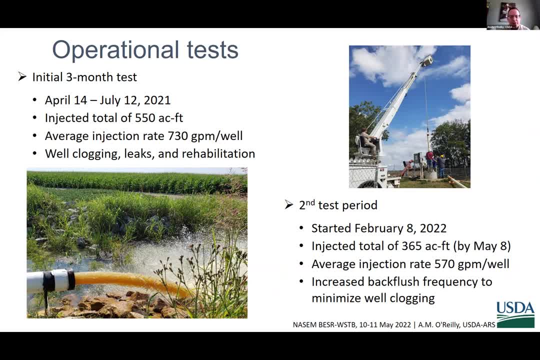 major clogging event requiring a rehab operation, And I'll get a bit more into that in the following slide. We have started a second operational test. that started in early February of this year. So far we've injected about 365 acre feet. We've reduced the injection rate to around 570 GPM per. 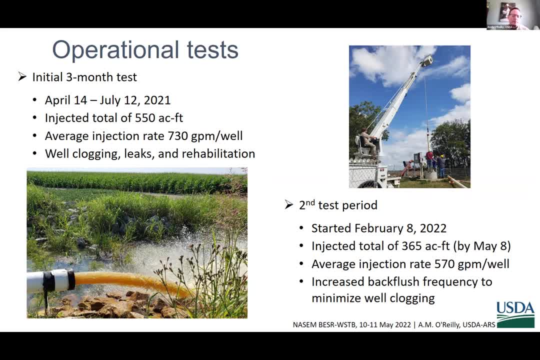 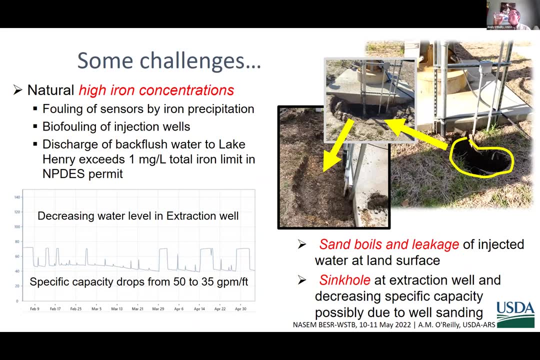 well, And also we've increased the back flush frequency And both of these are to minimize well clogging issues. Next slide, please. So some challenges. There's been many of them for the project, But just hitting some of the highlights The groundwater in the region has. 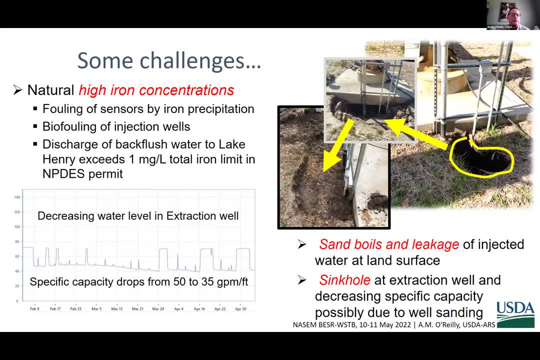 naturally high iron concentrations So that results in fouling of water quality sensors, fouling in the injection wells. I'll get to that in the next slide. Also, we discharge our back flush water to Lake Henry And the one milligram per liter is the typical iron limit for aquatic ecosystems. We're not able to. 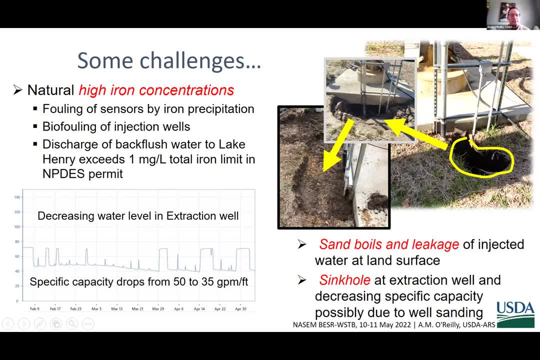 meet that? certainly because the groundwater naturally actually already has iron concentrations of about 10 milligrams per liter on average. The clogging event resulted in a sand bonus and leakage of the injected water at land surface, Something you definitely don't want to happen. 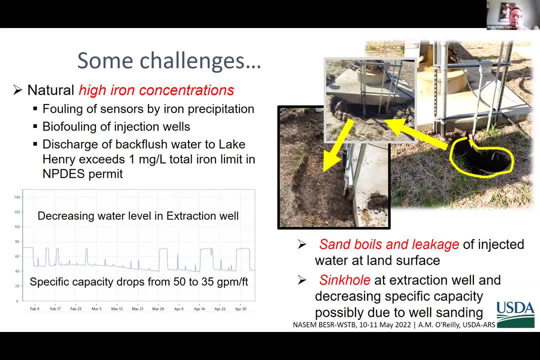 I think that's what Eric showed- A little bit of an example We've up here in Gee and Geeville and then a little bit into the пример as well and at some of these ones and this auction project in Geneva via the unlimited resource fund. 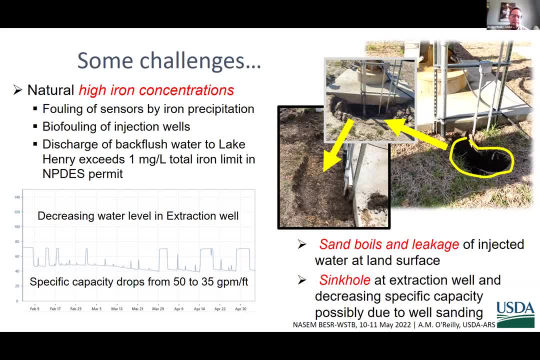 And these are right next to what was called, I think, Research Road ort Board, and a particular project is being performed for friends of Greenville, and that is we actually have been ables of a worker's lab at the work site. She's never been there, and so we're more than 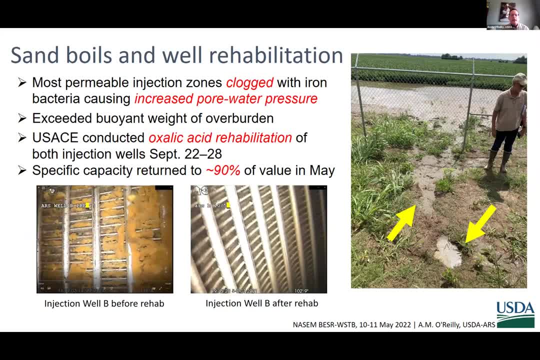 говорить of our province, of impending effect, But maybe the devious conditions are less than the extent of or related damage to sails and waterity issues and over time we're utaned from any risk factors that might be relevant, Such as Joe Wood. We've had a sinkhole develop at the extractio. 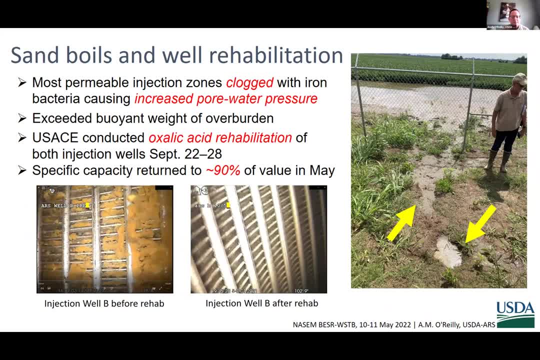 Here was our unhappy clogging event. In mid-July we got a phone call from a local farmer saying there's water flooding out around your wells. Is this what's supposed to happen? So we shut them off. We went out there the next day and, as you see on the right-hand photograph, 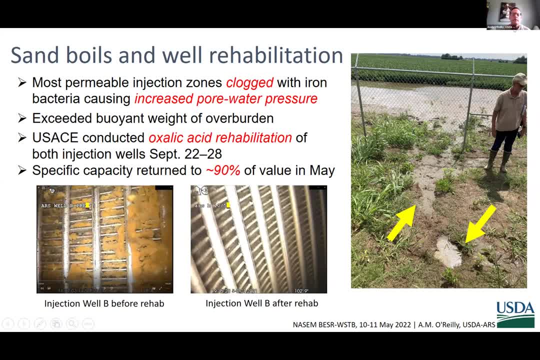 there are several holes around each injection well where there was essentially sand boils, muddy water coming out, injected water. In a nutshell, basically, we exceeded the buoyant weight of the overburden, which in hindsight seems pretty apparent, but at the time it wasn't clear. 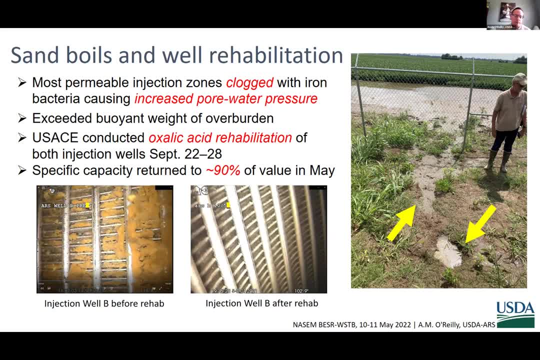 The Corps of Engineers conducted an oxalic acid rehab treatment of the wells. You can see here on the lower left-hand is a video log that the Corps ran. So the left-hand one is quite a metabiotic. The right-hand one is a biomass iron reducing bacteria adhered inside the well screen After the oxalic acid treatment. 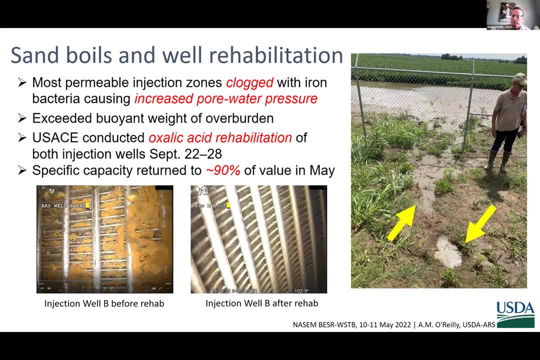 we had a significant improvement, as you can see by the right-hand photograph, and the specific capacity was returned about 90 percent of the value. it was in May, near the beginning of that first injection period, So we were really pleased that it all was able to be rehabbed. 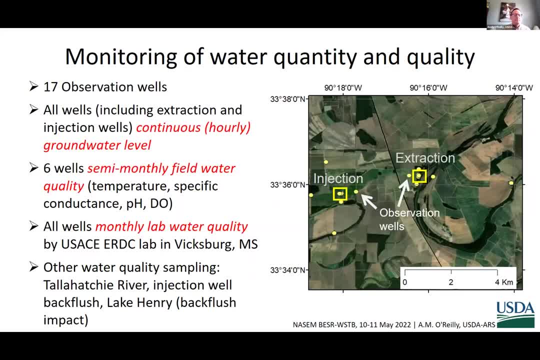 successfully. Next slide, please. Okay, so the last few slides. I wanted to touch upon more of the positive aspects of the project, so to speak, rather than the problems. We have an extensive monitoring network. The map to the right. as I mentioned earlier, we've got monitor wells around the extraction. 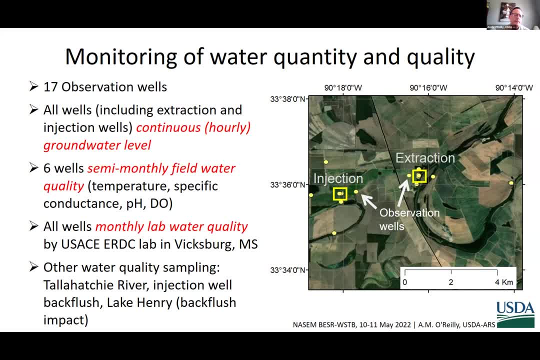 well site and monitor wells around the injection well site, 17 in total. All the wells are monitored continuously, at least hourly for groundwater level. Six of those 17 wells are monitored twice per month for field and water quality parameters, temperature and conductance, pH and dissolved 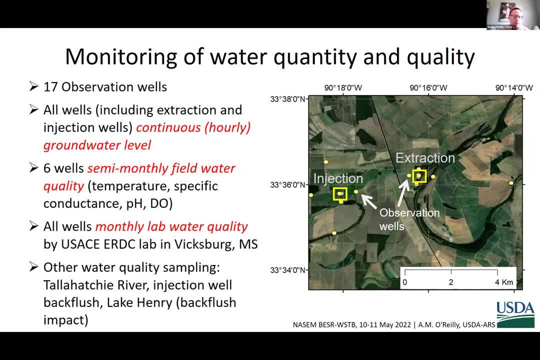 oxygen. While the system is operating. we sample all the wells monthly and those are analyzed by the Corps of Engineers ERDC lab in Vicksburg, Mississippi. And in addition to sampling monitor wells, we also sample the Talangie River. 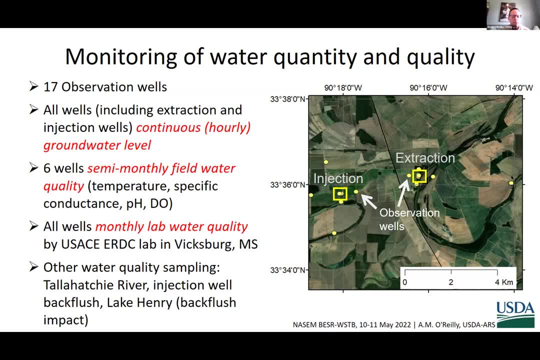 which is a large lake in the area of Lake Henry, and some are measured in the injection well back flush water as well as Lake Henry itself, in order to assess any impact to the back flush water on the lake. Next slide, please. Okay, so here's the data. Here's some of the data from our ground level monitoring. 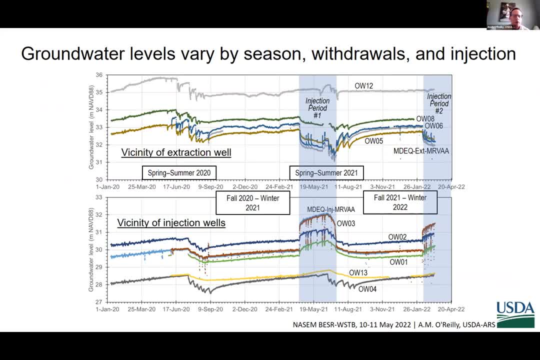 To sort of walk you through it. the upper graph are monitor wells near the extraction well site. The lower are monitor wells near the injection well site. We started collecting data there and, as I mentioned earlier, we started getting data from the groundwater level monitoring. the upper graph the monitor wells near the extraction well site and the lower are monitor wells near the injection well site. 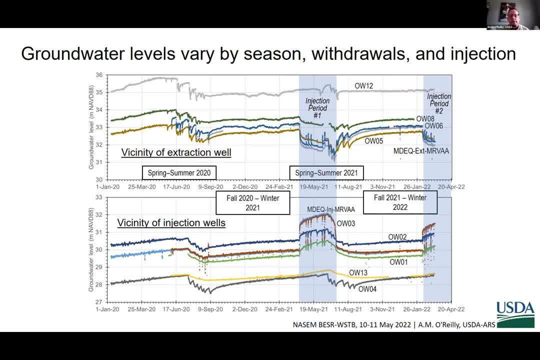 as early of January of 2020, so we have over a year of background data and we see some clear trends. There's not been much continuous water level monitoring in the alluvial aquifer in the region, but you can clearly see rising water levels during the winter and early spring. 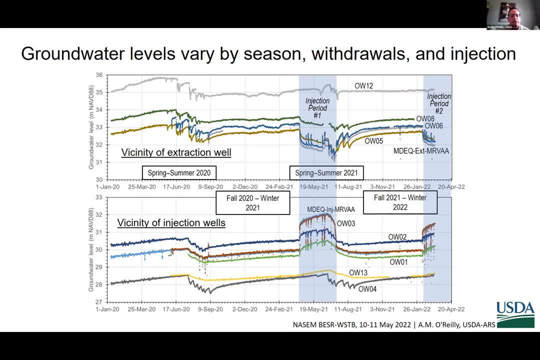 These drops in water levels in the spring-summer. those are drawdowns due to irrigation pumping. Then you have some recovery after that. Our first injection period shown by the first blue-shaded region was mid-April to mid-July of last year At the extraction well site. of course we had 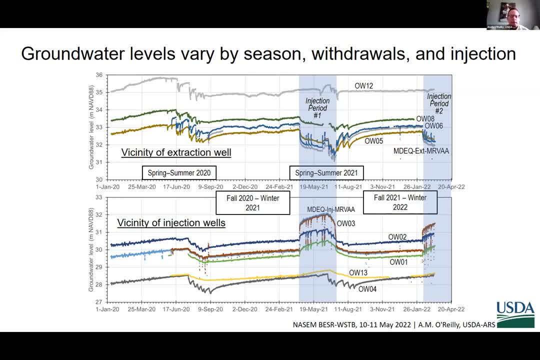 drawdowns of water levels near the extraction well. At the injection well, though, we had a rise in the water level at the monitor wells as much as about six to seven feet, and of course the rise was less The further distance you were from the injection wells. The section injection period is shown here. 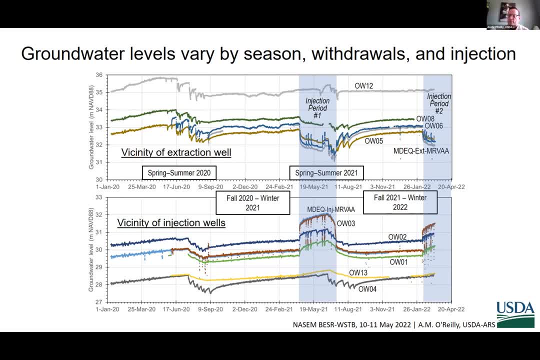 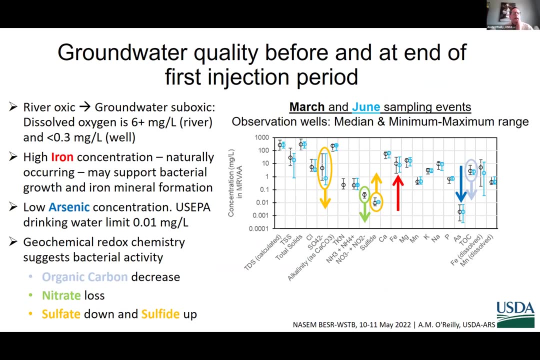 as well. We've had similar responses. then They're just of lesser magnitude because we have a lower injection rate this time around. Next slide, Andy. Okay, thanks. So this will be a last slide of results. A little bit of comparison of groundwater quality. 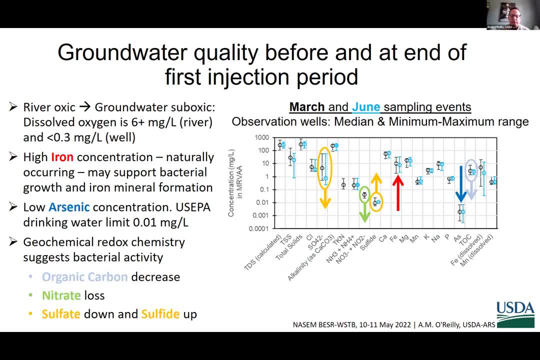 Before and And toward the end of the first injection period, The graph shown to the right. these are the various analytes we're sampling for What's shown and I'm showing the medium max and min values for the groundwater observation wells. The black data is for March, which is prior to injection. 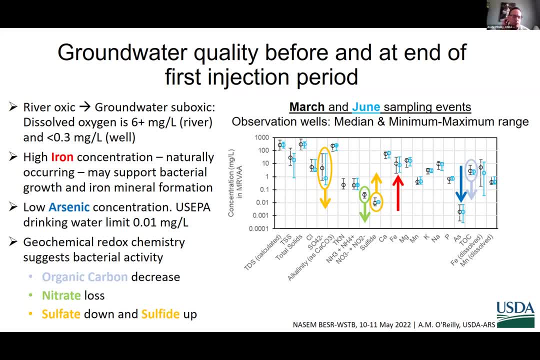 and then the blue are the concentrations in June, toward the end of that first injection, injection period. Just a few highlights I want to point out. The river water itself, of course, is oxic. The groundwater is suboxic. We have a DL of six or so milligrams per liter on average. 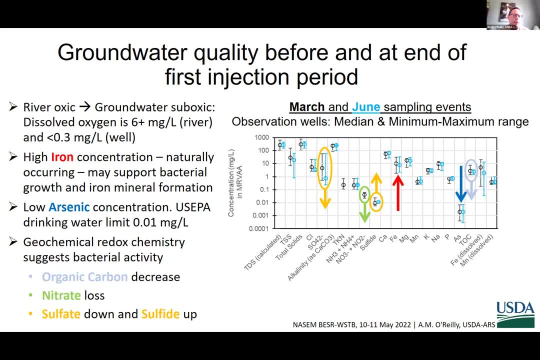 in the river, In the extraction, well, about 0.3 milligrams per liter, And in some of the observation wells it's essentially zero dissolved oxygen. We have high iron concentrations, shown by the red arrow. The median iron concentration is about 10 milligrams per liter, as high as 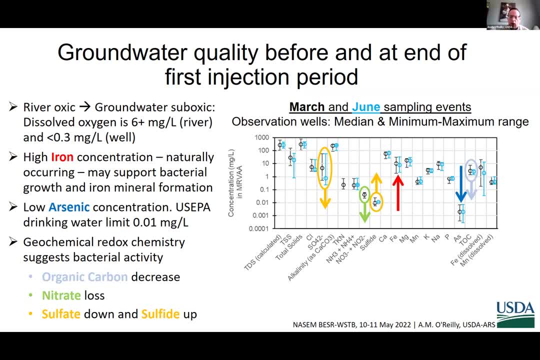 30 milligrams per liter And all iron concentrations exceed one milligram per liter, So that's certainly caused some headaches. as I mentioned earlier, We have low arsenic, or at least arsenic concentrations shown by the dark blue arrow that are below the US EPA drinking water. 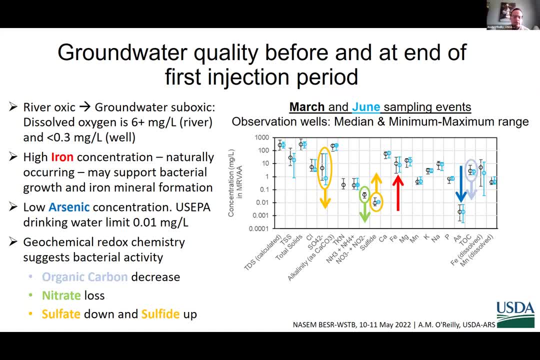 limit And there's been no significant change in those. And also we have some geochemical activity. We have some concentrations that I think are reflective of biogeochemical activity, Some changes in organic carbon concentrations in nitrate and sulfate, And next slide, 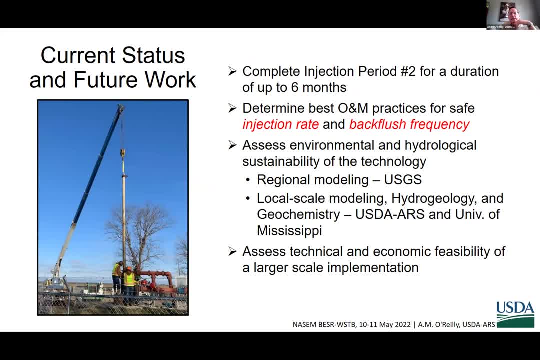 And just in conclusion, kind of where we're headed with this. we want to complete the second injection period. It's been running for about three months. We want to hopefully run it up for a total of six months. We want to determine the best O&M practice. 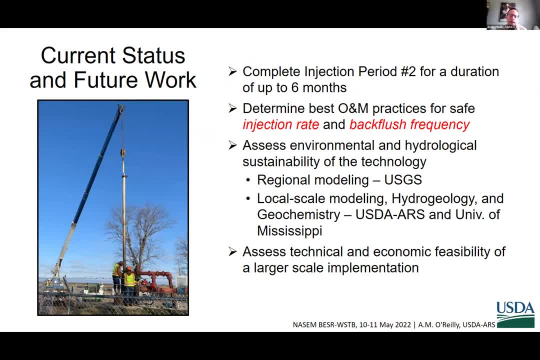 so far at the lower injection rate and the back flush. We're now back flushing twice per week. That has been able to maintain a stable injection well operation. So there's been no indication of clogging whatsoever in the injection wells the second time around. Ultimately, this is a pilot. 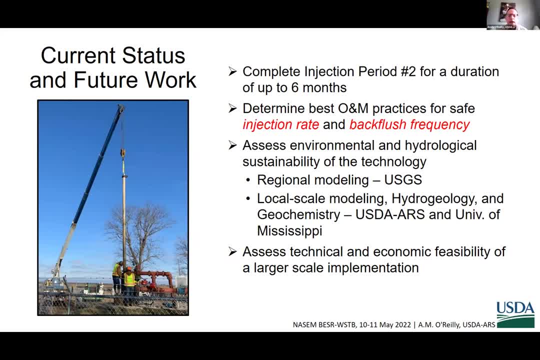 project. So we'll be making some estimates on projections of an expanded version of this technology. The USGS and others will be making some estimates on projections of an expanded version of this technology. The USGS and other is going to be involved in some modeling work with that And next slide. please. 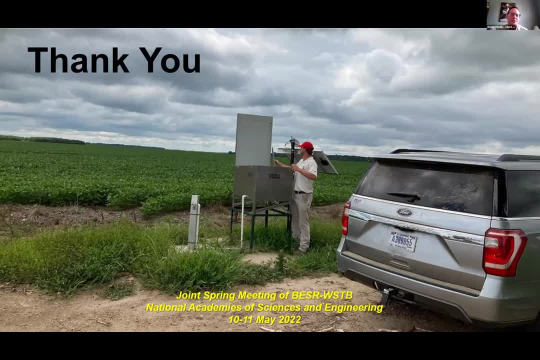 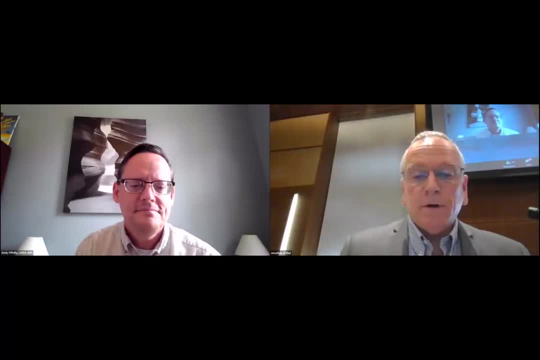 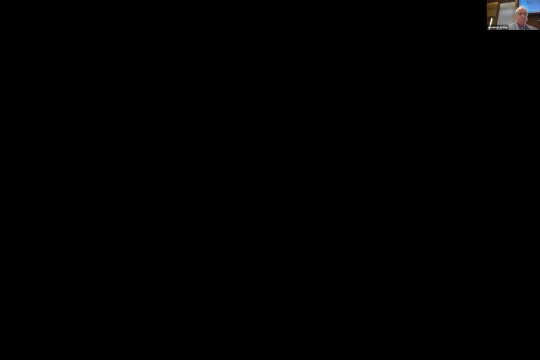 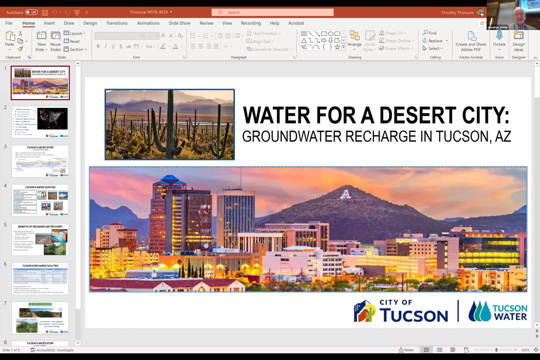 And that's it. I appreciate the opportunity to speak at all today. Thank you very much, Andy. We'll now turn over to our final speaker for the Sorry, That was me. It said unmute yourself, so I did, And that was a mistake. 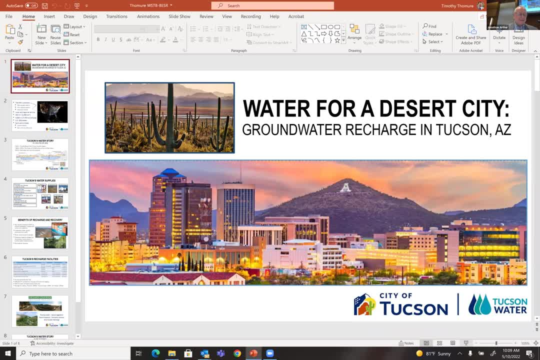 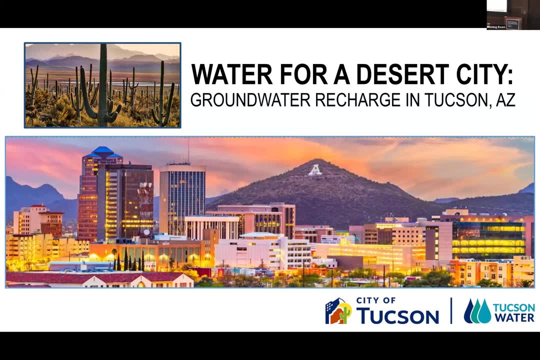 Oh, let's see. Well, Tim, you can help me pronounce your last name before we move along. It's Tomier Tomier. Thank you, Timothy Tomier. Tim Tim is the interim assistant city manager for the city of Tucson, overseeing the public works functions of the city, And he has served on. 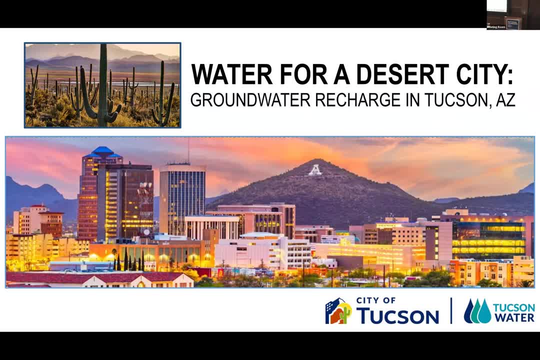 multiple, multiple committees related to reuse, drought, contingency water management and so on, And since we're a little behind schedule, Tim, I'll just turn it over to you. Okay, Thank you very much, And thank you for inviting me out today. 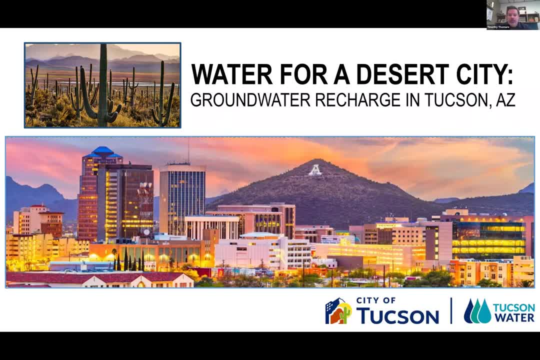 I'll tell a story about groundwater recharge in Tucson, And actually the upper left part of the cover slide shows our iconic Sonoran Desert with the saguaros, And in the background you can see some of our recharge basins in the Abra Valley, which is a big part of our water story. 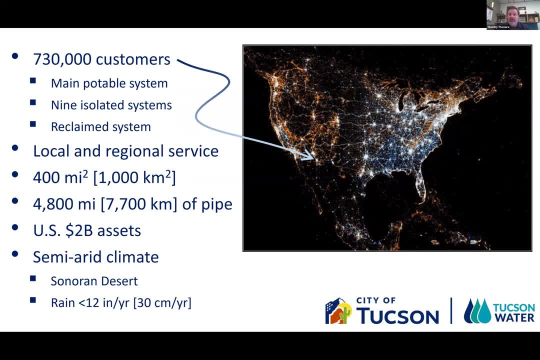 We are located in south central Arizona, So we're the second brightest light in Arizona behind the Phoenix Valley. We have about 730,000 customers through a main potable system, nine rural systems and a reclaimed water system. We do provide local and regional service in a 400 square mile area. 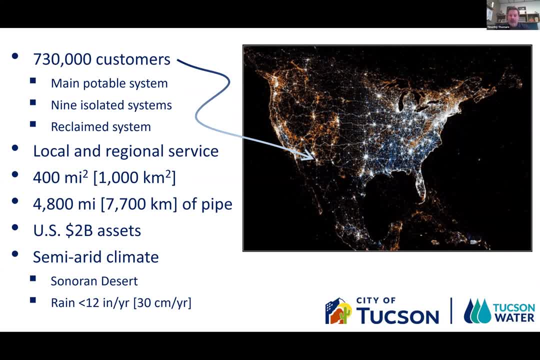 And we're in a semi-arid climate of the Sonoran Desert where rainfall is less than 12 inches per year And when it does come, it almost always comes all at once in our monsoon season. So we have adapted to our desert environment and managed aquifer recharge is a big part of that story. 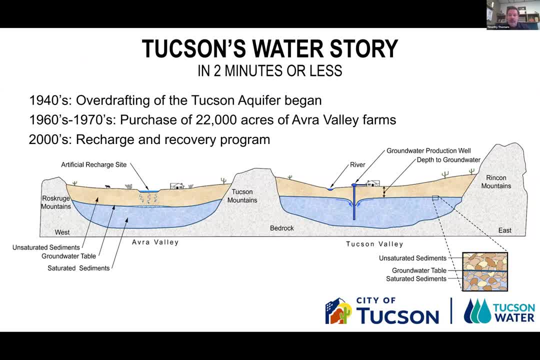 This is a slide that shows sort of the hydrogeology of the Tucson area. This is a cross-section running generally west to east across the slide, And on the right hand part of the slide is where urban Tucson is in the Tucson Valley. It's part of the city. 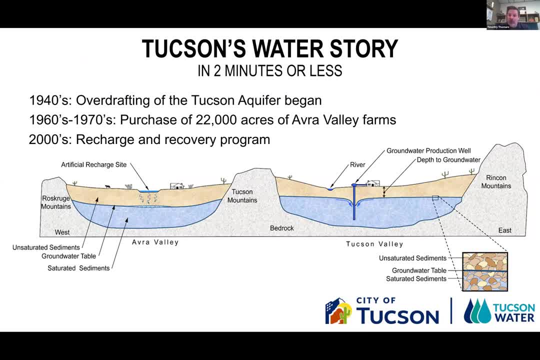 It's a very broad alluvial valley between mountain ranges on three sides, Sand and gravel and clay deposits inter-fingered, much like what you saw with Orange County, But a very productive aquifer over. we have productivity down below a thousand feet and it could actually go much deeper than. 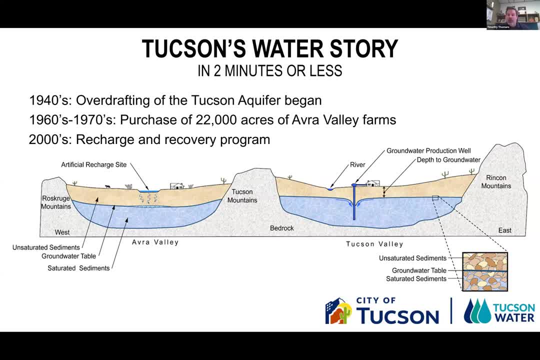 that The Santa Cruz River flows through that valley from south to north, But flow is a relative term because it does not flow very often, Although it used to be a perennial river. pre-development To the west of the Tucson Mountains is what we call the Avra Valley, which is an area where it was historically used for. 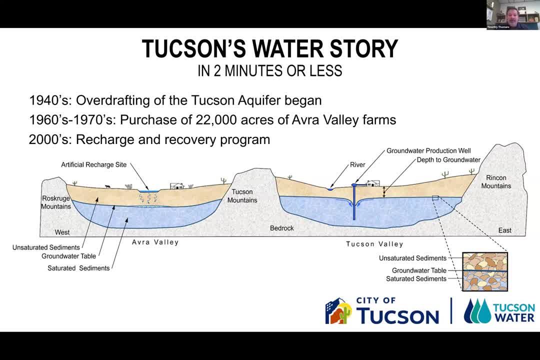 farming. A lot of cotton grow out in that area, But in the 1960s to 70s Tucson bought a lot of those farmlands, retired them for production to preserve the water for the future, And that's actually both been preserving of groundwater but also the location where much of our groundwater 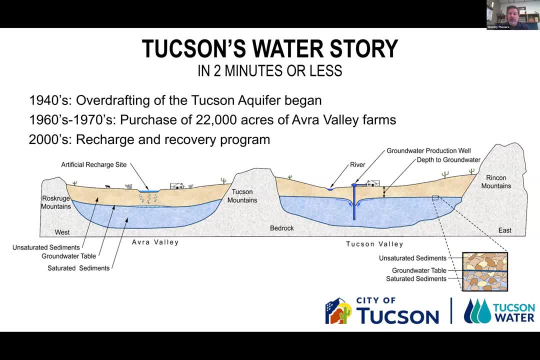 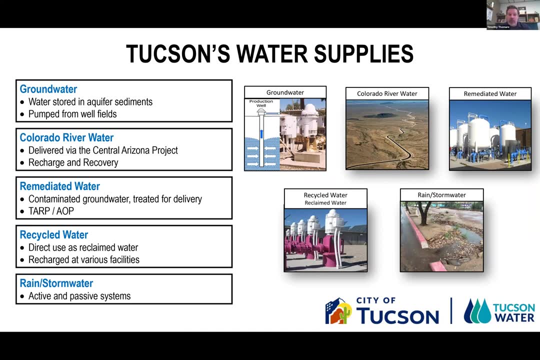 is being used to preserve the water. So we've been doing a lot of recharge and recovery efforts to undergo. So since the 2000s we've been doing significant recharge and recovery, although it began in the 80s for Tucson on the recycled water side. Our water supplies are diverse. We have our 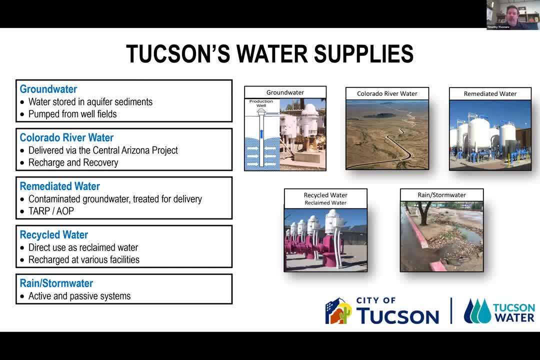 groundwater, which is our largest supply, but it's also our supply of last resort because we've over used it, We've abused it in the past. Our goal is to preserve it and enhance it for the future. So our water supplies are very diverse and we've extended it to the Central Arizona Project. 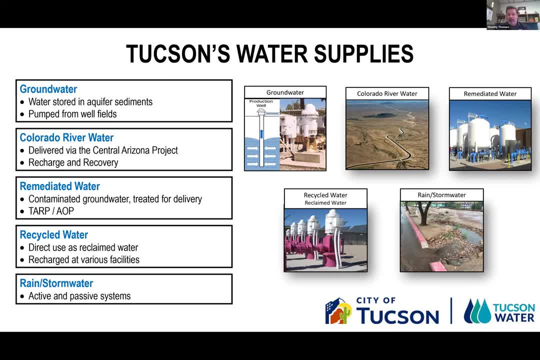 and that water comes into our customers' taps through our aquifer. We do recharge and recovery of that water. So we recharge it through constructed spreading victims- I'll talk more about that in a moment- And then we recover it through deep wells where it blends the 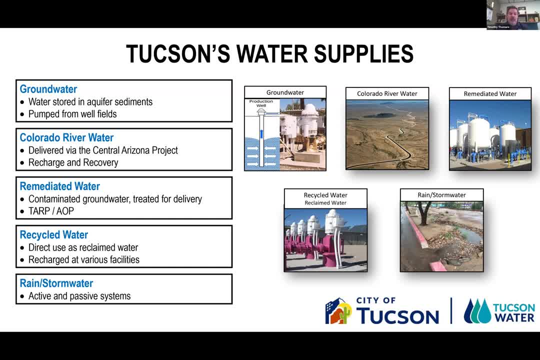 native groundwater and the Colorado River water that's been recharged And that's the product that we deliver to our customers: direct delivery through a surface water treatment plant. There's a book out about how not to do that. well, We also have generally pristine aquifers, relatively uncontaminated, but we do have a large 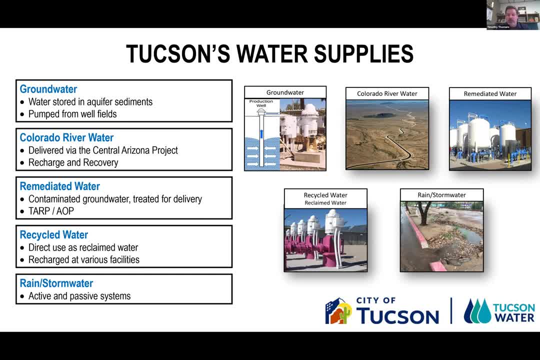 Superfund site associated with military operations in the area. So we do remediate some groundwater through an advanced oxidation plant. We do have recycled water. You often hear whether Tucson was first or Scottsdale was first. We disagree. It was a tie. We've been doing recycled water since the 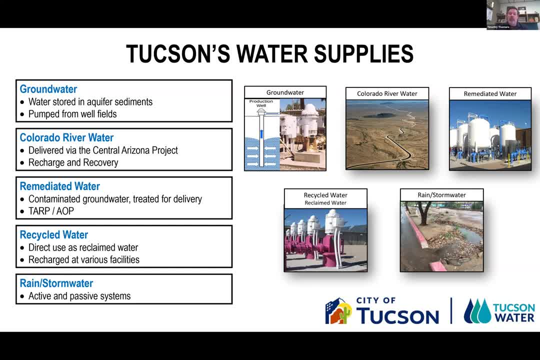 early 1980s. We do some direct through a purple pipe system for non-potable use, and then we do use the aquifer for storage for the future, And then we've begun to further exploit local rain and storm water. We don't get much of it, but what we do get is a significant amount that. 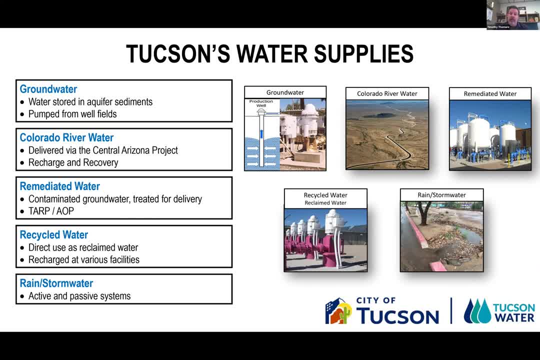 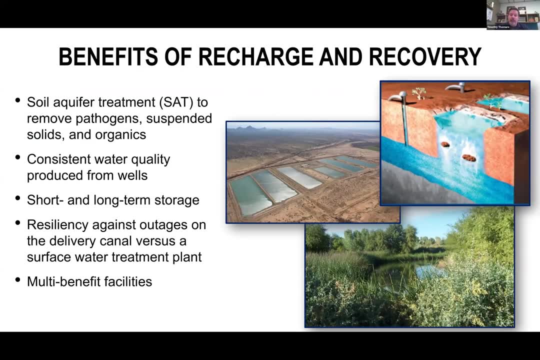 if captured, could both reduce the demand for our other water supply but also be used as part of our climate resiliency strategies in the form of augmenting tree canopy in Tucson. So we have a lot of efforts into the rain and storm water area For Tucson. some of the 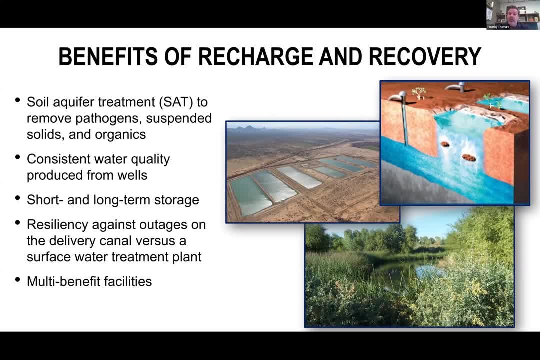 biggest benefits for recharge and recovery. beginning, our first recharge activities were with recycled water or municipal effluent. We found that at the time the regional wastewater provider was providing kind of a secondary resource for the water supply. So we've been doing a lot of. 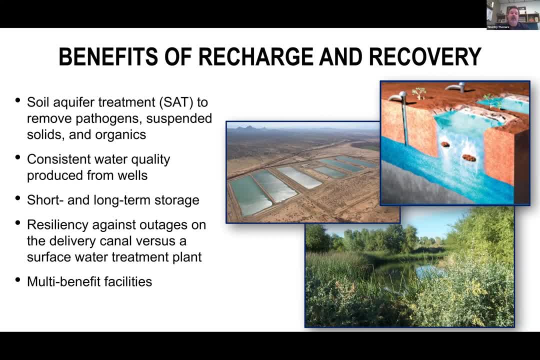 overhauling of the treatment sites that are in the hopes and dreams of replacing the ponds, and we've been doing very good work on that And we're really glad to have been able to do that And we're really glad to have the 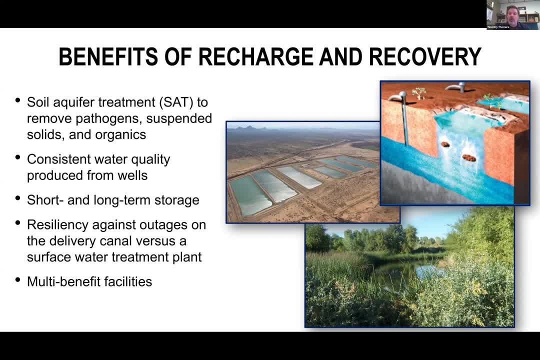 state of the art community to come to our hands and to have a very friendly message to people that they need to know, that they need to know about the water supply. We've been doing a lot of work that will help them to understand what they're considering. 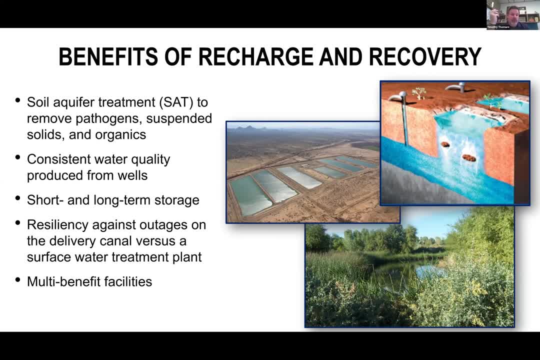 But this is in the early 1970s, in the early 1980s. that's actually when we started thinking a lot about it could go directly into the reclaimed water system. We find that both for the. we also find those benefits on the Colorado river side. 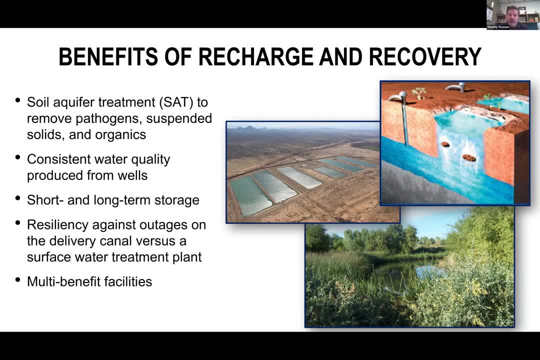 the aquifer treatment we do there and you can see the picture sort of in the middle of some of our large basins in Abra Valley from a different angle. We see the TOC removal. we see other stabilization of the water as it infiltrates through the aquifer and the Vadozone. 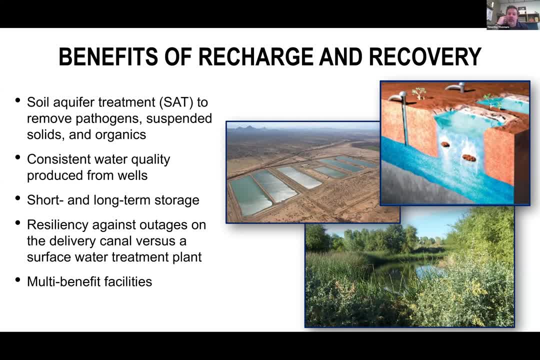 And we find that we can recover that water and actually deliver it directly into our system as a recovered water. We don't have to do any further treatment of that water, no additional filtration. all we do is disinfect and distribute And that water quality. 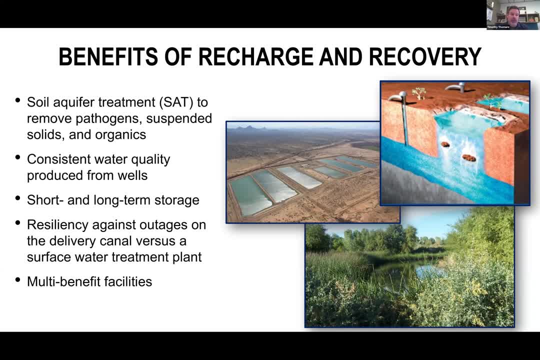 whether it's on the reclaimed water side or the potable side, using our Colorado river water, it's very consistent coming from those wells. So, unlike a surface water treatment plant that can have, when you're treating a river water you can have upsets in both how the plant performs. 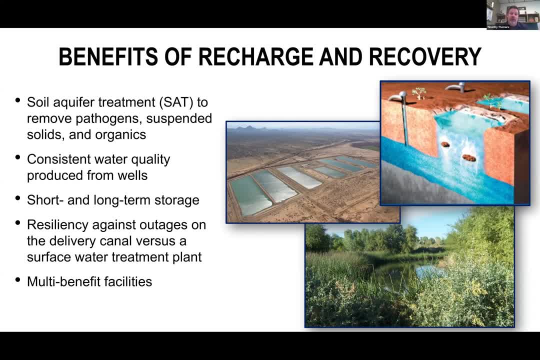 or failures of the plant, when you have, like, an algal bloom or something, come through the system. recharge buffers us from all of that. So we find that consistent water quality to be a major benefit. We use it for both short and long-term storage. 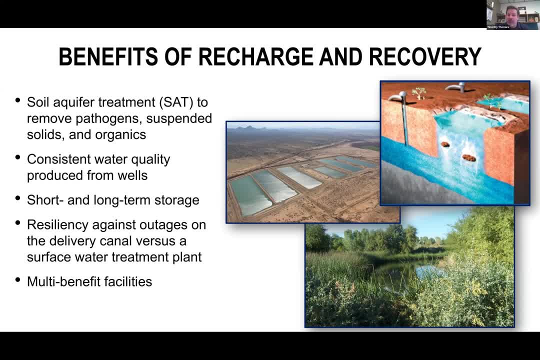 So we recharge it all and recover some of it on an annual basis to meet our annual needs, But then we have a net gain in water in the aquifer year over year, with both water supplies by recharging everything that we have a right to or the ability to acquire. 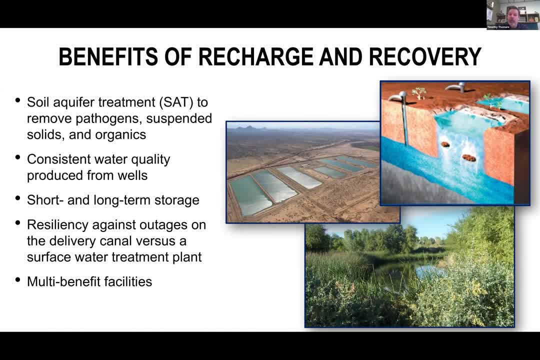 and then only using what we need on an annual basis. So we're net banking about a half a years of water supply every year in recent times. We do know that the Colorado river is undergoing multi-decadal drought- significant impacts from climate change. 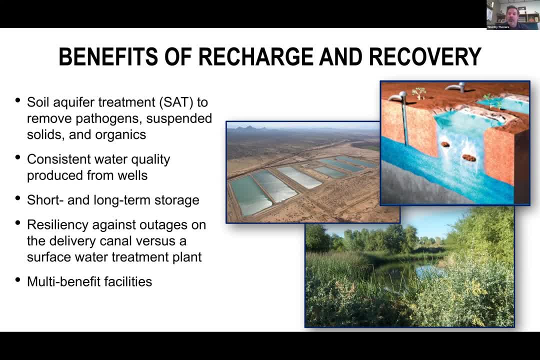 and entered its first shortage in 2022.. That has not yet affected Tucson because of our priority within the system, But we do know that we're banking water for a drier day. The use of managed aquifer recharge also gives us resiliency against outages. 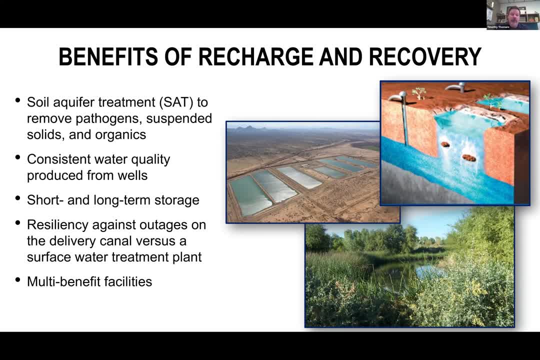 in our delivery canal versus a surface water treatment plant. If you're using a surface water treatment plant, you have to have water in the canal every day to extract, treat and deliver in order to have water for your customers When you have the aquifer between that source water. 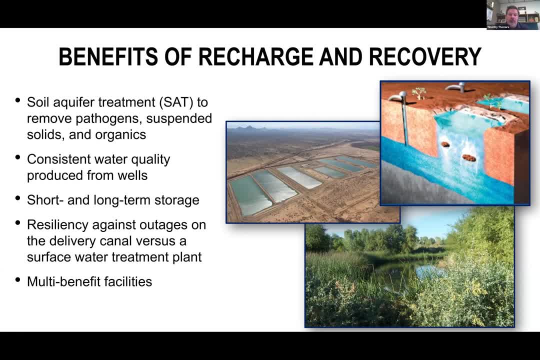 and that production. you can go months, if not years, of interruption on the delivery system and still meet the needs of your customers, Thank you. And then we've also emerged into recognizing that recharge facilities can be multi-benefit facilities. idol or right is a ear from our Sweetwater wetlands. 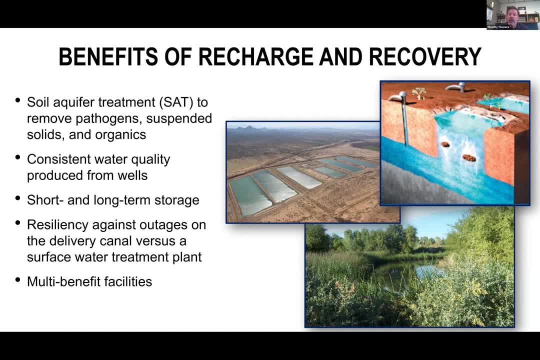 at our Sweetwater recharge facilities. We, when we first got into recharged, we were: fence everything off, make it square, make it boring. It's all about water into the ground. We've evolved into a more modern perspective on that. We're embracing the multiple benefits of recharge. 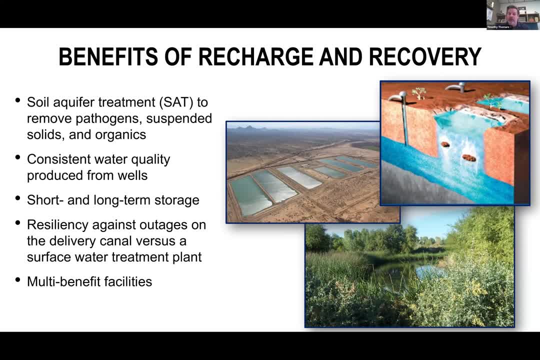 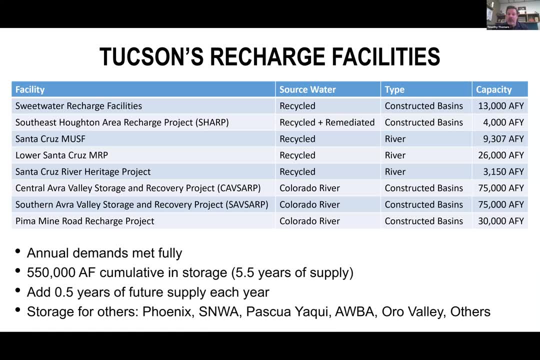 is where we are now and that invaluable present and practice that we deliver to our consumers و Just before you depart theacer- and into the future. so this is a quick snapshot of all of our facilities. we have a lot of them. we've been at it for a long time. we use both recycled water and colorado river water in our 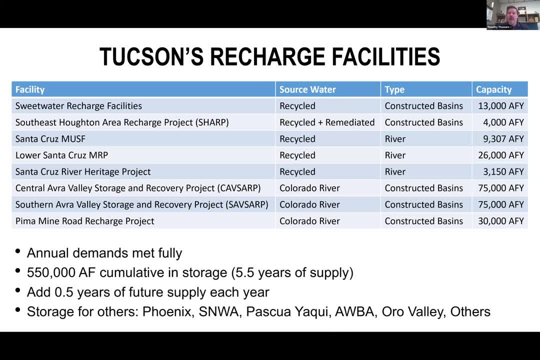 recharge facilities. in our case, everything is through either a constructed basin or the river itself and, as peter mock indicated earlier when he was telling the arizona story, when you use a native river channel you can, because our native river channels are usually dry but can introduce water into those channels and, through the permitting mechanisms, get credit for the. 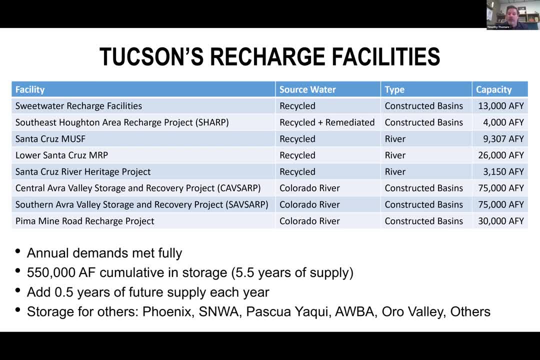 recharge that occurs. so we've actually been trailblazers on that and also expanded that to be multi-benefit facilities and moving that from more of the rural areas into the urban tucson. so i'll highlight the santa cruz river heritage project in a moment, but that's where we brought 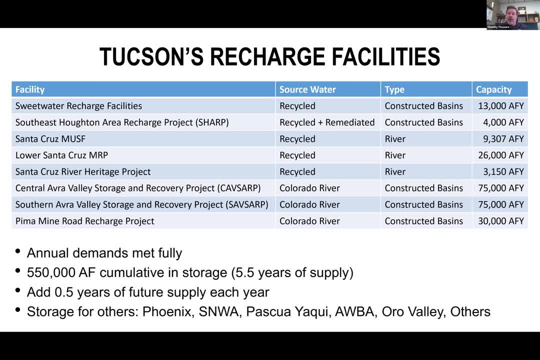 this multi-benefit in river recharge concept right into downtown tucson and also let a let a charge to change state law in order to get full credit for that recharge that we were creating. some of our facilities are crowd. they're large, some of them quite small, but through recharge all of our annual 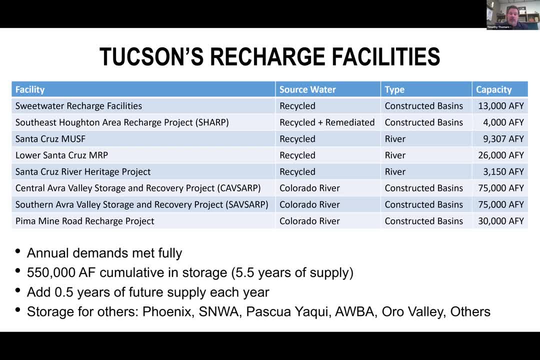 demands are met fully and in fact we, as i mentioned, we store about half a year of new supply every year for the future and and currently our current savings account in the aquifer, on top of all of the groundwater that exists, which is quite a bit and renewable or re annual recharge of natural groundwater. 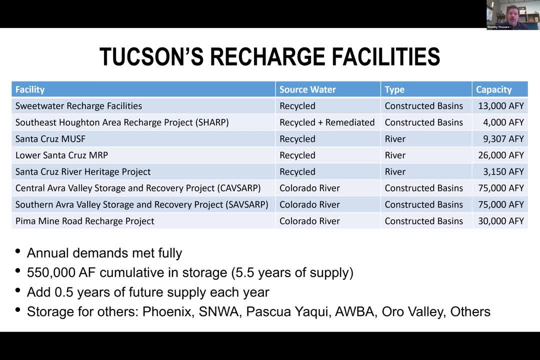 we have 550 000 acre feet of renewal water stored, which is about five and a half years of our supply. another part of our story is we store for others. this isn't just for tucson's put and take and storage. we store significant volumes of water here in tucson for the city of phoenix, for southern 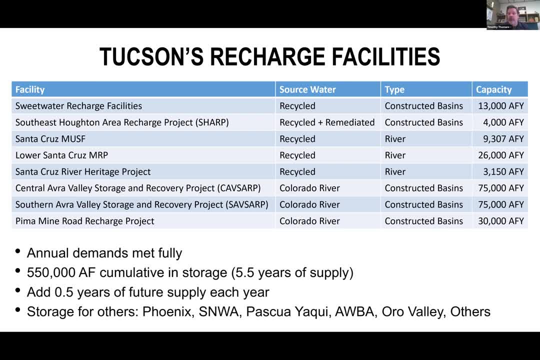 nevada water authority for the possibly yaki tribe, arizona water banking authority town of oro valley and many others where we actually are a savings account for several folks uh regionally, because of our approach to it, our plentiful aquifers and our success over time in managing 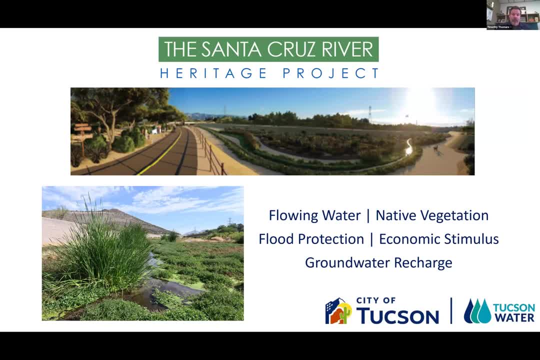 aquifer recharge. so just a moment on the santa cruz river heritage project and how we've evolved. you saw that air photo of the rectangular basins in the middle of the desert with concertina wire around it. we now have evolved to making it a part of the community and embracing water, not just for. 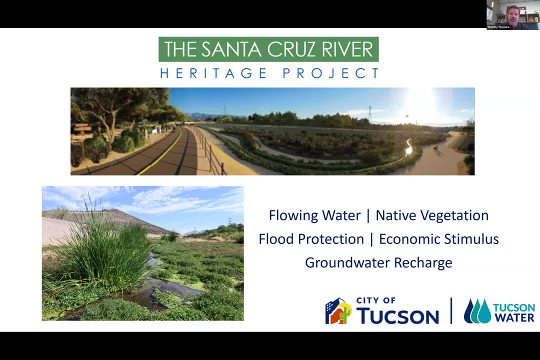 what it means to us on paper, or what it means to us for economic development or ability to meet customer demand, but what does it mean for the heart, soul and culture of tucson? the tucson began right in downtown, at the base of what we call a mountain, and that area has been continuously 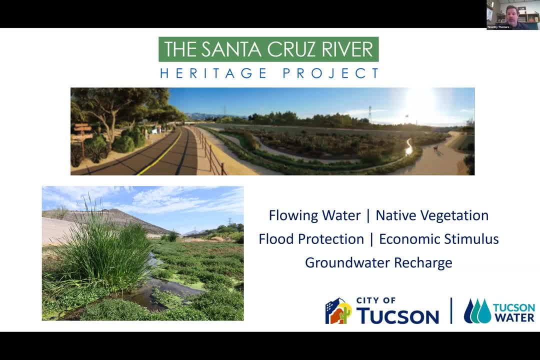 cultivated for over four thousand years, with, with um, tribal communities, native communities, and then the spanish conquistadores and now western european settlements. it's been continuously a story about water, but we had dried up that river since about the 1920s. the river no longer flowed. only during large rain events did it flow. well, we, using our 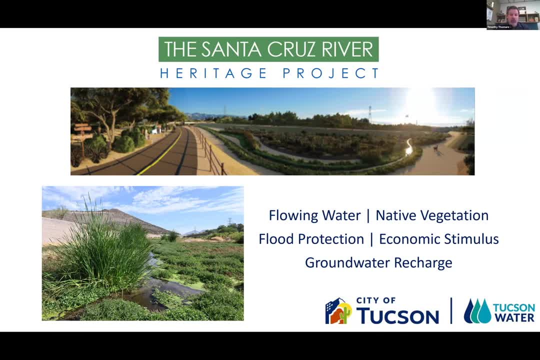 reclaimed water system and our management of of recharge. we introduced an outfall to the river river all the way to the right, uh upstream of downtown and you and you can see the. the ribbon picture is sort of a depiction of what our vision of what that area would look like in the future. 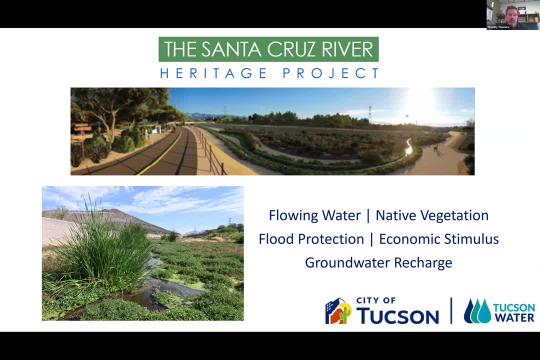 and the lower left is is a picture of how it looks after how it looked. this was only after about uh two to three months of charge has been continuous for now, going on three years. june will be three years. we have the benefits of flowing water in downtown tucson. we've been uh restoring uh native. 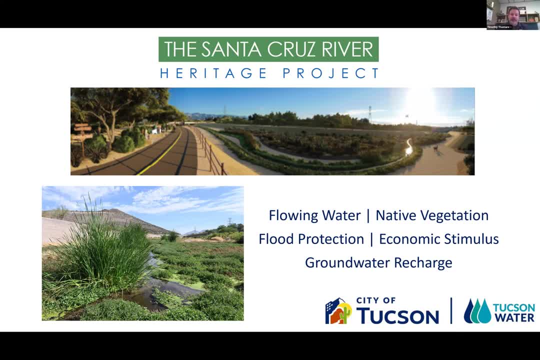 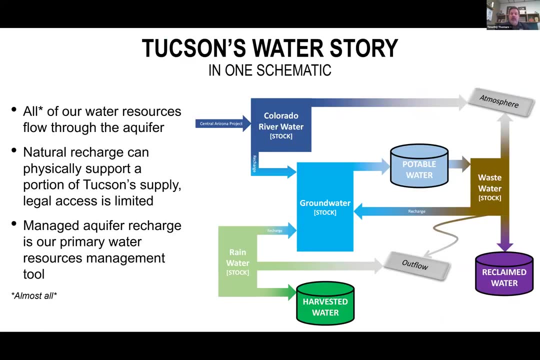 important area for wildlife to move throughout the community. we've embraced and protected flood protection, we've seen economic stimulus from having this flowing stretch of the river and of course, we've seen the impacts of groundwater recharge. so i'll conclude with my tucson's water story in one schematic, all with an asterisk, of our water. 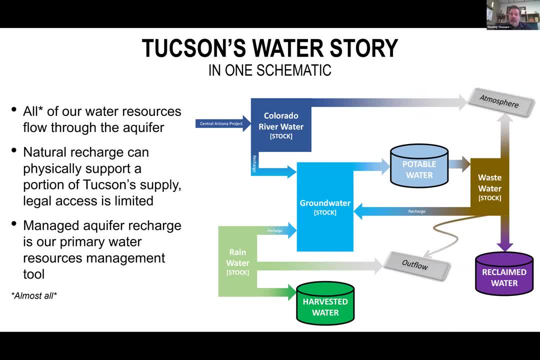 resources flow through the aquifer. this is a stock and flow diagram of our water supply and you can see the in the light blue, the groundwater in the middle. that's our largest stock of ground of water supply and you can see that most arrows flow into it, our colorado river water coming through the. 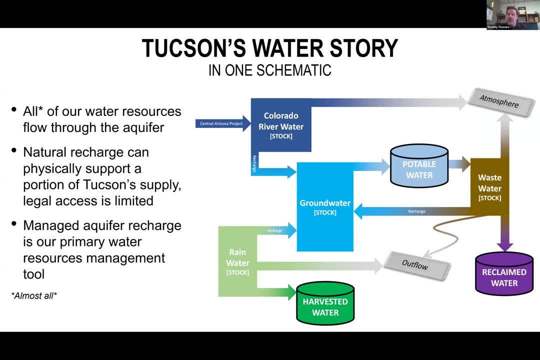 central arizona project. a bit is lost to evaporation, either on its way to us or in the recharge basins or after the fact. my light's about to go out, but the but the majority of it- 98 or better of it- goes into the groundwater and joins that stock for use for potable water and our 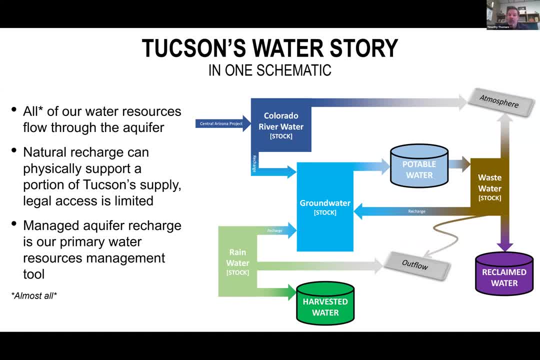 customers, and that's where the the vast majority of their water comes from. you can see that rain water joins the groundwater through natural and mountain front recharge, although we do have some that we're harvesting directly before it reaches the aquifer and using, and then we do have a small amount. 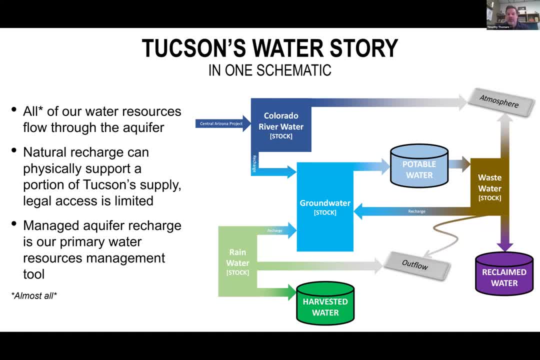 that flows out of the community. for the most part, tucson's a closed basin where what what happens in tucson stays in tucson, but during very large rain events we will have a pulse of water that flows out toward the gila river and then on the right. you can see that. 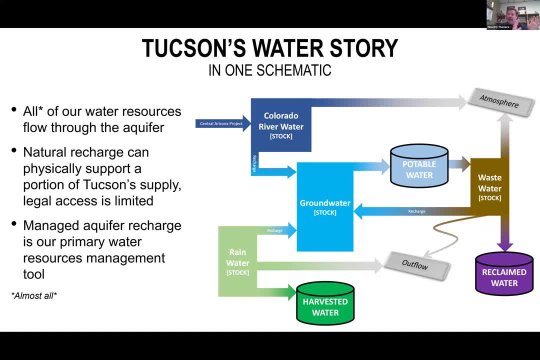 between around a single faction that we've found water, install water coolest, infill, plan water pump, boring water, hot air pump must buy earth and then solidified- per Bryant it stone. he does become potable water, regardless of how it became groundwater. we introduce it, it becomes potable water. we have a wastewater return flow to our groundwater or to 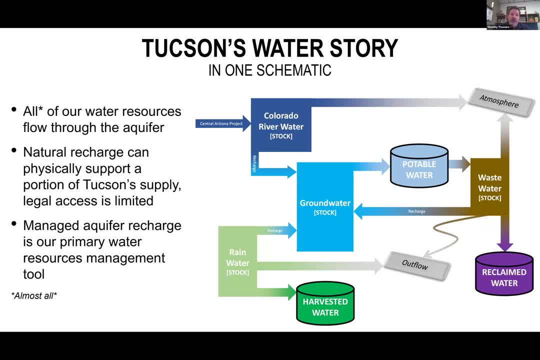 our users at the customer site. so while natural recharge can physically support a portion of tucson supply, our legal access to natural recharge is very limited, whereas manifold managed aquifer recharge is our primary water resource management management tool, andcilнее in Tucson. With that I thank you for your time and I think we're ready to move into a question. 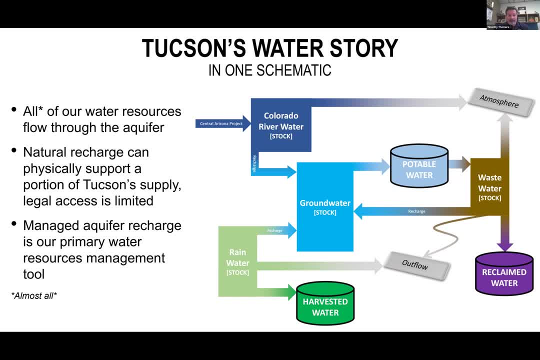 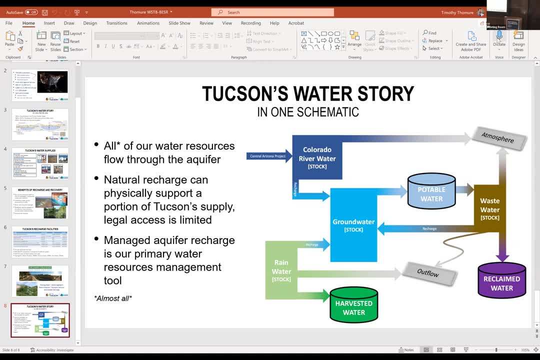 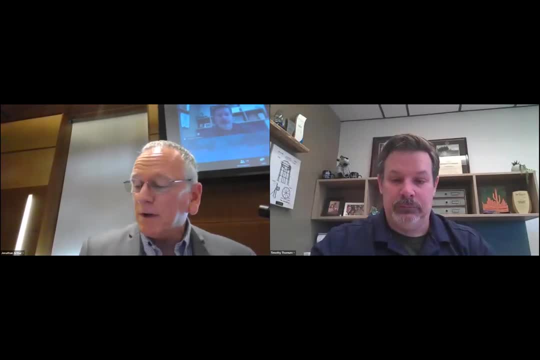 and answer session. Thank you, Tim. thank you very much. Fascinating story and I truly appreciated yet another example of geoheritage being woven into presentations as well. Now we're moving into our Q&A, which we will wrap up at two o'clock. Is that correct? Yes, So at this point the floor. 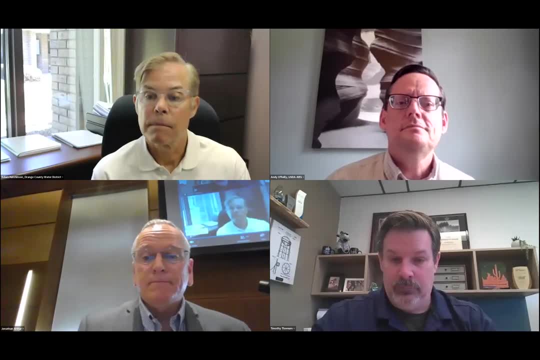 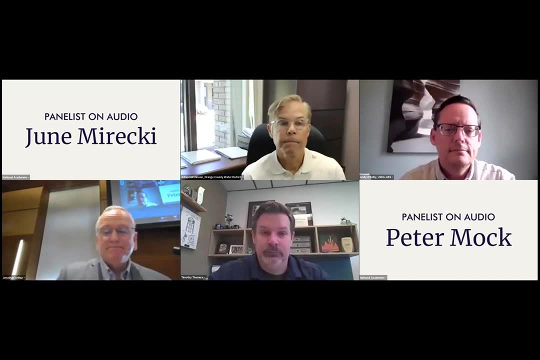 is open for questions for any of our speakers, Nusha. Thank you so much, everyone. This was fantastic. I have three questions. One is for Charles. I'm wondering what happens to the brine after what you do, and how does that? 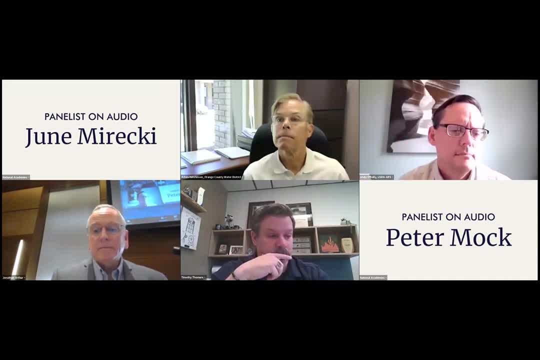 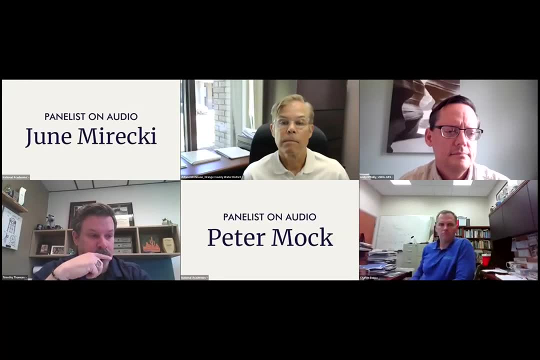 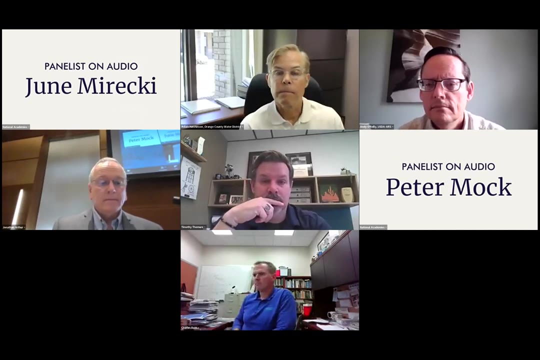 impact your outflows to the Chesapeake Bay. And if you covered that and I missed it, I apologize. And then I guess the second question is for Tim, and I wonder: how do you differentiate between natural and managed aquifer water? Is that through your accounting system or do you have a different way? since you touched on the legal rights, 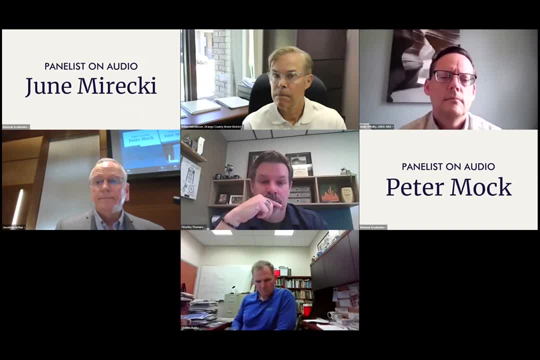 And, yeah, I actually go with those two and then, if there's time, I'll ask more. This is Charles, I'll go first. So with the advanced treatment approach we've taken, there is no brine return to the back, to the wastewater plan or anywhere, right? so the ozone biofiltration GAC approach produces some filter backwash waste that can give us a lot of brine. And with that I'm happy to move on to the next question. I think we have two minutes. Thanks everyone for your time. Thank you. 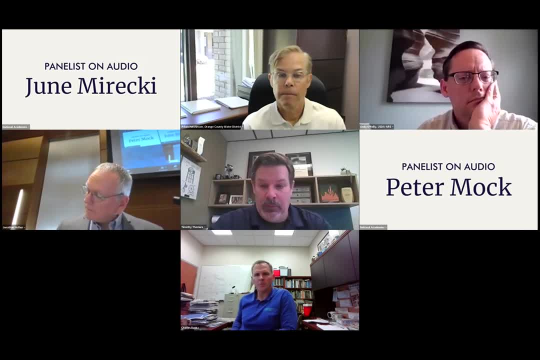 go back to the wastewater plant, but since there's no reverse osmosis, there is no brine, which is a nice benefit. Is that why you chose that approach? I mean, that's one of the reasons. Like I said, the big reason is that the TDS in the aquifer 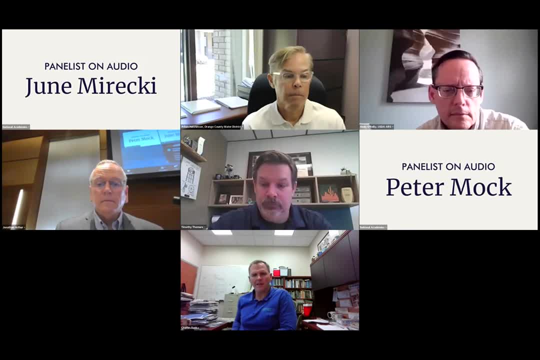 is already quite high and there's the presence of swelling clays, and we have local experience with recharge wells with low TDS water. that failed immediately. So right now the impression is that we can't recharge into that aquifer with real low TDS water sustainably, So we need that. 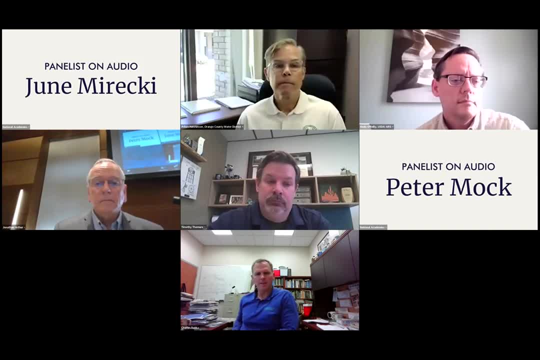 salinity for the aquifer. Of course, the treatment approach that I identified is also less expensive, both on a capital and an operational basis. It recovers nearly 100% of the water that's applied to the aquifer. So we can't recharge into that aquifer with real low TDS water. 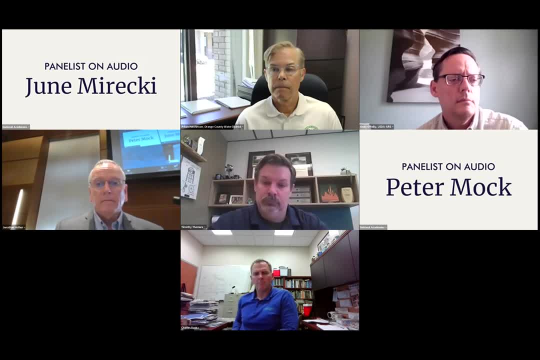 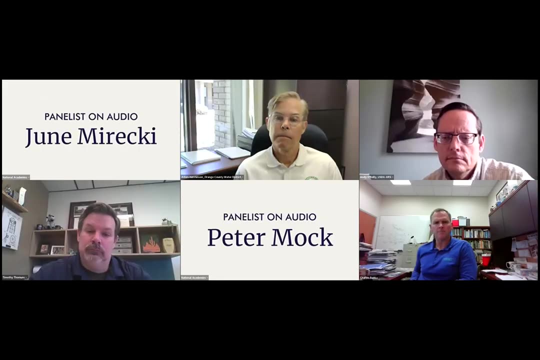 Because there is no brine return. But it's really important, of course, then to get comfortable with a non-membrane-based advanced treatment approach, And that's an active topic of a lot of interest around the US and around the world right now. Thank you, 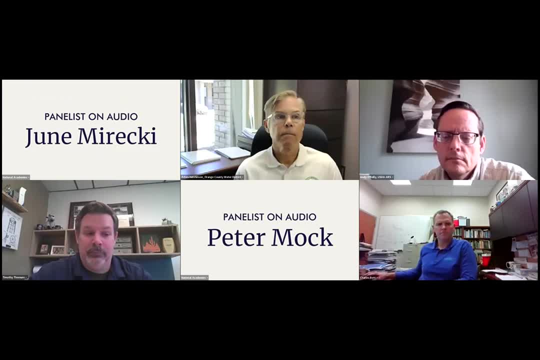 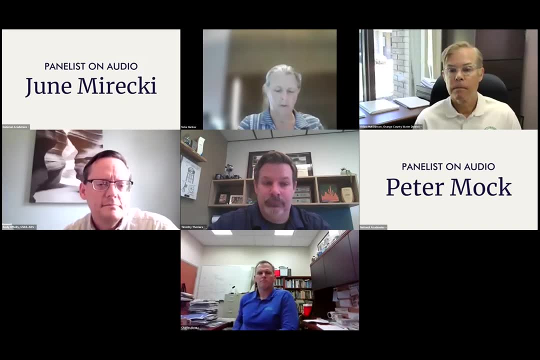 Okay, We'll go over to Nelia Dunbar. Yeah, I have a question for Tim. Okay, Tim, you mentioned that as part of your more modern approach to ASR in the Tucson area, that this helped you lead a charge to change state law, And I'm curious to hear a little. 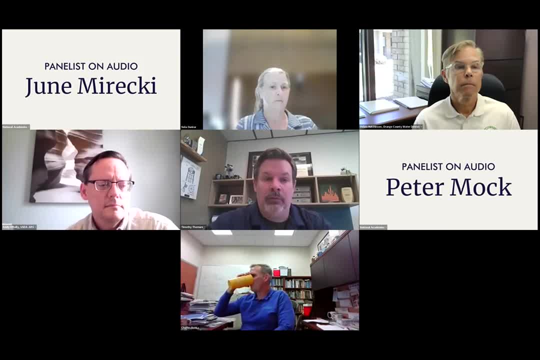 bit more about that process. Thank you for the question. So in Arizona we use the term managed aquifer recharge a little bit differently than we are in this room. When you're using a natural stream bed without modification, we call that managed recharge. 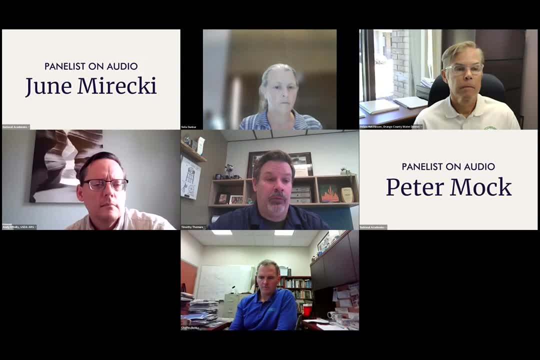 And the institutional framework first created in the 1980s and carrying forward through some revisions only allowed you to gain 50% credit for that water you would recharge. So you can physically show you're recharging 98% or 95% of that water after you account for evapotranspiration. But you would 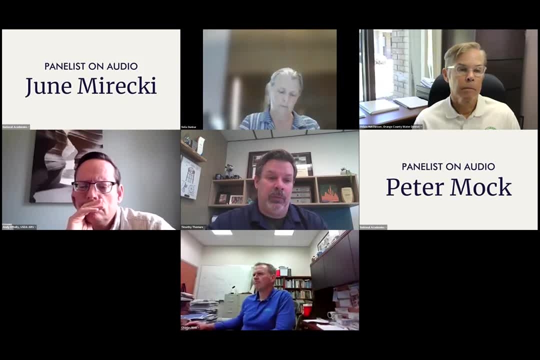 only get credit for 50% of the recharge And the other 50% is what they call they cut to the aquifer, And so that was a disincentive from using a river to do recharge when you could take that same supply and 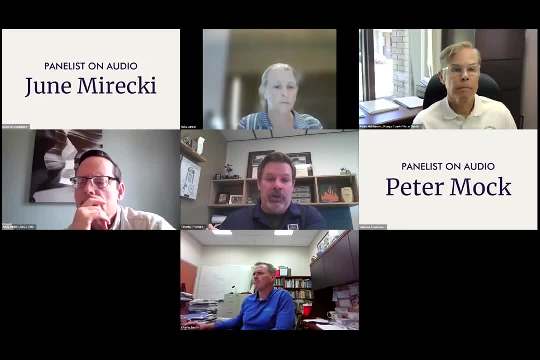 construct a basin outside of the river basin, off channel, and you could get 95% or 100% credit. So we actually got that changed in 2019.. It's one of those stories when we finally achieved leverage, The drought contingency plan, which is a Colorado River thing, needed to be passed, needed to have. 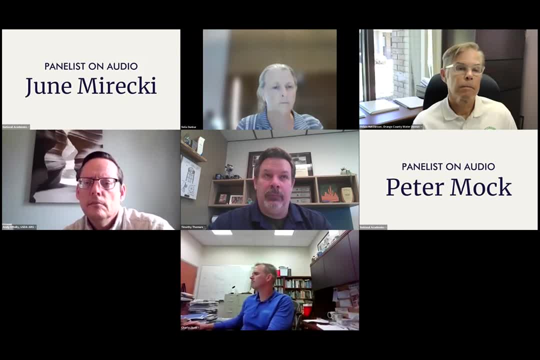 a broad coalition of stakeholders And long story short. in order to satisfy some of the concerns of agricultural users in central Arizona, Tucson was willing to commit to doing some things over a short period to shore up water supply for central Arizona agriculture if we got three or four. 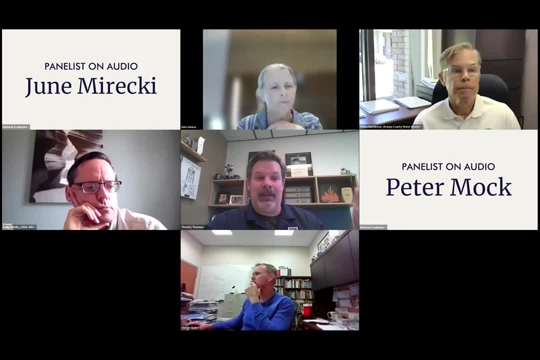 changes to the code that they made sense in 1980, but they didn't make sense in 2019.. So we got through that drought contingency plan legislation. we got the cut to the aquifer reduced for managed recharge- what we call managed recharge, riverbed recharge. 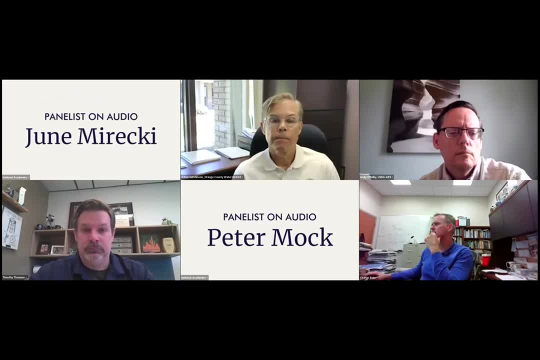 Thank you Great. Okay, we have a question from Rabia and then we'll go to David Sedlak. Hi everybody, This is Rabia Chaudhry. I'm from the EPA and I just want to caveat. 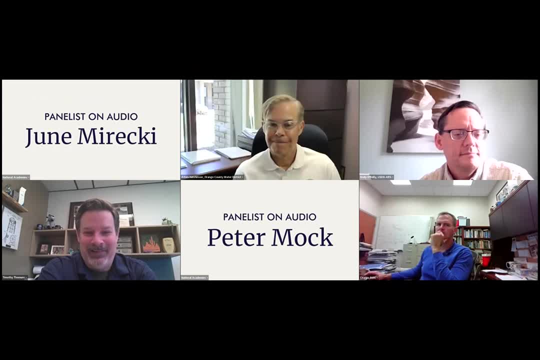 non-regulatory part of EPA. So please don't get scared when I ask this question. So I have two questions, one for Charles and one for Tim. Charles- really curious, you know, Hampton Roads SWIFT project is really revolutionary in the way you've managed your. 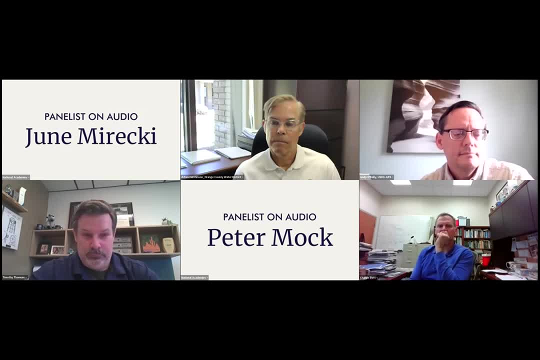 specific challenges around. you know outfall to the Chesapeake and the very strict TMDL requirements in that basin. I'm just wondering: have you had any conversations with other your peers? you know other wastewater treatment facilities up and down the Chesapeake. 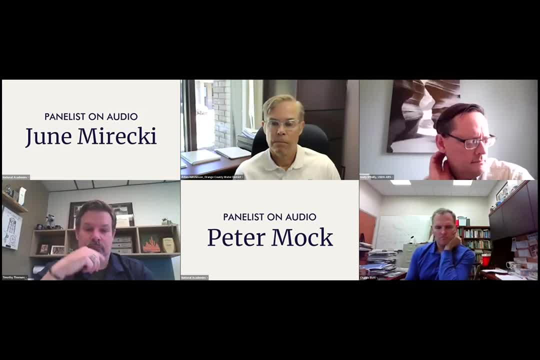 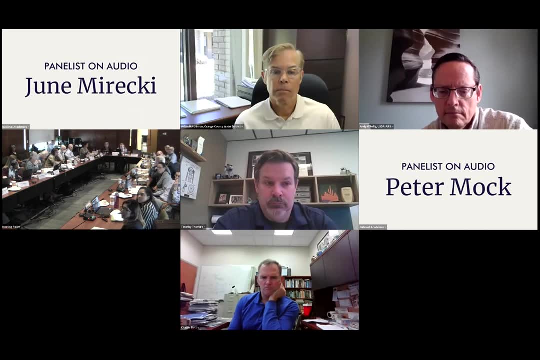 and how they're managing their discharges and whether they're thinking about approaches like yours and using MAR, because they're probably dealing with very similar challenges. that kind of drove you to do the approaches you've taken at SWIFT. Yeah, absolutely. 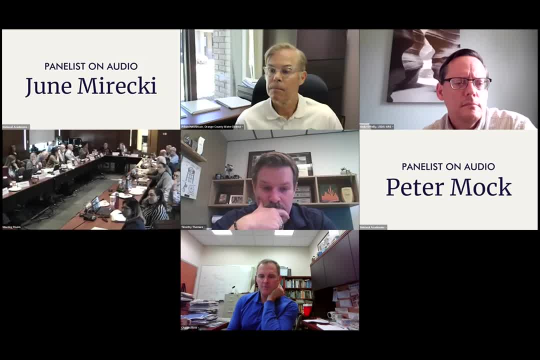 So we've had been a lot of conversation with Anne Arundel County in Maryland that's interested in a very similar approach. right now It's actually a little different, but similar technologies, similar aquifer system- not exactly the same. So yeah, I think there are some others interested. 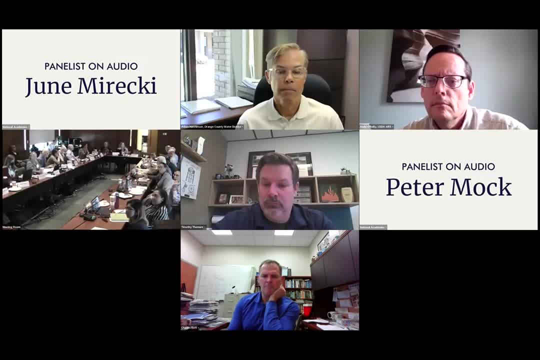 on the East Coast and, yeah, I can answer Absolutely. yeah, Thank you so much, and mostly I was asking this because we heard about a number of different drivers today for MAR, for water reuse, and this is a really interesting regulatory driver that. 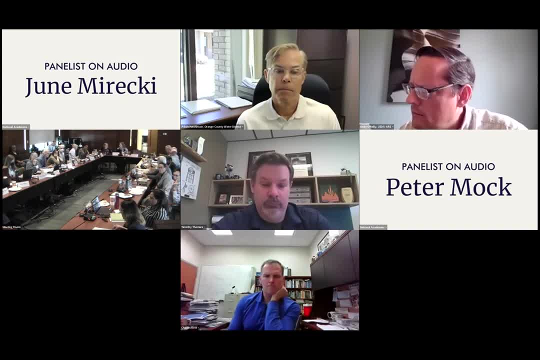 is pushing water reuse and MAR in a direction that we hadn't expected. And the other question I have is for Tim: Could you tell a little bit, just for information, what regulatory approaches are? you know you've mentioned credits in Arizona and we know there's, of course there's no water. 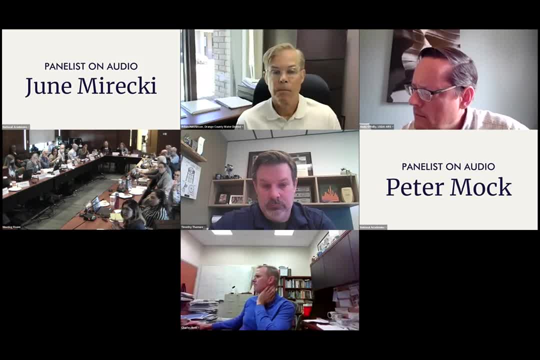 reuse regulations at the federal level, but there's no water reuse regulations at the federal level and as far as kind of in our understanding there's nothing really at the like in law necessarily at the Arizona state level. So could you help us understand a little bit about? 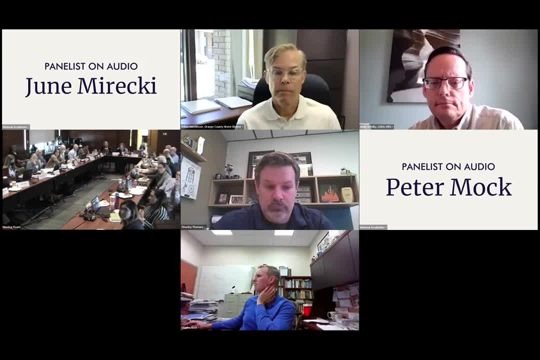 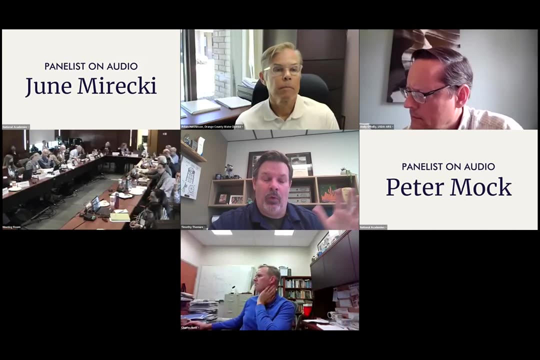 what levers and permitting systems you're using that kind of interface with your project, Thank you. Thank you for the question. So water is regulated in Arizona through two main agencies: the Arizona Department of Water Resources, which really focuses more on quality and environmental quality, and the Arizona Department of Environmental Quality. 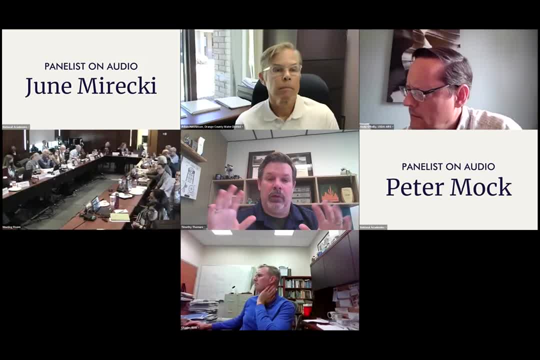 which focuses on quality and the environment, And there are. there is water code, there are things in Arizona's administrative code, but much of it- and some things- that becomes very difficult to change because now you have to have a legislative act to change it, but much of it flows through the 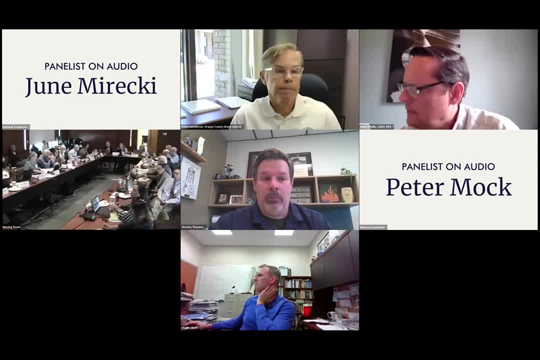 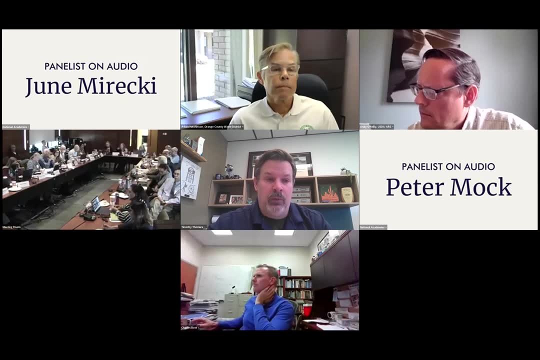 regulatory programs. So for any of our recharge projects there's a number of permits we have. If it's a recycled water side of the equation, we have to have what we call an aquifer protection permit which is more focused on the water quality side of protecting the groundwater. 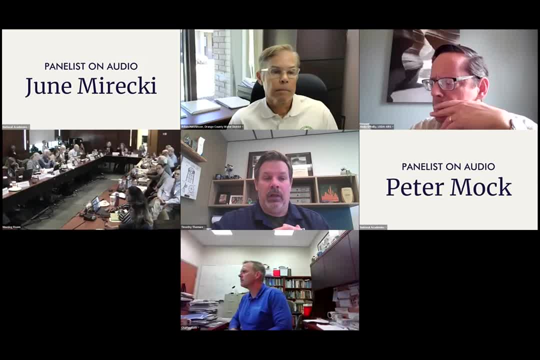 And then we have a facility permit which has all the regulations about how you operate the facility. Then we have storage permits and recovery permits. But all of that is kind of interwoven underneath the 1980 Groundwater Management Act, which really was the seminal. 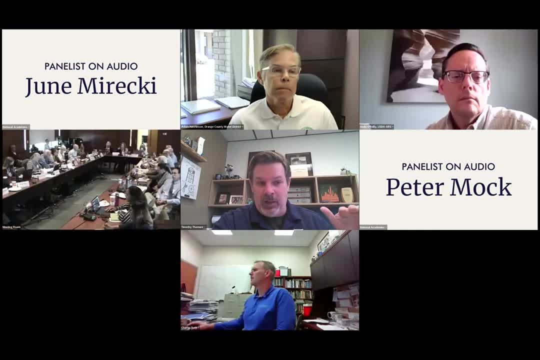 to where Arizona broadly moved from unsustainable to sustainable groundwater use. It's still on our pathway to coming out of that, but we had significant water level declines. Action needed to happen in order to change that trajectory. So born out of the Groundwater Management Act. 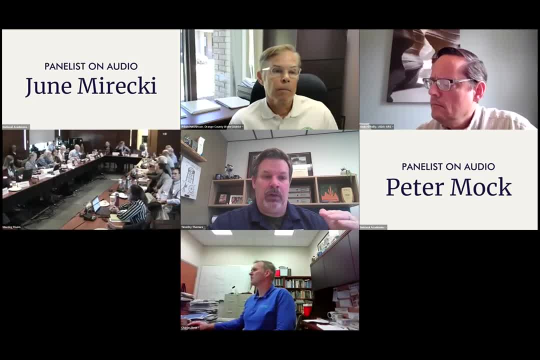 we have an Assured Water Supply Program, where all new development in the urban areas has to show a hundred-year assured water supply. Aquifer recharge is one mechanism by which we do that. So it's really a close relationship with the state and their regulatory authority. 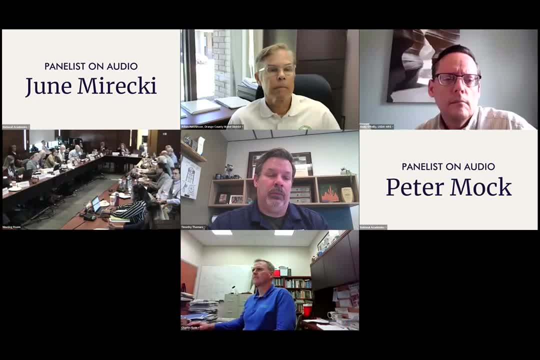 that leads to what Tucson does and others do with aquifer recharge. Hopefully that answered your question. If there's anything specific, let me know. No, that was great. Thank you, And to David: Yeah. So thank you everyone for some great presentations this morning. I'm sorry I couldn't. 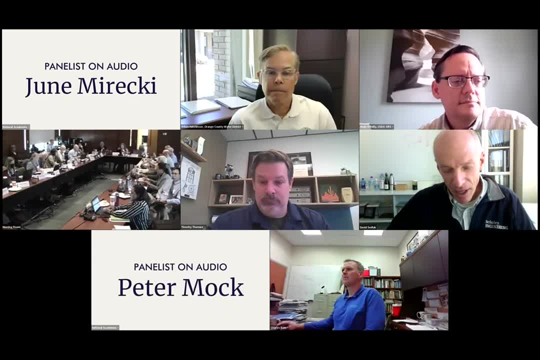 be there in person to engage with you. I have a more general question to everyone. except for people like Charles who are on the coast and discharging the ocean, This groundwater-centric view of managed aquifer recharge feels a little like a free lunch, That is, these flows that you're putting into the ground would have. 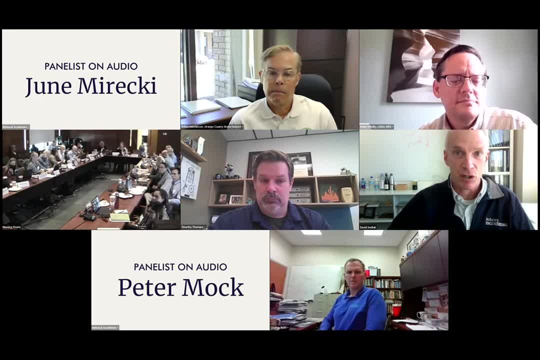 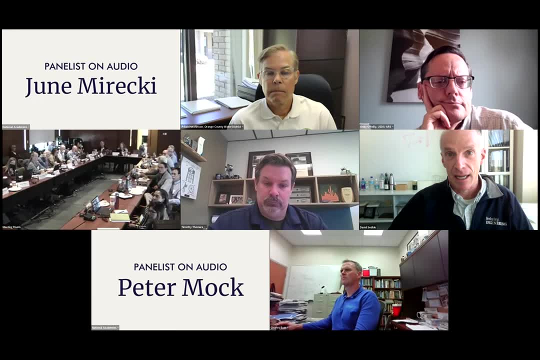 otherwise been base flow in a downstream section and recharged in another section of aquifer. They might have been environmental flows with the hydrology needed to maintain habitat for certain kinds of species, and they might have been someone else's water. So I'm kind of curious if there are examples from the presentations this morning about when the use 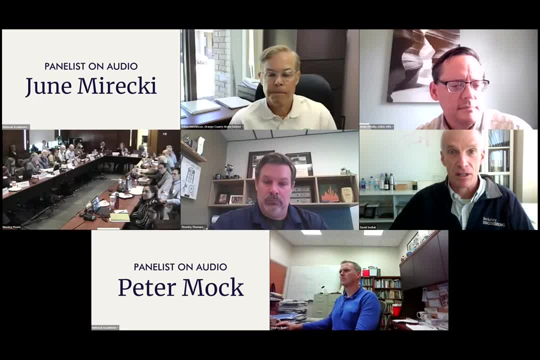 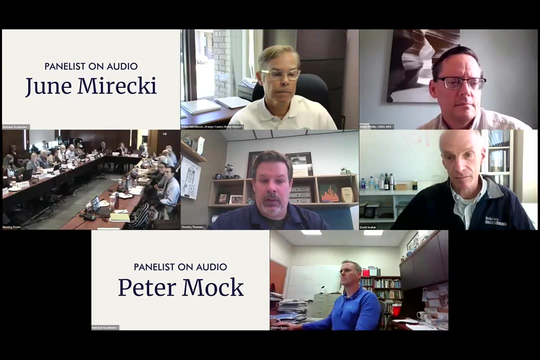 of managed aquifer recharge is restricted because those flows are not going directly to the ocean and are needed somewhere downstream for either ecological purposes or for water supply. I'm happy to dive in a little bit. Good to see you, David. So at least in Arizona there's not. 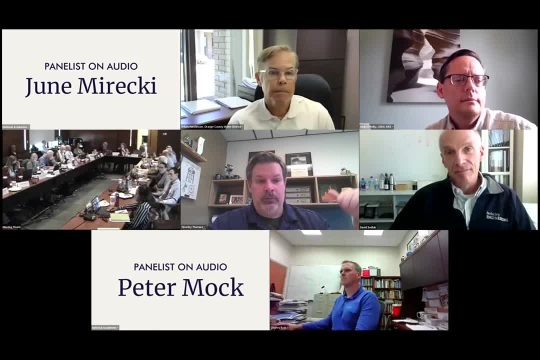 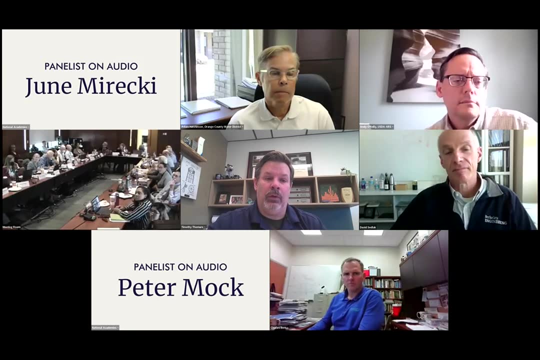 in at least historic time, not a connective river system that moves water from basin to basin. We do have subflow or underground flow from groundwater basin to groundwater basin, But where managed aquifer recharge comes in, it's almost always, if not always, a supply that you're either importing. 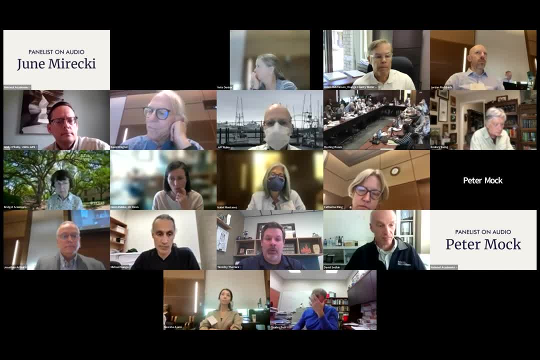 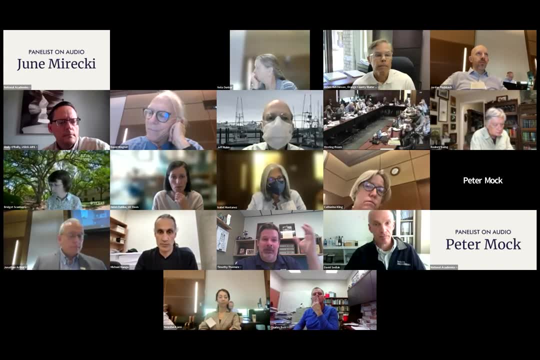 or you're taking out of the system and bringing it to the river. So it's only there because you brought it there. Colorado River Water Supply, So it's not, you could argue, downstream in the Colorado River. you're taking it out of that system. 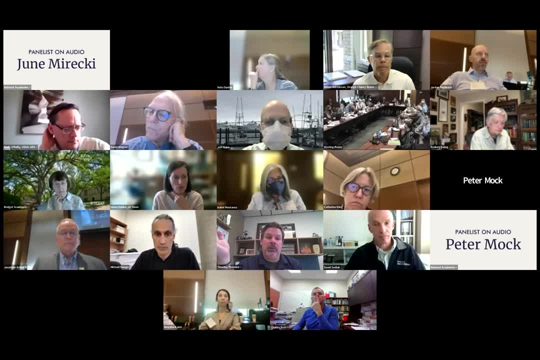 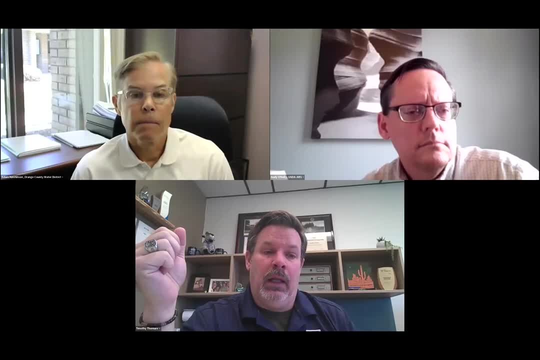 and bringing it to Arizona. But that's all part of that allocation scheme. On the wastewater side, we do have a complex ownership of that wastewater once it's been created And typically the whoever treats the wastewater owns the wastewater in Tucson. 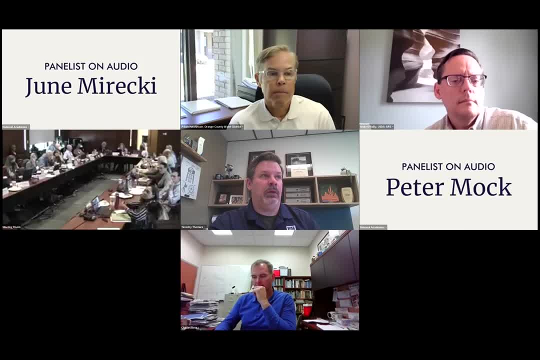 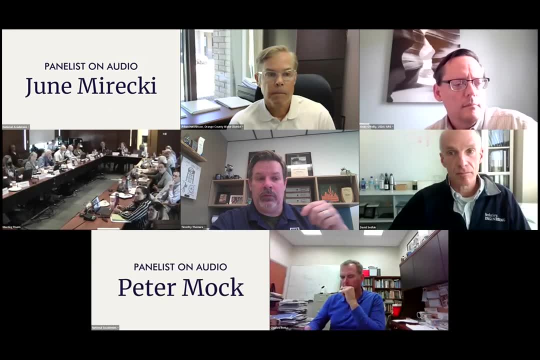 it's complicated by some IGAs. we have because actually we retain the ownership, But in our case we have some flow for environmental flows in certain segments of the river where it's been historically flowing as an outflow of a wastewater treatment plant. So 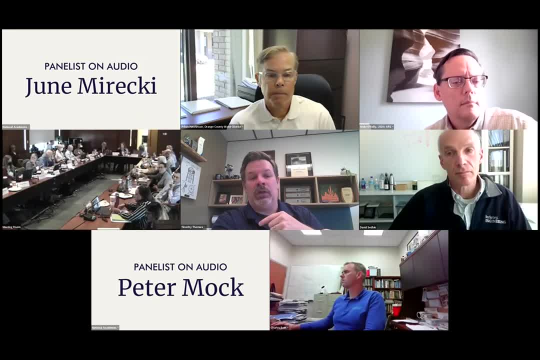 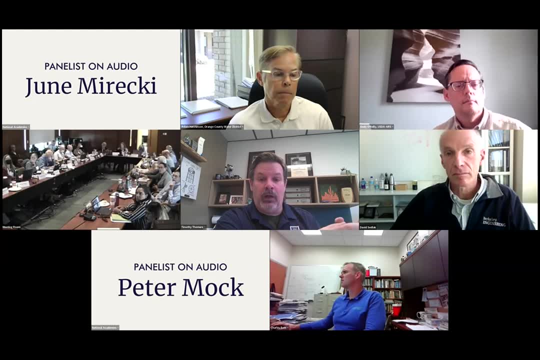 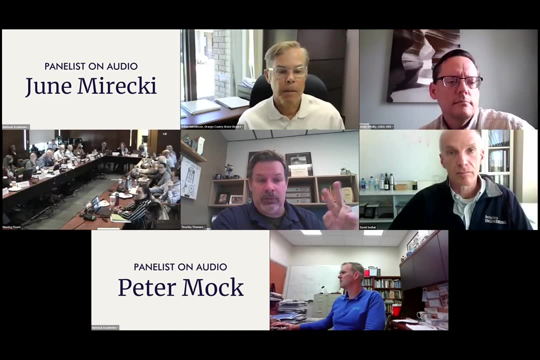 we've reestablished our riparian habitat And that change to state law was vital to remove that disincentive from us from taking it out of the river, Because otherwise your incentive was: take it out of the river because I can use it or store it, But if I left it in the river I lost. 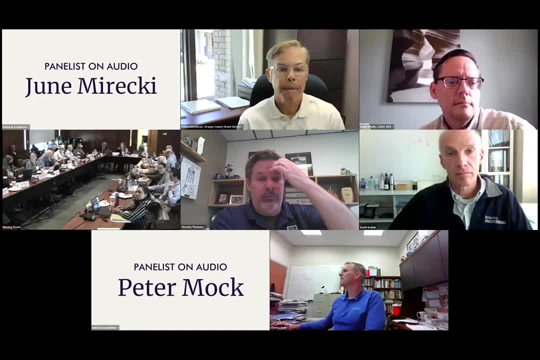 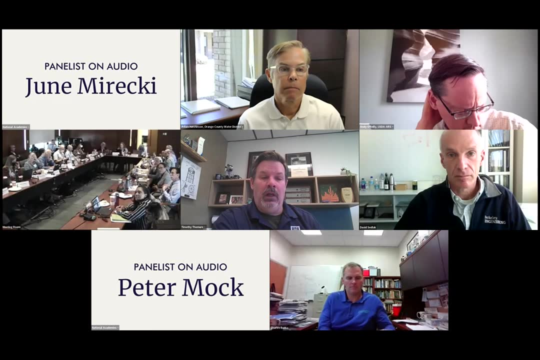 it. Now we've changed that, So now you can preserve that. And the other is that effluent becomes an appropriable surface water if you lose control of it once it hits the river system. So we actually in our managed recharge facilities when there's downstream appropriators. 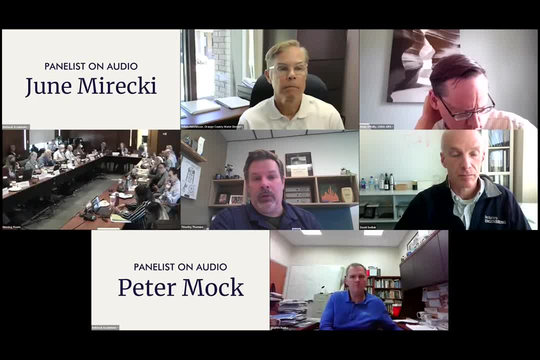 we actually account for that in our crediting and our use of that water in our facilities And we're even- you know, we're actually about to record that right now And we've done that over the next several years. Now I don't know if that's. 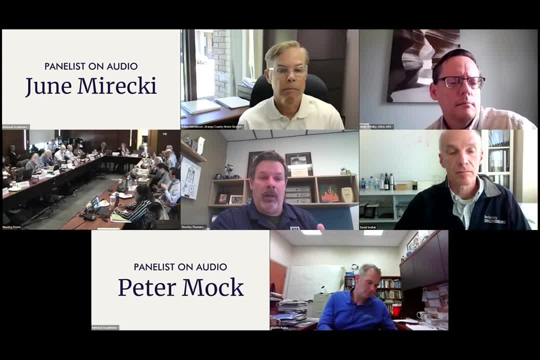 the reason why it's been so difficult. but if we're not enough to – even if we can get 100 ito that water in one place, which of course that's the way it can run, If it were able to get around the surface by a small flow rate, then we would be able to carry that water out. 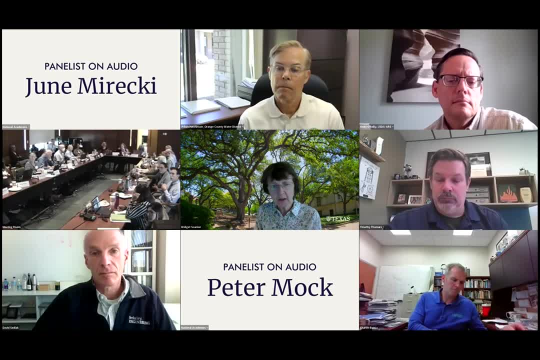 in our facilities and we would be able to continue the flow of that water to a larger enterprise, And so in our managed recharge facilities we're able to carry that water out, And so we've had some really, really good results in our studies over the years. 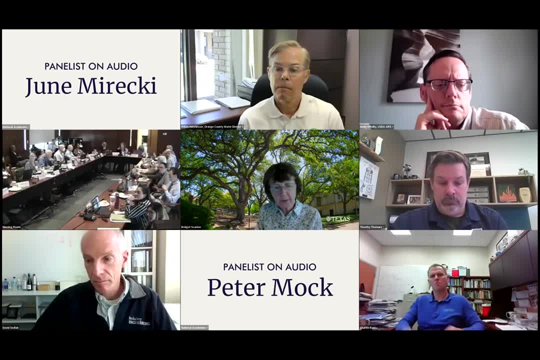 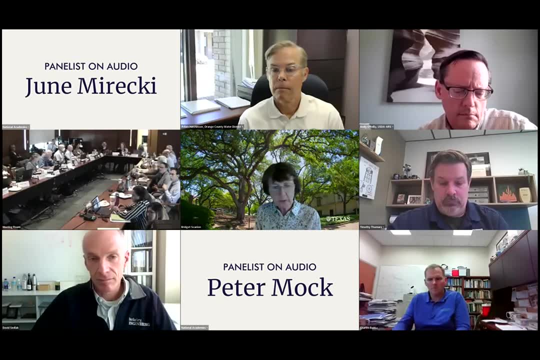 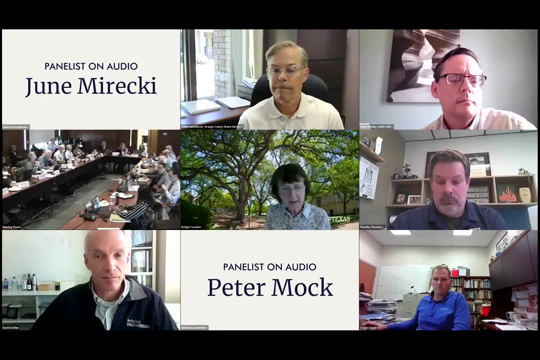 Thank you, David. We're excited to give our panelists a chance to comment on this flood flows they could capture- We did similar work in Texas and greater than the 95th percentile and we could capture maybe in the state And it didn't impact other water rights And then 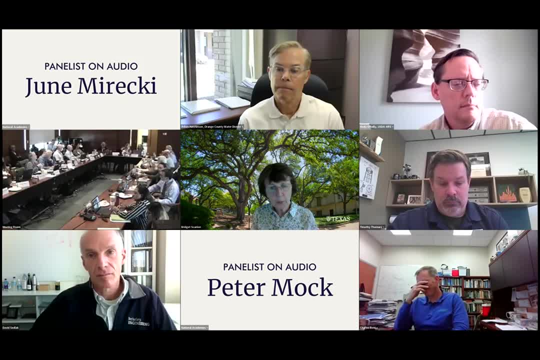 where there were detailed in-stream flows studies done, we would have to reduce what we could capture by about 30 percent and allow pulses through and meet different requirements for environmental flows. But it still suggested that there was a lot of water. but you can't. 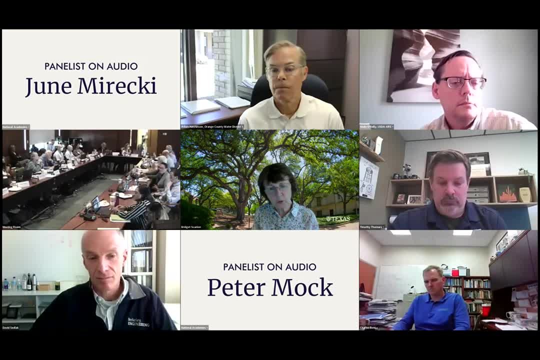 take it. I mean, it was there for several days and storing it and then getting it into an aqua takes time. So there are a lot of logistics that need to be managed to make it happen. But we did look at some of those aspects and I think possibly Helen did also. 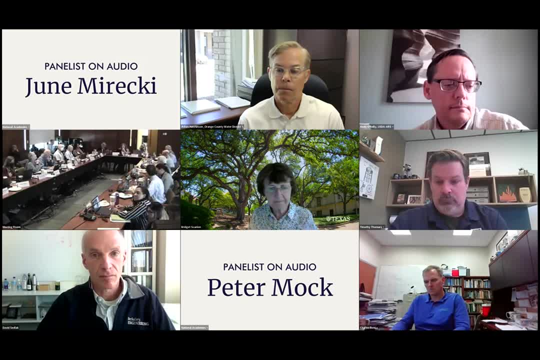 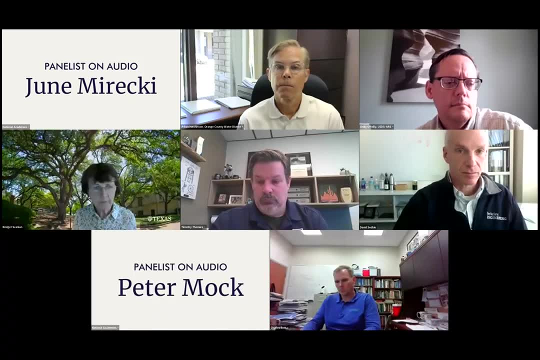 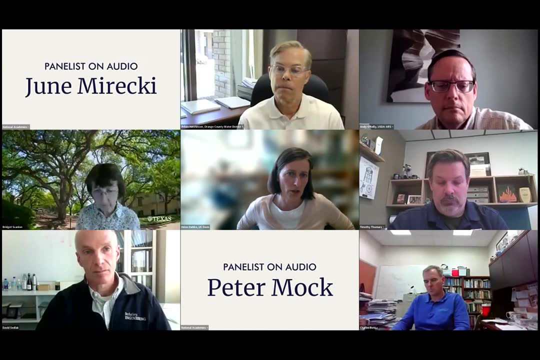 with her students. You did that analysis. Yeah, I can. I can add: We looked into diverting flood flows above the 90th percentile and looking into the outflows into the San Joaquin Sacramento Delta and at every point when we 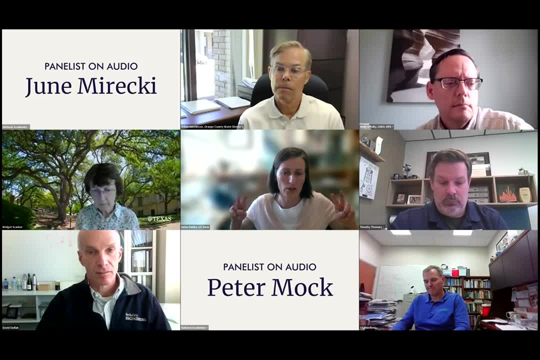 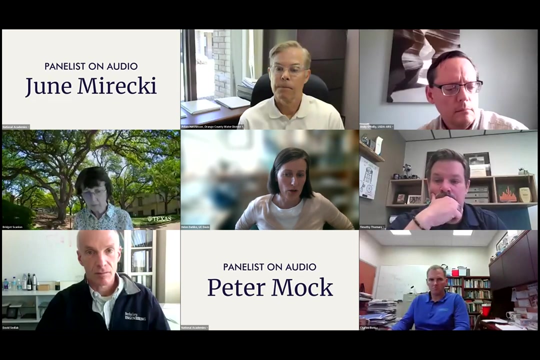 had high magnitude flows. the Delta was in so-called excess condition, meaning it met all the biological opinion criteria. And then, yeah, the 90th percentile is a criteria that is often also used to ensure that whatever surface water rights we have in downstream regions are met. Floodwaters are the only. 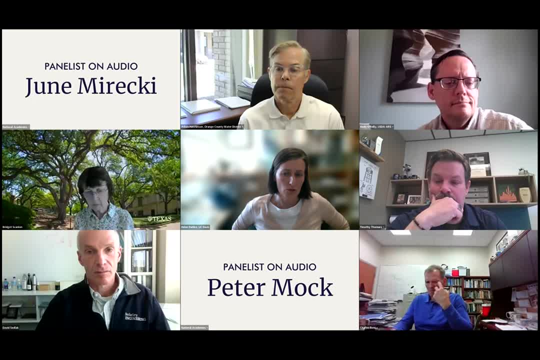 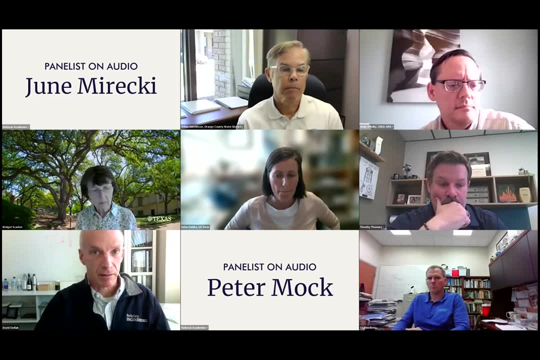 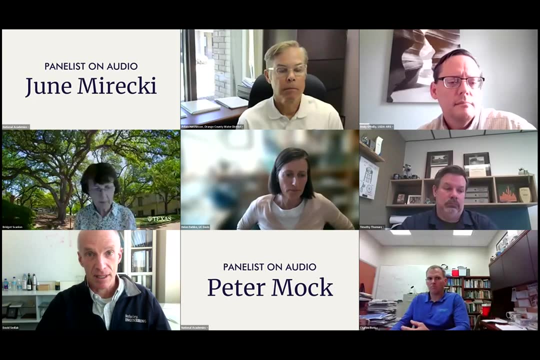 source we've left in California, So most normal surface water is already allocated. Yeah, I wonder if this issue is getting. it's certainly getting attention in California, but in the South Platte River, for example, or the Mississippi River, it seems like it's not something. historically people have been. 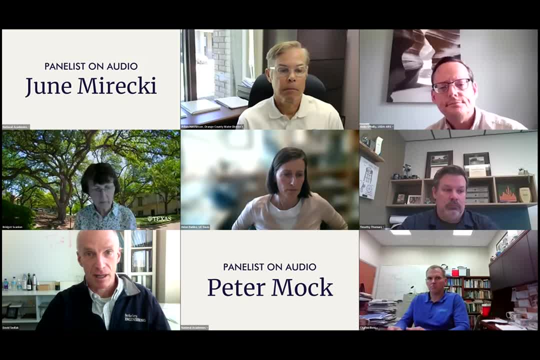 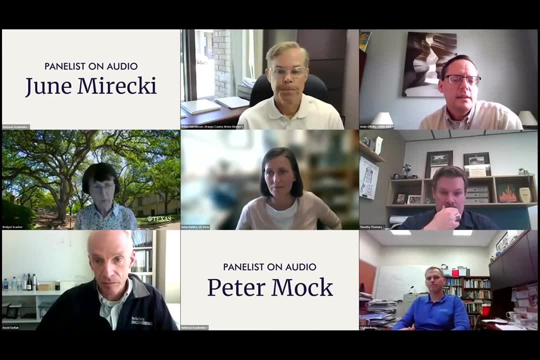 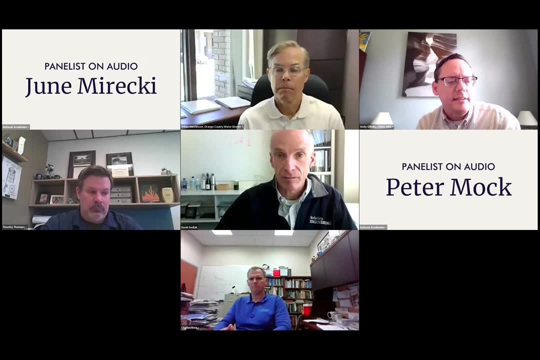 thinking about quite as much, and it would be nice for us to discuss or at least have an opinion about it. Yeah, I'll make a couple of comments about Mississippi. I think that's of course. we're still just in the pilot phase, but any larger implementation of this, I think that's you. 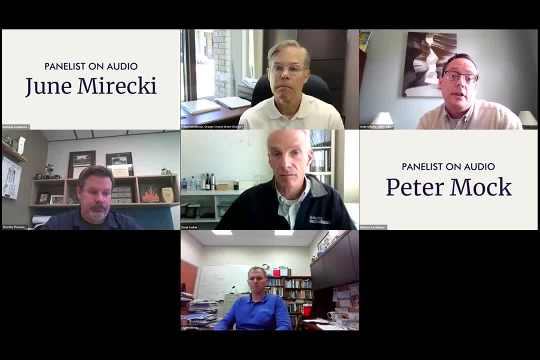 have to have some concern about impacting flows in the river. i mean the current pilot project at 1500 gallons per minute. that's about half a percent of the daily minimum flow. uh, daily minimum made flow in the river, uh, but you know, we might not need. 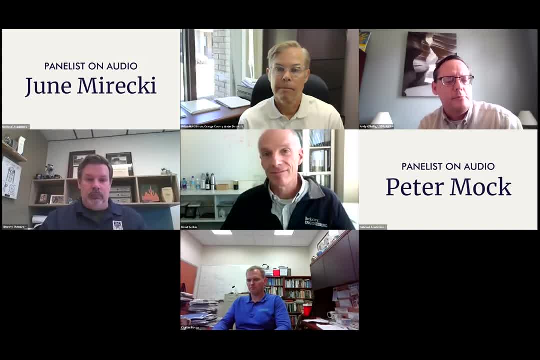 two injection wells. we might need 50 or 100 for a bigger scale implementation. uh, the other thing that's very interesting is um, the greatest drawdowns are in the central part of the delta, mississippi, uh, and the talented river is kind of on the east side of that, so it's not really 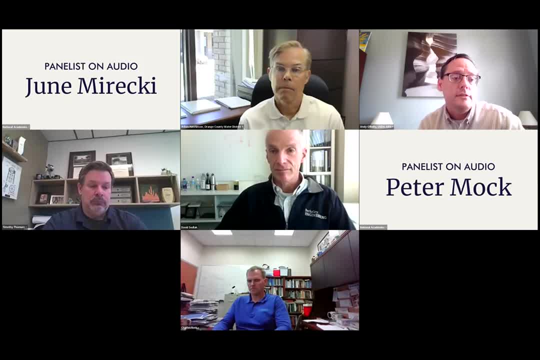 located in the the area of greatest drawdown. but rivers that do flow through that area of greatest drawdown have had major impacts on uh low flow. so if the idea of transferring that water and injecting it in the areas of greatest depletion would would help mitigate that to some degree. 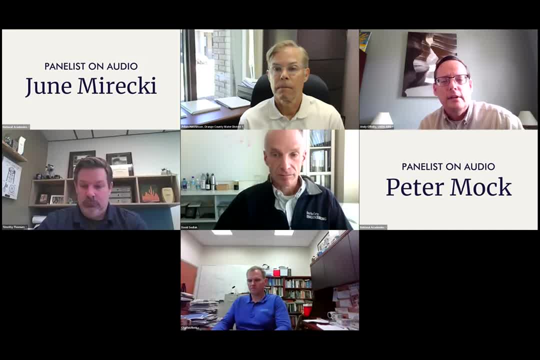 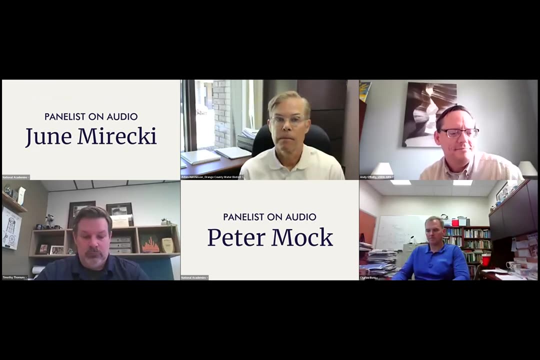 by rise, raising the water levels, and it might actually improve low flows in those rivers. all right, great response. uh, andy, while while we've got your attention, i noticed i was quite impressed by the number of monitor wells you have in your pilot. could you tell us a bit more about? 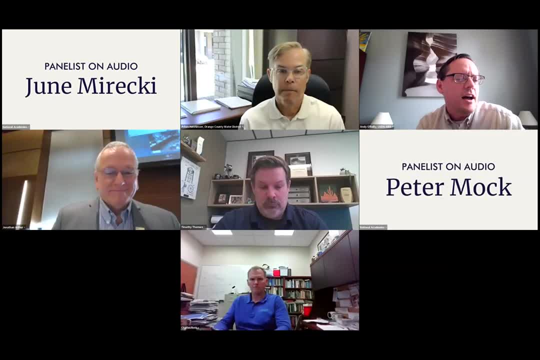 that. uh, yeah, there's um. well, first off, i'm a relative newcomer to the project. i wasn't involved in the design uh and building the system, but, um, it certainly has been helpful um to have a large number of monitor, wells, of course, it has challenges of of me maintaining that data. 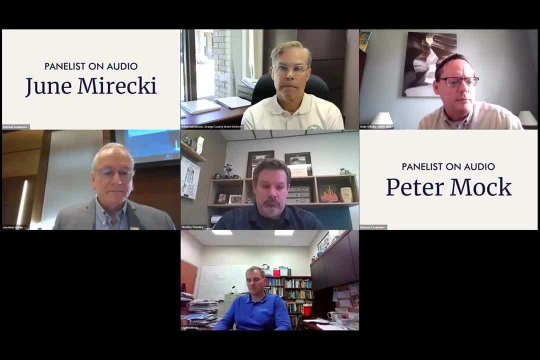 um and uh um, but i'm not thinking was number one. part of the reason for the large number is there really isn't a lot of groundwater monitoring done in the delta, mississippi. there has been for decades a twice a year uh potential metric map done in the delta. that's just been a fall and spring as far as 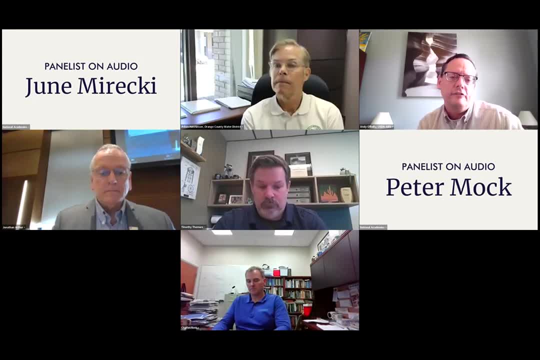 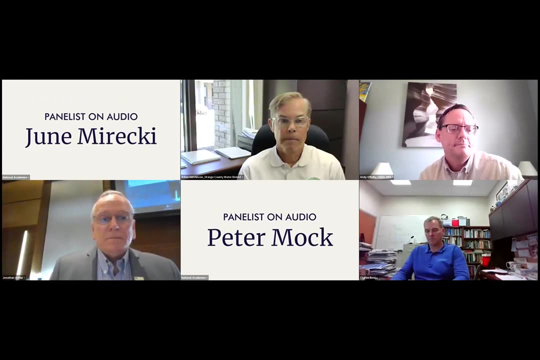 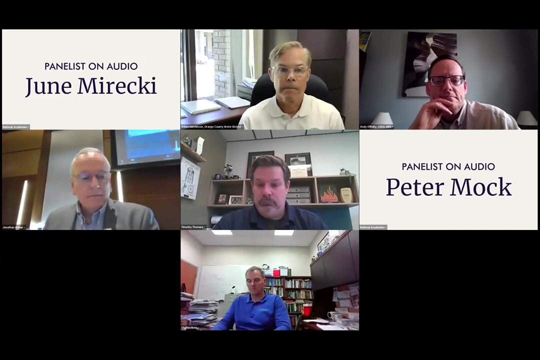 monitoring continuous water levels. there's very, very few of those of that data, um, in fact, we probably have most of it now and just for this, this project, all right, thanks, i'm scanning the screen for other hands up. uh, did you okay? oh, bill alley is next, and then bridget. 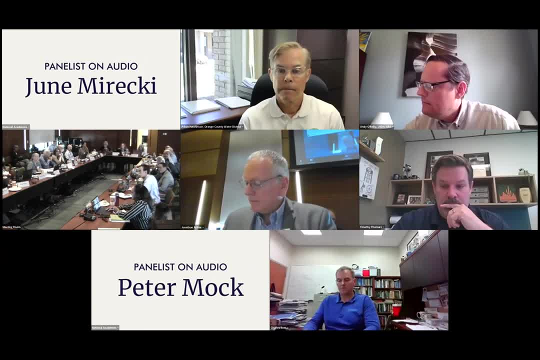 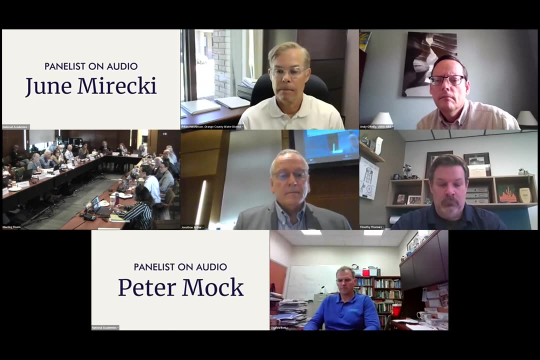 speaking. okay, thank you. uh, back to david sidlock's question. um, so, the example i gave in aurora. well, first of all, the map i showed for palatable reuse, you probably noticed that all those, most of the sites, were on the coast. so, uh, particularly in the west. um, the the one in aurora is interesting. 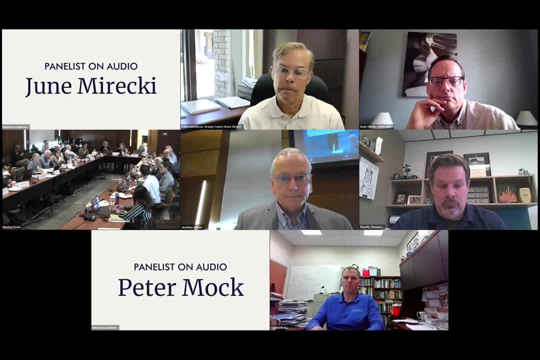 in the sense that aurora, like many communities along the front range, actually gets some of its water from the colorado river basin and from the arkansas river basin- and that's where we get water- And so that's transported over to the South Platte River Basin. 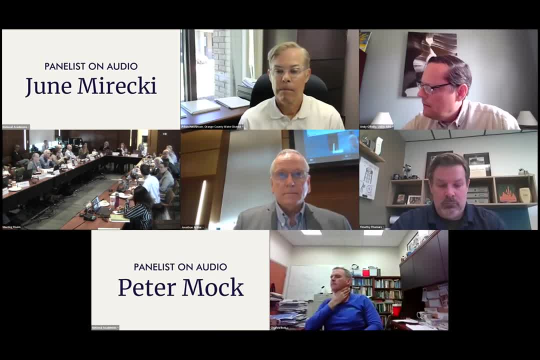 And so they actually can use that water to extinction because it's lost its connection to those particular basins. But the water in the South Platte is already over allocated And so they have to let that water. they're not treating that water they're treating. 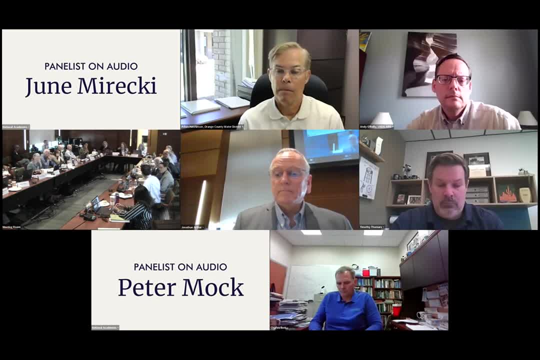 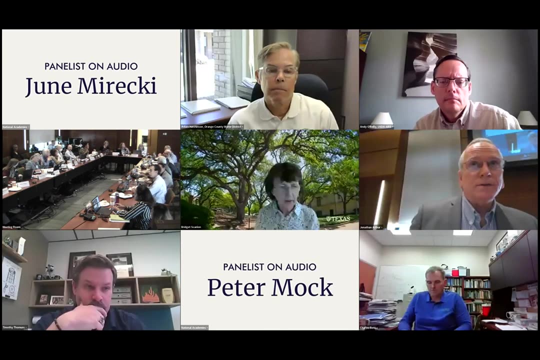 not molecule by molecule, but they're tracking very carefully the water that they get from interbasin transfer and that's what they're using for potable reuse. And Bridget, did you have a question? Yeah, I was just wondering if any of the people developing these projects has looked at the 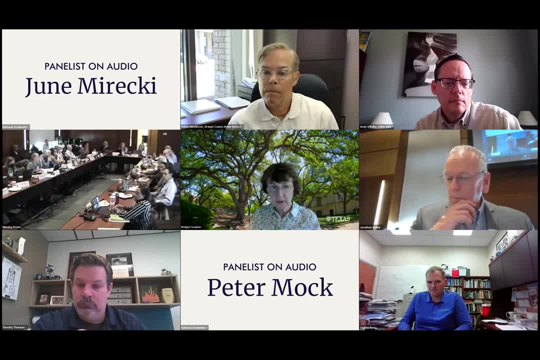 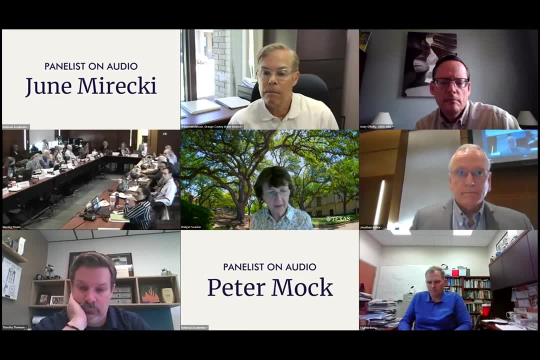 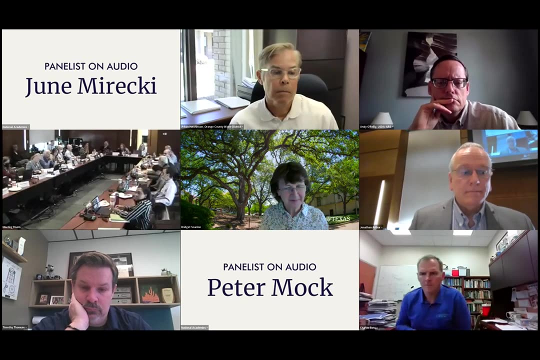 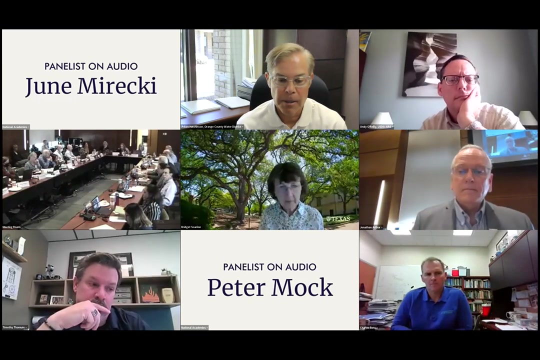 energy implications of different management scenarios and if they quantify greenhouse gas emissions or other things, or that was if anybody has thought about that. Yeah, I'll mention something Orange County has done So, as I mentioned, imported water is a big part of our supply- 25%- but that requires 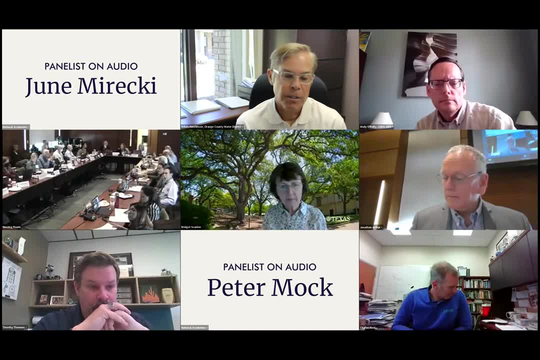 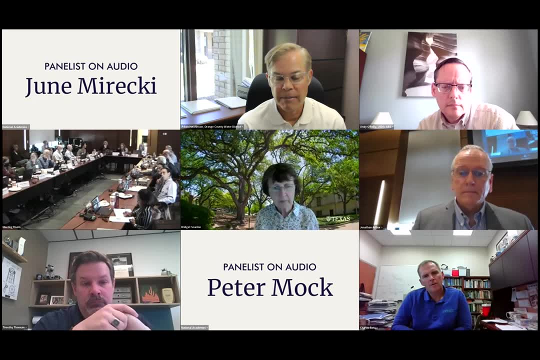 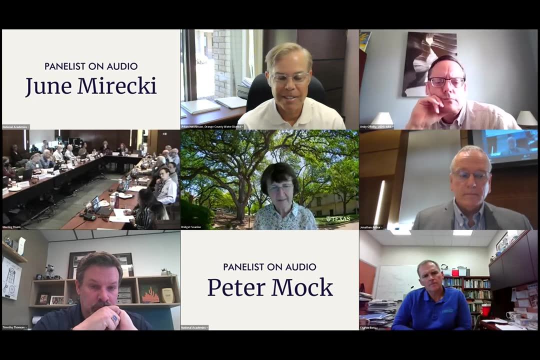 a lot of energy to move that water to Southern California. So we've done calculations to show that our stormwater capture efforts locally present a huge savings in energy And greenhouse gas emissions. So another driver in addition to water supply resiliency, just another benefit of trying. 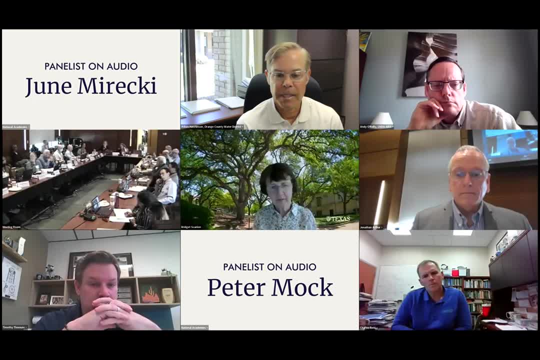 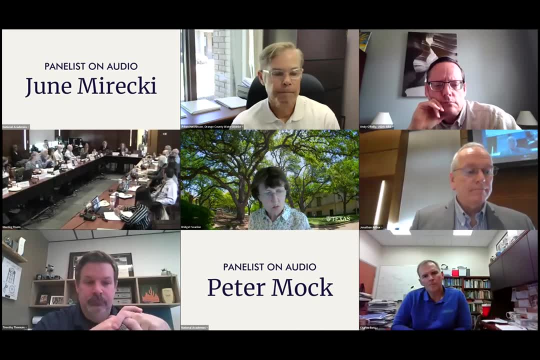 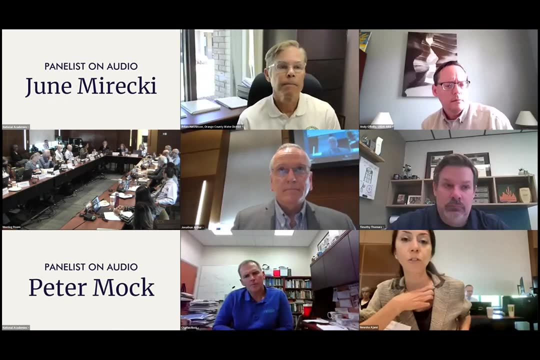 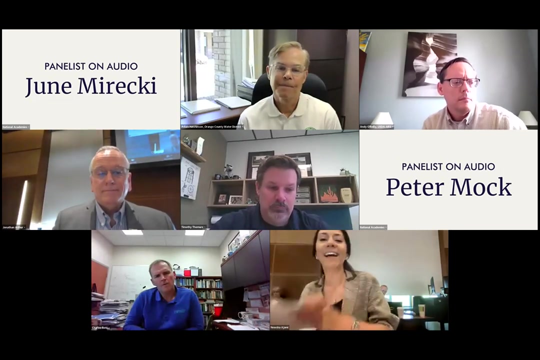 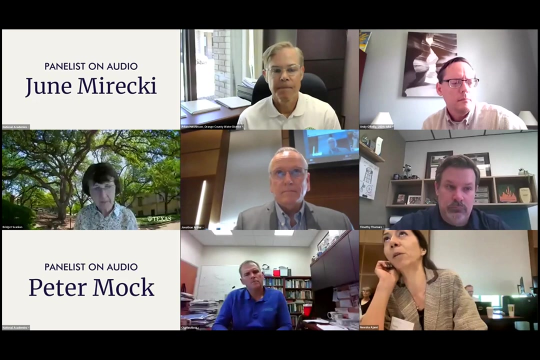 to maximize local capture of stormwater from an energy standpoint. Thanks, That's very interesting Just before I ask my question. one comment on your question, Bridget. sorry is that these are not wholesome answers, just because, even though maybe Orange County is not getting that water from Metropolitan that uses a lot of energy, that water does. 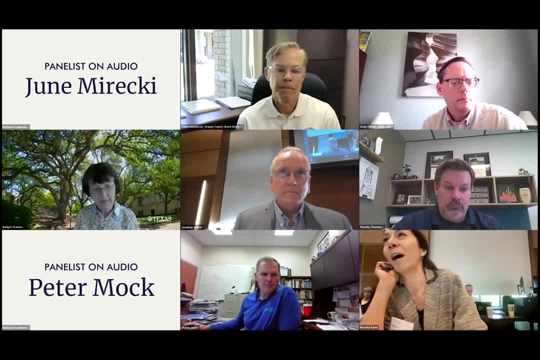 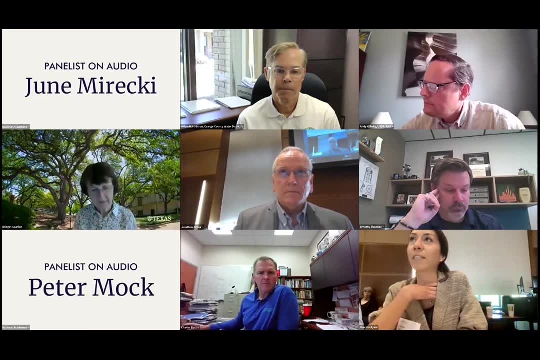 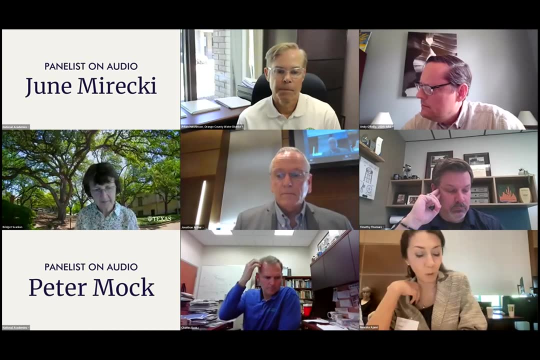 get transferred to Southern California and sold to others. So as a whole we are not really gaining. but Orange County is obviously, as a service area, is trying to reduce its greenhouse gas emissions. Yeah, So definitely not. So simply, specifically, we're not really seeing any éclairages from the offshore emissions. 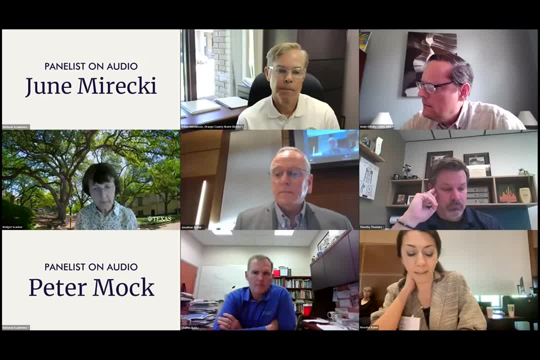 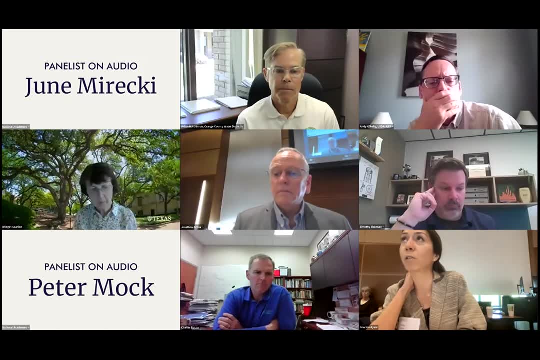 Just a followup to what David said. like is the regulatory requirement for the utilities, or waste water utilities- that are on the coast is very specific. So when you start reusing and recycling water, then you have less water that needs to be put back to the environment. 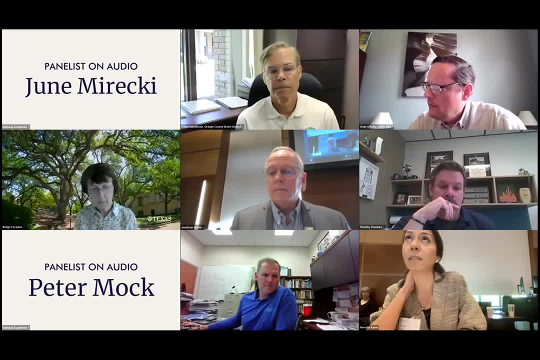 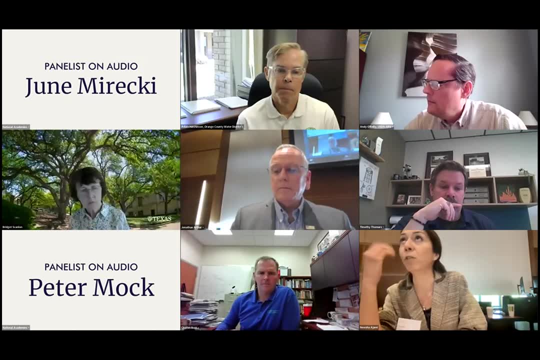 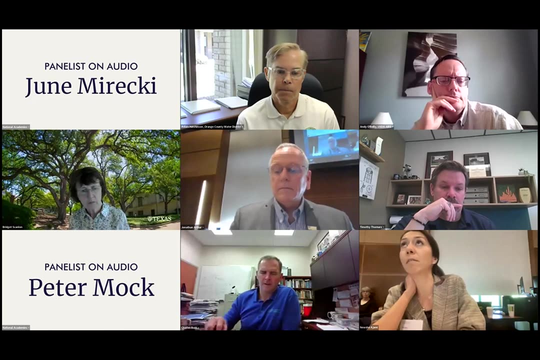 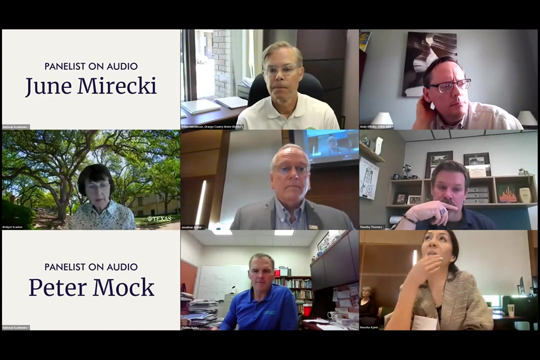 also the quality of that is lower. So I wonder, how does that- those regulatory requirements- impacting some of you that are in the coastal region, So basically trying to meet the EPA requirements on your outflows? I can answer that question very definitely. You know we've done a lot of work. 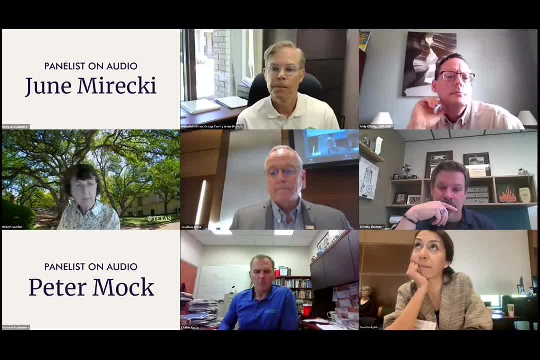 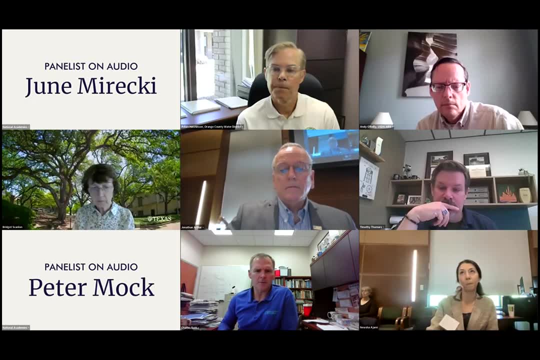 in this regard. So to give some perspective, you know we have right now seven- actually six- treatment plants bubbled together with a mass load allocation for total nitrogen and phosphorus And we can choose how we divvy that up, but that mass load allocation is headed steady down and has been. 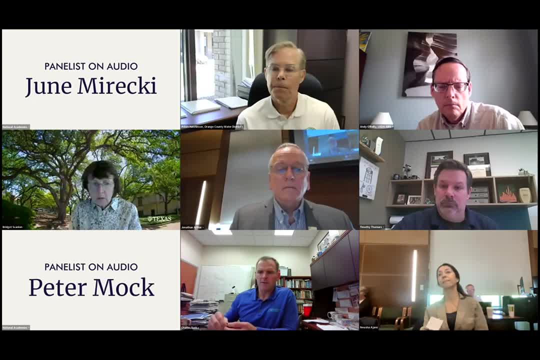 for a long time. And but we have flexibility, you know, to treat nitrogen and phosphorus, for example, at plants where it's least expensive to treat it, And we take advantage of that. Soon we won't be able to take advantage of that, basically because the limit will be so low. 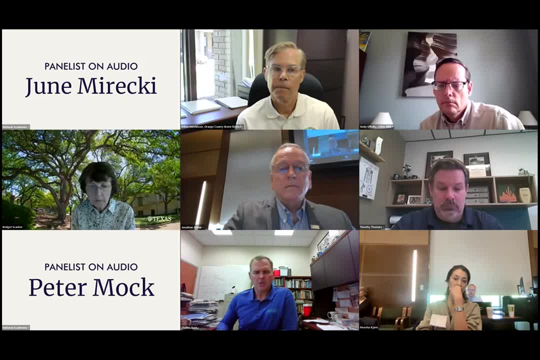 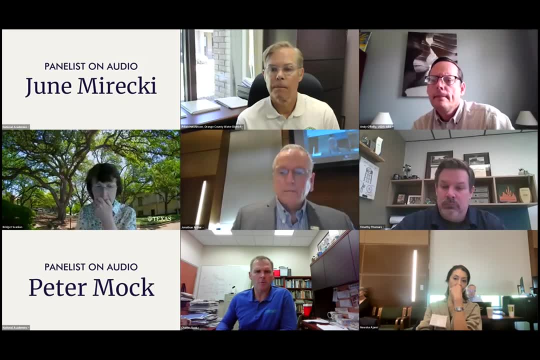 But what we, what we have done, is that that allocation is is will eventually, in the future, be based on our treated flow. So the flow that comes in the front door of the wastewater plant would be the basis of the allocation, So we can take advantage of the of the recharge that goes. 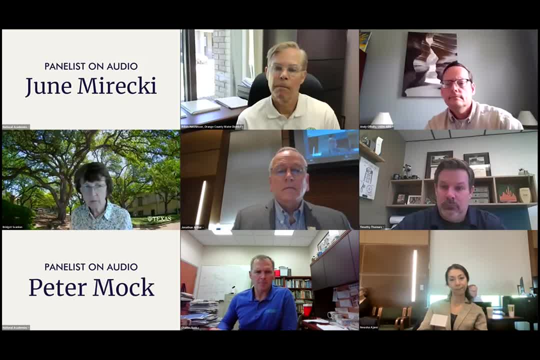 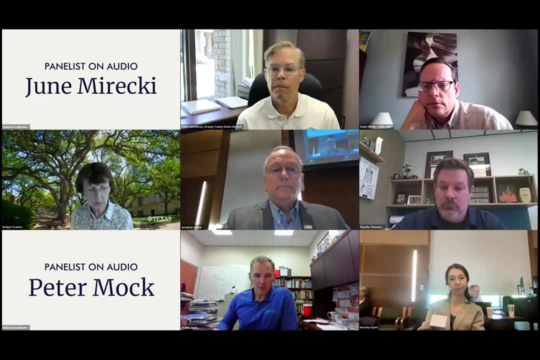 in the ground. So so one limit will be based on the flow that comes into the plant, And we can. we can benefit then from managed aquifer recharge, But we still have concentration basin based limits to deal with. So annual average concentration. 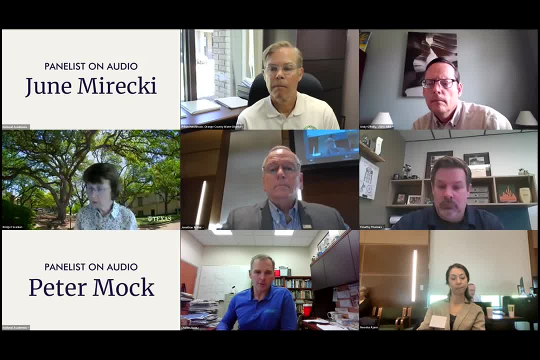 based limits still exist and afford nitrogen and phosphorus that is. And we still have, of course, BOD and TSS limits and ammonia limits and pH requirements and, you know, disinfection requirements and bacterial requirements. So we have all the same permit requirements. 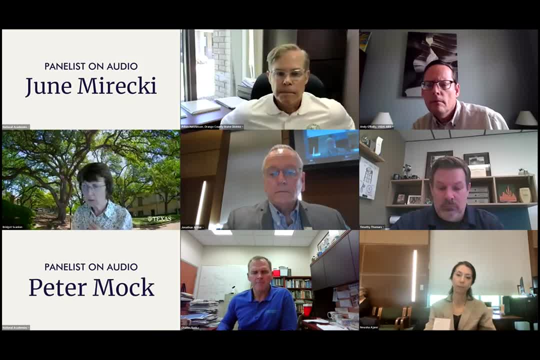 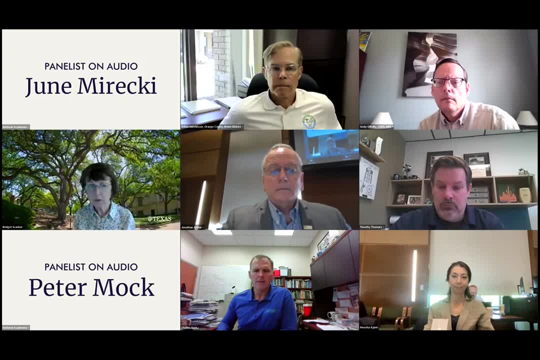 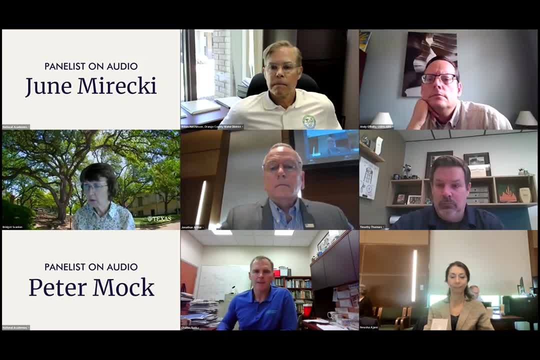 a concern that we have to manage really carefully. And yeah, and we have a lot of- I mean a large portion of the capital upgrades for these plants- is figuring out how to integrate well the wastewater plant and the advanced treatment facility to ensure we always have appropriate 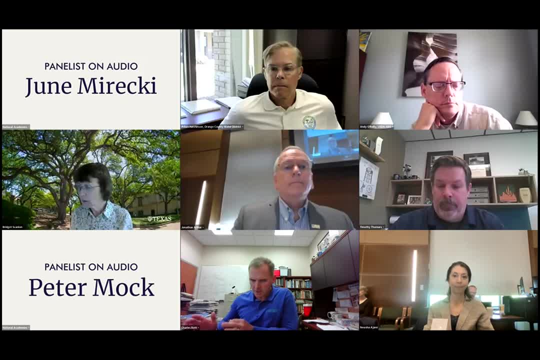 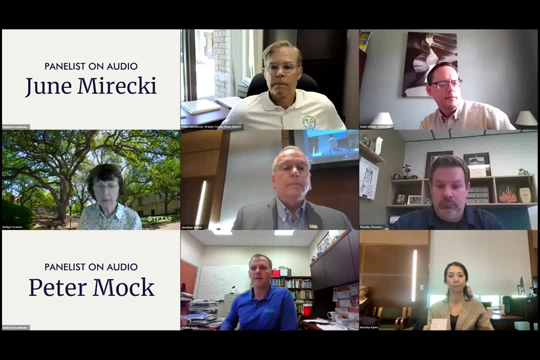 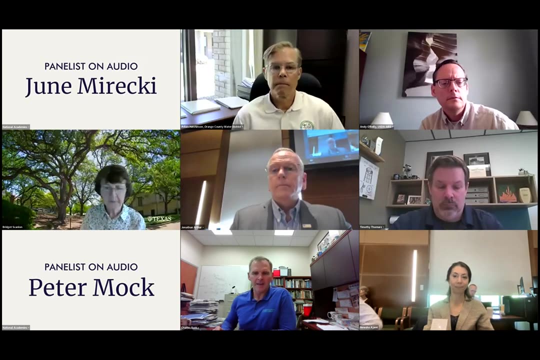 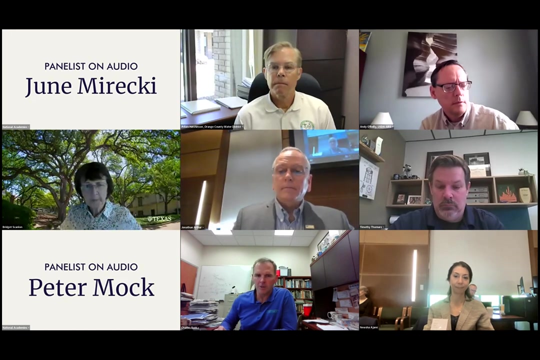 water quality at the outfall, in addition to the much harder actually is the water quality at the recharge wells. So it's a great question and it's one that that practically, I would say we've spent probably more time dealing with those questions That we have around the design of this with advanced treatment facilities, because we know what they need to be. we know what those facilities need to be. it's the integration between the two that's really challenging, great question. 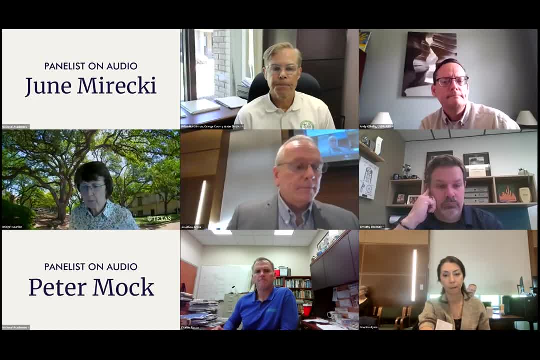 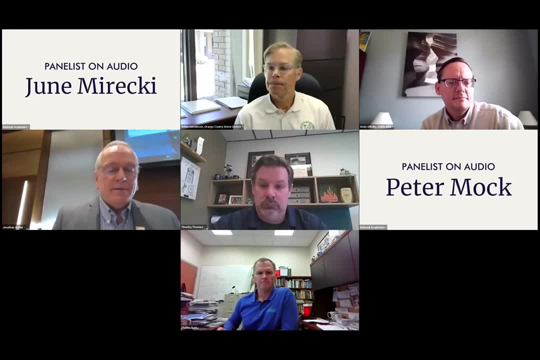 Nelia, did you have another up up? okay, okay, well, a question. I have a question for those working with ecosystem restoration That have that aspect to their, their projects. what is the greatest success and also the greatest challenge you have in terms of water compatibility issues- putting water back into the natural system? 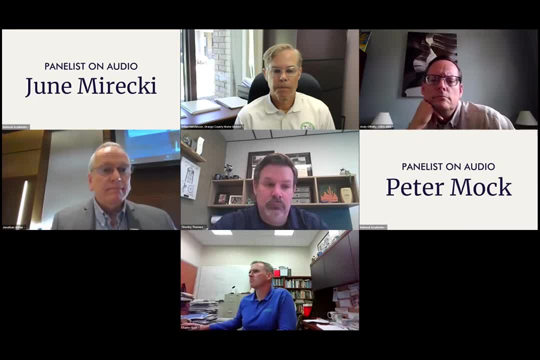 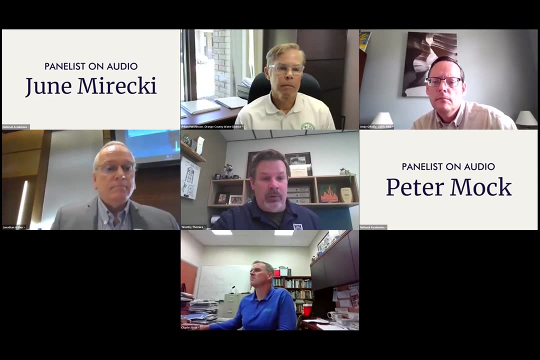 I think that's a really good question. I can. I can start When In our environment it's pretty simple recipe: if you put water into the desert, things happen, and so when we did our Santa Cruz river heritage project, We there were some concerns about emerging contaminants or P fast chemicals or things. 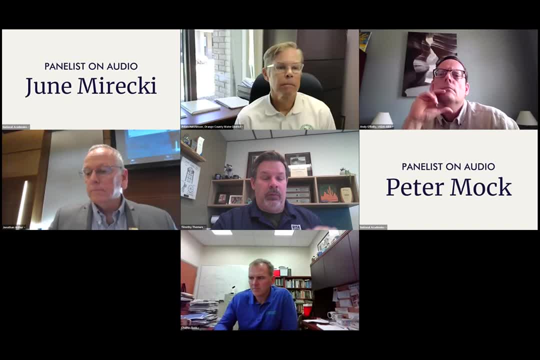 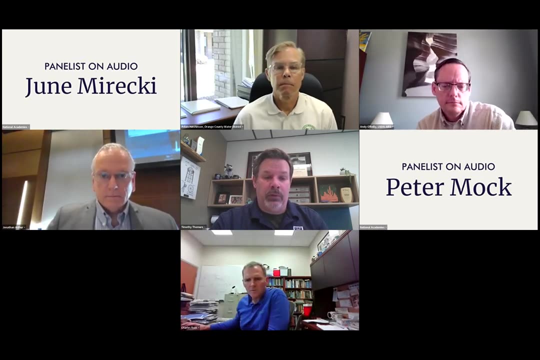 Of that nature. Luckily or unluckily, some of our the groundwater, shallow groundwater under our major river courses already been impacted by by things of that nature and the recycled water that we're discharging is is very low and in those constituents are very high quality. 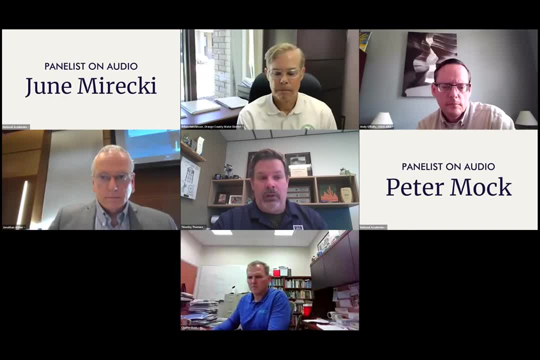 So it actually is a net benefit to the aquifer from both the quantity and equality perspective. when it comes to the riparian habitat itself, we saw Literally overnight impact from opening up that outfall. there's a local researcher to Michael bogan, who's a biologist. 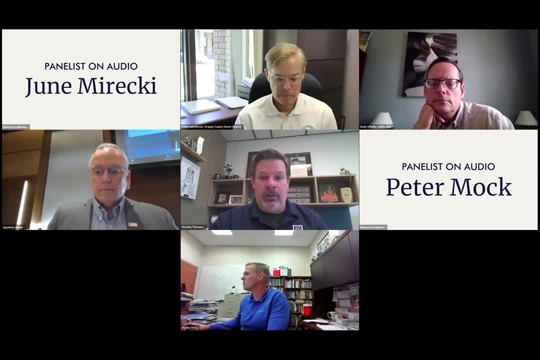 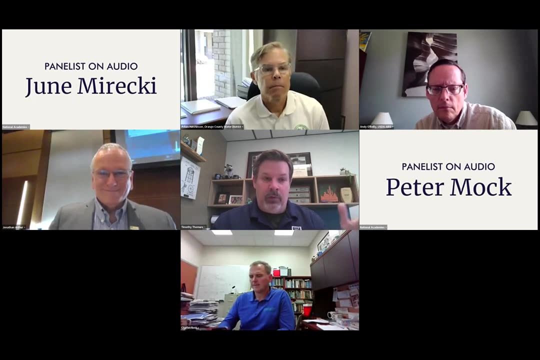 who immediately came out and started. the first thing he noticed was dragonflies, you know. so we're going from a dry river channel, literally sand and gravel. he started noticing dragonflies and dozens of species of dragonflies. I learned more about dragonflies in the first month and I ever thought was to know. 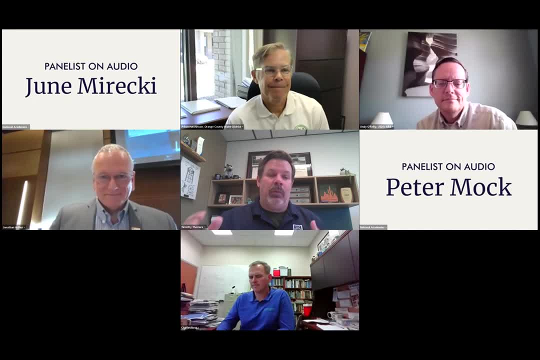 But We we, within several months we were able to actually work with fish and wildlife under safe harbor agreement to reintroduce The endangered Gila top minnow fish to that stretch of the river for the first time in 70 years. so it literally was an overnight transformation of that. 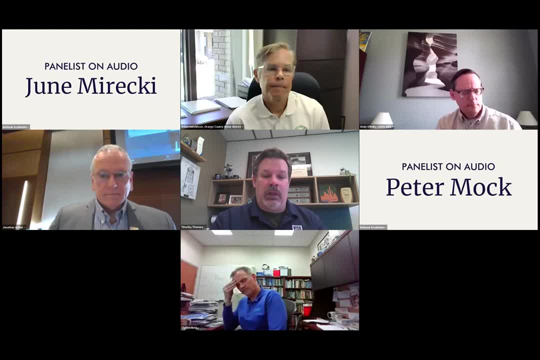 area, from a dry Baron dry river channel to a thriving riparian environment, and now we have to take good care of it. we have to manage, you have to keep the flows continuous, But water quality was not an impediment to any of those activities, including the environment. 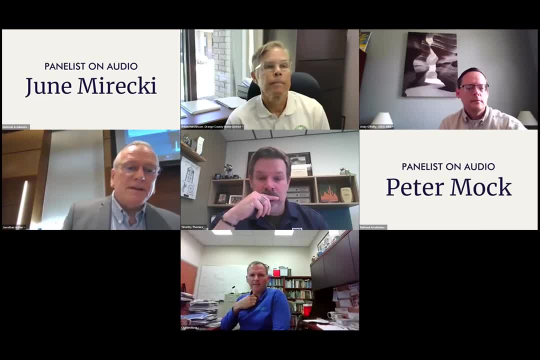 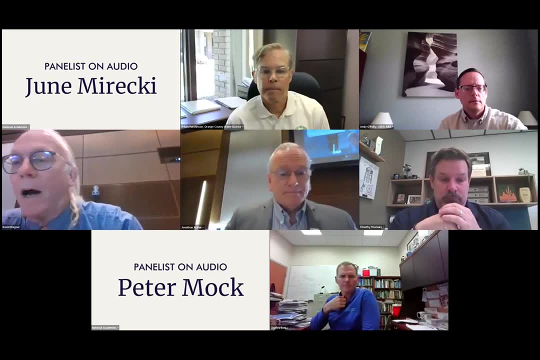 Thanks, TIM. Great story, yes, David wagon. Thanks. first off, I want to thank all of our speakers today. you've done a great job in kind of laying out the issues. my question is kind of broad ranging and I don't know if there's any one of you can approach it, but 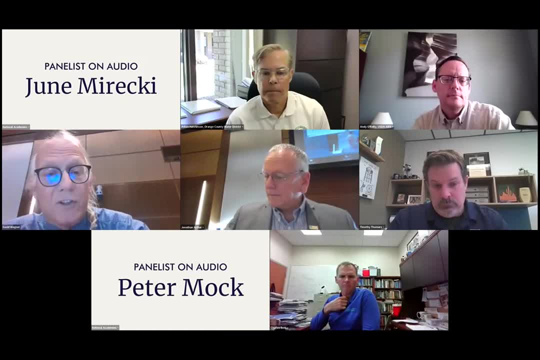 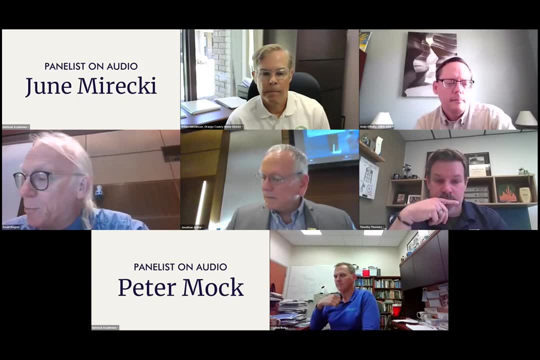 I want to throw it out there anyway. we in some of our is like Adam, you've clearly have a long history in using aquifer management, groundwater management etc. and also we've heard there are some new pilot studies that are just kind of gathering the data. as it is, I guess my question is: 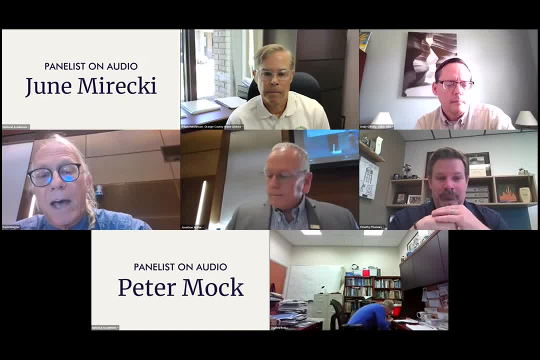 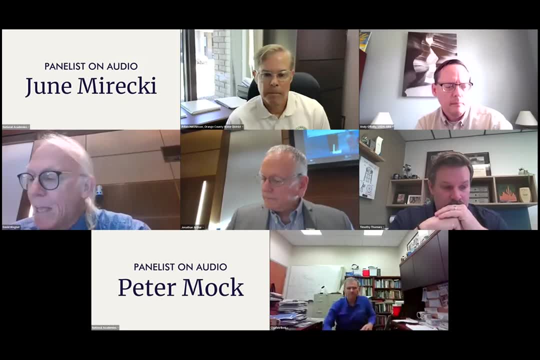 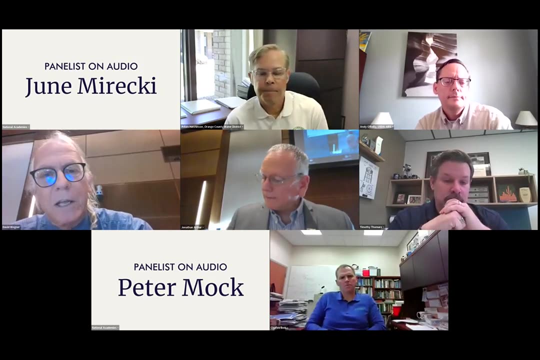 Where are the areas of research that are are needed to help move this along even further? is it water quality related? would that help? Is it the cost part of this in terms of gathering and reinjection? is there technologies that could be enhanced there, or is it regulatory? and i'm just. I want to get a sense of where. where can we help this initiative move along in the process? 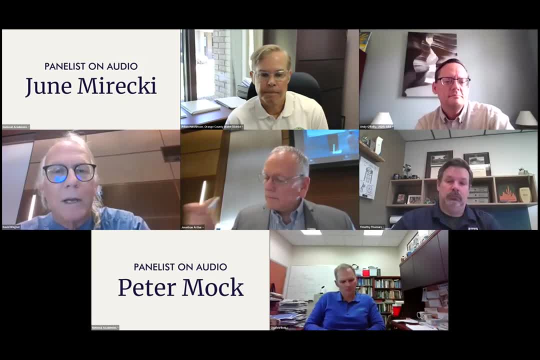 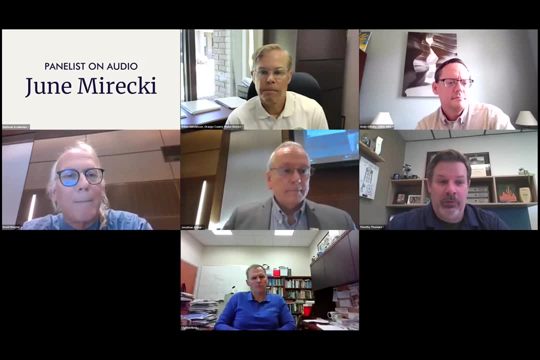 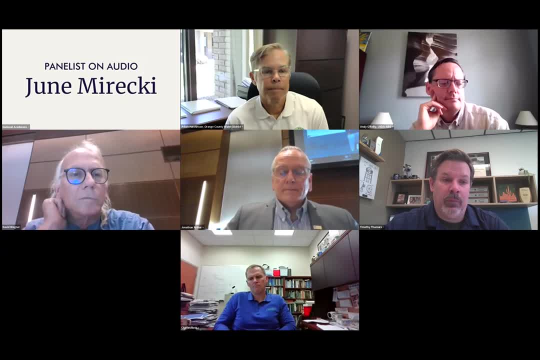 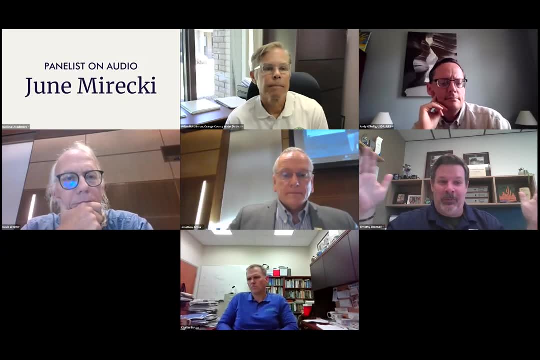 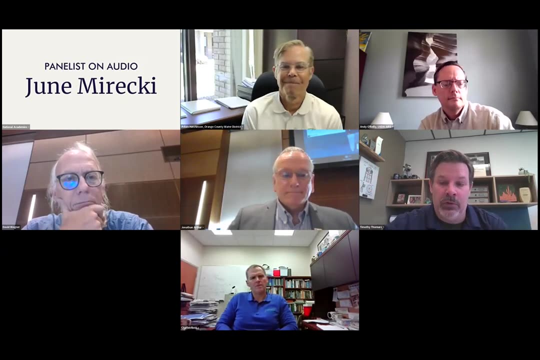 So I i'll leap to direct potable reuse, which managed aquifer recharge is, And potable reuse has a spectrum from indirect or de facto to direct. i'm not going to split hairs over how direct is direct, but in cases where recharge is a part of a, 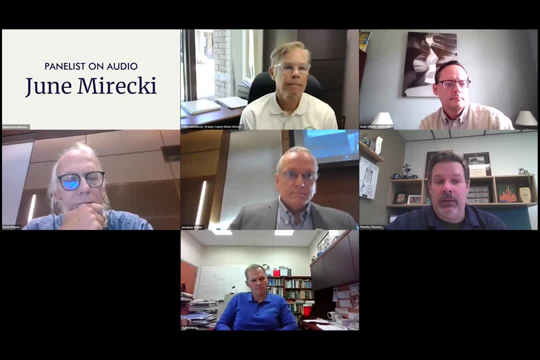 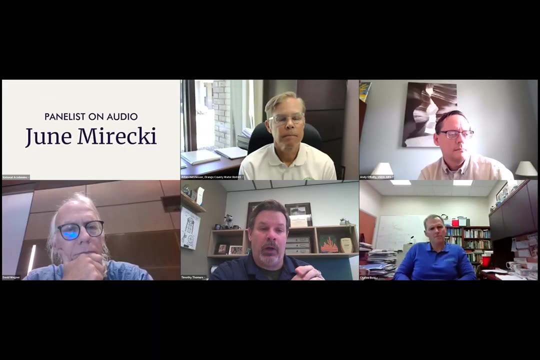 Potable reuse Scheme, Especially in inland areas. An area for research is In a coastal area. there seems to be A reliant- not always so more on the west coast- a reliance on reverse osmosis, Brian, creating a brine. that's part of your stream, that sometimes recapture, but there's still ultimately this, this waste product you have to deal with, whereas in in non RO treatment schemes, schemes 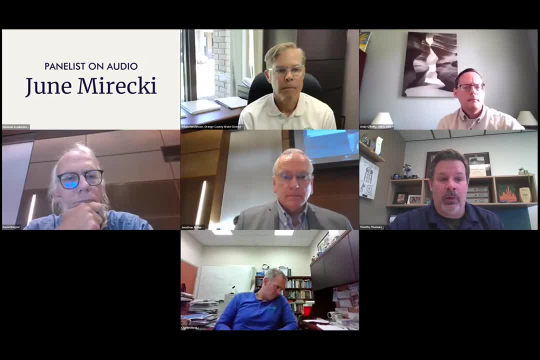 Often you can avoid, avoid. Often you can avoid, Avoid that brine and that loss of water. but it's it's a it's a newer approach to things and not as well studied as the full advanced treatment with reverse osmosis. so I would say from an inland perspective, 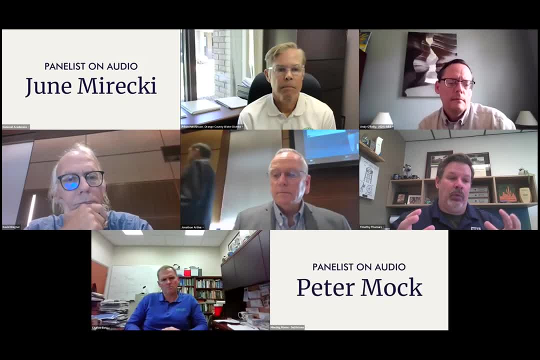 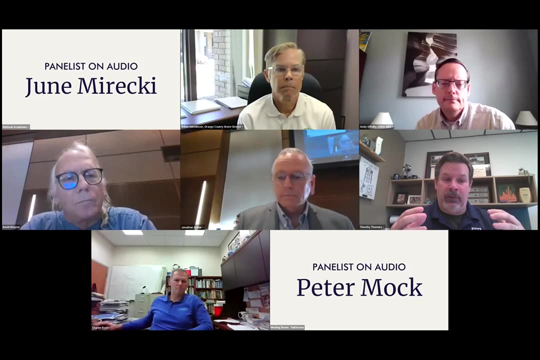 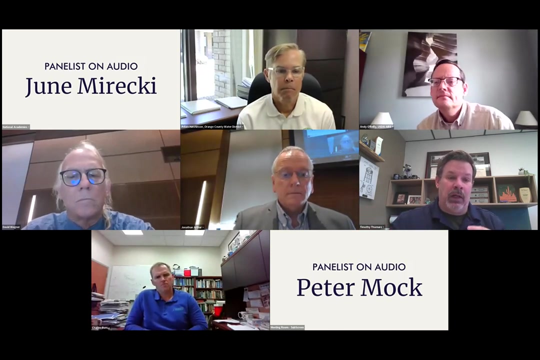 The role of recharge in that overall approach to potable reuse and how, from a regulatory and from water quality perspective, What are the acceptable treatment trains for portable reuse That we can have a high degree of confidence in and not say Adam's train is better than Charles's train or anything of that nature, because every geography, every situation is a little bit different- different opportunities, different challenges. and research into how to do that all well and not have a value between different approaches, I think would be helpful. 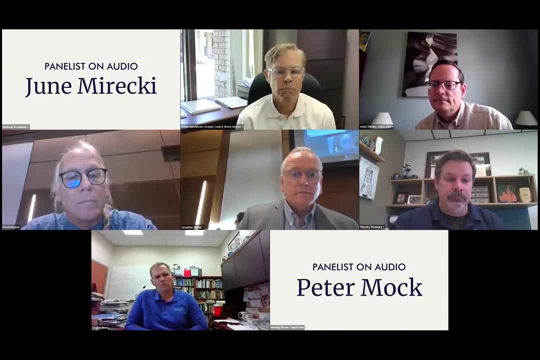 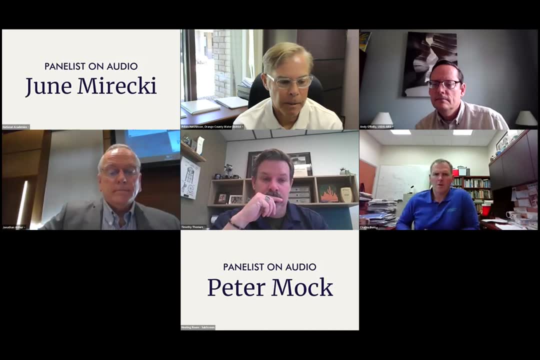 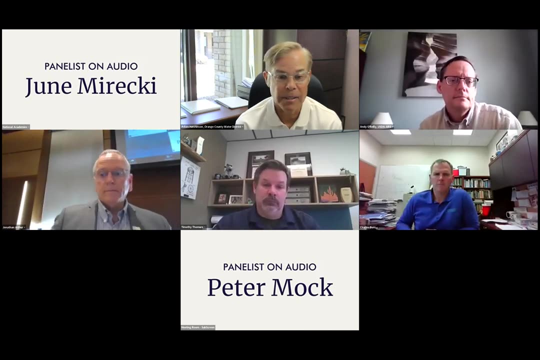 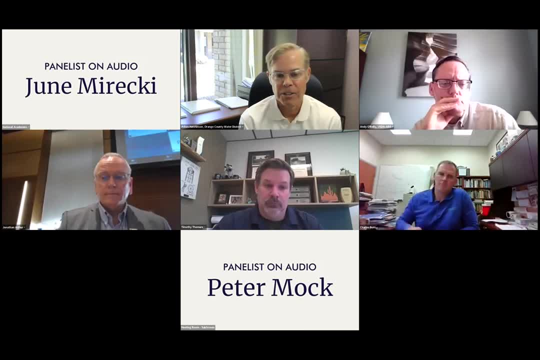 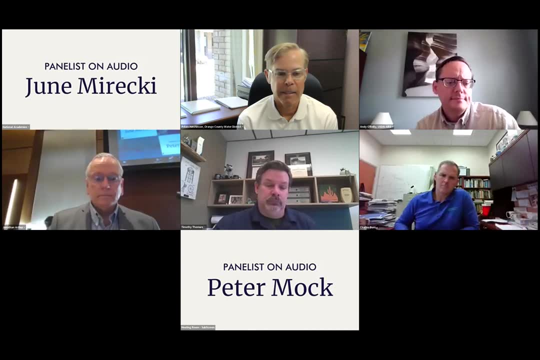 So I think one of the values you're going to this can provide it: just connecting people and getting people talking, because there's a lot of expertise, a lot of knowledge out there but if we don't know, it exists, Not available to us. 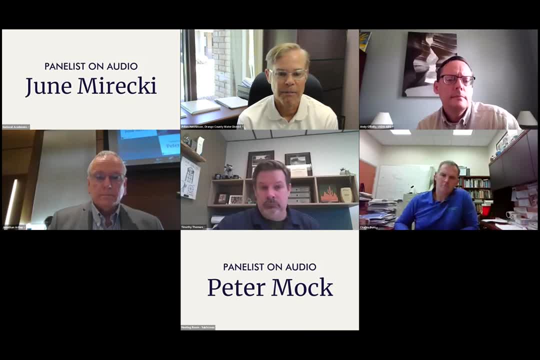 So I think really doing what you're doing here is very valuable to connecting all these people and getting the research and practitioners connected with one very helpful. This is Charles, you know. I guess I'll give one opinion that that in the, in the scheme of indirect portable reuse, the topic of pathogens rarely comes up, it seems, anymore. 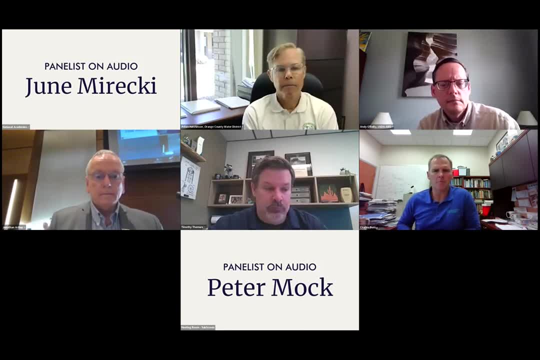 I know that's different in direct portable reuse, and the topic of pathogen removal is still right and shiny, But in in indirect portable reuse and managed aquifer recharge, really the emphasis is all on emerging contaminants by stakeholders. and And that then brings the question is: you know, of course, what's, what's appropriate, what's not. 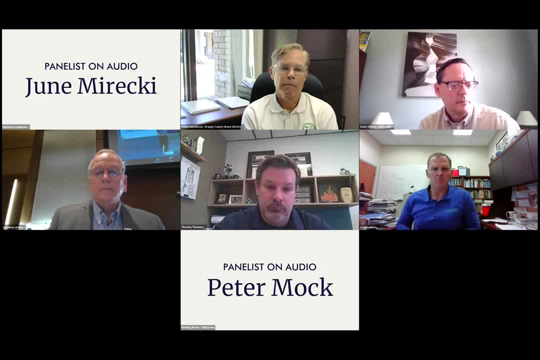 And and and and then goes to to see which is really measuring. you know bulk organics, And and and and. then goes to to see which is really measuring. you know bulk organics And not emerging contaminants. and you know the range of requirements for TOC is is tremendous out there. 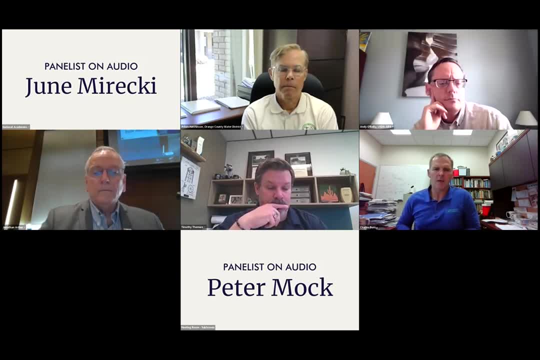 And and and. then goes to to see which is really measuring, you know, bulk organics. And and and and and. then goes to to see which is really measuring, you know, bulk organics In cases where reverse osmosis is not being employed. 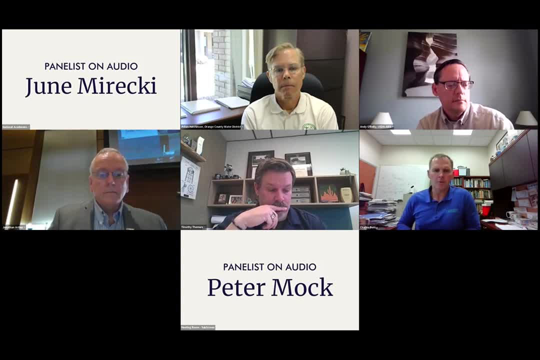 So so what's what, for a given circumstances, is appropriate or not appropriate in terms of bulk organics, and what's appropriate- not appropriate in terms of emerging contaminants is: is really a hard one to deal with. is really a hard one to to deal with. 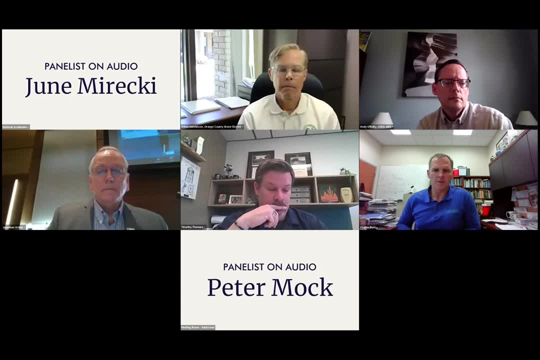 What we're seeing here, or you know lots of utilities because of the uncertainty And and of course you know bioassays and get at some of the problem and non targeted analysis, you know, kind of makes things even more complicated, I think, at this point. But this issue of where, where things are going, 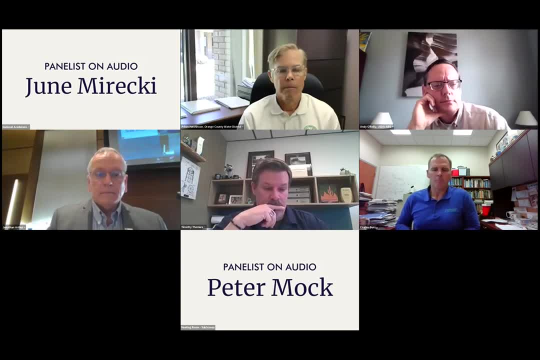 to go what's appropriate, what's not appropriate, And for and for there to be some some point of resolution on that, because you know those are the questions that come up. that's really where the question and concerns are from stakeholders right now. 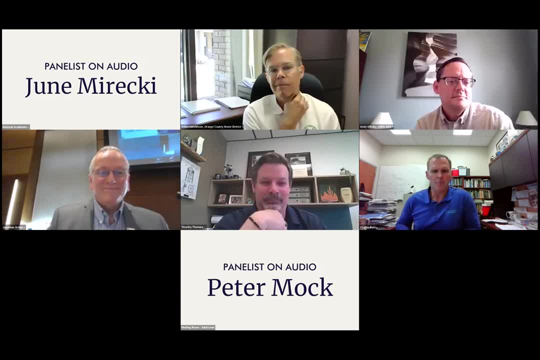 I don't know how to phrase that more succinctly or get at what the problem is, because I understand the nuance is tremendous And there's always things to talk about in this regard, But it just it seems like you know, it's it never. you know, there's always. there's always uncertainty and 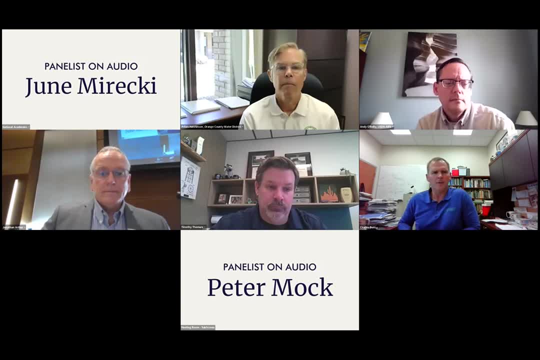 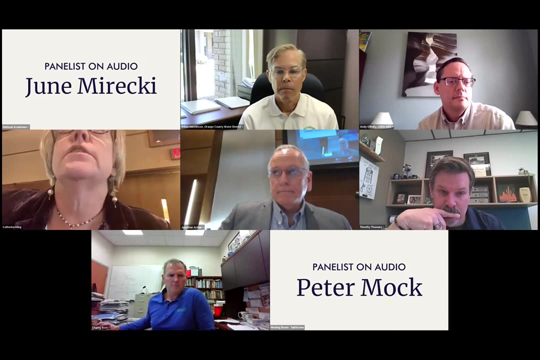 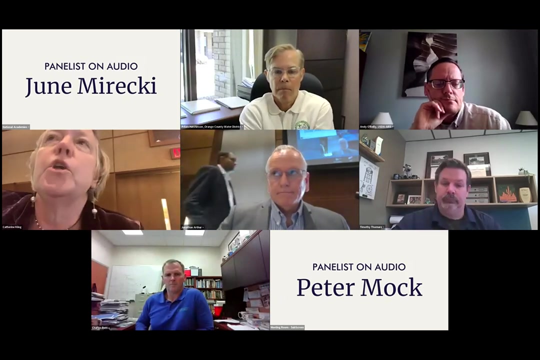 it's hard to get projects to move when, in the face of sort of unrelenting uncertainty. Great observation over to Kathy. Yeah, thanks. Just. that conversation was really interesting And made me want to ask each of you what, if any, public opinion issues do you do you face And how do you manage those communications. 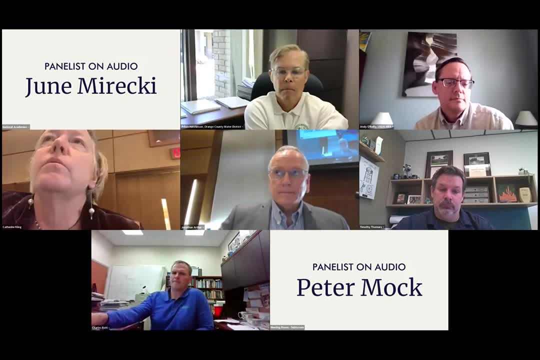 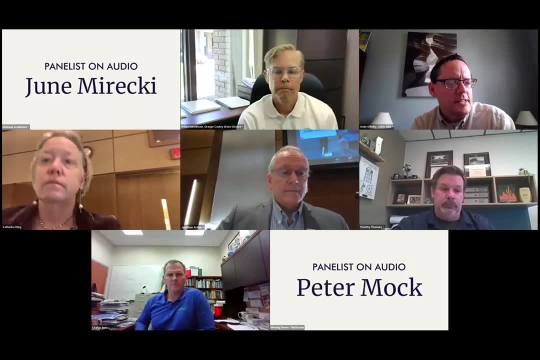 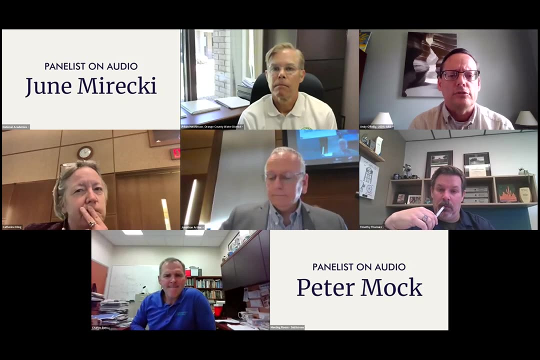 You know, is that a struggle? No problem, Just be interested in your comments. I guess I'll jump in As far as the Mississippi project, I mean, we're still in the pilot phases, of course, but and it's to serve the agricultural community, So it's really the producer end There's from. from the producer point of view, there's been a wide range of 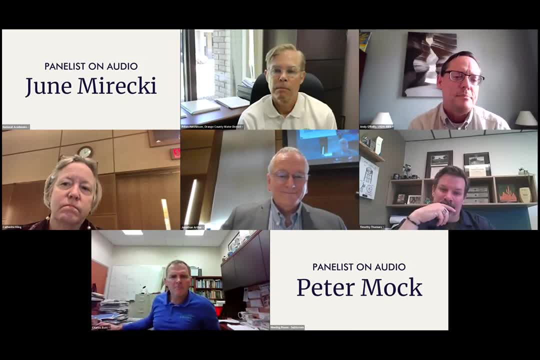 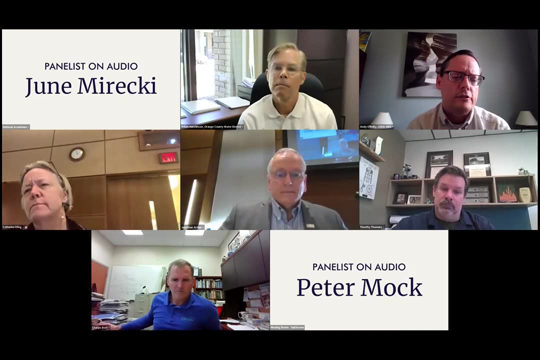 support or skepticism, as the case may be, of the project, And I think that goes toward a little bit toward the previous discussion. I think what Adam mentioned to just communication of information. I like I'm pretty sure this is the first and only managed aqua recharge project in the state of Mississippi.